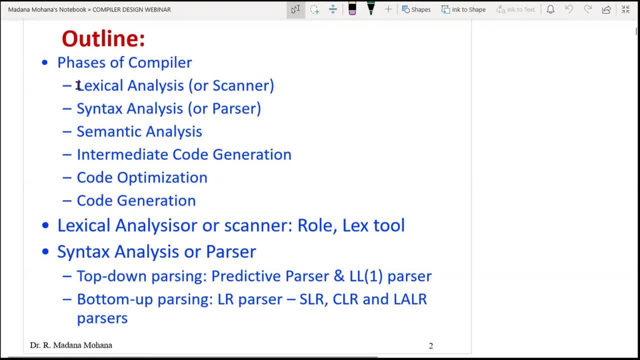 As you already know, In this series, briefly, we will review all the phases of the subject. One is called as electrical analysis, two is called syntax analysis, three is called semantic analysis, four is called square-to-shape code of integer and 5th is called 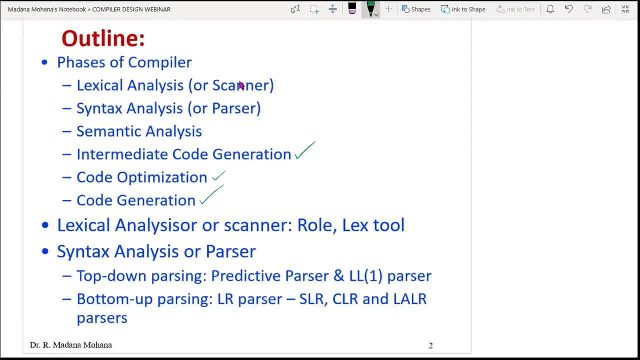 post assumption. The phase 1 is called R-type, So we will summarize here the diagram, followed by what is the input and output. after that we will discuss some more details about the next two, and later we will discuss about the second phase, tax analysis. 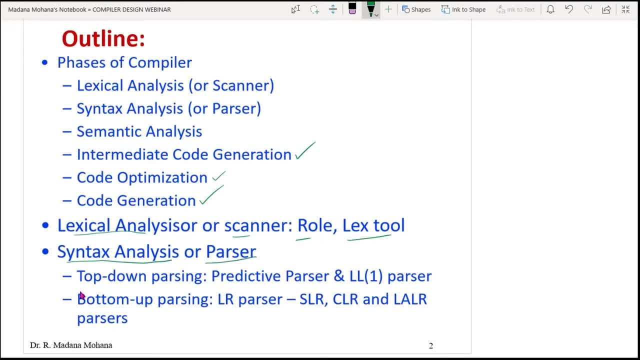 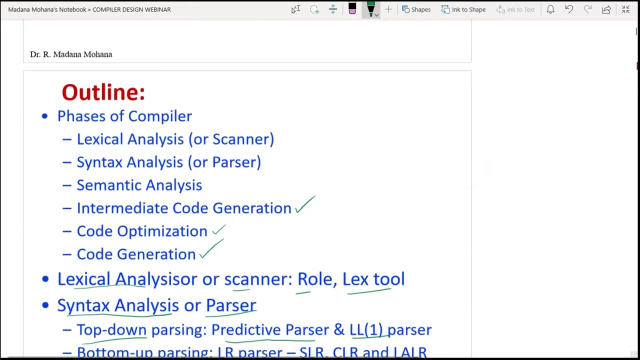 So there are few types of examination point of view. the parser- we are having three of them- address based on parsing and whatever parsing- we are having five of detail we will discuss end of this session. we can able to solve problem, so let us recall once the introductory concept definition. 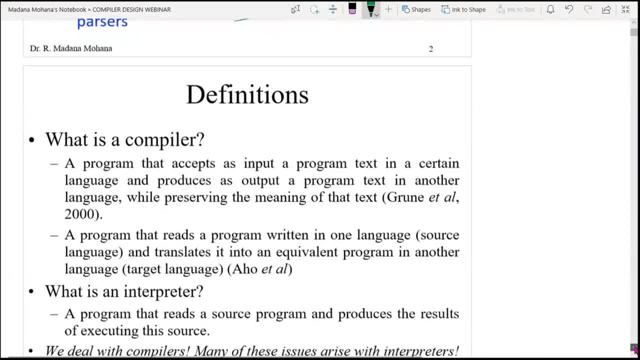 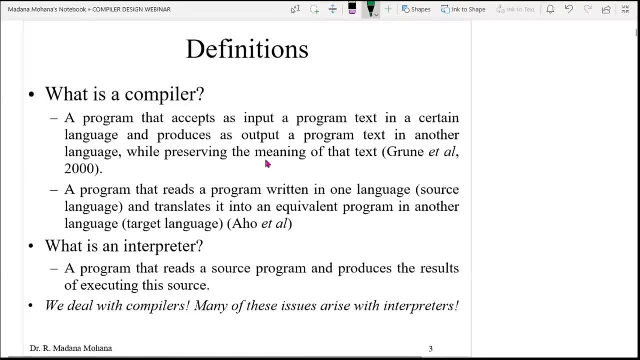 Correct. Excuse me, sir, Sir, your voice is very low. sir, Are you hearing now? So good morning sir. sorry to disturb sir. Now it is clear. So now it is clear, sir, but there are some disturbances in your network, sir. 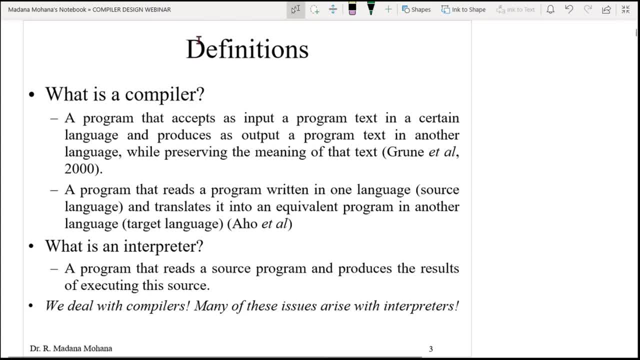 I mean some other sounds are interrupting this session, sir. Okay, sir, now it is clear, sir. Thank you, sir. Okay, sorry for the inconvenience. Let us move to the. what is a compiler? that everyone aware of the compiler. So, without knowing much about compiler, also indirectly, we are using that compiler. 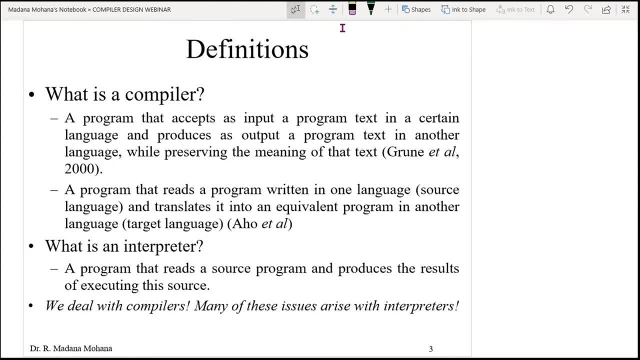 Okay, We are using the term compiler as a computer science student. So in first year you may studied C language and second year you may studied C++, Java, followed by various programming languages, So any programming language. whenever you are writing a program, what you have to do, as per the syntax of the respective programming language, you can write the program. 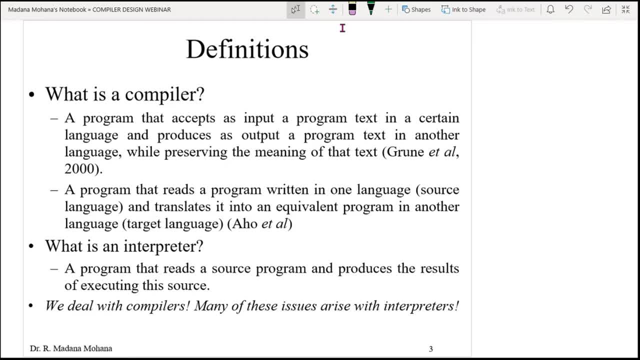 After completion of writing the program, what you have to do? You have to first compile the program term compile. So without compilation we cannot move ahead further. So what the compiler will do? Compiler will read the program and will check the syntax and also finds any errors are there? 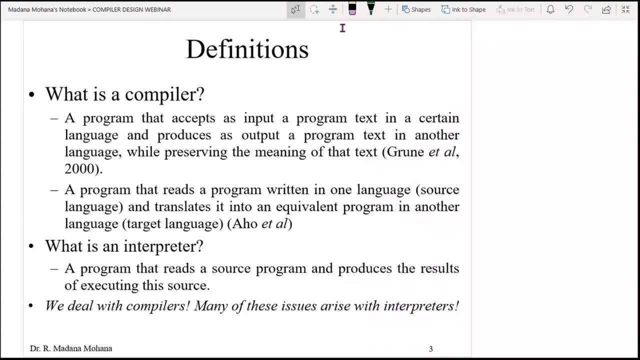 After rectifying all the errors, etc, the program is successfully compiled. So then That source program is converted into some other form. For example, if you will compile C program immediately after compilation, Let us see in your folder wherever you saved the program dot C. 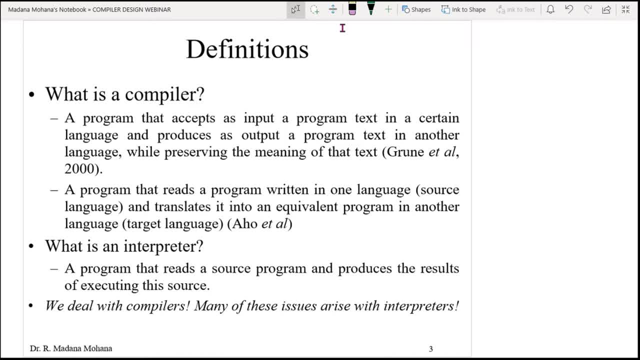 So then immediately after compilation- successful compilation- you will get some OBJ object file, dot OBJ. After compilation that object file is created. That means your source program is converted into some other form, So that can be done through compilation only. 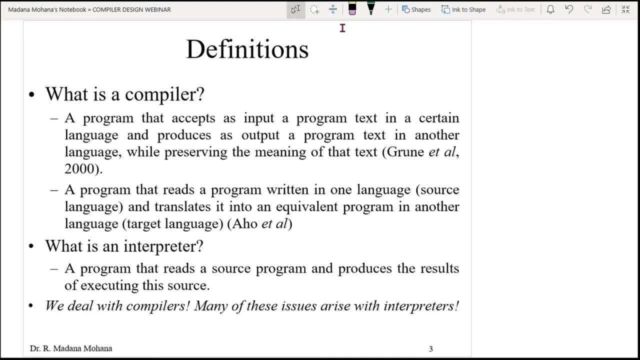 So once compilation is successful, then what you have to do You can run your program. So during running you will see output. whatever the given input, The output is produced accordingly. So that is the actually the process of compilation. 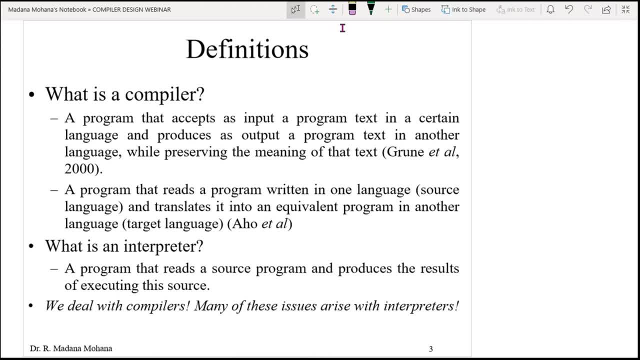 So, finally, a compiler which converts the source program into target program may be high level to low level, Then low level to machine level, like that. Finally, our intention is. so the source program is converted into machine level language, because the computers understand only the binary language. 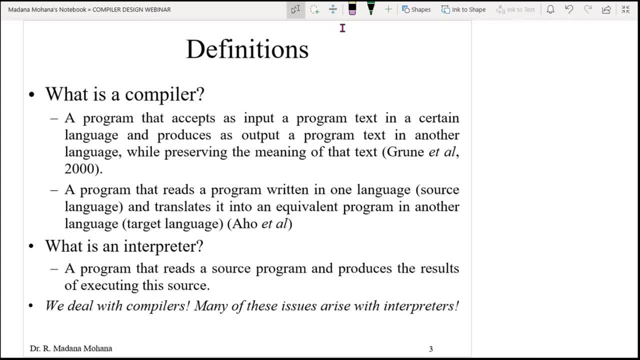 Any given language that can be converted into target language. Target language is our machine level language, So that is the process of compilation. So in addition to compiler, here we are having interpreter also. Let us see the differences. Okay, These two. 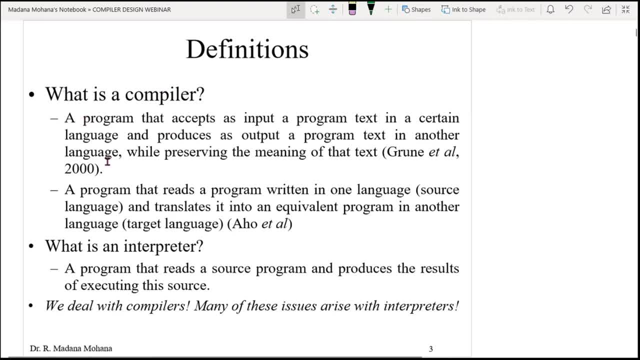 First see some definitions of compiler. So here a program. We are having a program. just now we discussed about C, For example, program which accepts input, A program text. So whatever the program, we have written in the form of some source string or some high level format, etc. 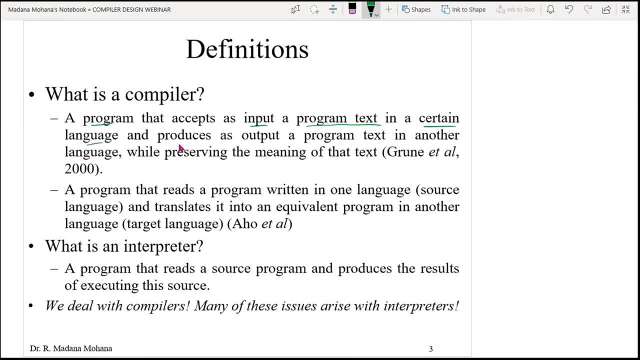 So in a certain language and produces output. So it produces output of that program Again, text format in another language. So the output cannot be in the same language, what you have written, the programming language. The output can be in other form. 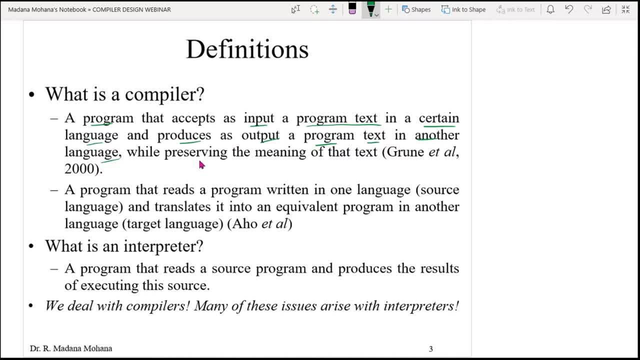 So whenever converting input to output- here one important point- It has to preserve the meaning of text. So that means, suppose you have given some input, So then it has to produce the outputs accordingly, correctly, So it won't change the meaning. 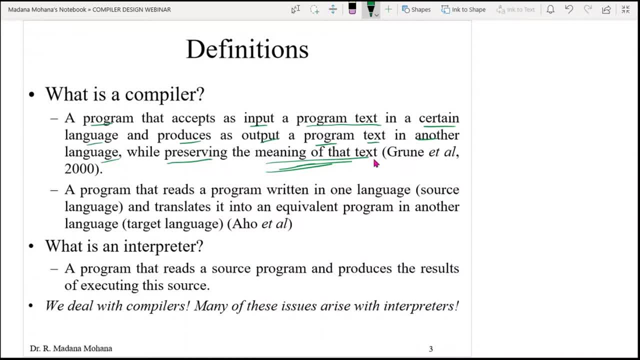 For example, your program is addition of 10 numbers. You have given 10 numbers, So the output should be compulsory. It should add all the 10 numbers, So that logic should be preserved like that. So this is one definition. 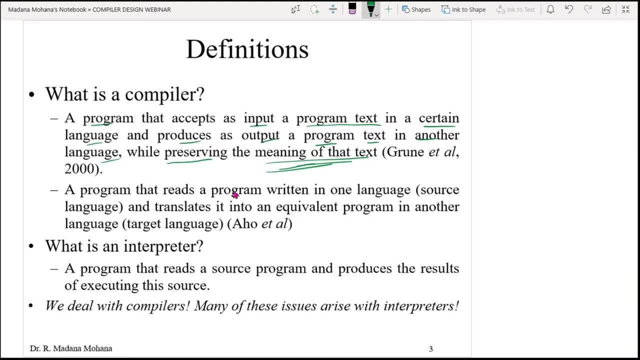 Then, coming to our compiler design, regularly used definition by our prescribed textbook Aho et al: A program that reads a program written in one language. So whatever the program that can be written in one language, that language is called as source language. 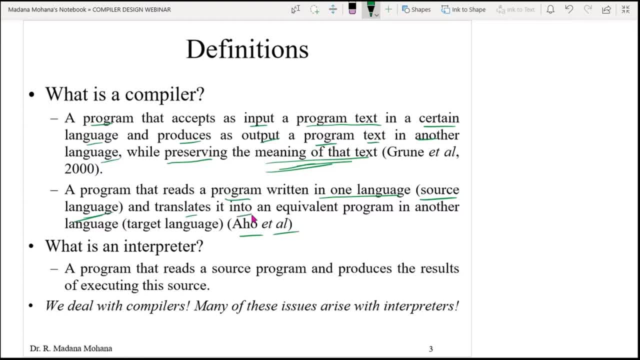 That means our input language And translate it into an equivalent program in another language. Now, what is the another language, Target language? Now, here our source language is the input. Then we have to convert into target language. So for this how this will be done, 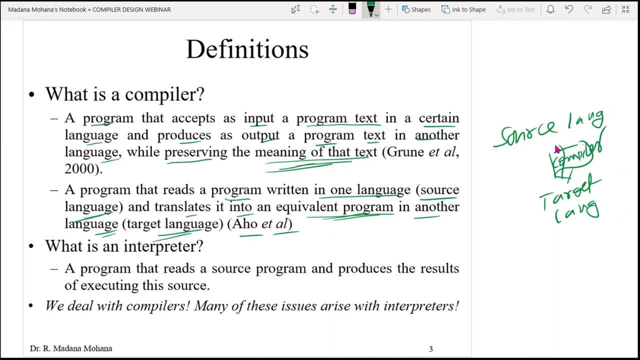 Here we will use the compiler. So compiler is a translator which converts source language into target language. That is the simple form of definition of compiler. Then what is an interpreter actually? So here also, a program that reads a source program produces the results of executing this source. 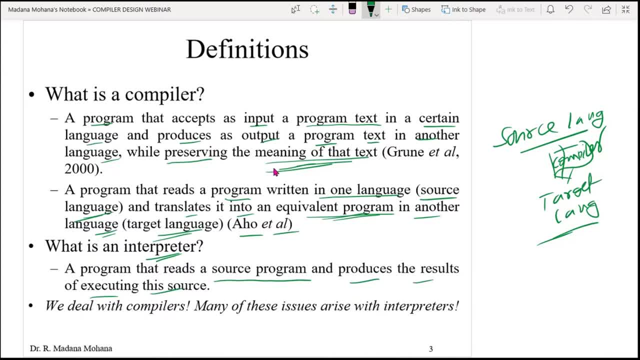 So immediately, So compiler the entire program That can be converted into directly. it won't convert into our target language some intermediate level Like step by step. it converts one form to other form by depending on various internal connections. 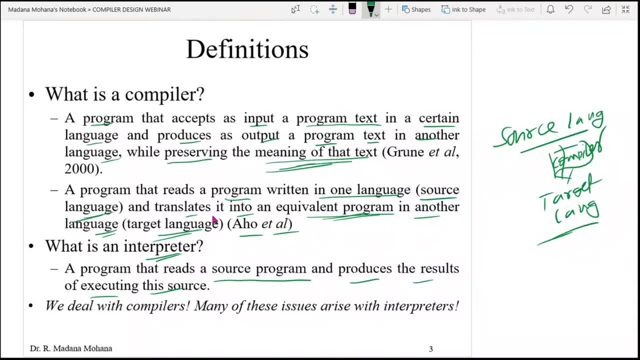 Those we will call it as phases actually, Whereas interpreter. so line by line it verifies, Then it produces. what is the final output? by seeing the execution. It won't see the phase by phase, So completely after execution, only it produces. 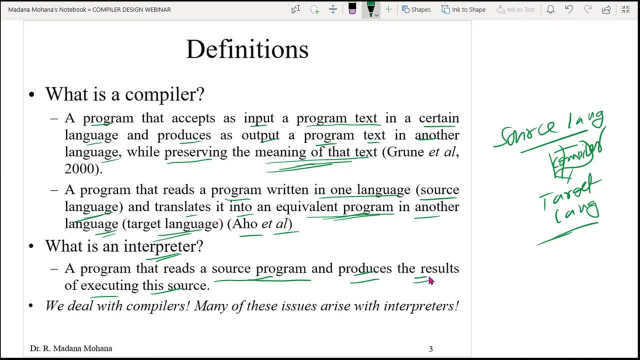 So program that reads source, program produces the results directly of executing this source during execution. So here we deal with compiler. So many of these issues arise with interpreters also, So you already aware what are the differences between compiler and interpreter. 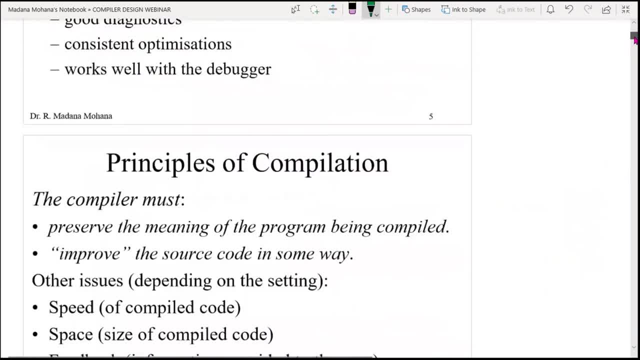 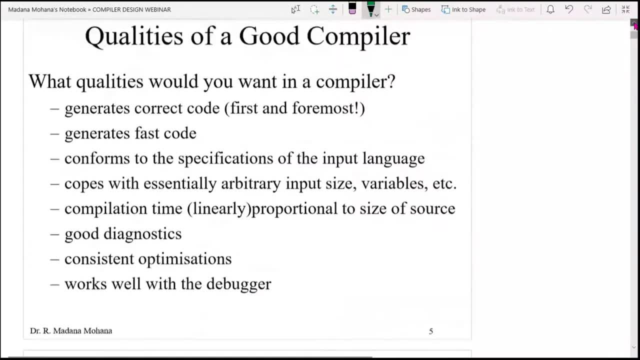 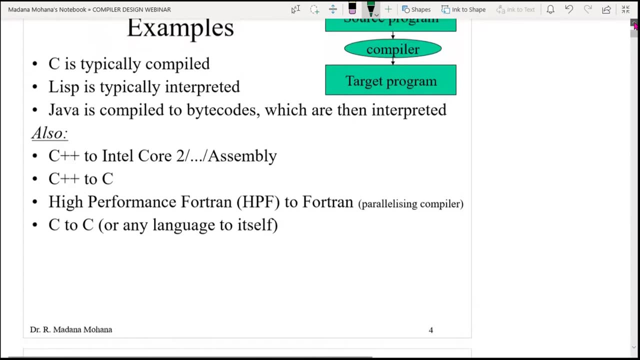 So those you can, Maybe for short answer question you will get What are the differences between compiler and interpreter like, So you can prepare that question For short answer, part k. as for our exam pattern, Okay, now Let us see some examples of compilers. 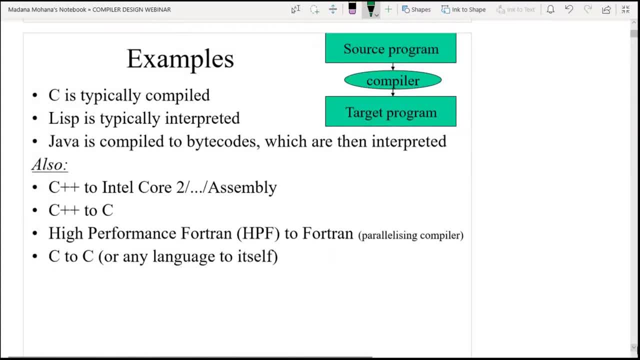 So this diagram just know what I explained. Here you can see The role of compiler. we can take input that can be written in source program, That can be converted into our target program. Here this is the role of compiler: This program is converted into target program. 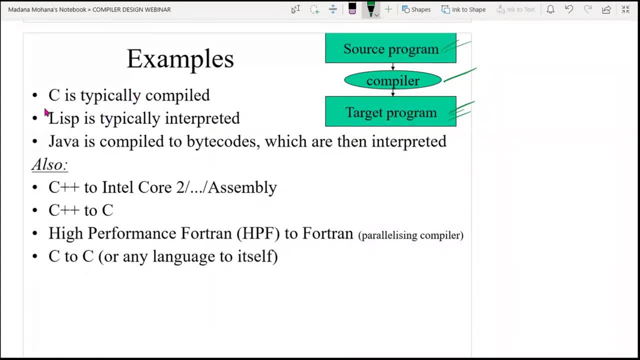 For example. here some examples of compilers are: C is a typically compiled programming language. Then Lisp is another programming language. This is interpreted, not compiled. This is typically interpreted language. Then Java- everyone aware of the Java- Is a compiled that can be converted into byte codes. 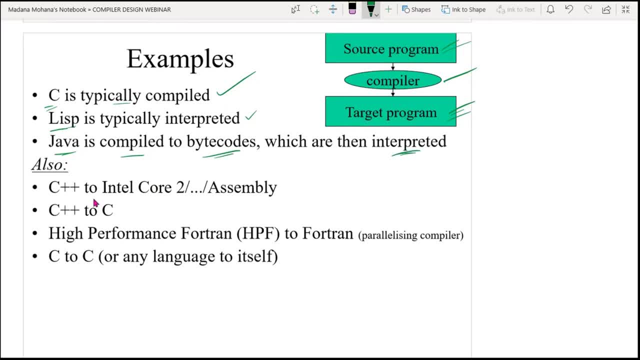 Further, those are all interpreted. Some other examples also, like C++ to Intel core to assembly language, Then C++ to C, Then high performance, Fortran to Fortran. This is parallelizing the compiler. Then C to C, That means any language to itself. 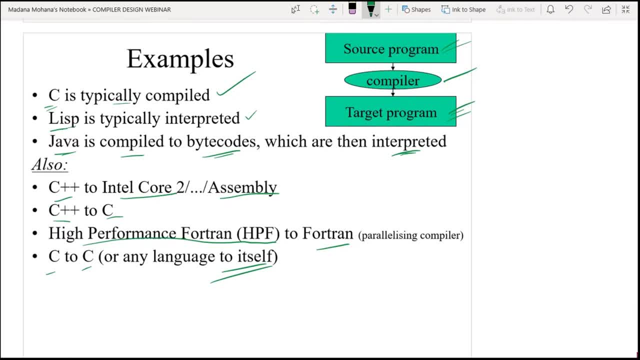 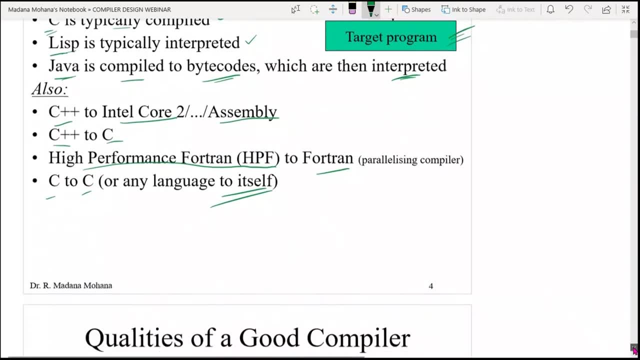 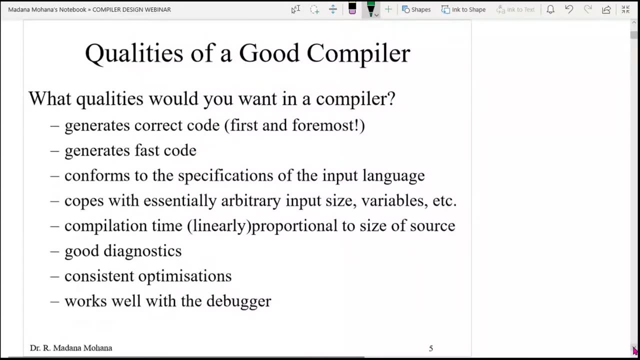 So these are all some of the examples of Compilers, Followed by interpreter also. Okay, now Let us see What are the qualities of A good compiler. So many compilers are there, So any compiler may needs to satisfy. 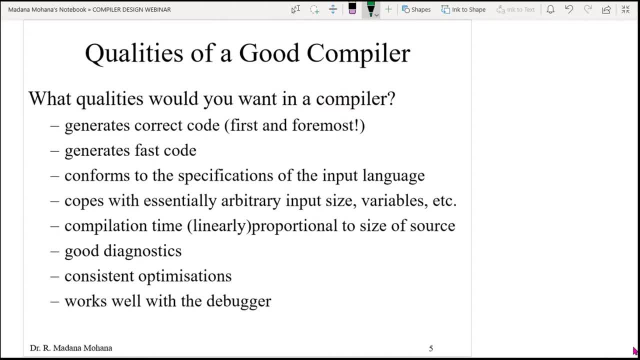 Some good factors, Then you can see there is a good compiler. So what qualities would you want in a compiler? Our first target is, first and foremost, It has to generate the correct code. So then it generates whatever the code that can be executed. 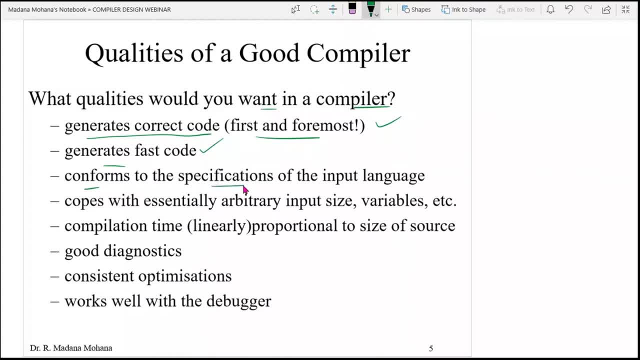 Fastly Then conforms to the specifications of the input language- Whatever the input language, So it should be- Satisfies the specifications of the input language And it copes essentially with arbitrary input size Variables etc. The size also considered here. 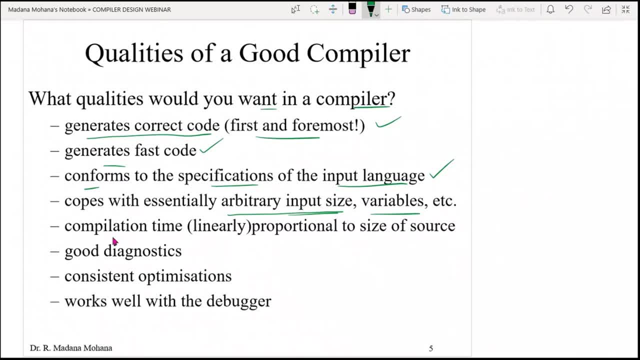 Without wasting unnecessary size. Then the compilation time, So it is proportional to size of the source code, That is linearly. Then good diagnostics. That means it produces Whenever errors are occurred. Then errors can be diagnosed, Sized, rectified. 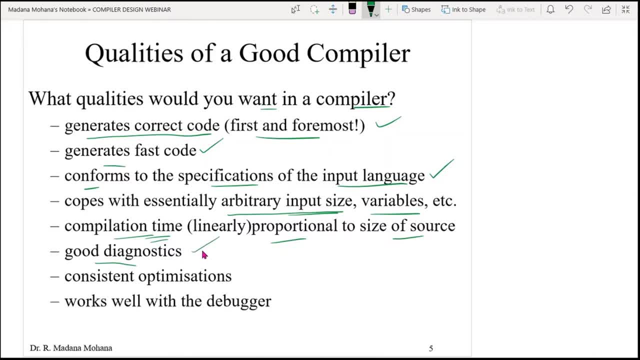 Then consistent optimizations: Whenever you are optimizing a code, Some consistent methodologies You have to maintain. And also works well with debugger. So these are all the Some of the qualities of A compiler. Okay, So let us see. 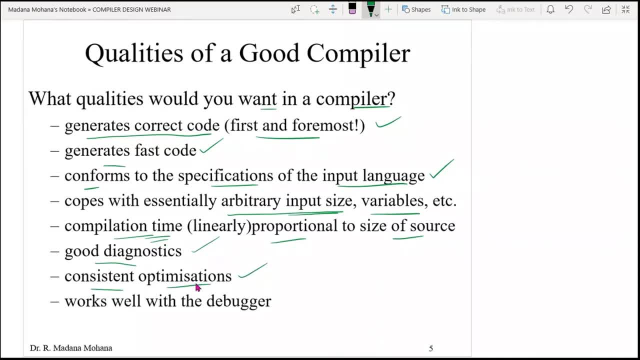 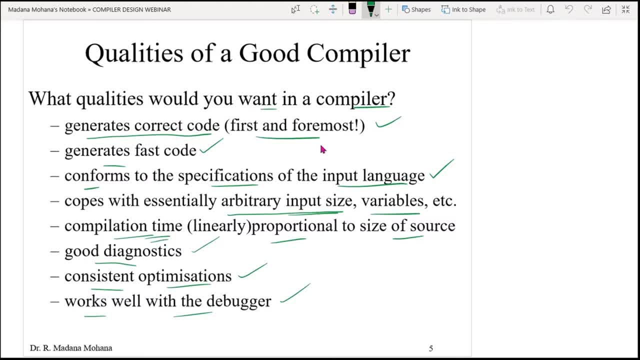 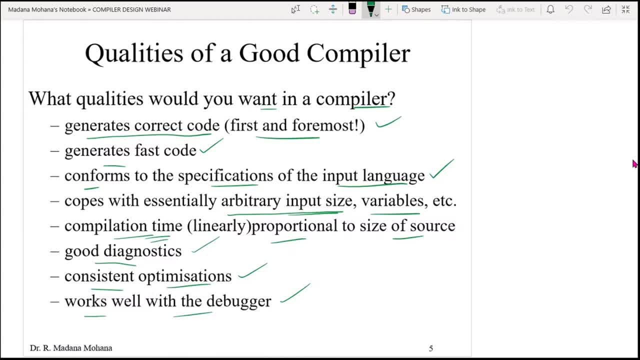 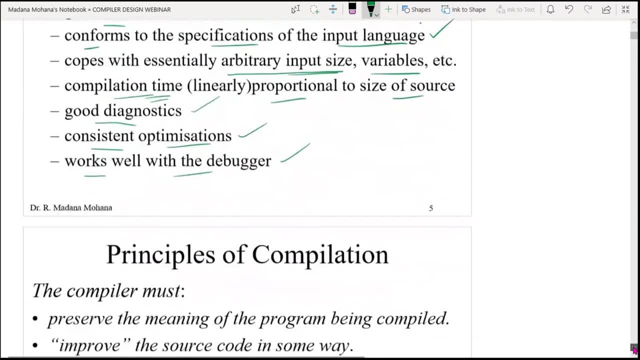 Long ways. Whatever The Corresponding compiler We are using, So compulsory, So it has to satisfy Some qualities. Then Let us see There are some principles Of compilation. The compiler Must Preserve The meaning. 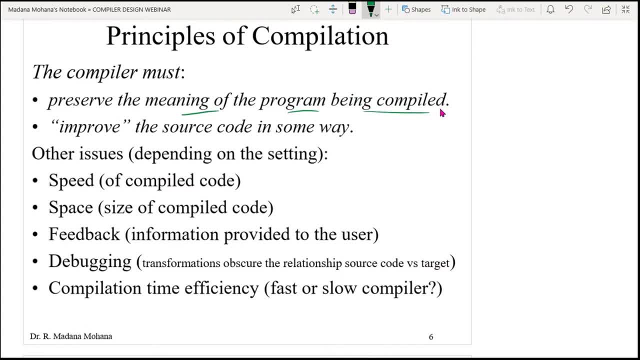 Of the program Being compiled From a compiler. And the first point we already mentioned, whenever the source program is converted into target program, that is, input is converted into output- compulsory it has to preserve the meaning. so then, improve the source code in some way. there are some other issues also, depending on the 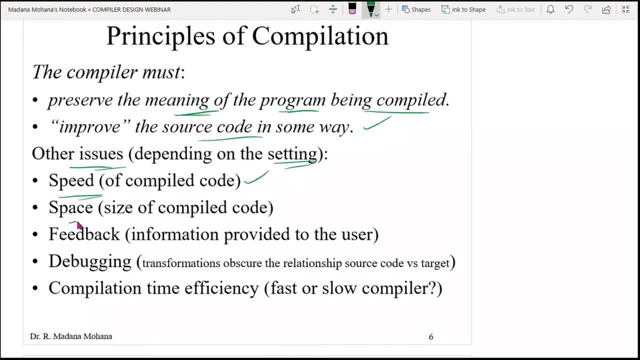 setting, that is, the speed of compiled code, then space size of the compiled code, then feedback information provided by the users, whoever using then debugging the transformation, subsequent the relationships source code versus target debugging at the time of rectifying the errors. then a compiler isn't time efficiency, whether it is fast or slow compiler, so all these issues needs to be. 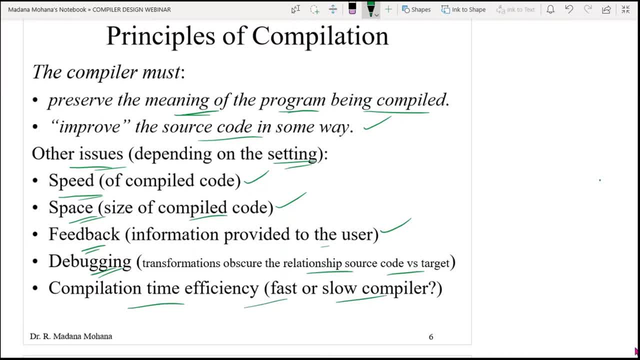 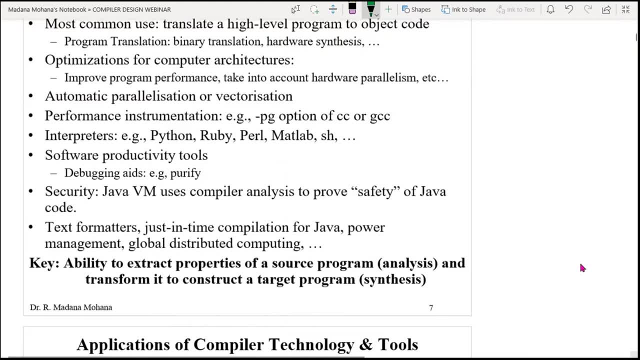 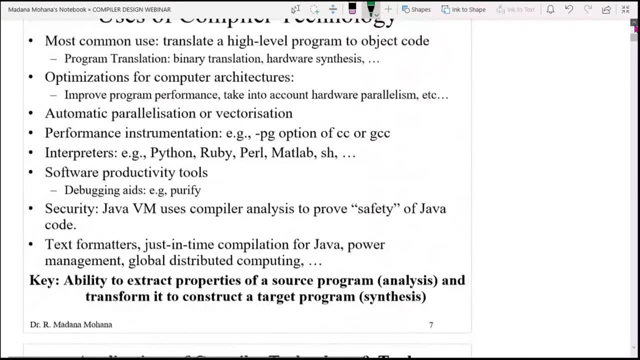 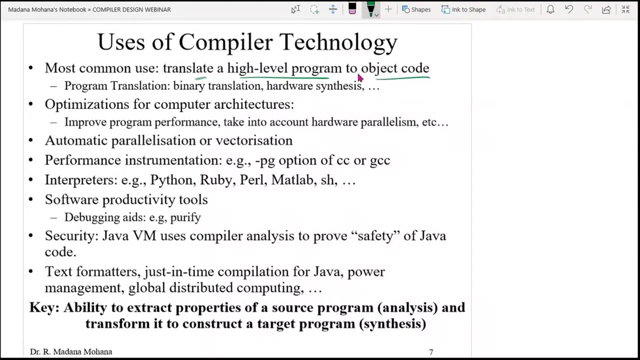 addressed. these are all some principles of compilation. okay then let us see some applications or users of compiler, so where actually compilers are used, then followed by some applications most common uses for translation purpose- translating high level programming into object code, for example program translation. there is binary translation hardware. 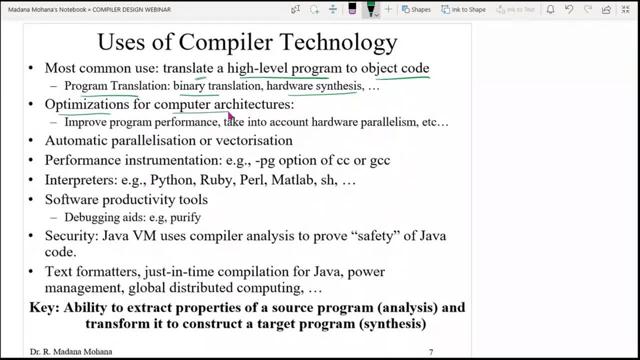 services, etc. then optimization for computer architectures, which improves program performance. take into account hardware parallelism. because of this, these are all advantages. then automatic parallelization or vectorization. then performance instrument implementation. example iphone, pc, option of cc or gc. these are all available, the compilers in unix or 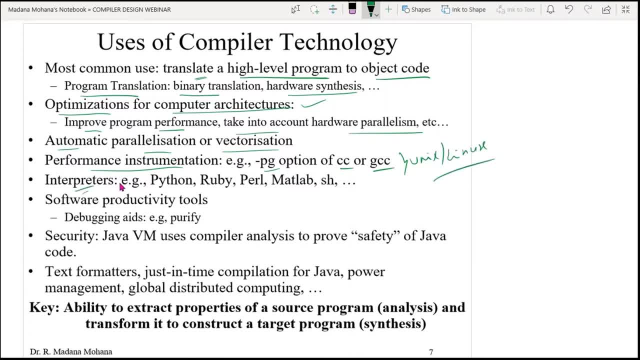 linux flat operating system, then interpreters like python, ruby, parallel, matlab, ss, etc. then software productivity tools like debugging aids, example, purify, then security, using some java virtual machine which uses compiler analysis to prove safety of java virtual mission software. so we will talk about both, that there are some ways to create a network of java code. 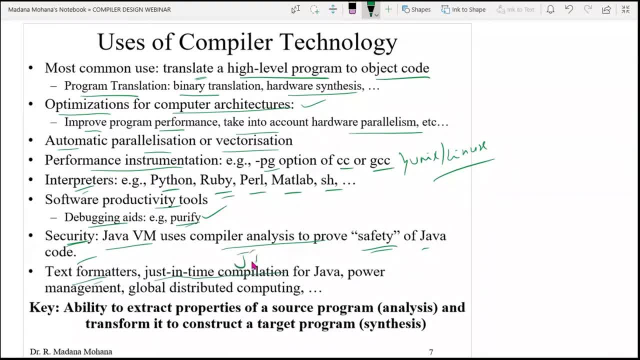 then some text formatters like just-in-time compilation, that you will call it a zip compiler for java, then power management, then global distributed computing, etc. so the key is here ability to extract properties of a source program- that is analysis part- and transform it into to construct a target program. that is synthesis part. in the entire of compilation part, we are having two parts. 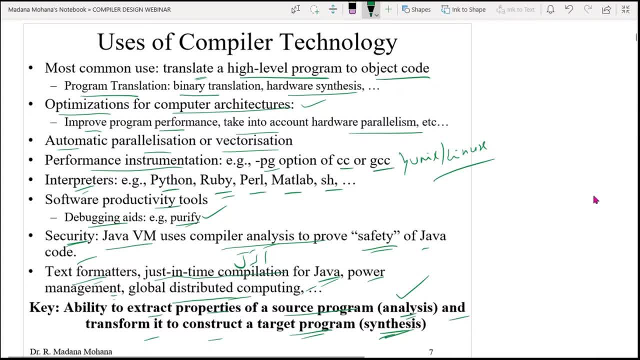 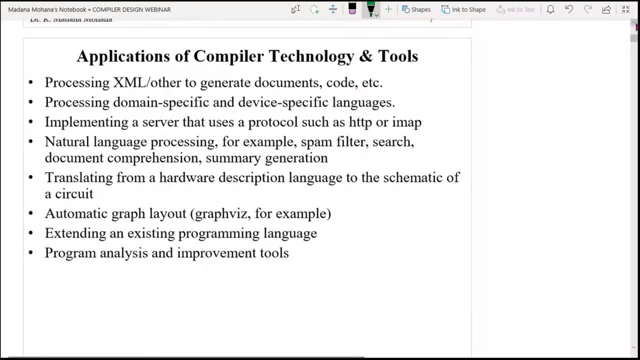 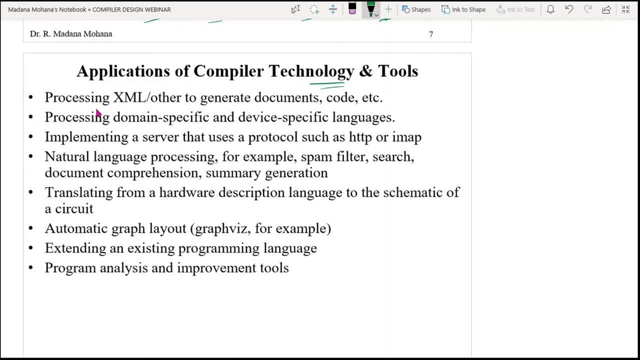 spot and synthesis spot: analysis spot, that is related to source program, then synthesis spot that is related to our target program. now let us see some application software, compiler or compiler technology and tools so here for passing xml, extension, markup, language and other to generate documents, code etc. then passing some domain specific. 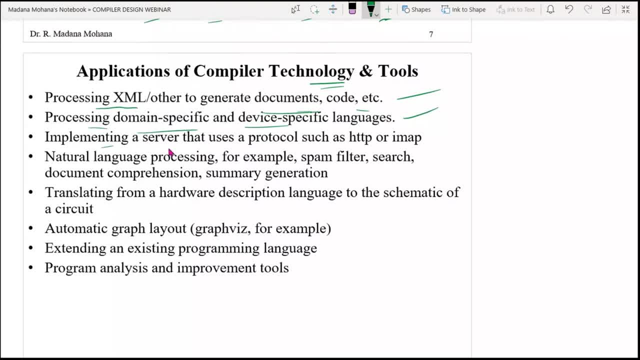 and device specific languages and implementing a server which uses a protocol such as hypertext transfer protocol or imap, etc. then natural language processing is one of the emerging area in nowadays we are talking about artificial intelligence, so data science, machine learning. here natural language processing also plays important role in this emerging area. 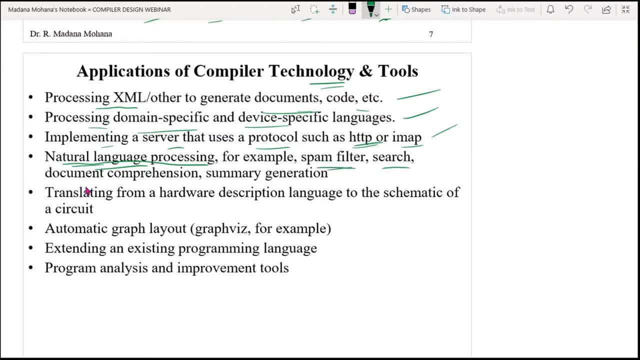 for example spam filter, search and documentation, comprehension, summary generation, etc. then translating from a hardware description language, hdl. so the schematic of circuit this is actually ec related. they are having v, h, p, l, p, p, l etc. for hardware also this will be used compiler. then automatic graph layout like graph. 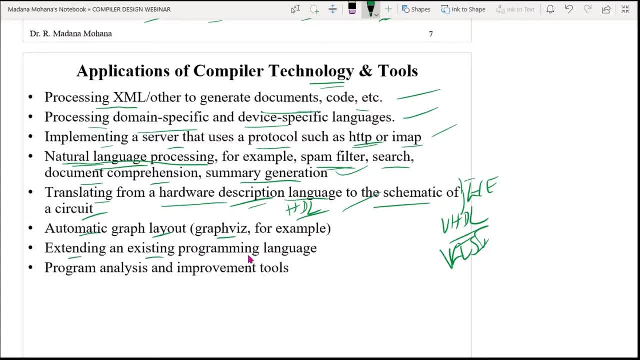 beads- this is one example for this. then extending an existing programming language to other languages by incorporating some of the features. then program analysis and improvement tool. these are all some of the applications of compiler technology, and so these are all some of the uses and applications of compiler. now move to 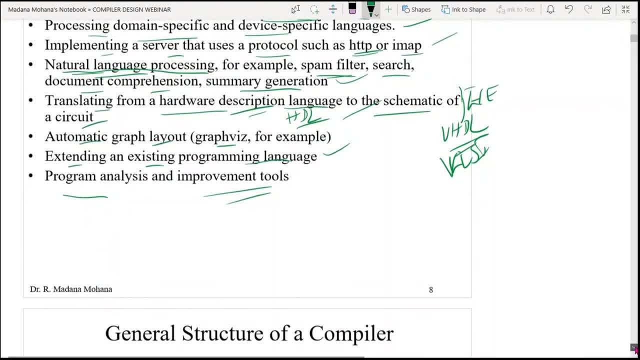 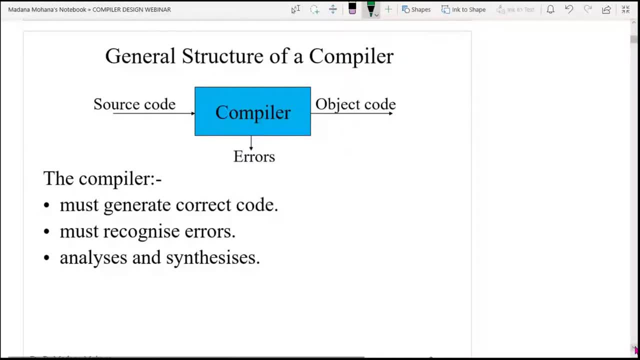 what is the structure of the compiler, the general structure of a compiler. now you know what is the compiler which converts the source code into object code. here we have a source code which converts the source code into object code whenever converting the source code or source program into target or object. 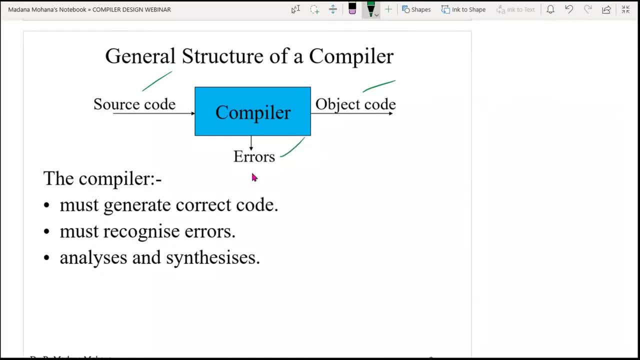 code. during this process it encounters errors also. okay, now this is the general structure of a basic compiler which takes input as source code and produces output as the target code or object code. then during the compilation process, it generates errors also. then the compiler- good qualities of compiler. just now we 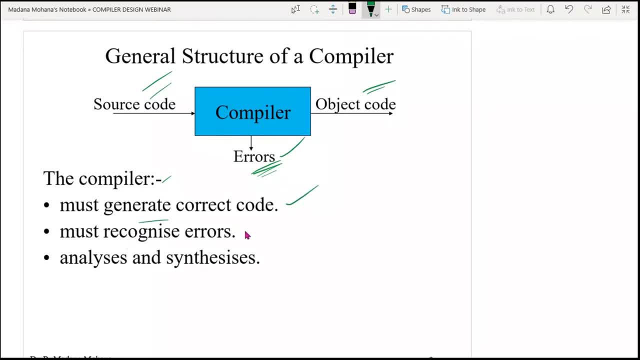 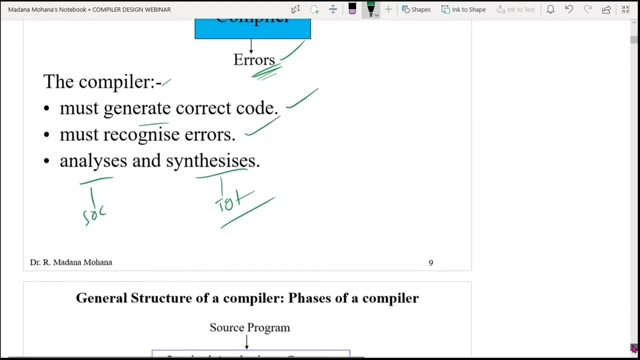 addressed. it must generate correct code. it must recognizes errors and analysis and synthesis part. analysis is related to source program. synthesis is related to target is the role of compiler in the compilation. okay, now move to. there are some pages of compiler. according to this, this structure, source code, is converted. 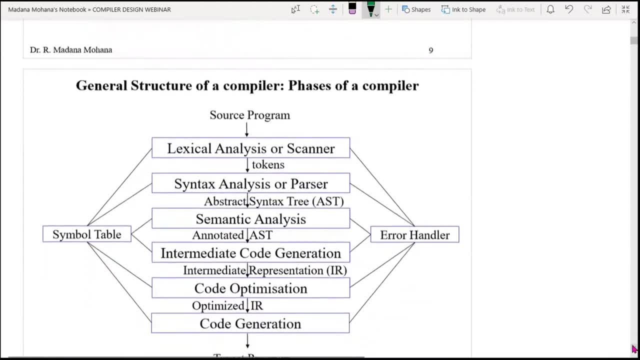 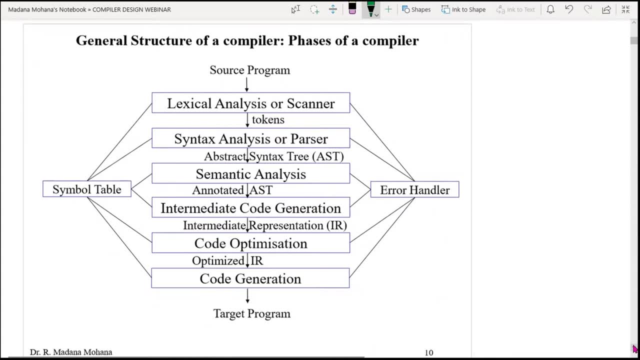 into the object code or target code directly. it can't convert in single step. we are having various pages, so this is the one important question. in first unit in examination you may get this question: explain various pages of compiler with neat block diagram or explain the phases of compiler with the phase wise input. 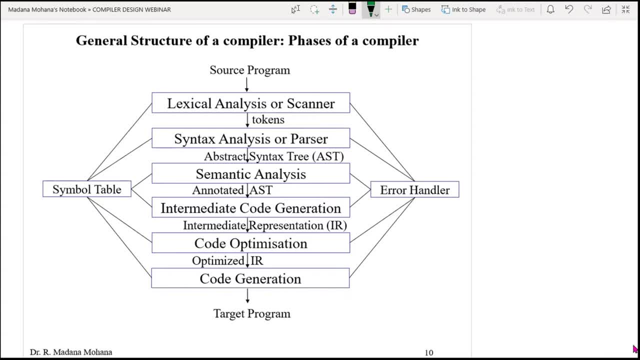 and output by taking one example or they will give an example. so translate the given source program into target program by producing phase wise inputs and outputs, like any of this question. so first, this is the block diagram of pages of compiler. in the compiler we are having total six pages. so 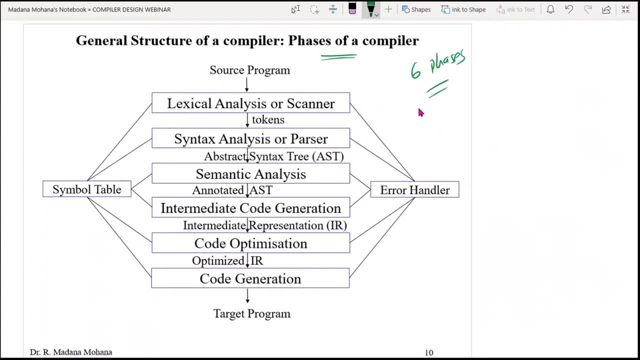 all the six pages. order needs to be maintained. we can't change the order. so the first two phase is called as lexical analysis, also called as scanner. the second page is called as syntax analysis, also called as parser. the third page is called as semantic analysis and the fourth page is called as intermediate code generator. 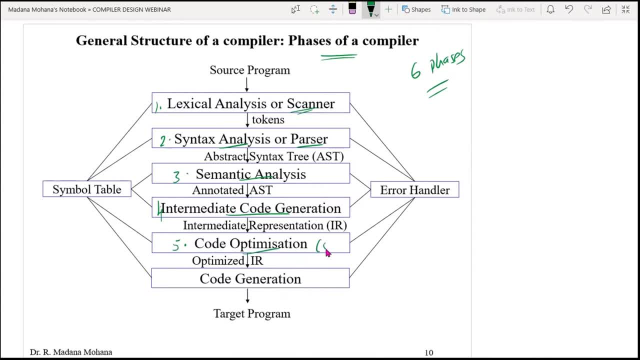 then fifth page is called as code optimizer- this is optional phase actually. then the sixth page is called as code generation. so all the six pages we needs to maintain the order. we can't take the last one be the first one, middle one be the last one. like that the order. 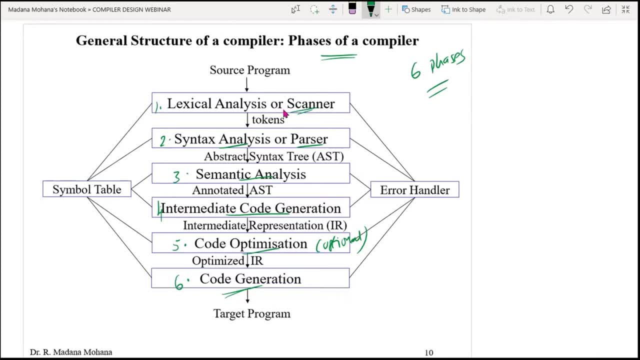 should be follow the same order: first, lexical analysis or scanner. second one syntax analysis of parser. third one semantic analysis. fourth, one intermediate code generator. fifth, one code optimization. sixth, one code generation. so all pages are internally connected. so here you can see all this. you can make it as one box. so now you can see our previous diagram, what it will be so this 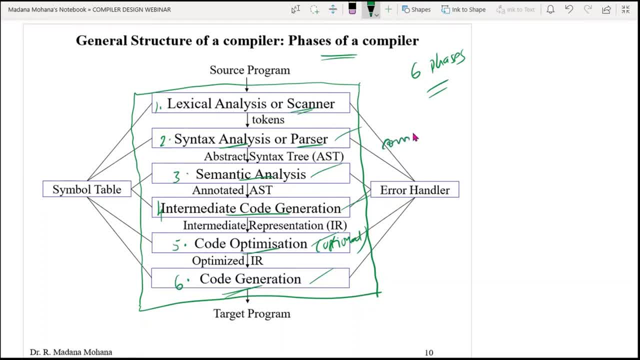 will be like this. now this entry will be like this. now this entry will be like this: now this entry box is compiler. know its box is compiler. what is the input source program for the output target program in the previous diagram? widen the simple structure. same only, but internally the compiler is. 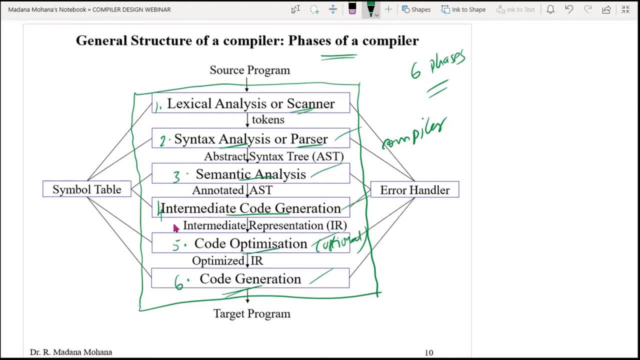 divided into six phases. all the six phases are given in the order. what are the ordered? so say, water needs to be maintained. okay, now for each phase. so we have to take the input. so then for first phase, the input. input, the source program is converted into some intermediate representation. now that 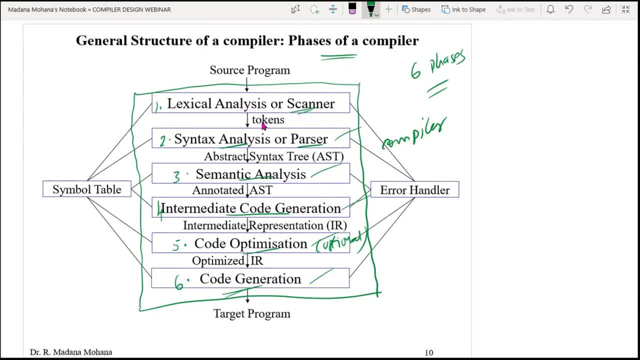 is the output of first phase. now output of first phase becomes input of the second phase. then second phase takes output of first phase as the input and produces some output. then that output will be treated as input to the next phase, like that. so one phase input should. 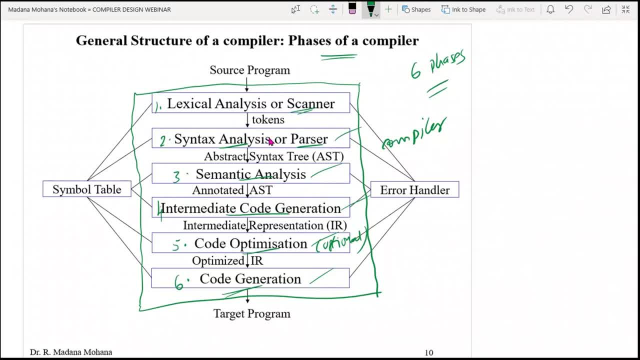 be the- I mean one phase output should be the input to the next phase, and so on. then, finally, coming to the last phase, the code generation. its input is output of the fifth phase, that is, code optimizer. then, finally, what is its output? our required target program? this is: 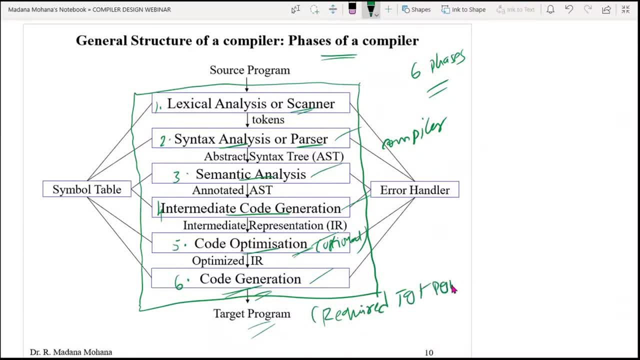 our required target program. we have taken input as source program. source program is converted into target program. this is our required target. So how this will be converted in different phases. ok, now each and every phase in the previous diagram. there we are having error, also error component. so that is why here every 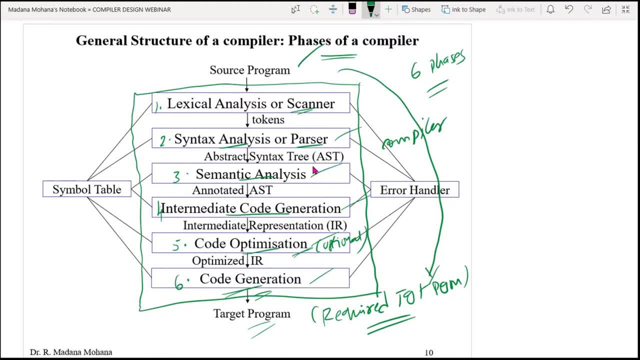 phase encounters or occurred errors, those can be handled by using error handler mechanism, using some error recovery strategies, phase wise. whatever the errors are encountered, there are some error handling mechanism. So how this will be converted in different phases. ok, now, each and every phase in the 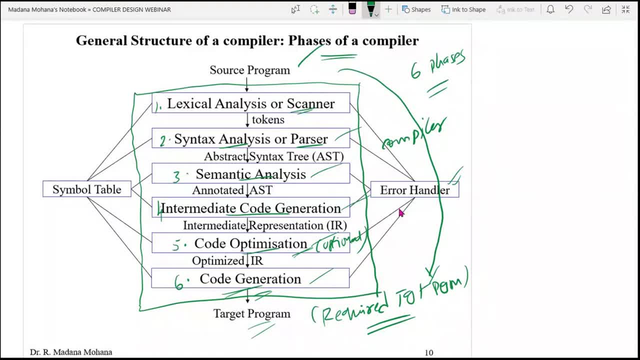 previous diagram. there we are having error, also error component. so that is why here every phase encounters or occurred errors. those can be handled by using error handler mechanism. so commonly the error handler is connected to all the phases in the diagram you can see. so all the six phases are connected to the error handler. then in addition to this we: 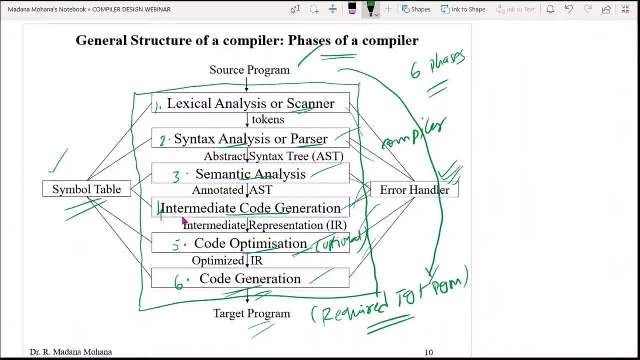 are having another component which is called as symbol table. this symbol table will be treated as the data structure, so which is used to store the information about the phase, the phase wise, the information related to the program, some important information like variables. that means identified, some constant information in the memory, where those are. 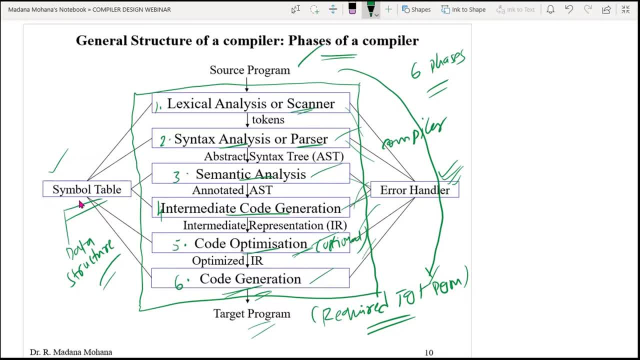 all stored, that location, etc. that can be stored by using symbol table. that is why this will be considered as data structure. this is also connected to all the phases, which are the phase whenever it requires the information about data structure. actually, this information will get collected in the data structure which is taking place in the data structure. the 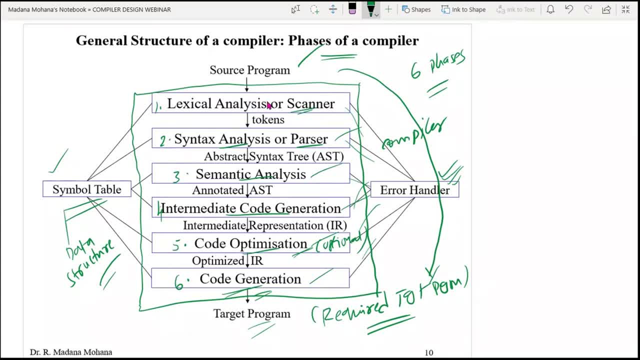 The identifiers or whatever the information available in the program wants to access, so it can access from the symbol table, like memory, where it is stored, in which location it is available. So this is the block diagram or functional diagram of pages of compiler. So here briefly I will explain phase wise what is the input and what is the output. so 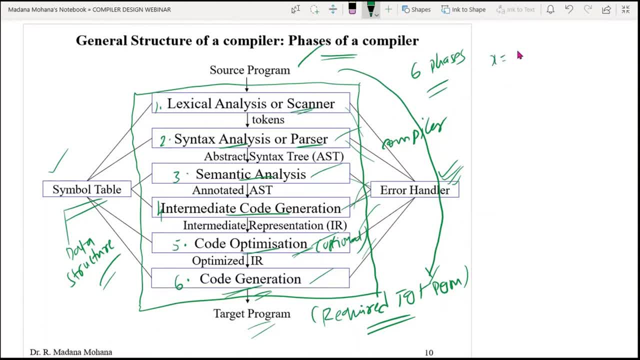 by taking one example. So let us take, for example, x equal to y plus z into 10. so this is the source program. This is the source program which is called as input. ok, now, first lexical analysis. So lexical analysis, or scanner, what it produces? it reads or scans the input, string or input. 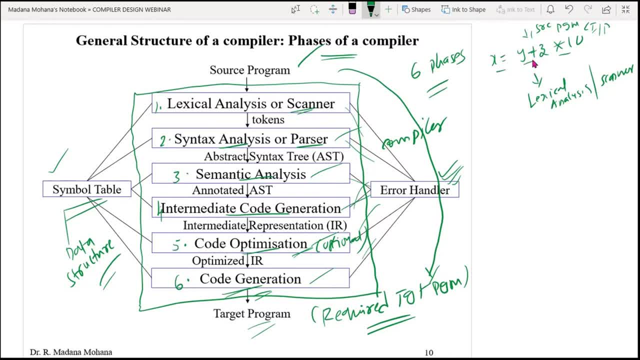 program From left to right and identifies in the given source program what are the things presented. so that means these can be grouped. the sequence of characters are grouped into one category that we will call it as token. it produces token as the output here. so what is token? 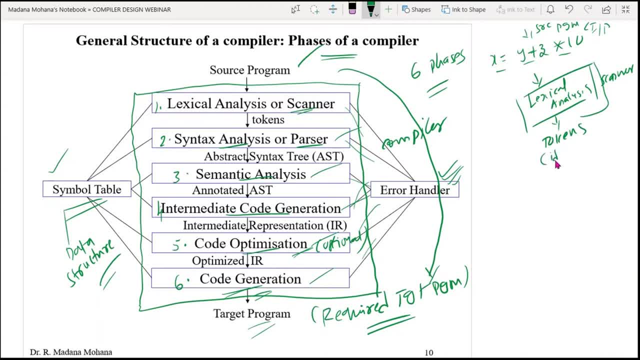 sequence of grouping of characters, for example identifiers, Then constants, then keywords, then operators, etc. these are all the frequently used token. So in your given source program, let us see: here we are having x, y, z. what are x, y, z? these are all the variables. now, this variables, now we will call it as identifiers. so x you may. 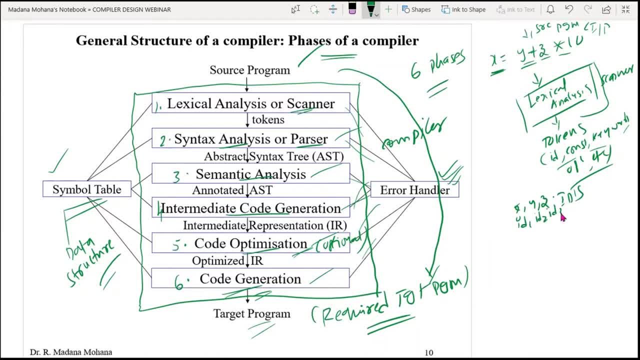 call it as id1, y, you will call it as id2, z will call it as id3.. Now we are having Equal plus. into what are these? these are all called as operators. actually we are having: equal is assignment operator, plus is addition operator, then aspect is multiplication operator. 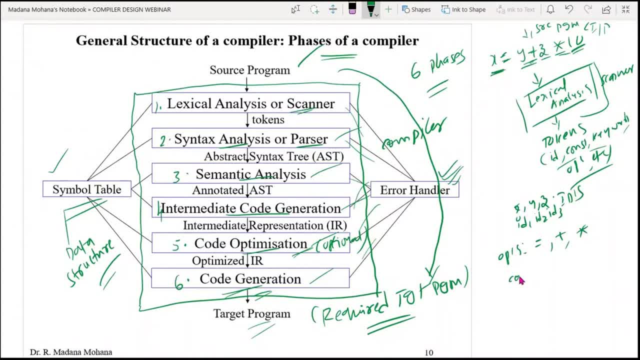 then we are having a number 10. what is this number is called, as this is constant here- 10.. So, like that, the lexical analysis or scanner, which reads the source program from left to right And identifies in the source program what are the tokens available, then it groups all. 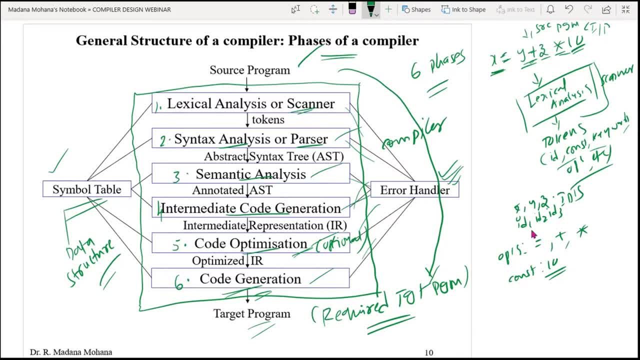 the related tokens into one group. all identifiers are one group, then all operators are one group, then all constants are one group, like that. this is the output of lexical analysis or scanner, So that is called as token. so now here, this is the output of the token. now this token. 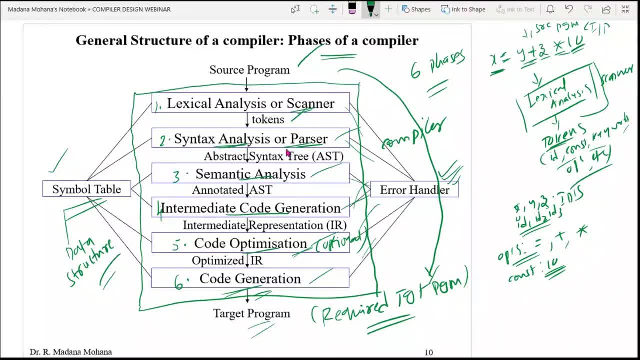 will be considered as input to the second phase, that is, syntax analysis or parsing. So now let us see what is the output of the token. then what syntax analysis are parser produces the tokens that can be represented in the hierarchical form that is called as a tree, tree structure, tree structure. this tree will 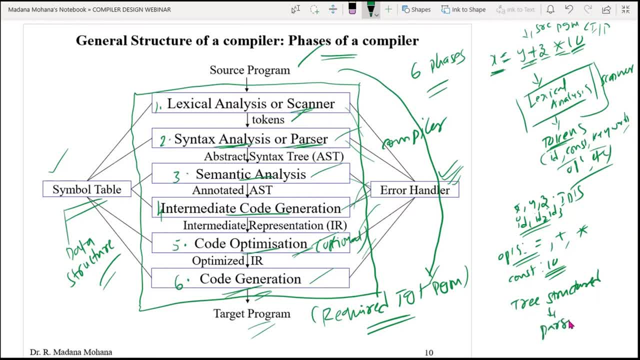 call it as what we will call it as parse tree. we will test parse tree. we are having another tree, also syntax tree, but these two are different, parse tree and syntax tree. both are not same. so parse tree is nothing but for the given grammar. so we are having a grammar in syntax. 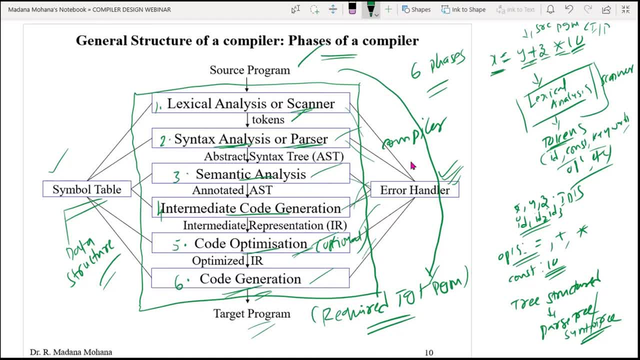 analysis, are parser. so the programming languages are described by a grammar which is called as context tree grammar. that also we will review briefly. so from the grammar if you want to derive a string using the productions, so the process of derivation, so step by step, whatever the productions we substituted, that can be represented hierarchically in the form. 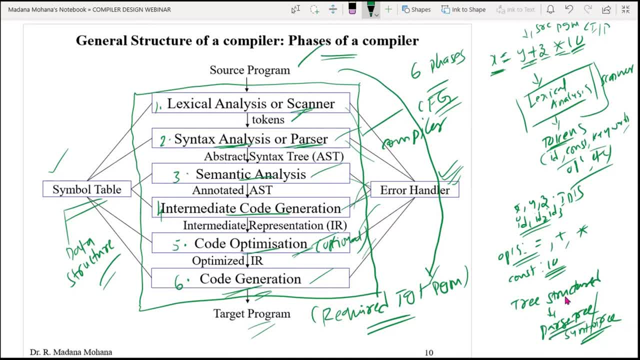 of tree, that tree is called as derivation tree or parse tree. then without using the grammar, by considering only the string, you can construct a tree. then that is called a syntax tree. so syntax tree hides the grammar symbols only. it contains the terminals. that is the difference between a parse tree and a syntax tree. 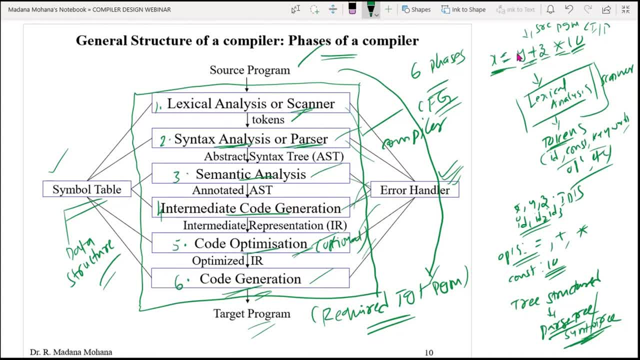 Okay, now the tokens here. you can see here there is no topic of grammar. so this expression x equal to y plus z into 10, this can be represented in the form of tree. now that tree is called as syntax tree, so the output of syntax analysis are parser, so abstract syntax tree. why you? 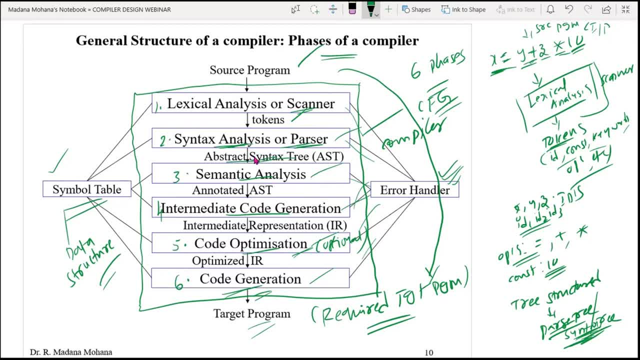 are calling it as abstract syntax tree hiding. so it won't shows the grammar variables, only it shows the terminals in the form of tree. so it is called as abstract syntax tree and simple terms as tree- that is the output of syntax analysis- are parser. okay, now what semantic? 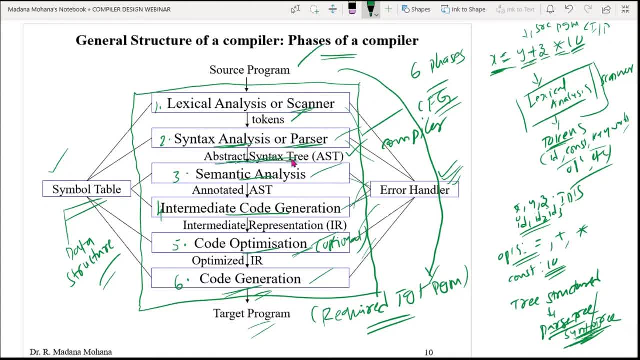 analysis will do, will take input as the same syntax tree. whatever we constructed from the syntax analysis are parser, then it provides some semantic actions, some validations. suppose you are having in this expression 10. is there 10 actually constant? what is type of this constant, whether it is a constant or a constant? 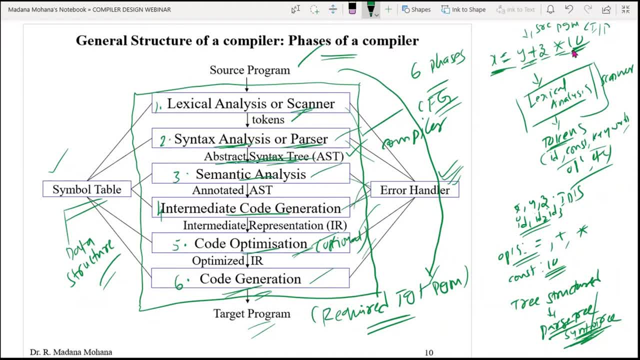 What is the type of this constant? So integer value or floating value? so what is this conversion like? into? to float or something? so that type conversion is not there here directly. a constant is there. it provides the semantic checks or validation meaningful form. so that is the output of semantic analysis. 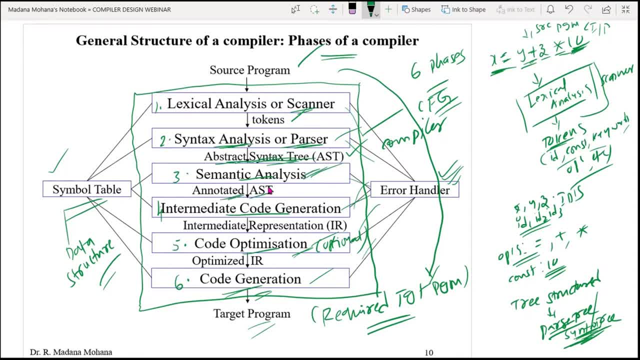 that we will call it as unnotated abstract syntax tree. in the syntax tree, wherever the respective values are there in the particular node, it can be labeled. Notices anything but labels. labeled the meanings are the semantic checks in the respective nodes wherever that value is there, for example in the tree 10 where the 10 is connected in. 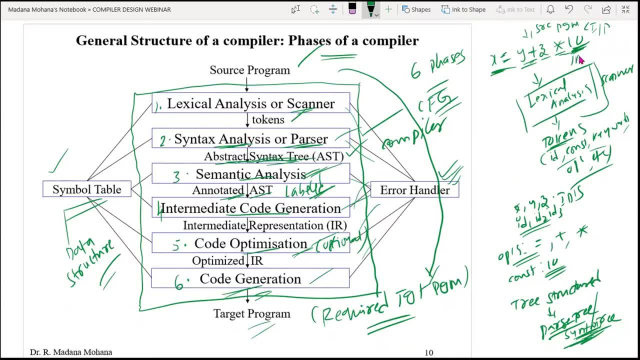 the tree in that node it gives some type conversion like into to real or into to float something. so this is the semantic check or validation. these type of validations or checks can be done by semantic analysis. again, output of semantic analysis: also same syntax, the only part- annotations are added. there is only different. 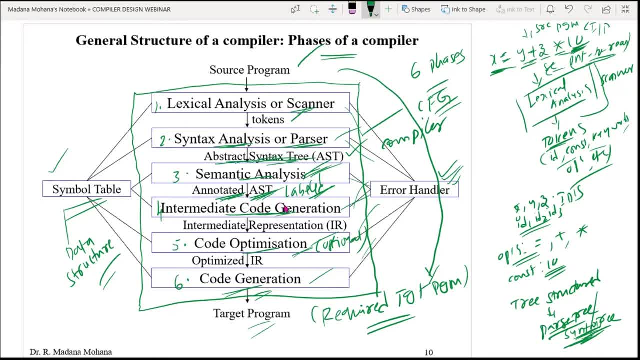 Okay, now the next phase: intermediate code generator. what it takes? it takes the unnotated abstract syntax tree constructs. those can be converted into some intermediate form. so the output of intermediate code generation is called as intermediate representation. so what are the various intermediate representations? even the abstract syntax is one intermediate representation. there are some other intermediate. 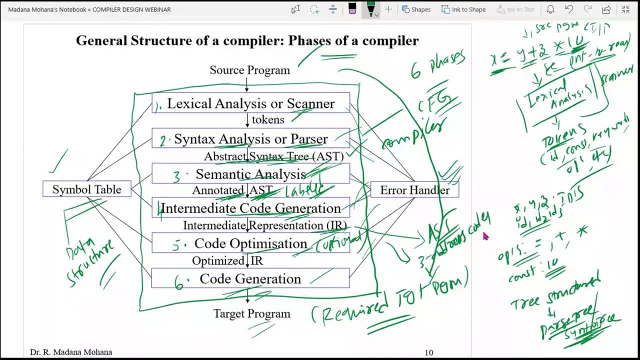 representation also like three address code. so three address code. the general form is x equal to yopz. here y and z are operands, op is the operator, then x is the resultant operand. so here three addresses. so one address for y, one address for z, one address for. 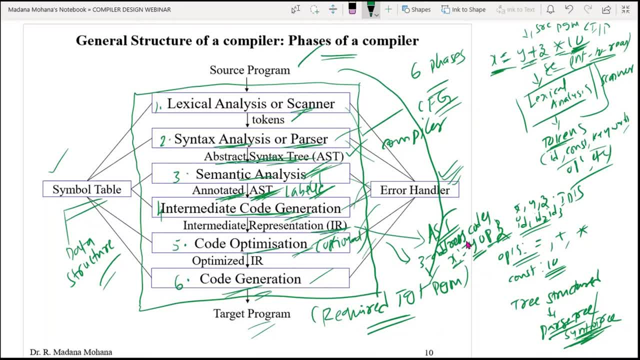 result x. that's why this is called a three address code. this is general form of three address code. in three address code we are having various representations, like triples, then quadruples, then indirect triples. so three types of three address codes are this: 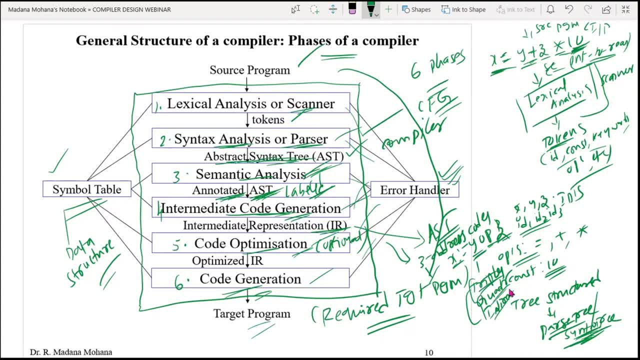 is very important in intermediate code generation. in examination you may get explain various three address code forms with an example or for the given source program, convert into three address code With quadruples, triples, indirect triples. so this question is important there. these 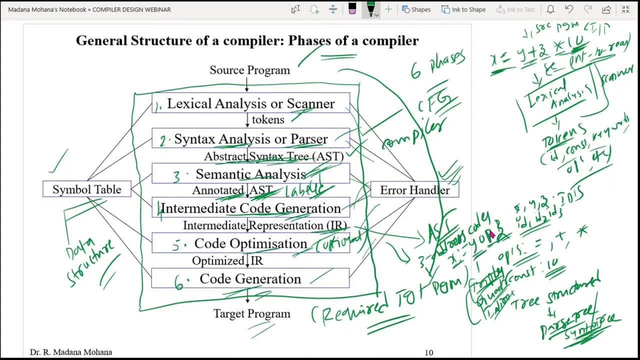 are all various intermediate representation forms. Ok, now these intermediate representation forms. so if you are having some repetitions, some duplications are there, so those can be reduced or optimized. for that code optimization is used. what code optimization will do? wherever the possibility to reduce, then some of the 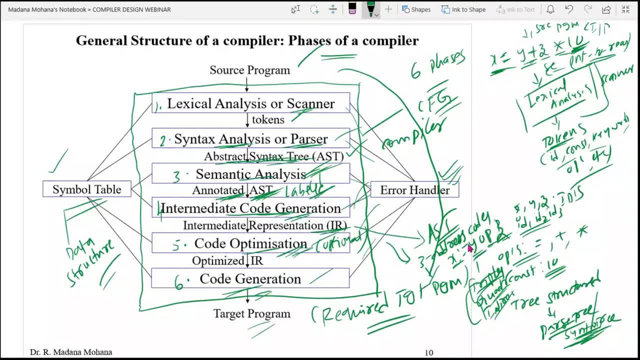 triples, then some duplications are there. Ok, So these are some of the temporaries or the variables, so it can be optimized and produces the same as intermediate code, form only, but optimized intermediate code. so once you know the intermediate code output, the code optimization output also safe, but some lines may be reduced. 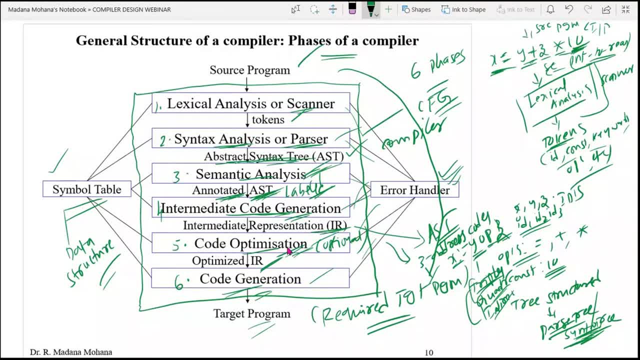 or merged with others. that is optimized code. so whenever you are doing optimization, compulsory again the meaning has to be preserved. so that is the code optimization phase. then finally, what the code is. So what the code generation will do. the code generation takes the optimized intermediate. 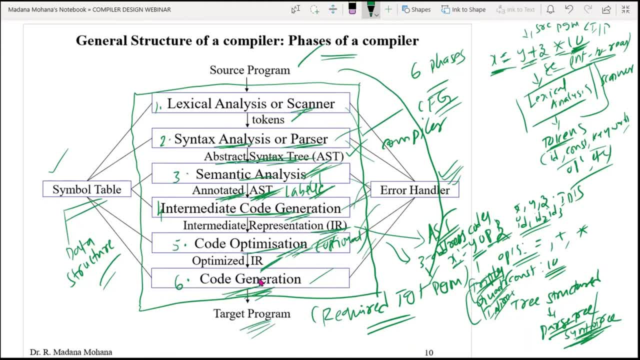 code at the input and produce the target code, the code generator, directly. it can't produce machine language, the target program that can be written in assembly language program by using assembler. by using assembler it converts assembly language programming into machine level language. So using compiler directly. we can't produce machine language. 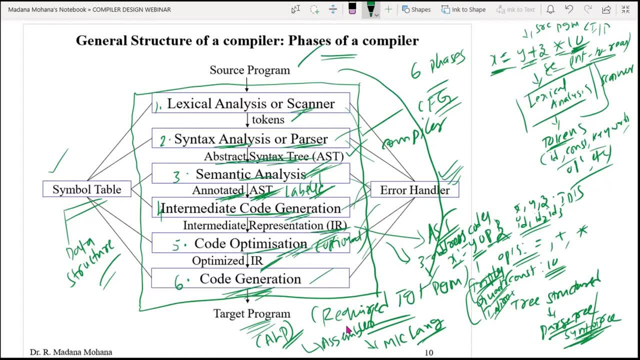 Ok, Machine level language. so we can produce output as in assembly language. using assembler is the another compiler which converts assembly language program into machine level language. this is your real target programming language. that is our machine language. So this is the process of compilation. now you can see, phase wise, the given input. how. 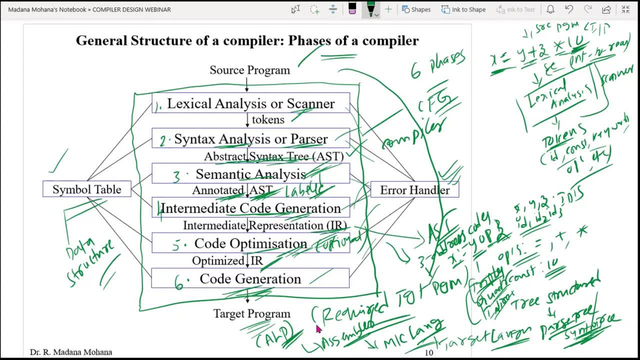 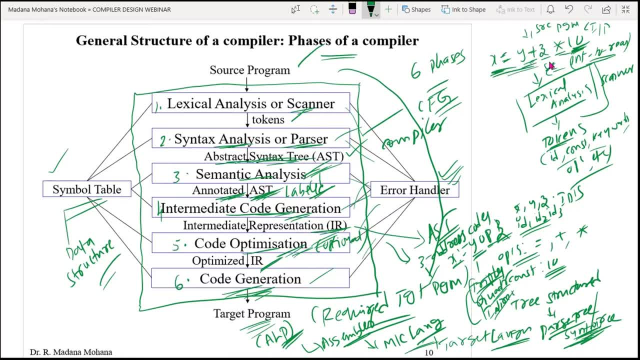 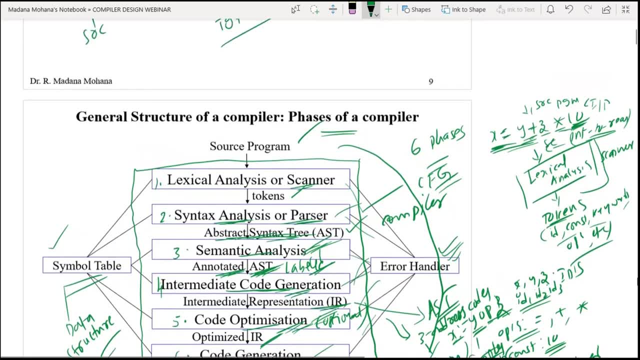 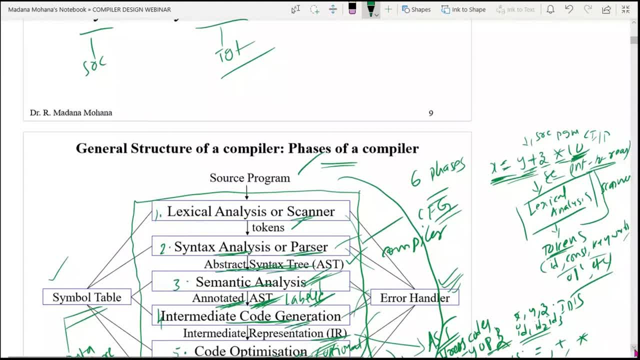 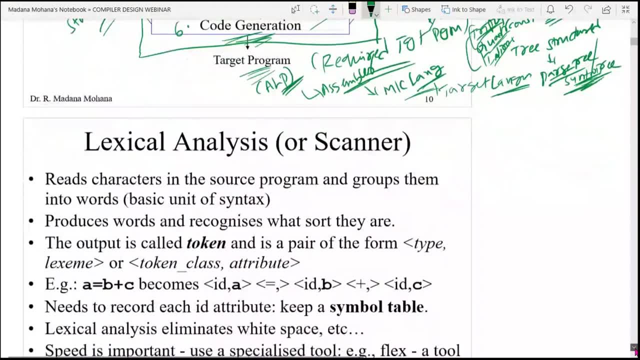 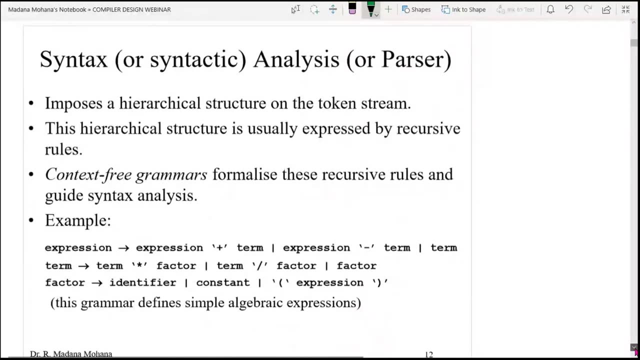 Ok, the same. whatever I explain here I have given I skipped all this because we will concentrate more on the problems. So anyway, I will save this ppt also. you can go there see. this is a very, very important part. Ok, to later, if you want. Here you can see the parse tree also explain. just see one example. 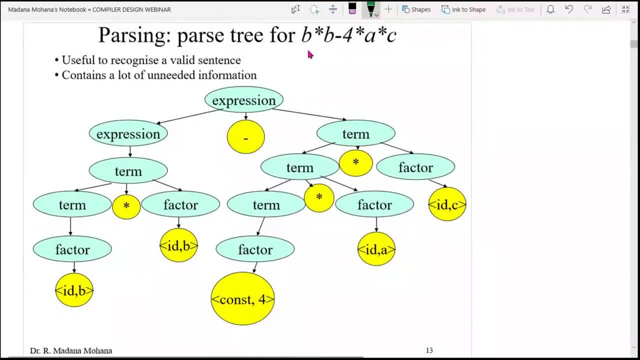 here. So parse tree for the expression. actually this is b square minus 4ac. That means here the expressions, any powers you can expand, like b into b minus 4, into a into c. See one expression, What we have considered: x equal to y into z plus 10, any expression we can. 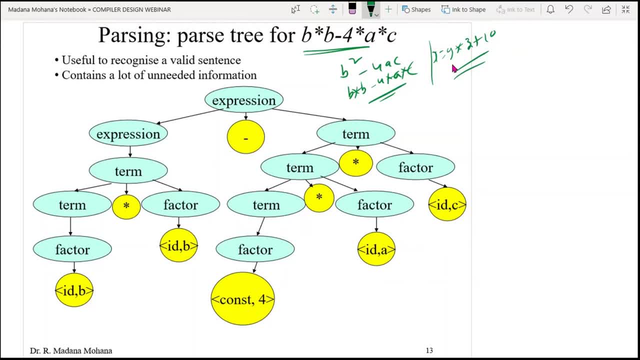 convert into it parse tree. So whenever, if you want to construct parse tree, compulsory grammar is required, that is context tree grammar. For syntax tree grammar is not required, only expression is required. So actually here the grammar is in our simple terms. I will: 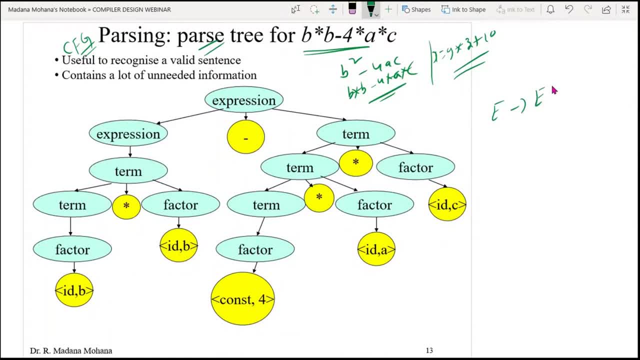 write here. This is called as arithmetic expression. grammar e equal to e plus e, then e derives e minus e, then e derives e into e, then e derives E by e, something like this: So then you are having e derives t term, then t derives. 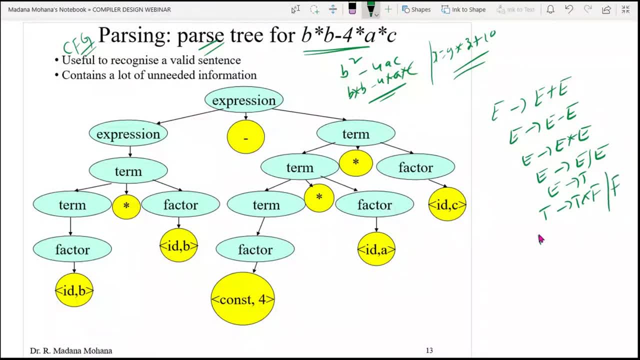 t into f, f, then f derives e, within parentheses or some identifiers or constant etcetera like this: This is the actually arithmetic expression grammar, So here the string is b square minus 4ac for this, if you want to draw its derivation tree or parse tree. So here first you can. 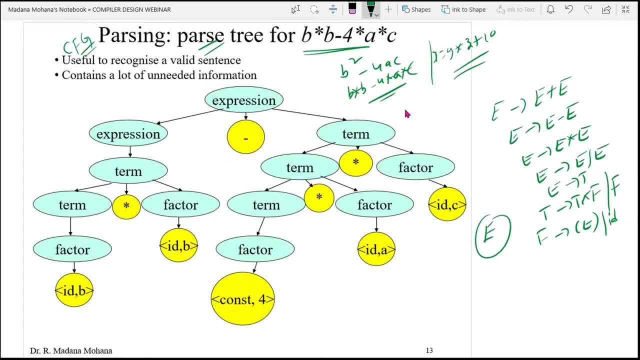 take the starting variable. So you can take the starting variable. So you can take the starting variable as the root. Now e is the root Here. what your contains, your expression contains minus actually. So first you can take the expression related to minus this. 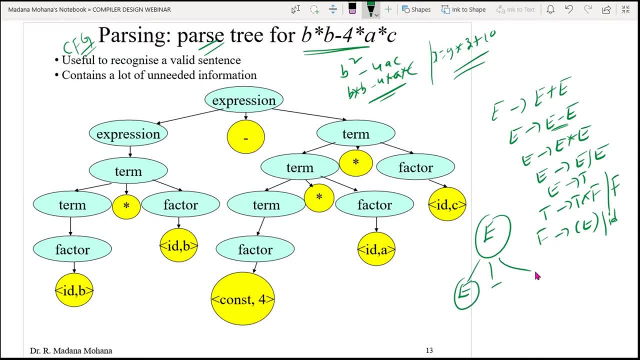 one. You can connect e minus e, So all the internal nodes you can include within circle, then link nodes which contains terminals. we cannot include circle. Now here you can see left hand side of minus what you want, b square actually. So b square means that you can. 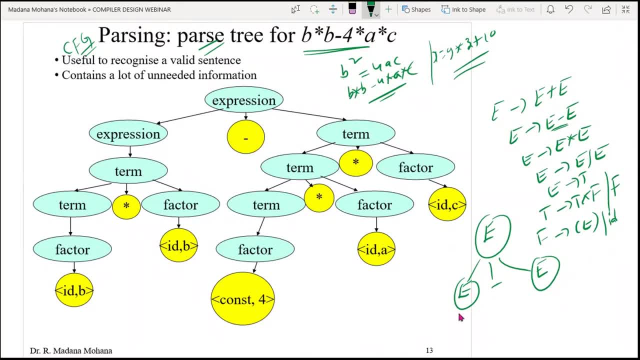 свой a received representation like this. This means again, what is this one? into expression you want E derives. actually you want e into e. So then, before into your left hand side of, into what you want you want, you can do some identifier then the right hand side of. 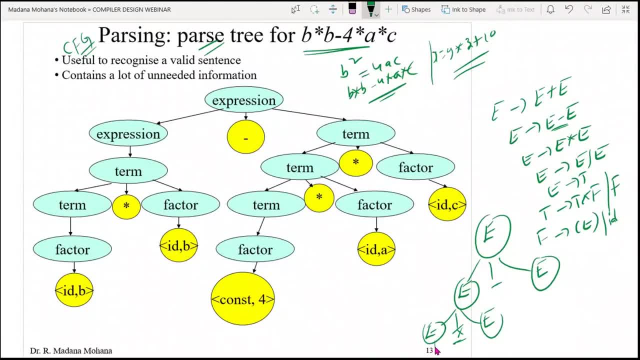 into also identifier. So you are having e derives t, then t derives f, and then f means you are having identifier. So now you are having b- right hand side, e into expressions, then e into e, so this is b and this is the subset of terms there you want. Now you can get ourît Veronica problem. theseurar Rutners function is an operational behaviour of the Russian Ruby, Shouldn't you look? Any other problem can be solved again. what is this one into expression? you want e derives. actually want e into e, but then 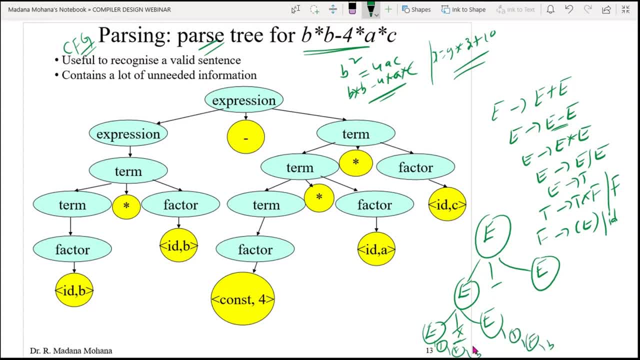 before, into left hand side of, into what you want. you want some identifier, Then the right F derives here, then F derives B. now you can see B into B here, B square minus, then what you want. again you want into so 4, into A, into C, so again you want into expression. 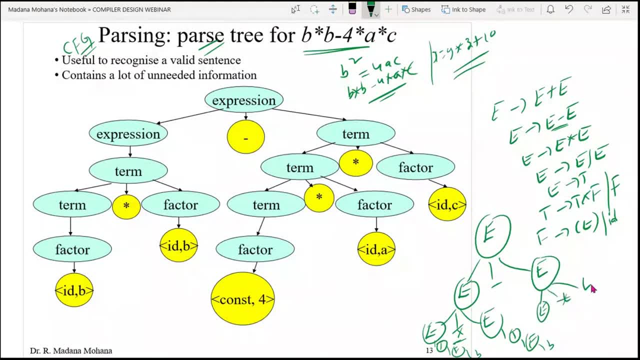 here we are having E into E, so left hand side up into what you want. so again, here you are having, you are having, here you can see, T into F. why? because you are having constant also where the constant is in F. so here again you can take: E derives, so E derives T. then 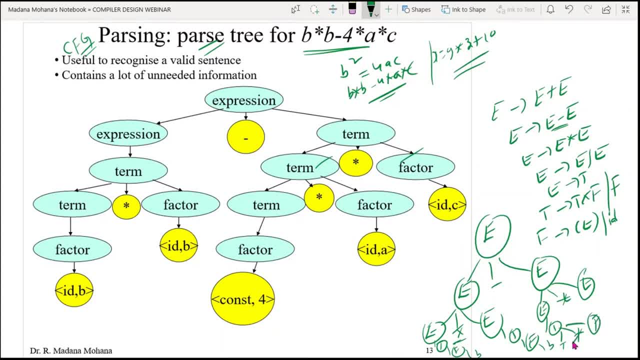 T derives what you want. T into F actually now here before into what you want actually 4 you want. so T derives F, now F derives. we are having identifier as constant also, so directly you can take the 4, then 4 into again what you are having: F derives ID. so 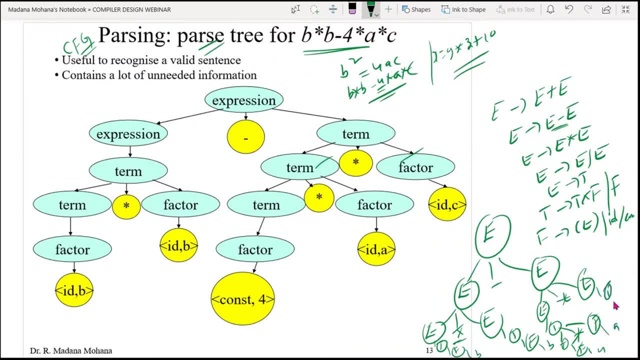 what is this one? A, so again into your E derives T, T derives F, F derives. identifier. what is the identifier here? C, now you can take all the leaf nodes from left to right in this 3, first what you are having, B into, so B into B, this one, then minus, then the left. 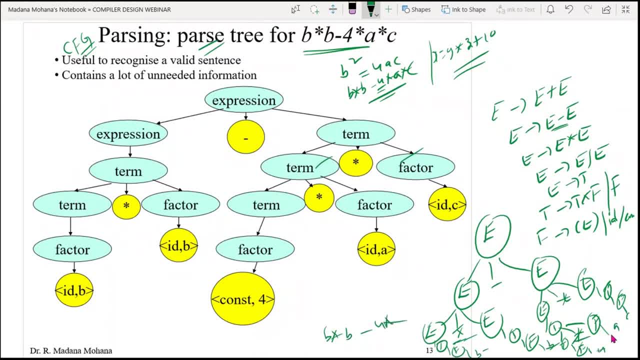 most one is 4, then this one is A. Now you can see our input string is derived here. now this is called as derivation tree or parse tree. here in detail explanation is given. this is simple, simplified form. by taking leaf nodes from left to right you will get the string. whatever the string, this 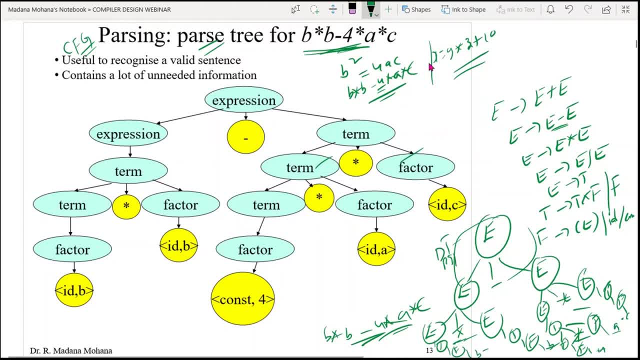 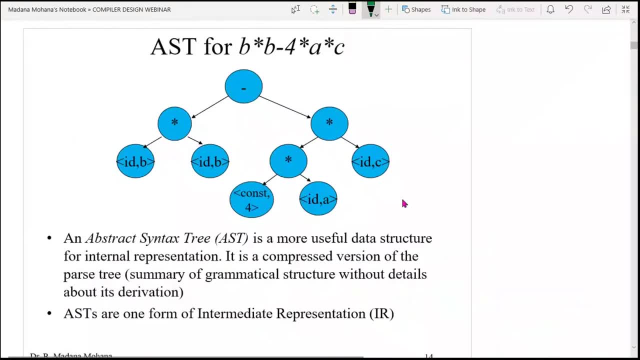 is the derivation tree or parse tree. now for this: how to construct the syntax tree for syntax tree: here the variable is a string. The variables are hided. it won't show the variables, it shows only the terminals. Here you can see B square minus 4AC. only for this expression the syntax is constructed. 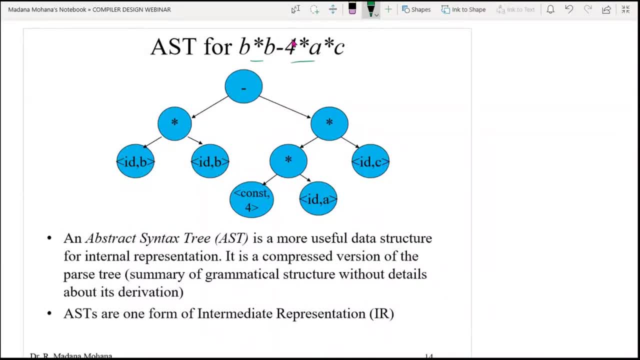 here. grammar is not required Here. first we have taken any one as the root. now here you can see B square minus 4AC. so minus is the middle one. so now minus. you can construct it as the root. so minus of. 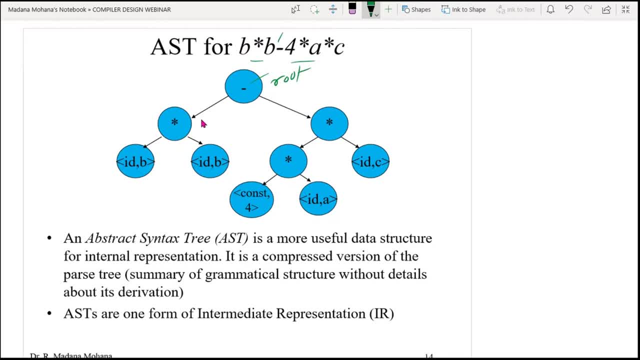 the left hand side what we are having again into operator. So here one point you can remember: the root and all internal nodes are labeled with operators. then all the lift nodes are labeled with the operands. here you can observe: So minus is the root node, then into is another interior node. 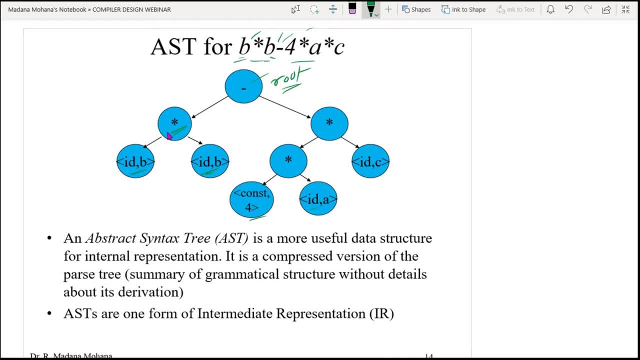 So minus left hand side into again it has b into b left side is b, right side also b. then after minus right hand side again we are having two intus 4 into a, into c. So again you can take into as the interior node left hand side of this, for example. again 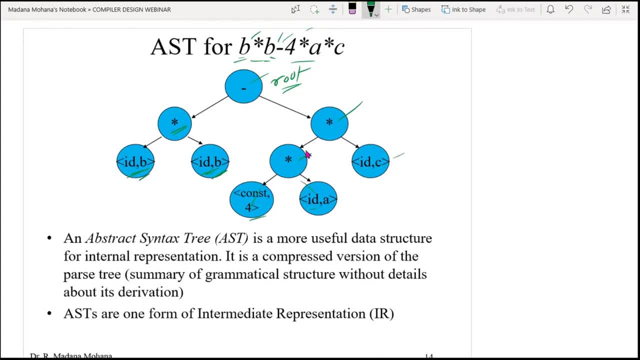 into a, 4 a, then right hand side c. Now this is called a syntax tree. now you can see the previous one is derivation tree are parsed. this is the syntax tree. the differences between these two you can observe carefully here. no grammar is used here, only the string is used here. 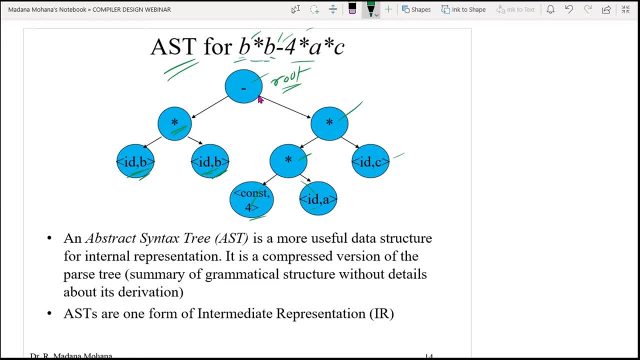 So in the derivation tree are parsed tree the root and internal nodes are labeled with grammar variables. So in the derivation tree are parsed tree the root and internal nodes are labeled with terminals and leaf nodes are labeled with terminals, whereas in syntax tree the root. 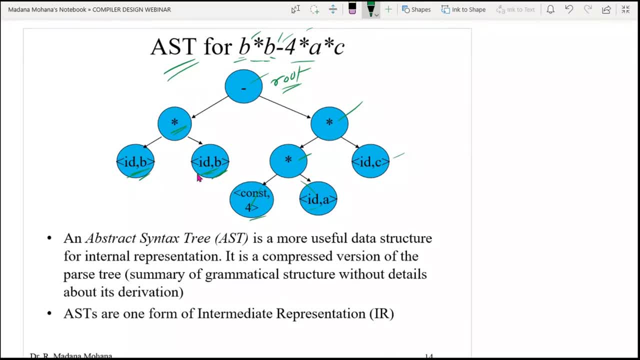 and internal nodes are labeled with operators, then the leaf nodes are labeled with operands. So this is the difference between derivation tree and parsed tree. So this abstract syntax tree is actually is one of the form of intermediate representation, the intermediate code, fourth phase. 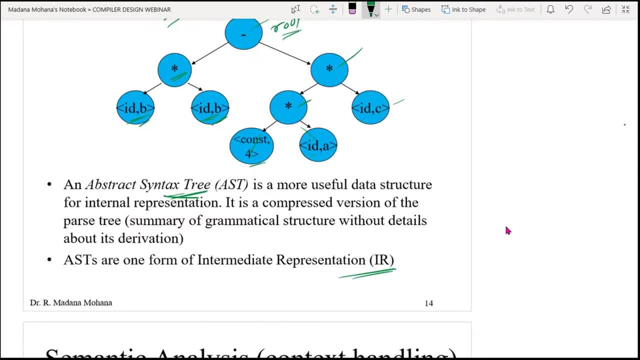 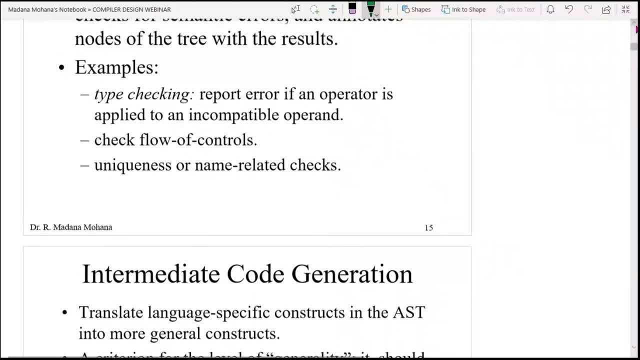 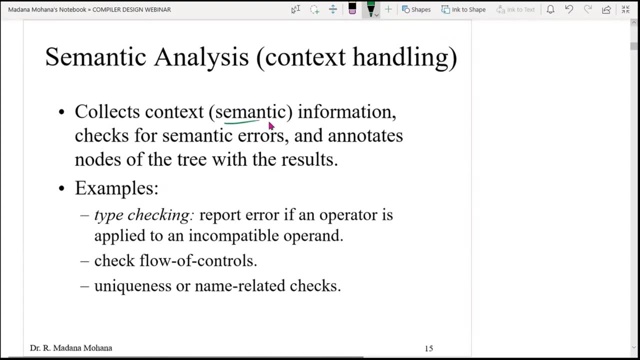 So what is the output it produces? so one of the intermediate representation is this syntax tree, then semantic analysis. we already mentioned what it provides. semantic checks, context handling, So collects the context, means semantic information, checks for the semantic errors. and annotates means labels nodes of the tree with the results. for example, type checking is one of the important. 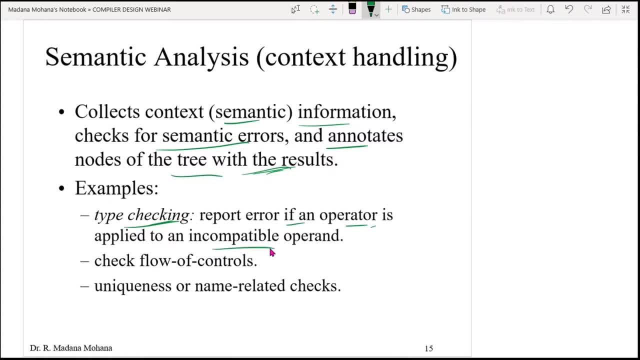 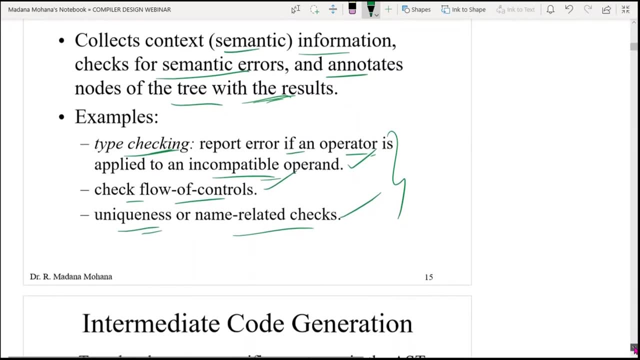 concept report error if an operator is applied to an incompatible operand. and also check flow of controls, Then some uniqueness or name related checks. these are all some of the examples of semantic actions. Then intermediate code that we already explained, that unnotated abstract syntax, tree constructs. 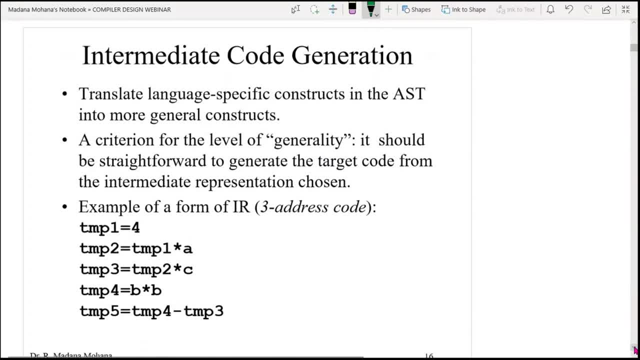 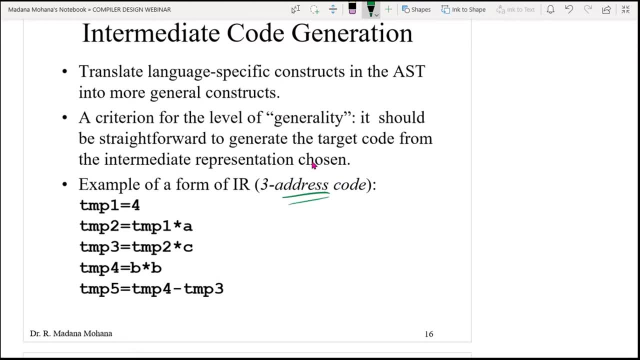 that can be converted into some intermediate representations. abstract syntax tree is one of the intermediate representation in addition to. we are having three address code. just now we explained, So this is one example. the same three square minus four ac. this is the three address code for this. first we have taken that constant in one temporary that can be multiplied with. 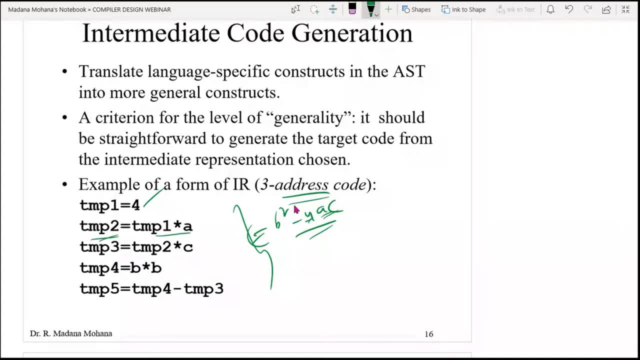 a that is temp one into a that is stored in another temporary. So then that can be multiplied with c. so this one, this one, into c that can be stored in another temporary. So then the left hand side, b into b that can be stored in another temporary, then the 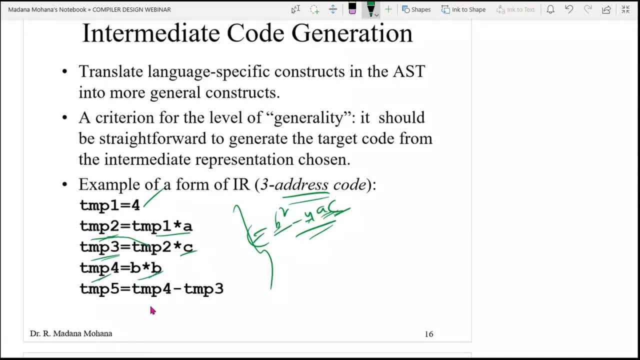 temp five, the result equal to this. one temp four minus temp three. this is the actual three address code. this is one intermediate representation, So here some temporaries may be removed, or because here one, two, three, four, five temporaries are used, So here instead of for example here temp one directly, you can take some four into a. 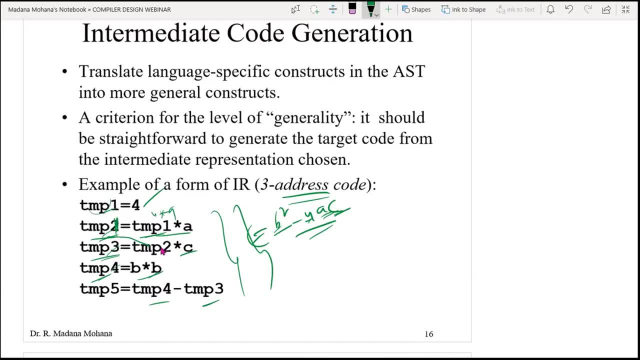 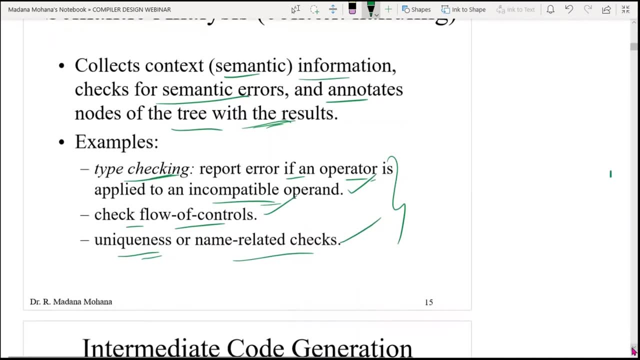 as temp one, then one temporary is optimized like wherever possibility, So we can optimize the temporaries. then that is called as optimized temporaries. So this is the optimized intermediate code, that is three address code. that is the code optimization. So then finally code generation in code, code generation what we will do that optimized. 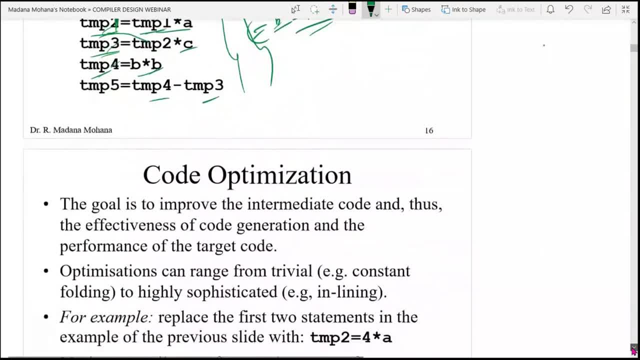 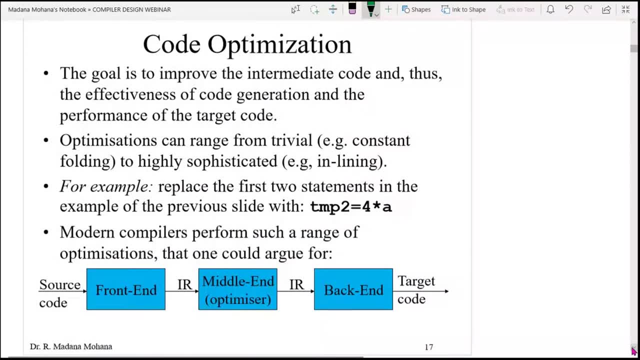 three address code that can be converted into assembly language program directly. we can't convert into machine level language, So it converts into assembly level language. by using assembler we can convert assembly language into our machine level language. So this is the code optimization. just know, whatever we explain, it takes the the front. 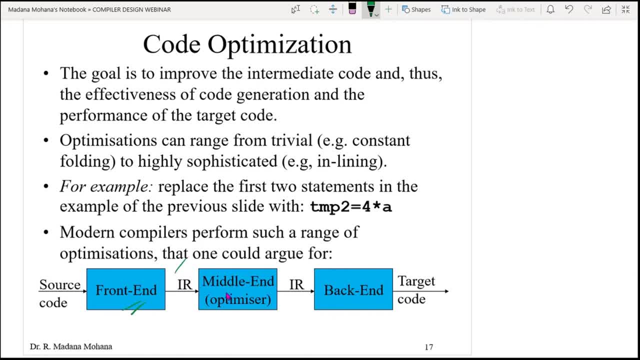 end, then output of the front end intermediate representation. So optimizer is the middle end, which is optional, actually by default optimization taken place again. it produces same intermediate code with optimization, then back end, what it takes. the optimizer code is converted into target code. here the target code is in assembly language. 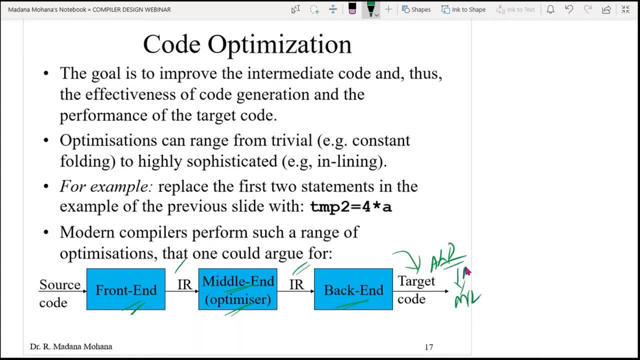 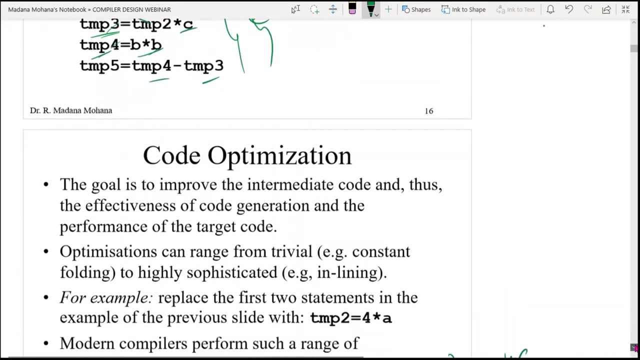 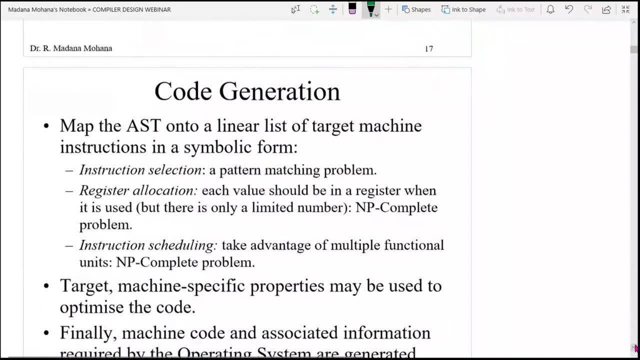 program that can be converted into machine level language. So this diagram shows the role of code optimizer in the compilation. okay, now then coming to okay. this is the detailed explanation about all the phases, with example. then code generation: first it produces assembly language program by using some basic code. 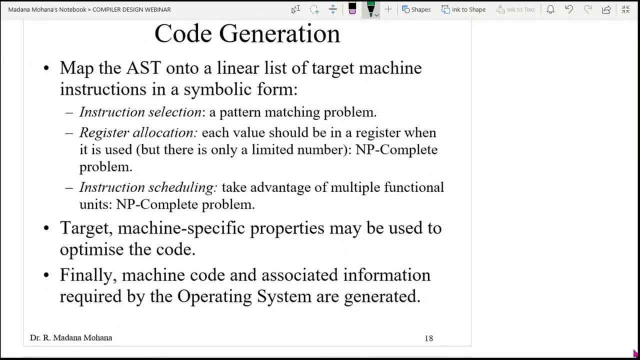 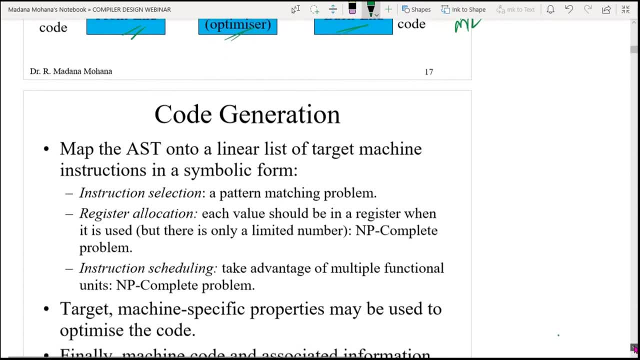 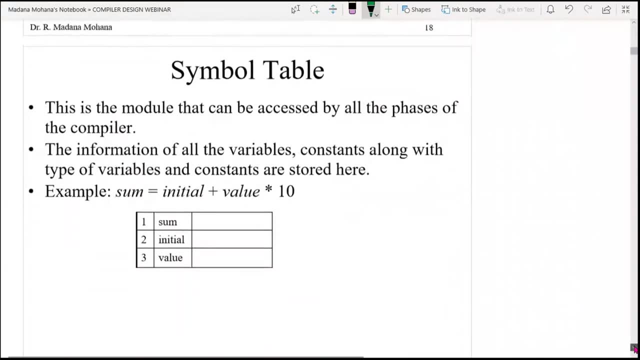 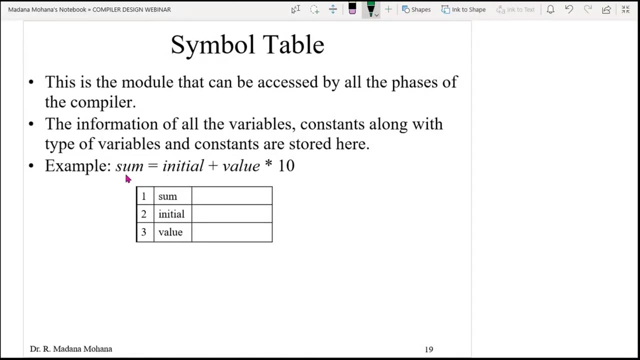 Okay, So let us see some basic code generation algorithms. okay, now we will move to the lexical analysis phase, some important concepts we will discuss. So before that, let us see some more points related to symbol table. in the compilation model we have seen the symbol table, one example here you can see. I told at that time the symbol. 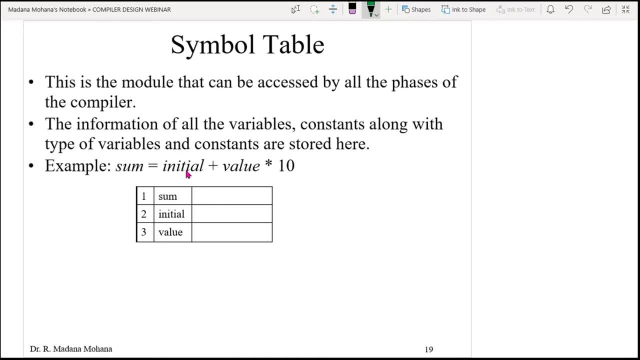 table is a data structure which is used to store the information about pages. what type of information is stored? Actually, identifiers related information can be stored into symbol table. for example, in this we are having: sum is one identifier. initial is one identifier. value is one identifier. 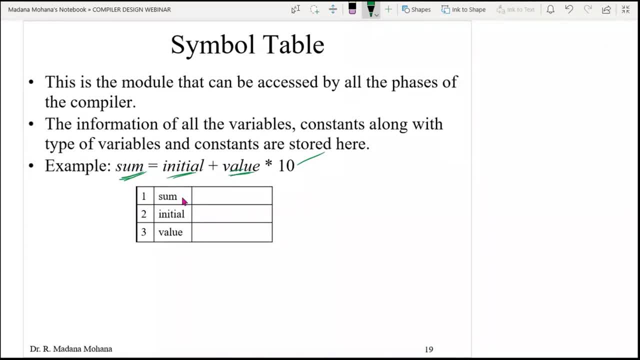 So now, in some particular locations, it stores all the identifiers in separate locations. for example, the location one sum, then second location, initial, third one is value, like this: okay, now for any phase, the information regarding these identifiers required It takes from the symbol table. this is one simple example of so this is the module that 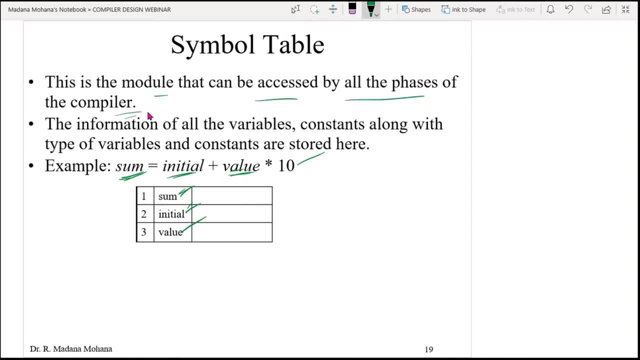 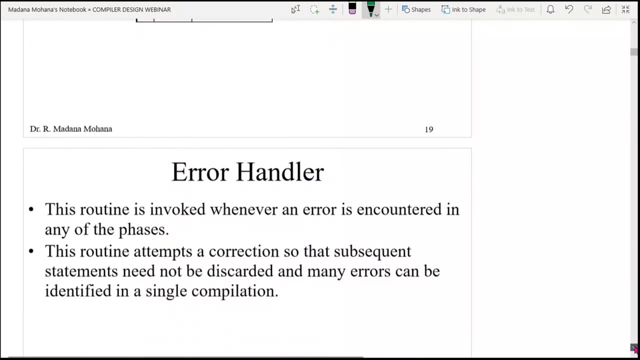 can be accessed by all the phases of the compiler. the information of all the variables, constants, along with type of variable and constants, are stored here. that is, simply tokens. the token information is the one example of symbol table representation. then coming to the error handler. So what is the error handler? phase wise, it encounters errors, then by invoking some error, 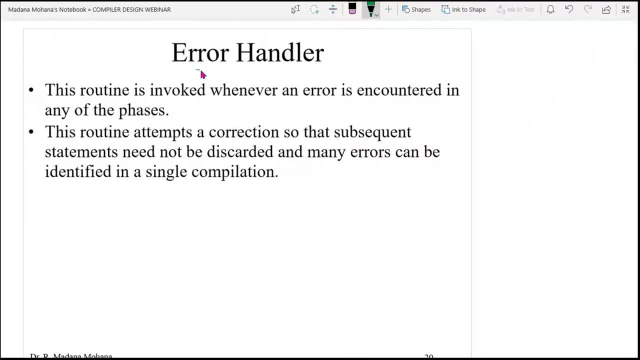 recovery strategies, those can be handled. So error handler invoked whenever an error is encountered in any of the phase, all the phases connected to the error handler. each phase encounters errors, So this routine attempts a correction. that is error correction, so that subsequent statements need not be discarded. 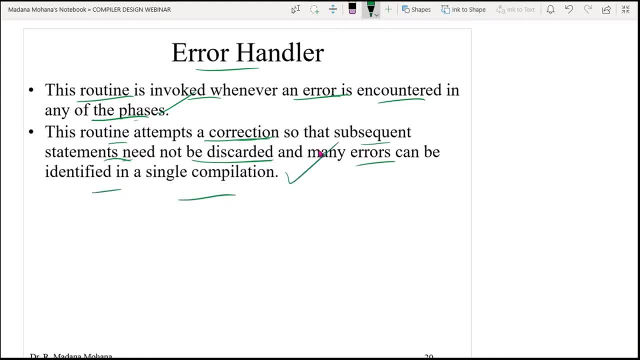 And many errors can be identified in single compilation. So if you want to rectify the phase wise errors, then finally, whenever you are compiling your program, it is very difficult to trace all the errors. So, finally, that is why, phase wise, if you can rectify the errors wherever error is occurred. 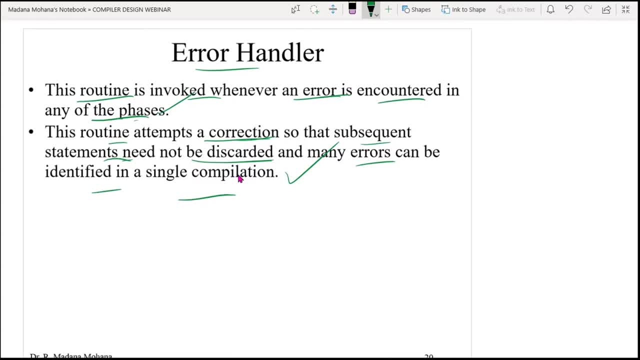 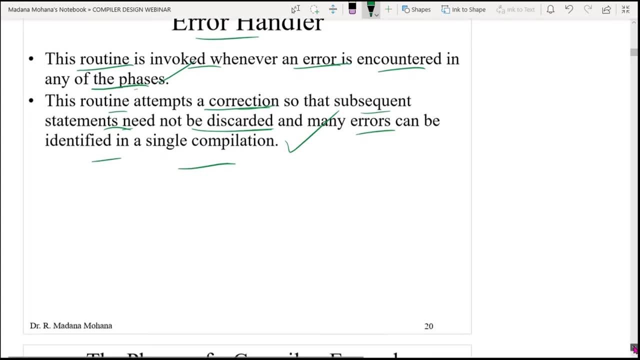 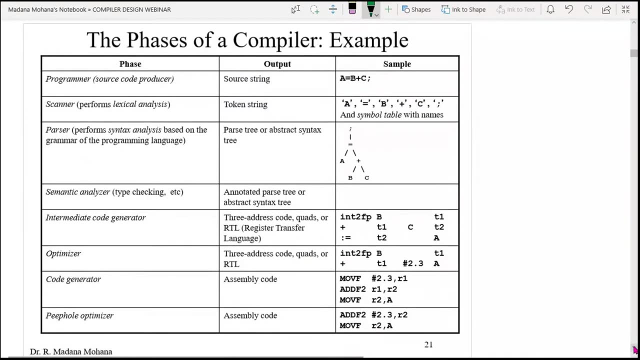 then that can be discarded, if any error statement, by invoking some error recovery strategies, then it is easy to compile your program files. So, finally, instead of struggling at the end, ok, now, finally the glance: the phases of compiler. whatever I explained here, all the phases at one place, are shown in this table. 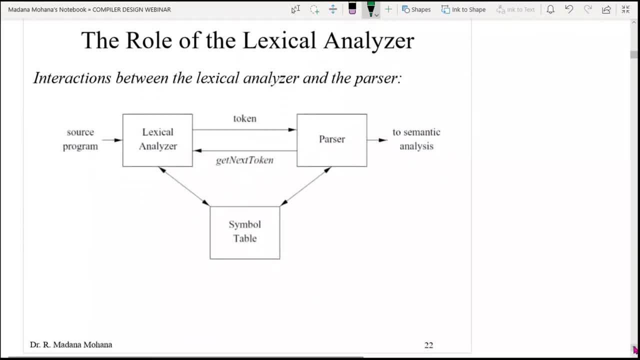 any example you can take So you can convert into phase wise. so that is the phases of compiler, with detail explanation about all the phases. So then, coming to the lexical analysis or scanner. here, quickly, we will see the role of the lexical analyzer or scanner. 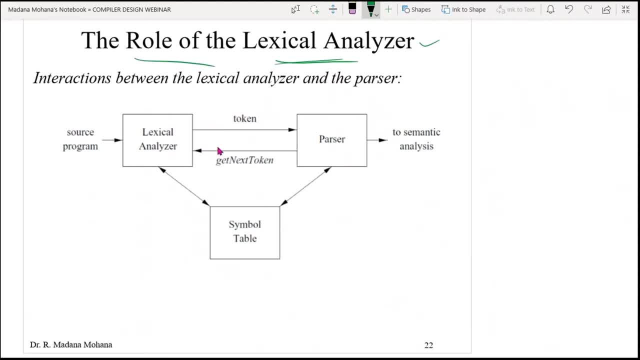 So this diagram shows in the compilation model what is the role of lexical analyzer, how it is connected to the next phase, that is, the second phase, parser or syntax analysis. Here you can see for every phase. you can keep the compilation block diagram as the base. 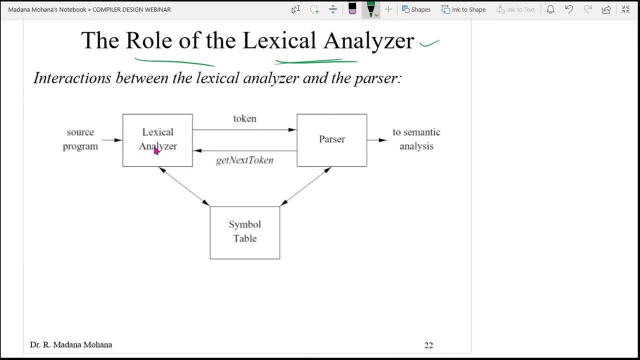 Whichever the phase we are discussing or studying, take that phase, then what is the next phase? then how it is connected, What is the input and output? only these things you can keep in your mind. Now we are talking about. lexical analysis is the first phase. what is the input of lexical? 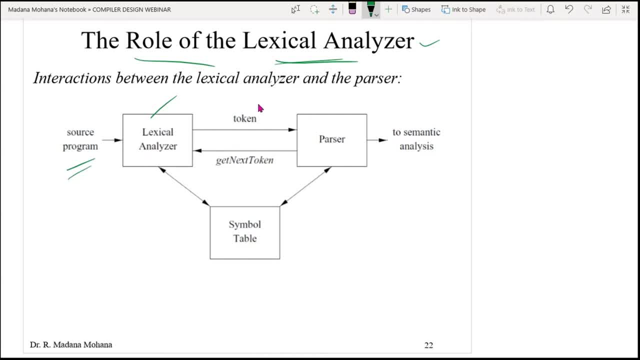 analysis source program. then what is the output of lexical analysis that we know token? this is connected to the second phase: parser or syntax analysis. Now the parser or syntax analysis take input as token, then produces syntax tree that can be connected to the next phase. So here the next phase. no need to draw other phases, just we can give what is the next phase. 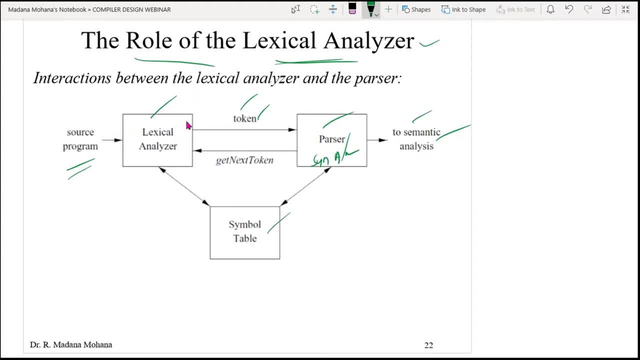 that say: Then commonly symbol table is connected to all the phases. here you can see, lexical analyzer produces output as token, then token will be considered as input to the parser or syntax analysis. So then that token is represented into hierarchical form, that is parser derivation tree. that will 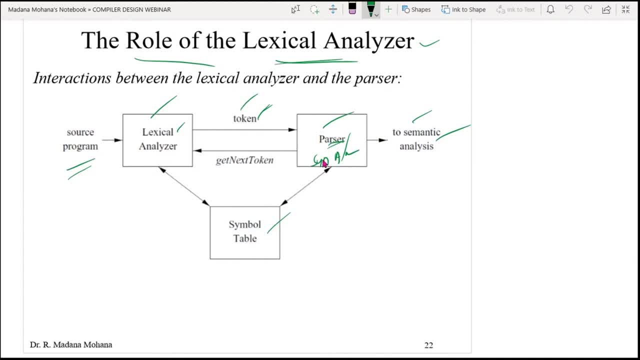 be given to the semantic analysis phase. Then again It asks for next token. get next token from the lexical analyzer, like every token that can be represented in the hierarchical form, then any information required for the lexical analysis or parser, like identifier, constant, etcetera, that can be stored in the symbol. 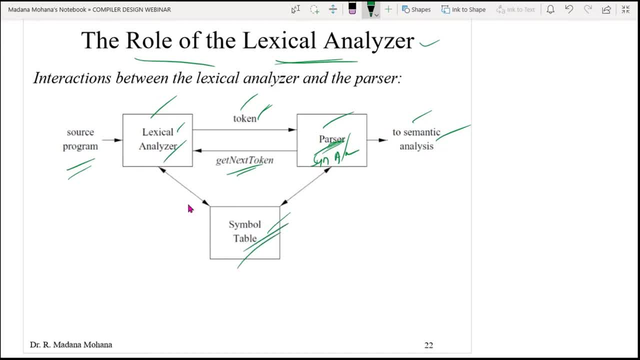 table that can be accessed in both directions. So lexical analysis stores information here. symbol table gives the information to lexical analysis. parser stores information on symbol table. symbol table gives information to parser- Both way communication. So this is the role of the lexical analyzer in the compilation model and how it is connected. 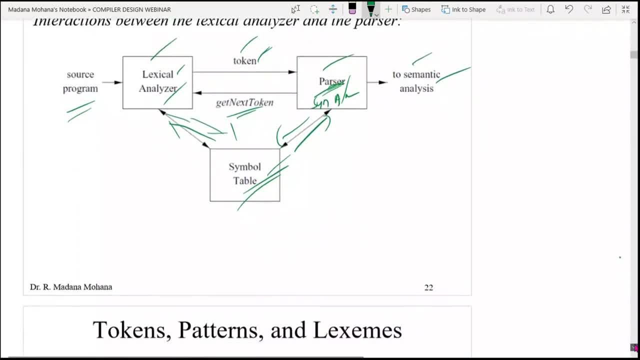 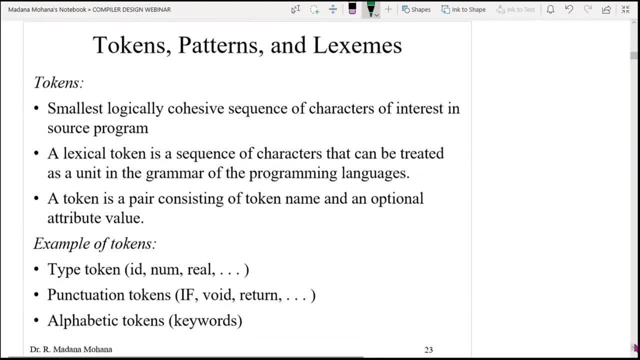 to the next phase, that is, syntax analysis or parser. Ok Now, here we discussed about the term tokens, but inner centric token. we are having other definitions also, because in the lexical analysis these are all very important, even some short sentences. you will get defined token pattern lexemes or for the given source program or 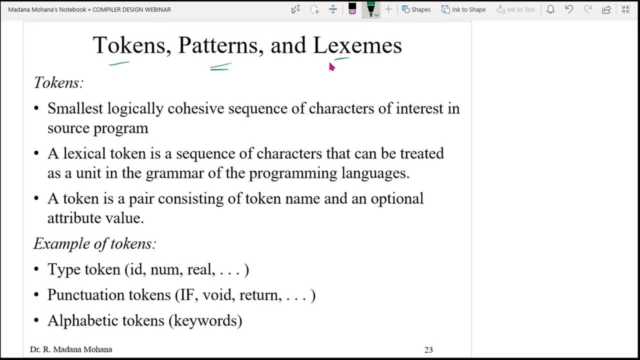 input find what are the tokens, what are the patterns, what are the lexemes? that is right. we have to know the definitions and examples. So token we already discussed. So again you can recall once what is the token smallest logically cohesive sequence of characters of interest in the source program: see smallest logically cohesive sequence of. 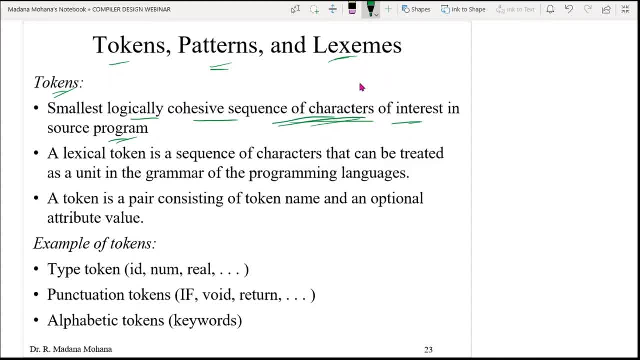 characters of interest. That means all identifiers are one group, all constants are one group, all keywords are into one group, all operators are into one group. So these grouping of sequence of characters are called as tokens, So a lexical token. what is the output of lexical analysis? token is a sequence of characters. 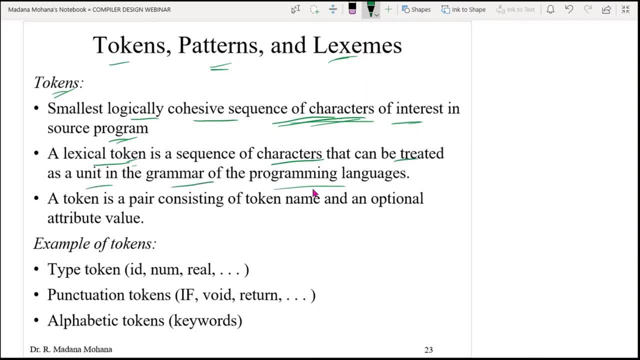 that can be treated as a unit in the grammar of the programming languages, A token that can be represented as a pair actually consisting of the token name and an optional attribute value, like this. So we can represent. So this is a token: for example, id here value. for example, here, id one comma x, x is the identified. 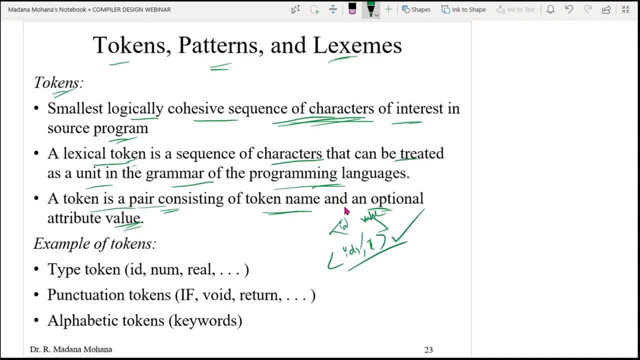 one. this is the representation of token. So examples of token, for example type tokens identified. So then number, then real etcetera, Then some punctuation type tokens, Then some punctuation type tokens like uppercase. if then some void return, then alphabetic tokens. 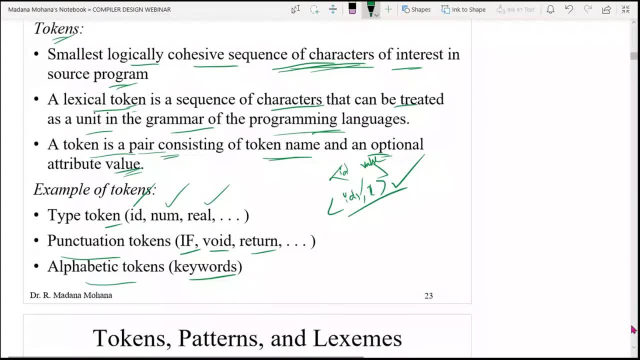 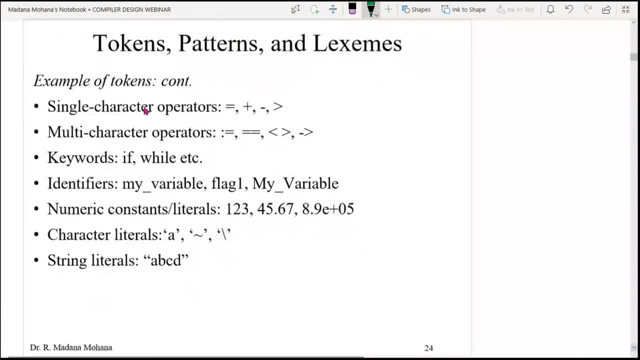 like keywords, then even some other operators also there operators also, you can consider each other, tokens, single character operators like equal plus minus, all the relational operators, only single character, multi character operator, colon equal or double equal, not equal. So then Then again keywords, some if while for etcetera, then identifies with our user defined identify. 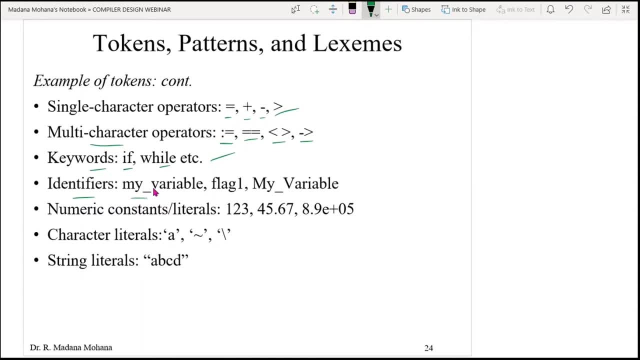 my underscore variable. the name should be in single. we want combine multiple strings. you can use underscore, some flagged one, even identifier consisting of starting with letter followed by digits, then repetitions. also my underscore variable, etcetera. this is a user defined identifier. Then some numeric constants are literals, like one, two, three, forty, five point, six, seven. 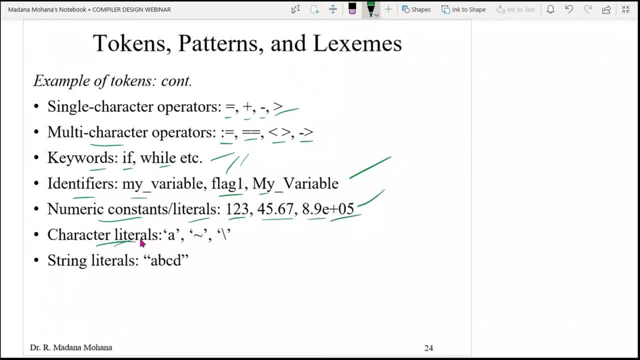 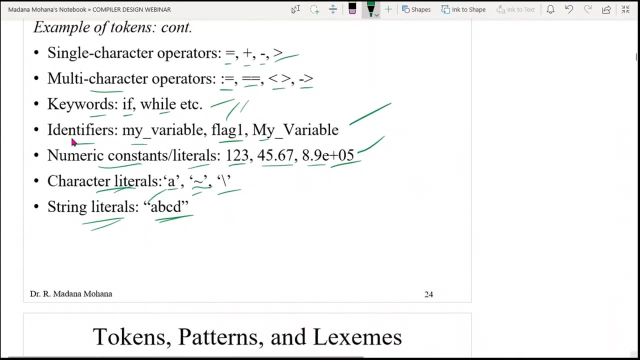 exponential value, eight point nine, e, power, etcetera. Some character literals within single quotation, suppose a similarity. then r, etcetera, then some string literals. that string can be within double code, like. these are all some of the examples of token. see: by seeing all these you are programming language, any programming. 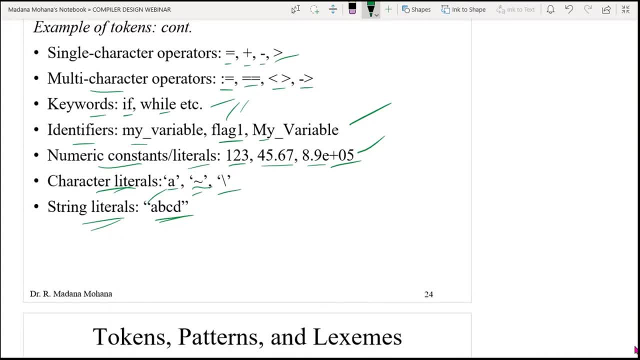 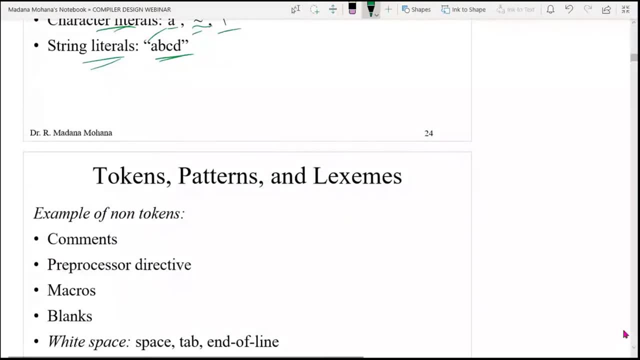 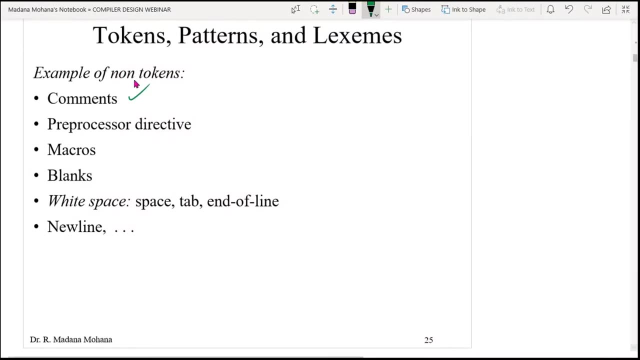 language, any program Which is combination of all these type of tokens only. ok. now there are some non tokens also. Let us see some of the examples of non tokens. so comments are not tokens. these are all non tokens. then preprocessor directives also, like has, include, has defined, these are also not. 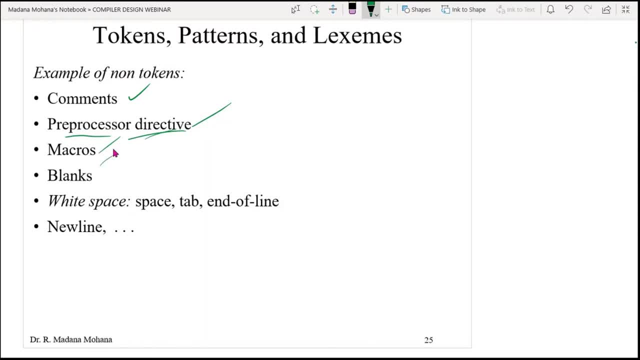 tokens. these are non tokens. then some macros: blank white space space tab. end of line. new line: these are all not tokens in any programming language any of these are all the. these are all not tokens which are called as non tokens. so here you need to identify only tokens in. 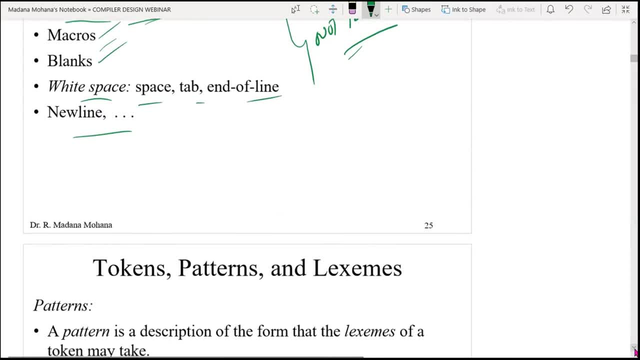 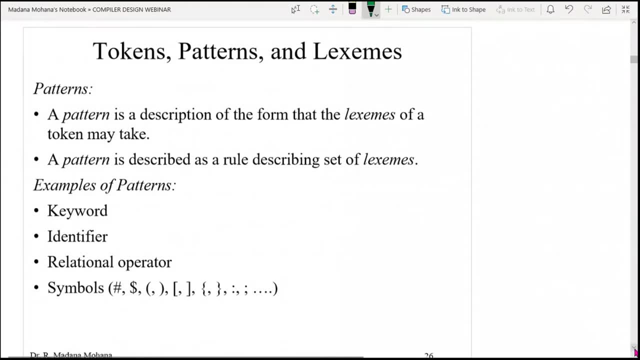 the program. then, coming to the other two terms, patterns and lexemes. so what is the pattern actually? so, pattern is nothing but in the given source program, by reading the input, character by character, what is its name? actually the description? actually the description, a pattern is a description of the form that the lexemes of a token may take. what is lexemes? 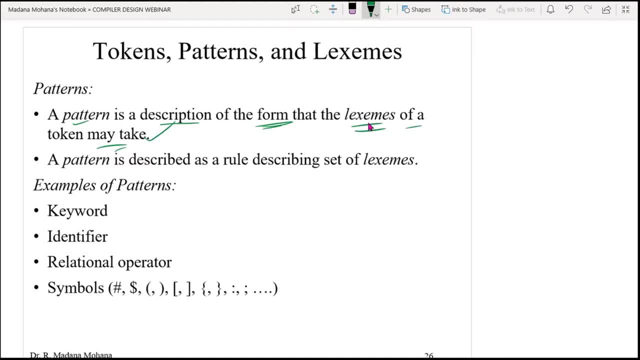 the actual values in the given source program are called as lexemes. for example here: x equal to y plus z into ten, x equal y plus z into ten. these are the lexemes. Then what is x? what is x actually? this is identifier. the meaning identifier: y is also. 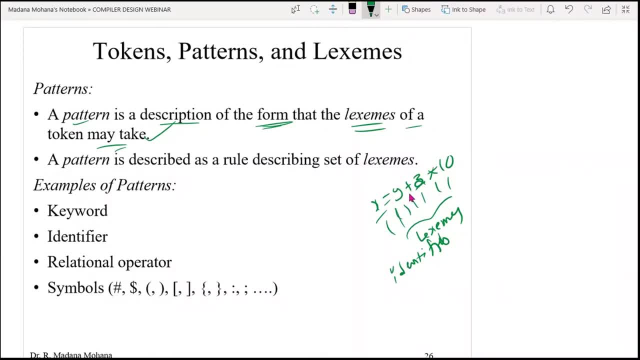 identifier z also identifier plus is addition operator, equal is assignment operator into the multiplication operator and this constant, the names, the descriptions of the lexemes, are called as patterns. Then what is token? You can represent the token like pair format, the token name, comma value. so there is token. 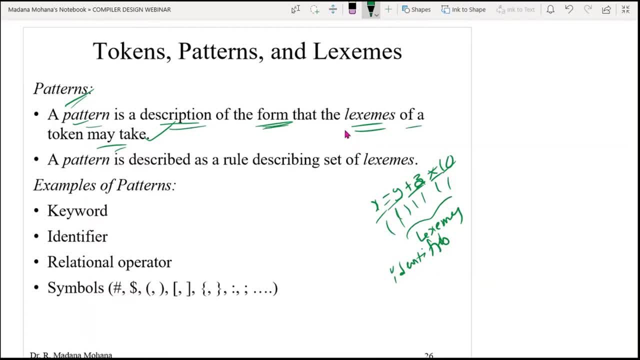 now you can see. a pattern is a description of the form that the lexemes of token may take. a pattern is described as a rule describing set of lexemes, for example, examples of patterns. what type of patterns are occurred in any program? that means tokens, only keywords is. 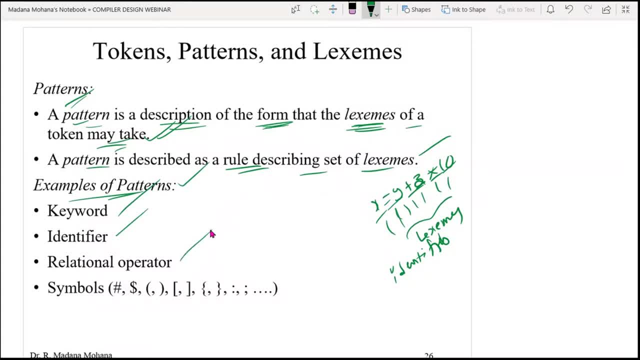 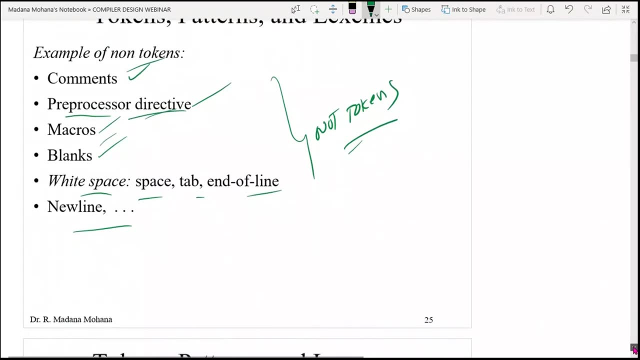 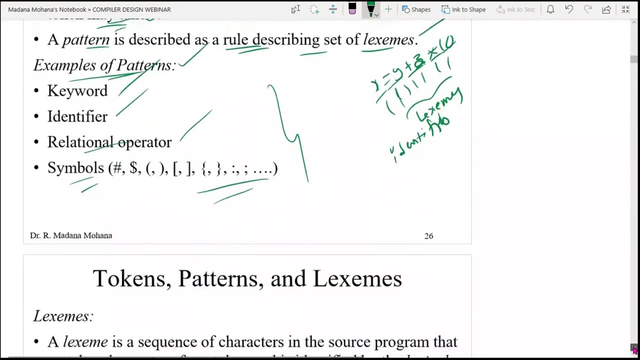 one pattern identifier is one pattern Operators, also some categories: relational operator, arithmetic operator, etc. then there are symbols. these are all some of the types of patterns. then lexemes: in the given source program, whatever the values from left to right, all are called as lexemes. 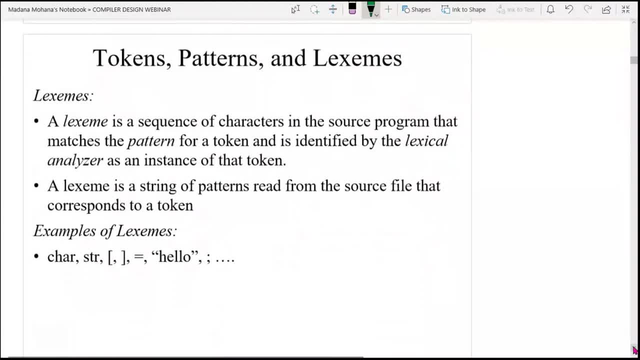 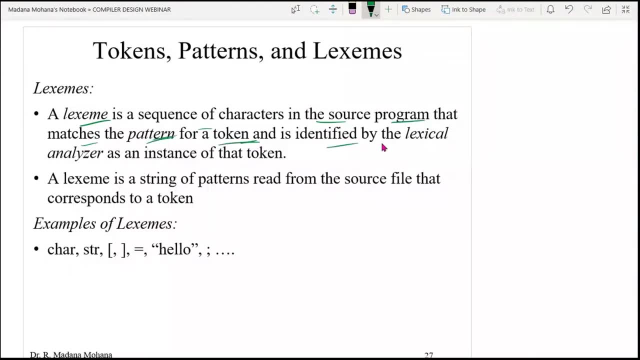 A lexemes sequence of characters in the source program. as it is. you can take sequence of characters in the source program that matches the pattern for a token and is identified by lexical analyzer, which is an instance of the token. A lexemes is a string of patterns read from the source file that corresponds to a token. 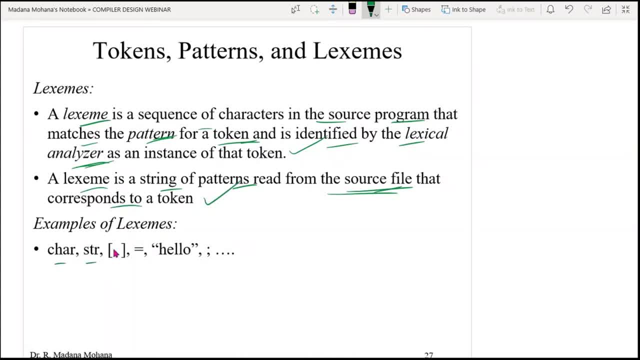 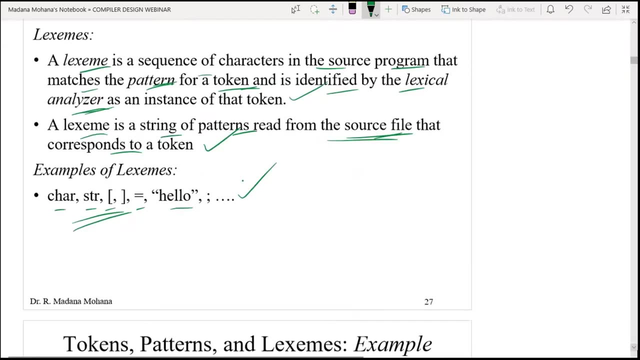 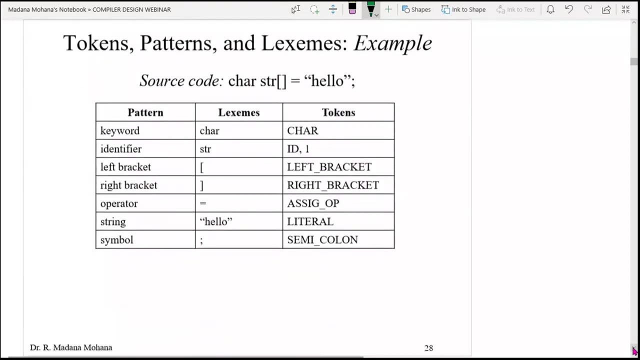 for example, here you can see characters, string, the array, brackets, whatever, each and every thing you have to consider. in the given source program that is called as lexemes, then the description of the lexemes is called as pattern, Then the pattern representation by grouping, that is called as token. now all three at one. 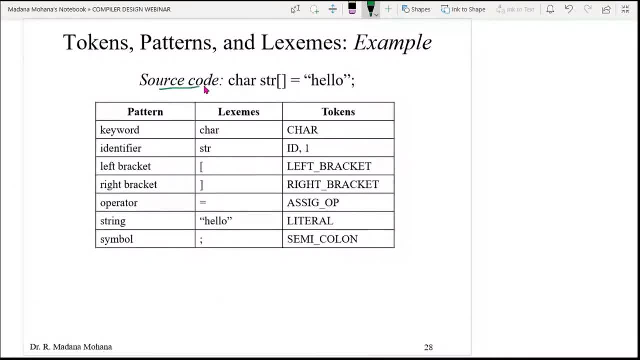 place. let us see this example: So source code equal to character, array type and what look ended with every column. So let us see Now in this, now you can identify what is pattern, what is lexemes, what is token first to pattern before pattern, first you can write down lexemes as it is why? because from left. 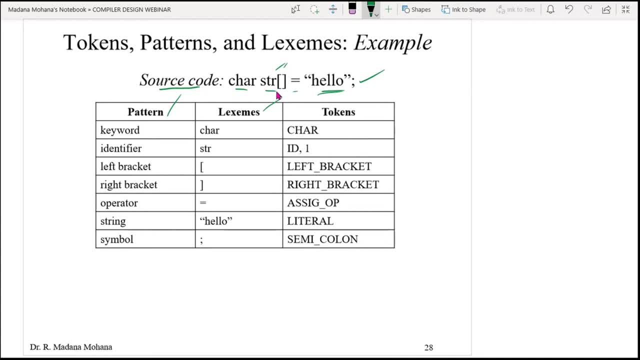 to right in the given source you can separate all characters. So here first we are having ch, here this is one type, data type, so separate type, then string is one name of that character, whatever we creating the array string, then array, open bracket, then closure bracket, next equal assignment operator, then literal in the literal we are. 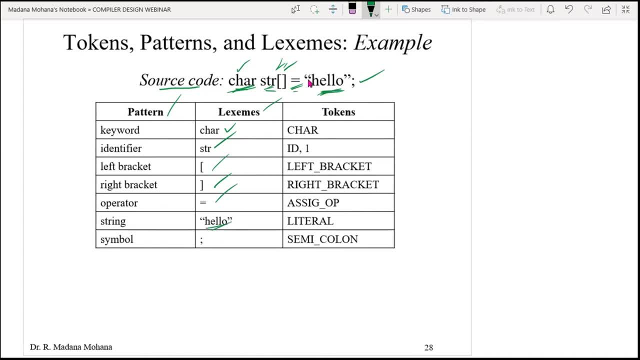 having string so that you can include. we can't separate the quotations: open quote, end quote and hello why? because this is a literal, can be treated as single string. include as it is ended with semi colon. now, let us see So all we have listed. now you can see one, two, three, four, five, six, seven, total seven. 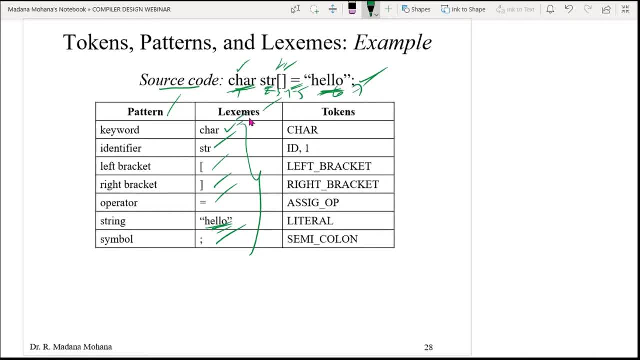 items are listed. These are all called as lexemes. now you can describe the names of these lexemes. what is character? this is actually keyword. what is str? this is identifier. what is this bracket? we will call it as array bracket, left bracket, or sometimes we will call it open bracket. 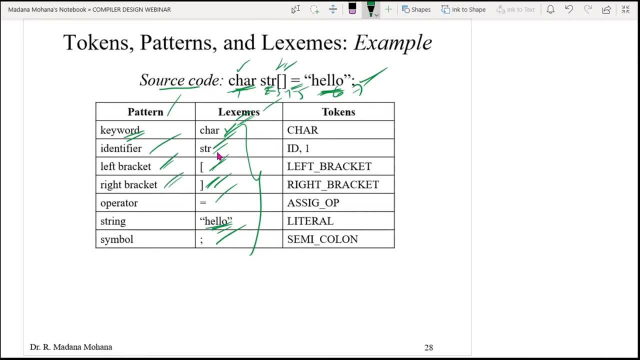 then this is array closure bracket. that is right bracket and equal. this is operator. then hello, this is actually literal. the string, then semi colon symbol. So the description is called as pattern. now, based on the pattern, you can define the tokens. now the tokens are represented. now you can see the keyword. actually keyword can be represented. 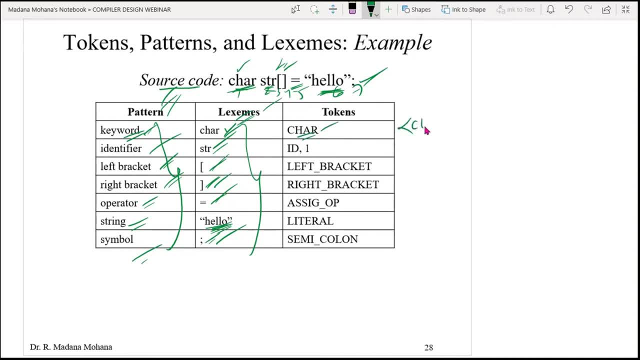 with the name character. actually you can represent like this: thar thar comma value. this value is actually optional wherever it is required. What you can use is the token representation. Generally tokens are represented with uppercase letters for discrimination. then identify: actually. here you can see id comma one. here two values are there. this is the name of the token. this. 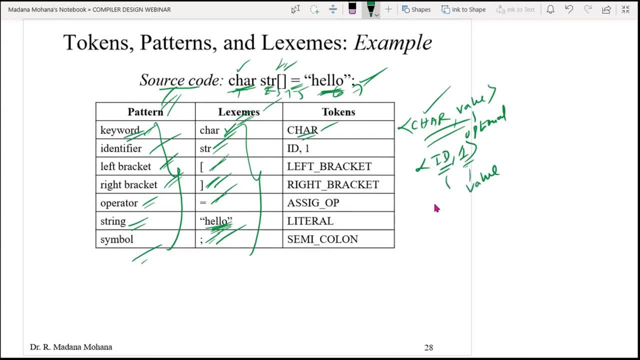 is the value pair, so name, comma value, then left bracket, so left underscore bracket, then right bracket, right underscore bracket. then operator switch to the name of the operator. actually the token exactly specifies the names. so here what is this operator called? assignment operator, in short form, a, s, s, h, d, underscore op, then this string actually hello. 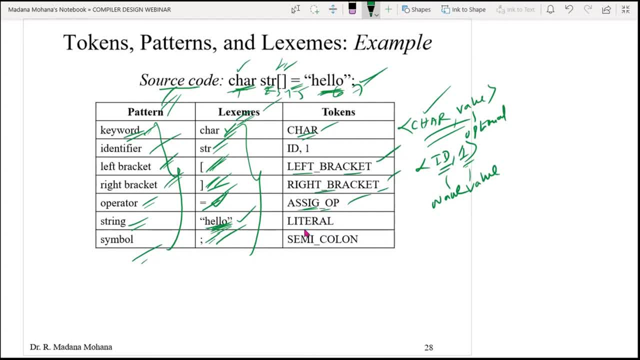 what is exactly name of the token? literal, literal category, then the symbol. what is the name of the symbol? semi colon, semi underscore, colon, like this. so any given source, string or input you can identify. what are the patterns, what are the legions, what are the tokens? first, 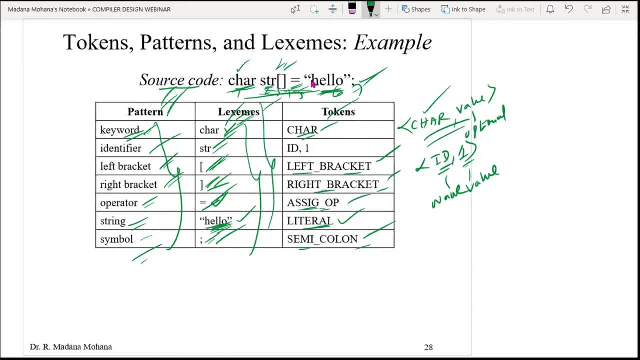 you can list the legions as it is in the given source program by separating all. then you can provide the description of these legions. that is pattern. then you can represent into tokens with specific names. so that is the token pattern and legions. so this is an important 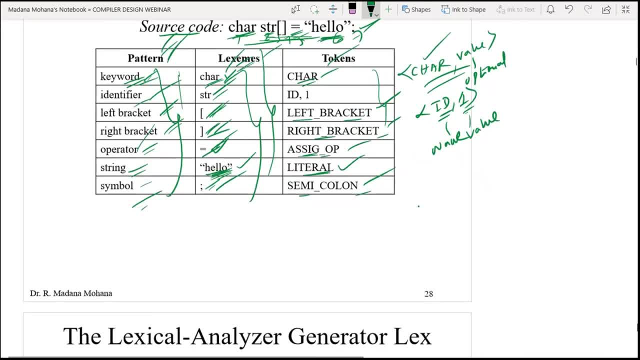 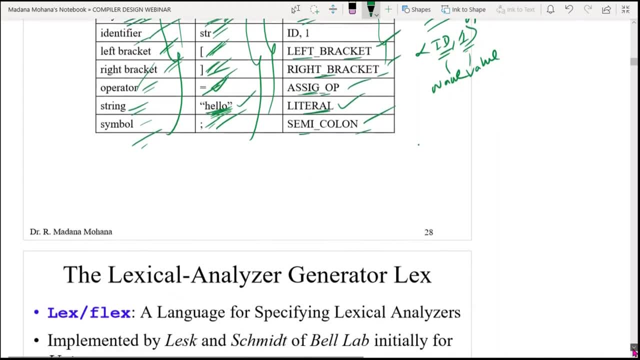 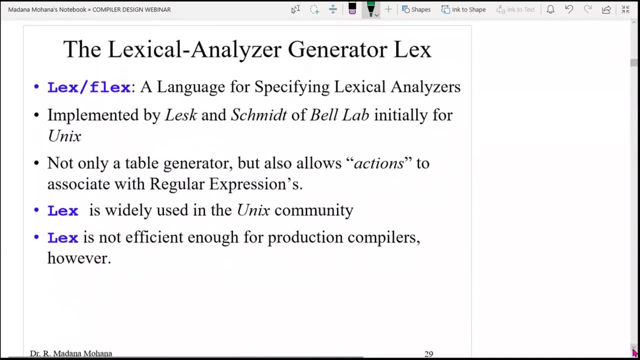 one even for lexical analysis. further, by using this you can represent these tokens into regular expressions. Then regular expression to will construct automata. then by using automata we can recognize the tokens, whether these are all valid or invalid. acceptance of the tokens. ok, now another important concept: in lexical analyzer or lexical analysis, we are having automatic lexical analyzer. 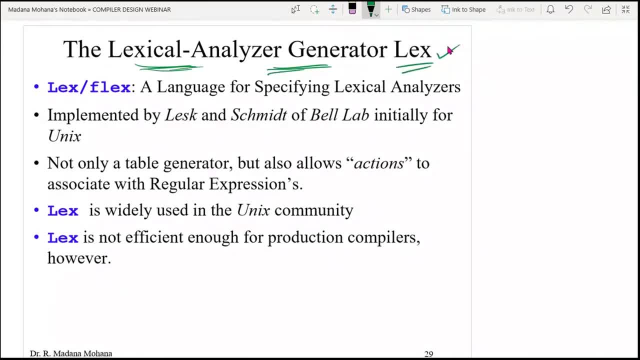 generator, one tool which is called as lex tool. sometimes in examination they will ask this question also. explain about the lex tool, This tool, or write the lex program for recognition of tokens, etc. Just briefly we will see about this one. so actually lex or flex in the unix or linux platform. 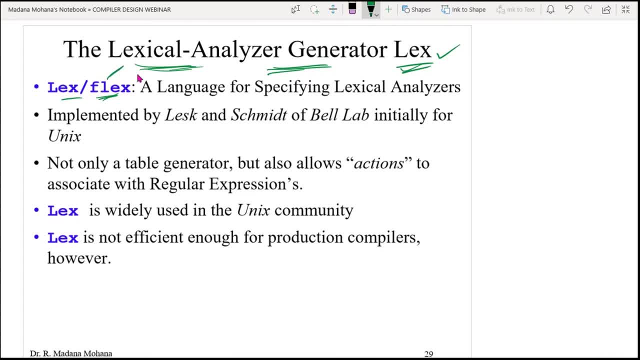 the tool name is called as flex software, automatically it will commit as inbuilt. inbuilt tool, so lex or flex, a language for specifying lexical analyzer. this can be implemented by the scientist lex and skimming at bell lab, initially for the unix platform. so not only it is a table. 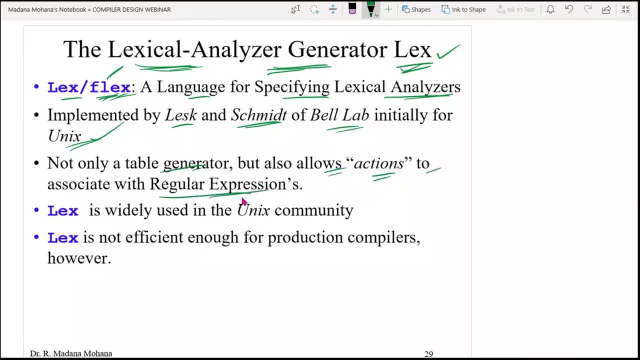 generator but also allows actions to associate with regular expressions. so lex is most widely used in the unix community. then lex is not efficient enough for production of compilers, however, so some aspect few. so this is good one, especially in the unix community. So let us see the example of the lex tool. 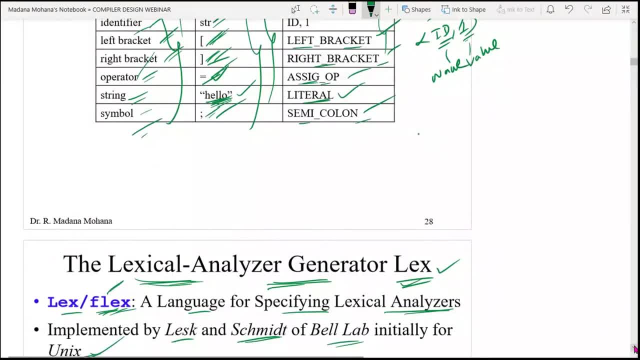 So let us see the example of the lex tool. So in the example of the lex tool we have a lex program, which is a program that can be written in the unix and linux environment. If you can see the working of lex tool, the diagrammatically, the structure or the role, 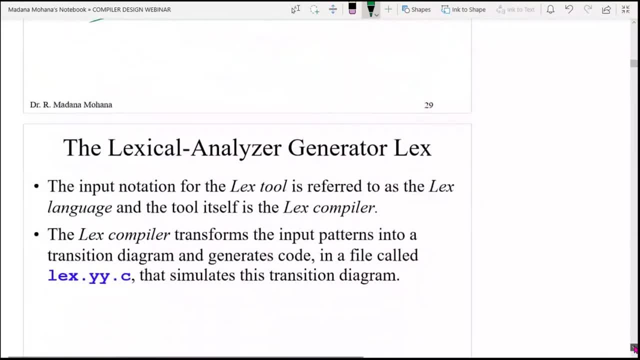 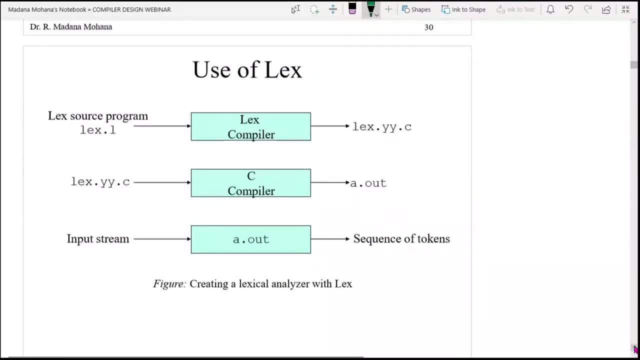 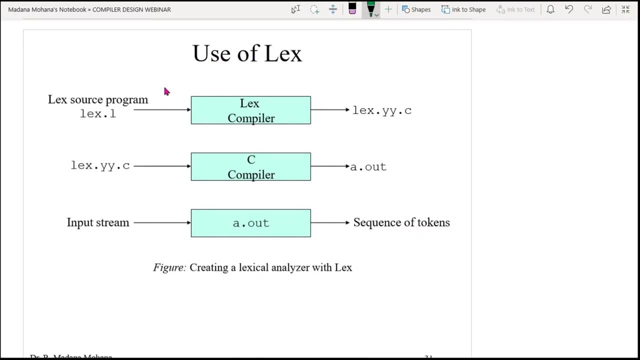 of the lex tool is represented here. let us see the diagram. So in the examination compulsory you have to write this diagram whenever you will get question on lex tool. So this can be done in the following steps. first, the lex program that can be written. 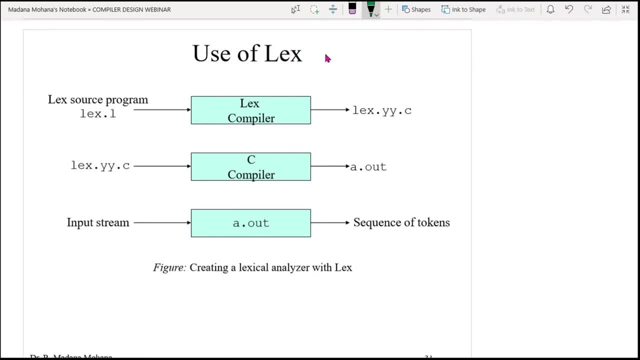 in the unix environment That can be written in a language which is called as lex language. the extension of lex language is dot l, So file name dot l. So for example, lex dot l is the source program, then that can be compiled by using lex compiler. 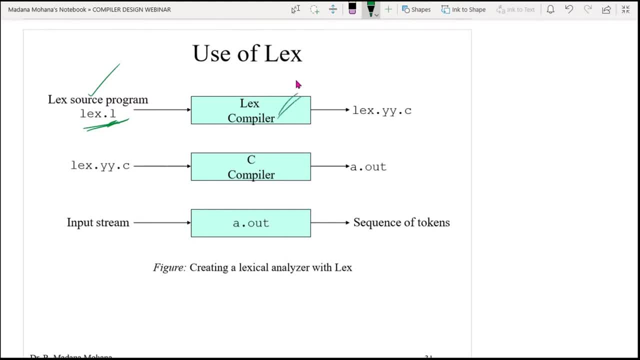 in the unix or linux it will comes the default compiler, So we no need to install separate software. so just we have to call the software in the unix or linux environment. Then using the compilation commands so we can compile the lex program. So using lex compiler, the source language that can be written into lex language converted. 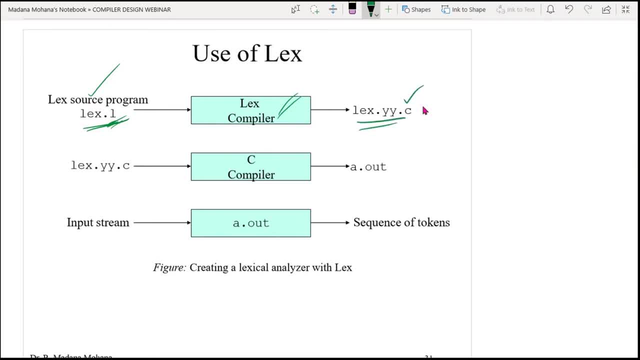 into other form, So that form is called as c. actually this is c language, So the lex language is dot. l is converted into dot c directly. it would convert into object lex language to c language. So the output file name. by default it is created like this. 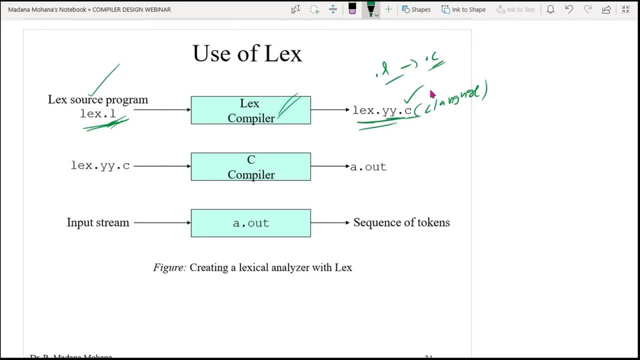 lex dot yy dot c. ok, now this is the c program actually, and c program is compiled using c compiler. Now the second step you can take, the c compiler input is the c source program which is the output of lex compiler. lex dot yy dot c. 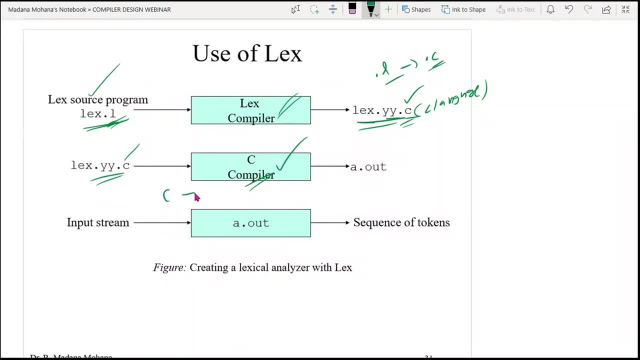 Now normal c program. whenever you can compile using c compiler, then it converts into some object object file. that is a dot out. This is object file. now this object file is again what it contains. it contains the input stream as the input and it produces a tokens sequence of tokens here. why? because lexical. 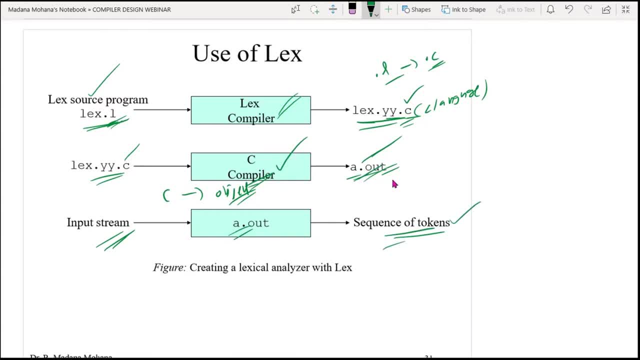 analyzer generator is part of lexical analysis, that is, automatic lexical analysis generation. the output of lexical analysis is token only. So whenever you are using any tool related to lexical analysis, what it produces output as tokens only. it won't produce as output as your target program. why? because this is 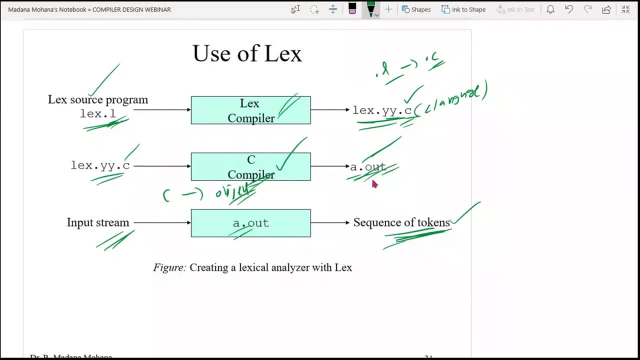 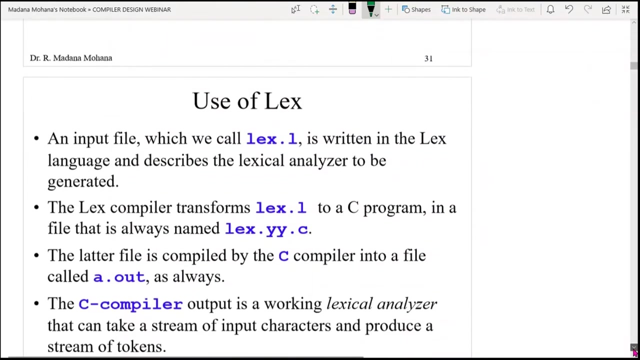 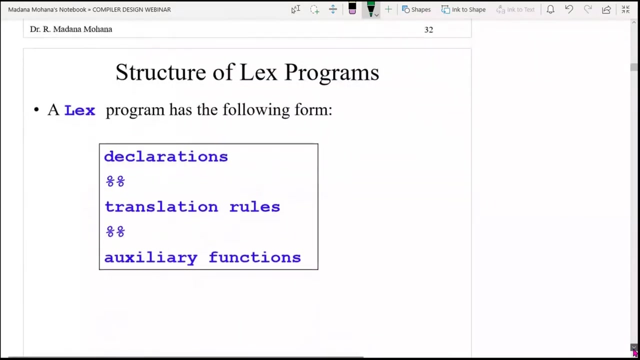 only lexical analysis related This is the use of lex tool, that is, creating a lexical analyzer with lex tool. then what is the structure of the lex program? So lex program, actually it consisting of three parts. so that is, first declaration, followed by acceleration, Then auxiliary rules, then procedures. it had three parts. the lex program has been had the 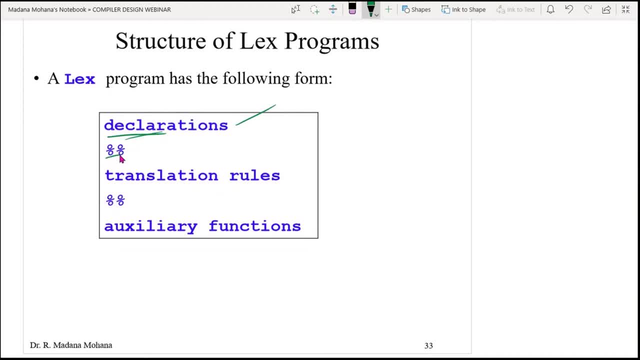 following three forms: first, declaration part within this symbol, double percentage symbol, so you can declare. then all the constants, whatever the tokens you can define, then the rules for the tokens, that we will call it as translation rules. there is second section, Then any methods of translation. 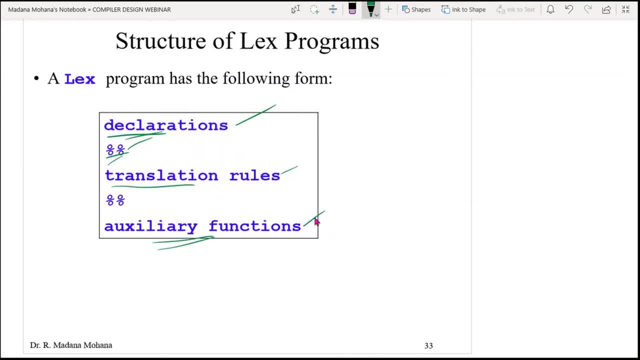 Then any methods are there that you can use auxiliary functions. are there so any lex program consisting of these three parts: the first part, declaration of all the manifest constants and all the tokens, etcetera. then the rules for identifiers, whatever, etcetera. you can define the rules and any methods you use to do so that methods are used in the translation. 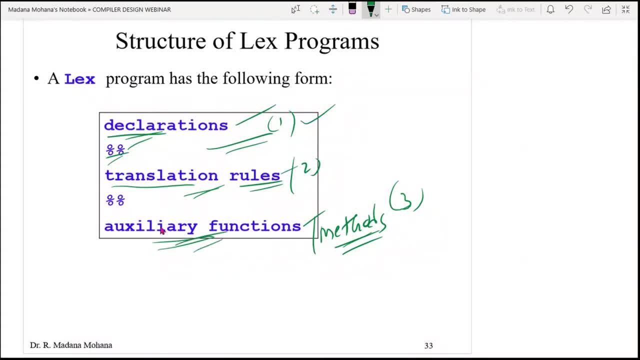 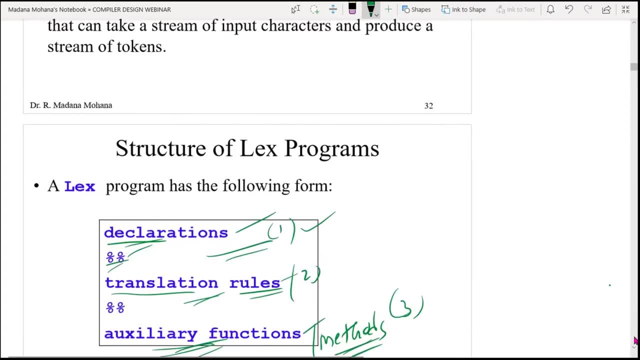 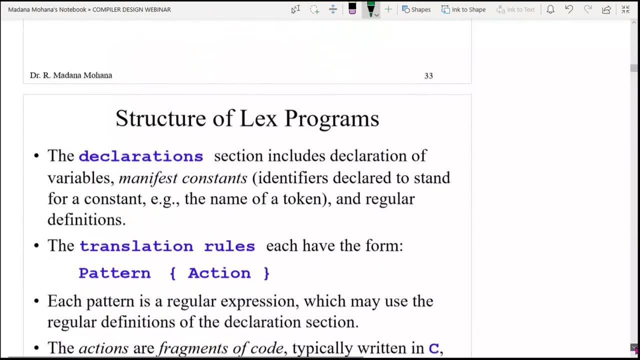 rules actually, Then the implementation of the methods can be defined in the auxiliary functions. This is the structure of lex program. ok, now that is all about lexical analyzer generator tool, then the role of the lexical analysis, then tokens, patterns and lexemes, etcetera. ok, 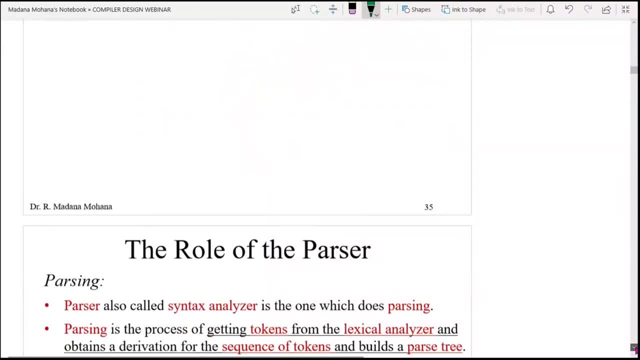 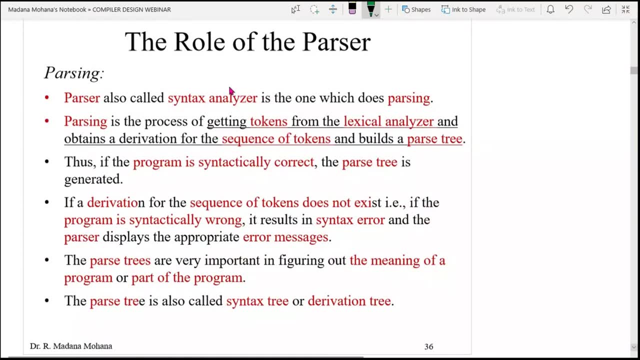 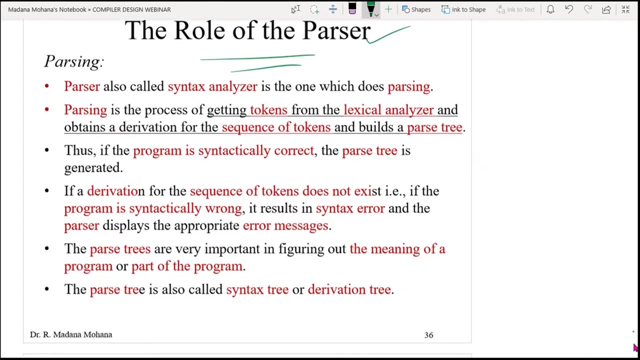 Now we will move to our next two phase, that is, syntax analysis or parser. this is very important Because here more problems are occurred in this. here also let us first recall the role of the parser or syntax analysis- see the diagram- the role of the parser. so in lexical analysis, 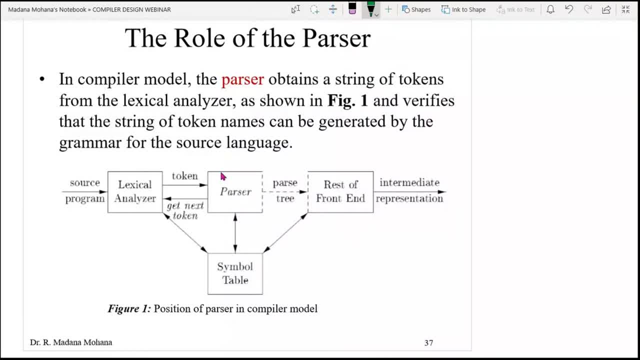 we already mentioned the similar diagram, so but here you can consider the parser, followed by next right part of the parser or syntax analysis. so up to this same in lexical analysis we discussed Now after parser what it contains actually the semantic analysis, intermediate, code generation, code optimizer, then code generation here all the other pages. we will consider it as the. 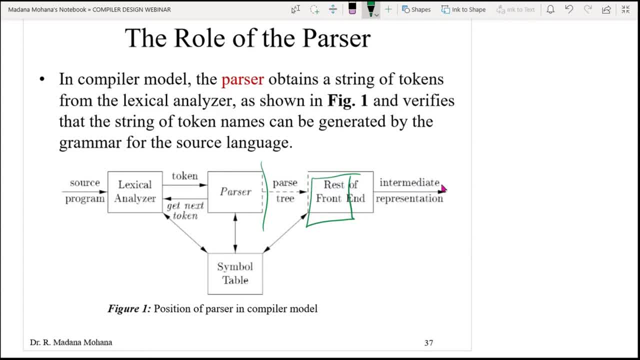 rest of front end. so till intermediate representation. ok now. so output of the parser or syntax analysis, which is parse tree, that is abstract syntax tree. ok now, that will be considered as the input to the next phase, semantic analysis. then semantic analysis provides some semantic checks or validations, so by using annotations then that can be converted into some intermediate. 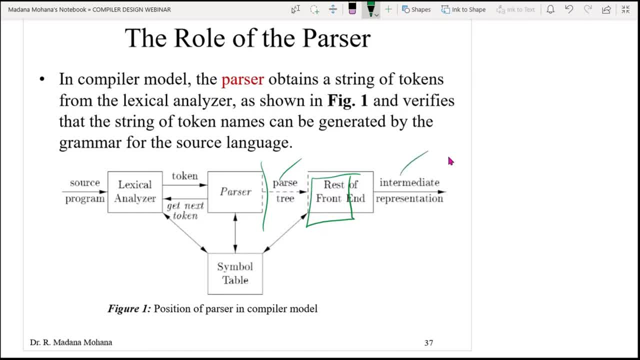 representation in the abstract syntax tree or tree address code form like that. further pages will be continually added. now the role of the parser or position of the parser in the compilation model. here you can see the input of the parser is token. output of the parser is parse tree or abstract syntax tree. ok, now here also symbol table is connected. 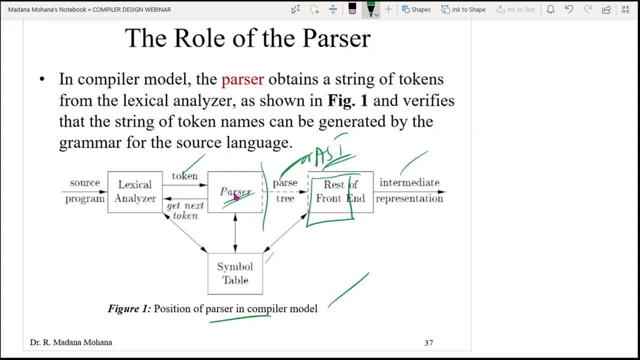 then what is the role of the parser which takes the tokens from the lexical analysis and converts the tokens into hierarchical form, which is tree form, which is called as parse tree? ok, like for every token that can be represented into in the hierarchical form, then the information about the tokens that can be stored in the symbol table, whichever, 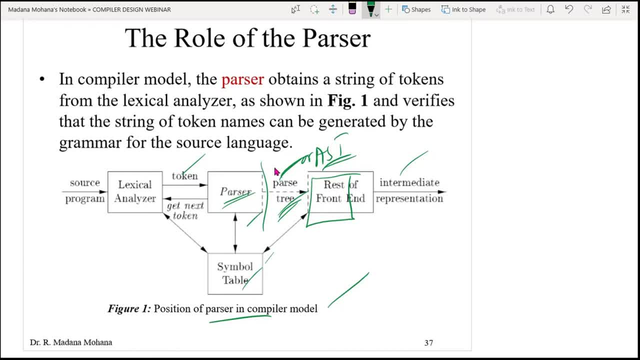 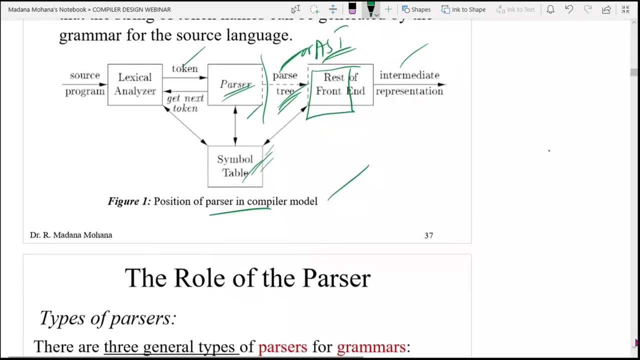 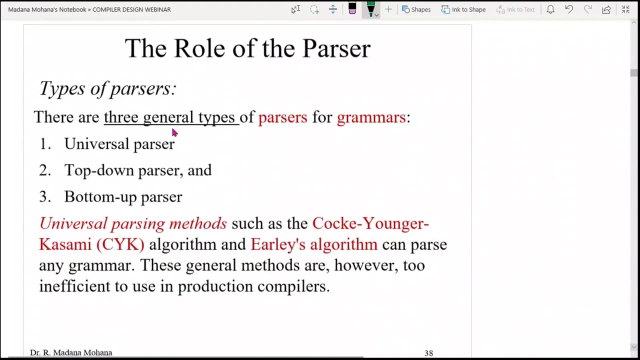 is required whenever we are constructing a parse tree. so you want actually, what are the variables, what are the constants, so that information that can be taken from the symbol table. ok, now, this is the role of parser in the compilation model or in the pages of compilation. ok, now, what are the types of parsers we are having? so, mainly we are having three general 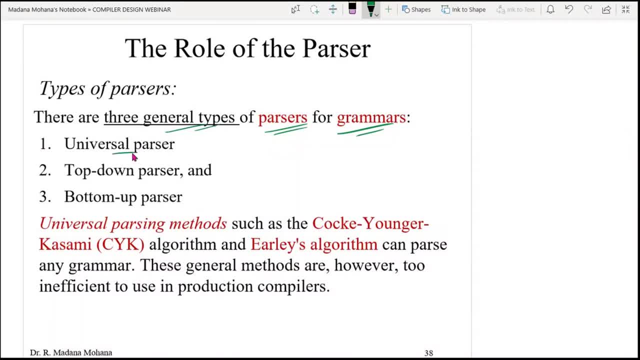 types of parsers, for a grammar. the first one is called the general type of parser and the first one is called as universal parser. the second one is called as top down parser. third one is called as bottom up parser. that universal parser, that is the basic one, that we won't. 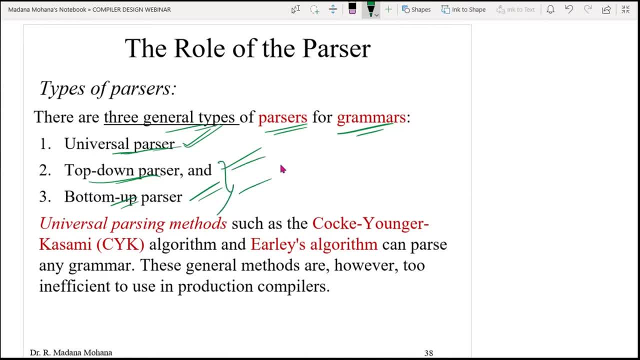 consider. so we will consider only these two: top down parser and bottom up parser. so what are the universal parsers? universal parsing methods such as like cyk algorithm. so that is cock anger, kasami in formal language and automata theory course. in our previous semester we studied we are having the membership algorithm of context free grammar, cfg membership algorithm. 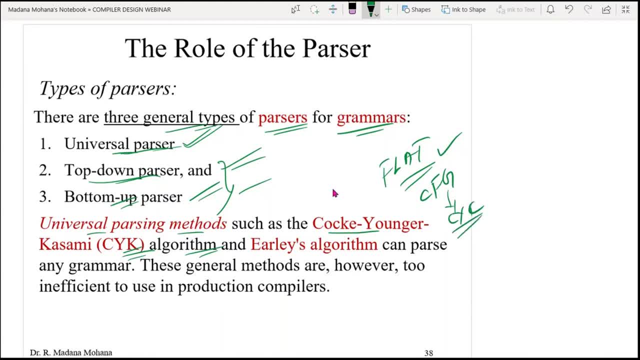 one that is pyk. so here this will be considered as a universal parser and some earliest algorithm which can parse any grammar. these general methods are, however, too inefficient to use in production of compiler. that is why we cannot use. here we will concentrate on the top down. 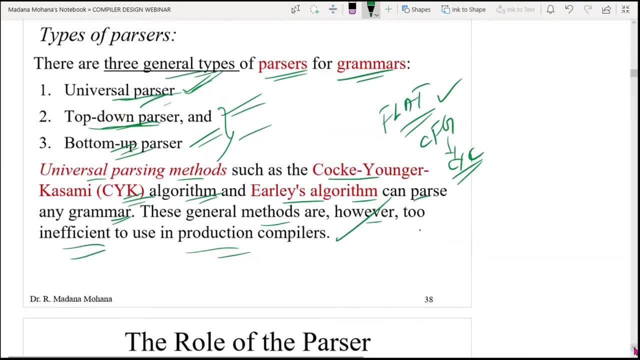 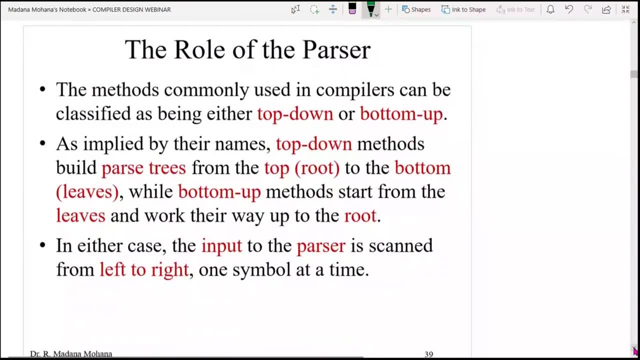 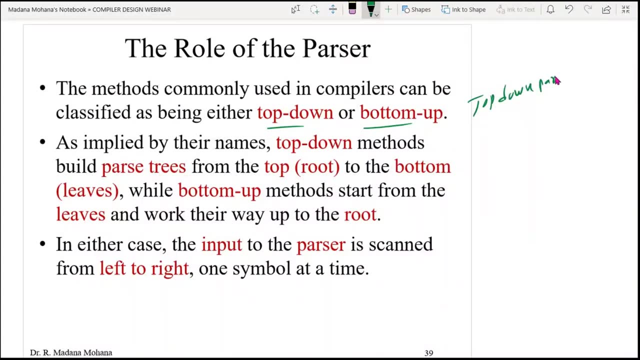 and bottom up parser. Now, what are the top down and bottom up parsers? the methods commonly used in compiler can be classified as being either top down parser or bottom up parser. so top down parser: construction of the parse tree starting from the root and proceeding towards its children. so this is 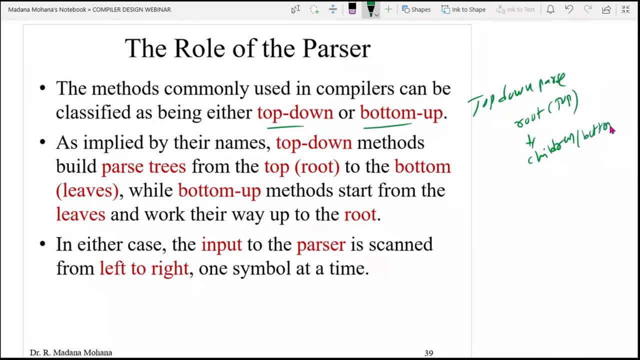 the top root, Then bottom what it contains children. this is called as top down parser, whereas bottom up parser reverse. bottom up parser will take children, means here will take the string, then will derive its root. here you can see this is bottom up parser. so in the derivation top. 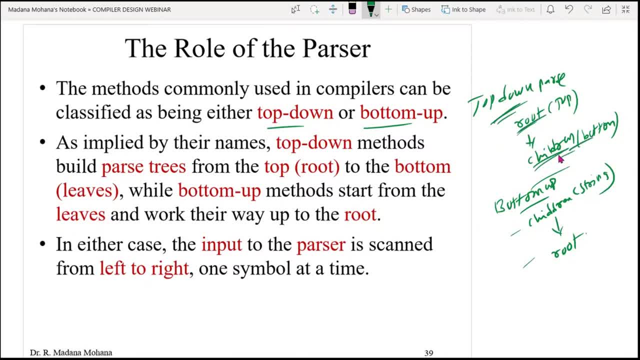 down parsing means will take root and derive its. children means string. Here you can derive string, whereas bottom up parsing means reverse substitution. we can take the string, then derive root. root means starting variable. the grammar is a simple representation of top down parsing and bottom up parsing. 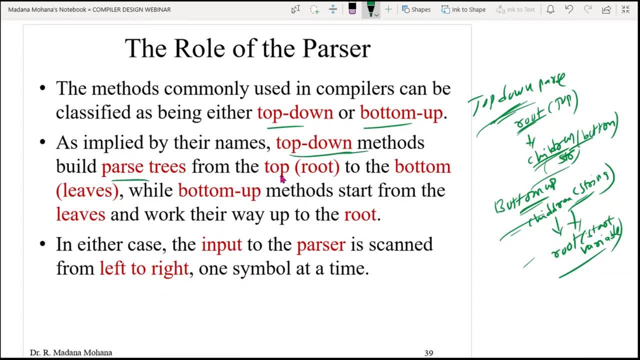 So, as employed by the names, top down method will parse tree from top root to bottom, that is, leaves, while bottom up parser starts from the leaves and work their way to derive its root. So in either case, the input to the parser is cannot from left to right, only one symbol. 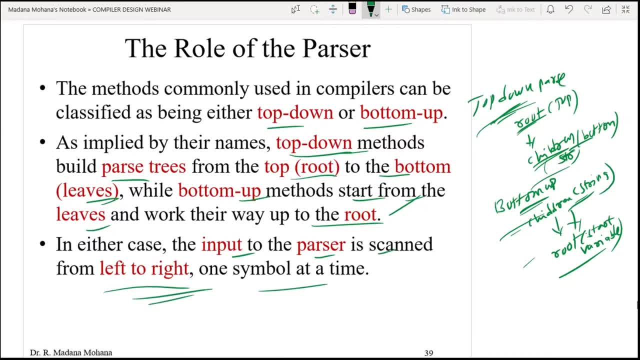 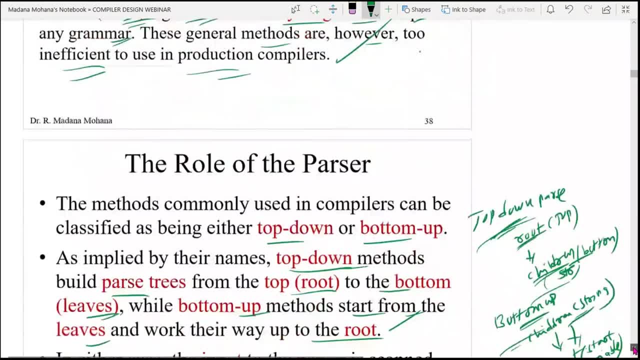 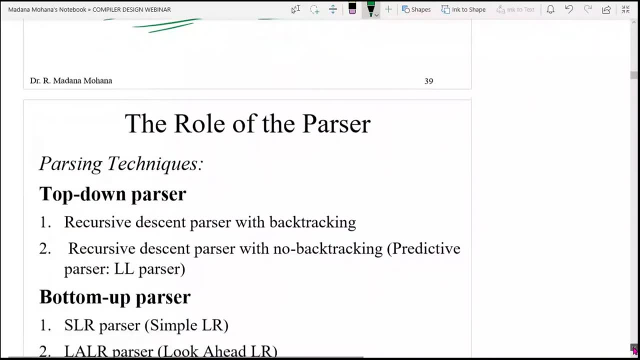 at a time. so these are all top down and bottom up parser. Now let us see what are the techniques of top down and bottom up parsers, parsing techniques. this is a very important topic in the entire of second unit. we are having total three plus two, five problems. 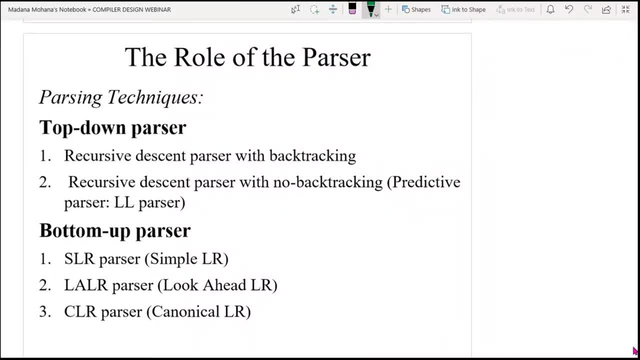 Definitely you will get two questions because you are having internal choice, unit wise. two questions will be given one question. you have to answer either first part or second part. like all units, you have to prepare. there is no choice: overall choice. you are having unit wise choice only. 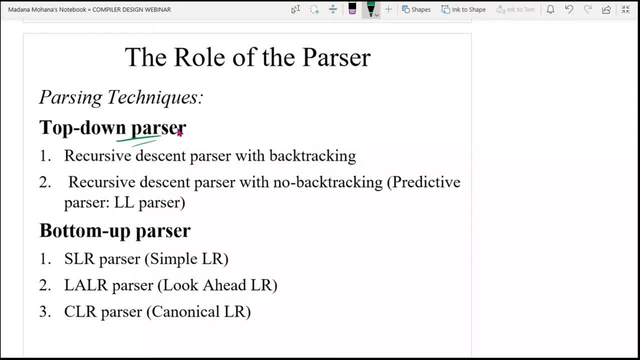 Now for top down parser. what are the various techniques we are having in top down parser? we are having recursive descent parser with the backtracking. this is very simple: you can define recursive procedures for each and every unit, Each and every grammar symbol. then recursive descent parser with no backtracking, then that. 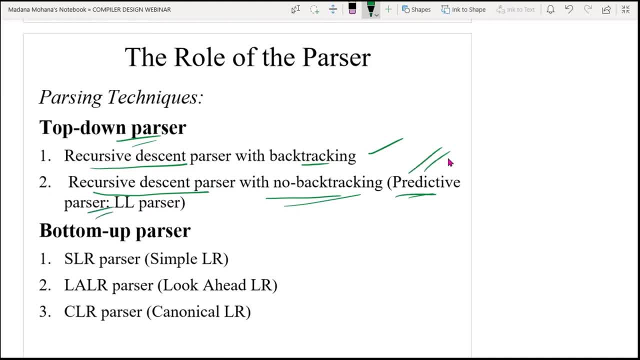 is called as predictive parser. this is very, very important predictive parser- definitely you will get this question In the predictive parser. we are having LL parser also. once you know the predictive parser, just for one rule you can define: is it LL parser or not? then, coming to bottom up, parser: 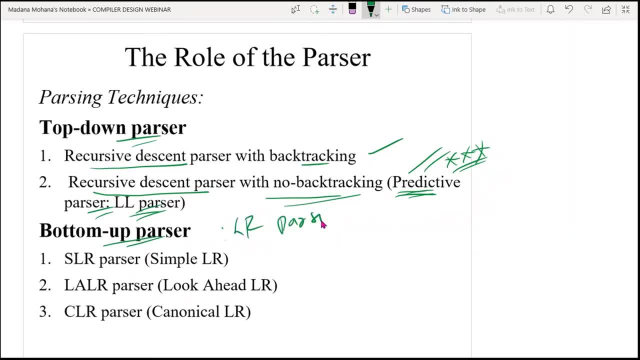 in bottom up parser We are having LR parsing. so in LR parsing we are having three techniques. one is simple: LR, it is called as SLR, then second one is called as CLR, canonical LR, CLR, then third one: look ahead: LR, LA, LR. so these two are powerful LR parsers, actually powerful LR parsers in 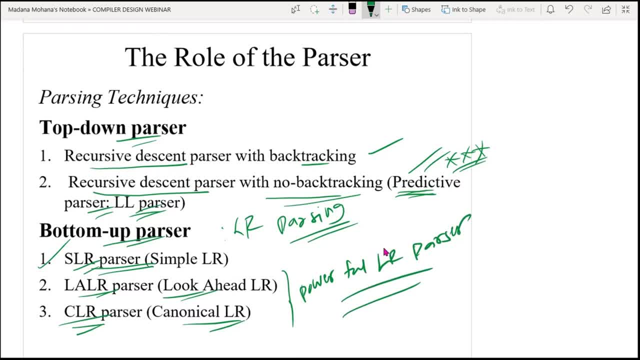 our syllabus, see they have mentioned powerful LR parsers means LA, LR, CLR. then simple LR means the basic one. ok, now for all these three LR parsers, the common things you needs to be followed, common factors for all LR parsers. model is same, then, parsing for all LR parsers. 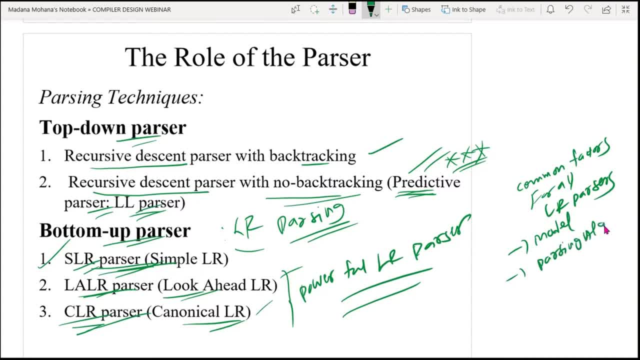 model is same, then parsing for all LR parsers model is same, then parsing for all LR parsers algorithm is same. these two are common. then where this are all deepen, parser to parser parsing table is different, only parsing table. parsing table is differ, but the model once suppose in examination we will get any question explained. SLR parsing model. explain. 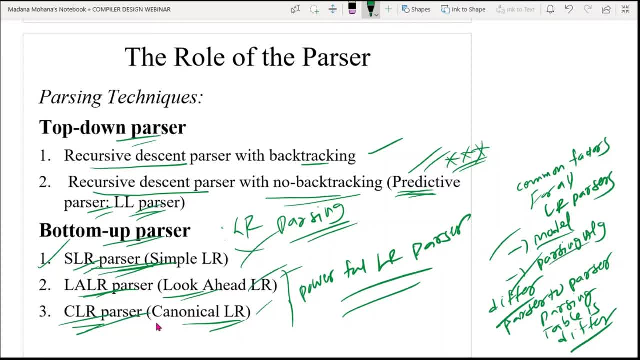 LA LR parsing model. so Essentially, explain a single esta right Ok. LALR parsing model. explain CLR parsing model and explain the parsing algorithm of SLR parsing algorithm, of LALR parsing algorithm, of CLR, the common LR parsing algorithm. only you can explain, but you can make the name as if it is SLR or CLR. LR, that is the only, but everything. 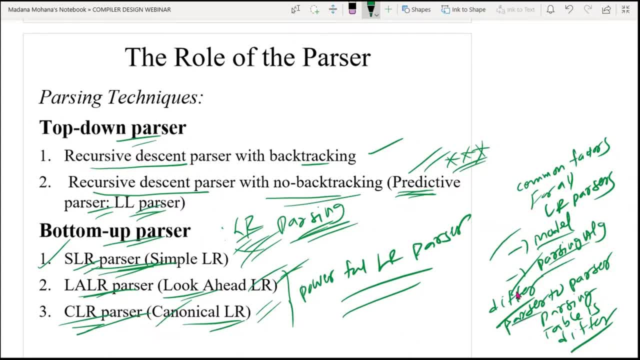 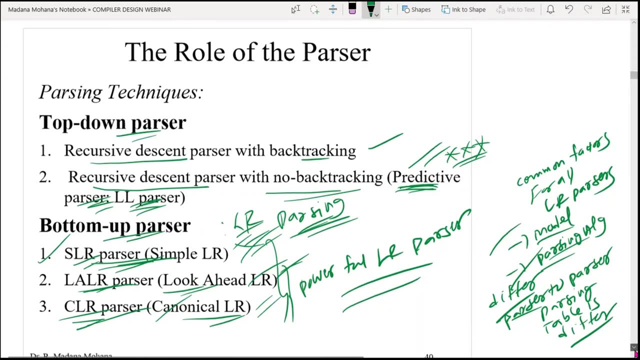 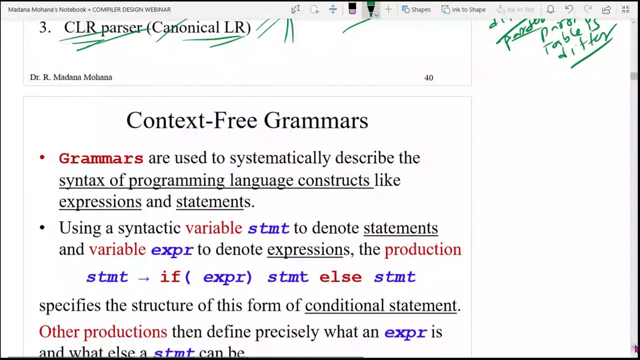 is same model, also same, only parsing table is differ from parser to parser. now, here we will focus on how to construct predictive parser, followed by LL parser, then the three parsers, three plus one. four problems we will discuss briefly one by one. ok, now, before that, here for the parser context, free grammar plays major role. just see the glance of context. 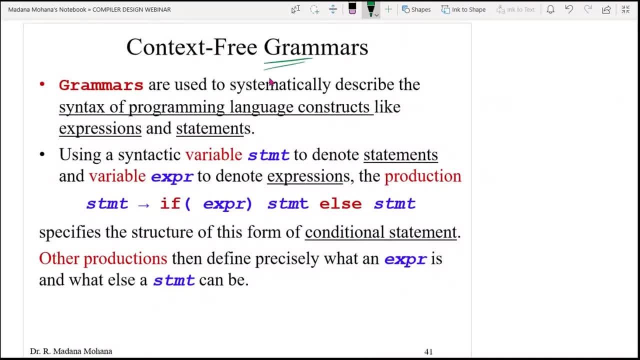 free grammar, even in formal language. automata theory also. you studied the CFG concept. that is for type. So what is CFG concept? For which type this grammar comes? we are having type 0, type 1, type 2, type 3. this is regular. 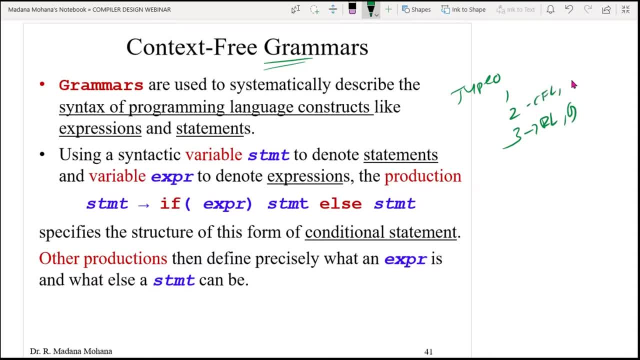 language: normal grammar. this is context free language. context free grammar. then type 1: context sensitive language. context sensitive grammar. then type 0. this is phrase structured or undistricted language, Undistricted grammar. the language is called as recursively enumerable. ok, now, where you studied context free grammar in type 2 C, this is a triple definition. VTSP V set of variables. 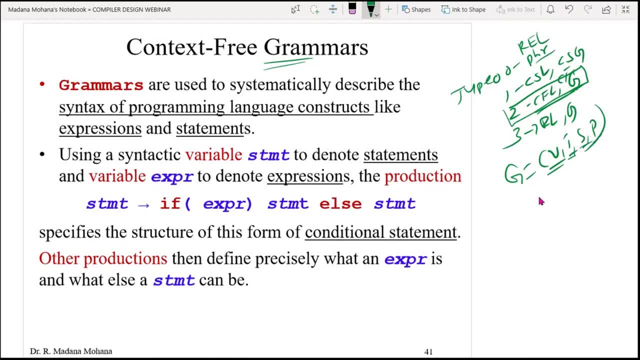 T terminal. a starting variable production. P set of production. the productions are of the form: alpha derives beta, whereas alpha belongs to V. single variable beta belongs to V. union T. String of variables are produced in the form: alpha derives beta, whereas alpha belongs to V. single variable beta belongs to V. union T. String of variables are produced in the. 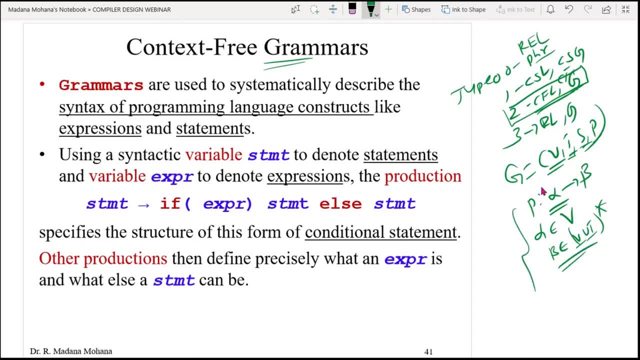 form alpha derives beta, whereas alpha belongs T, terminal, unless alpha belongs to V, equal ham certa coming from alpha zero. So there exist a two set of the two set of the terms is this: moto, Vova, V, setup called 2.. now if you have studied context free grammar, you can become better able to understand. 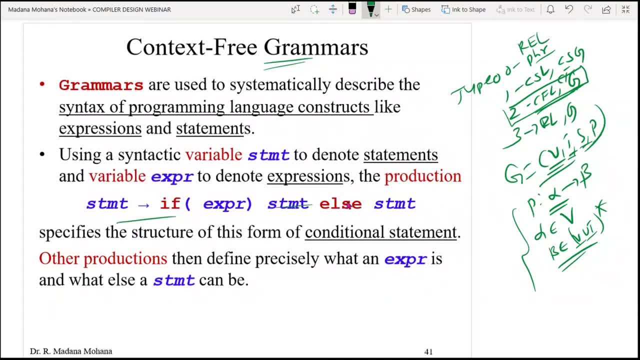 the generalε interpretation of context free grammar In why, for context free grammar, your defenders are sending commands. as probation, we are using statement equal to that is represented with arrow derives. if the condition can be represented within parentheses here, expression condition, then statement 1, STMP, else statement 2. so this is one grammar example of grammar. ok, now here. 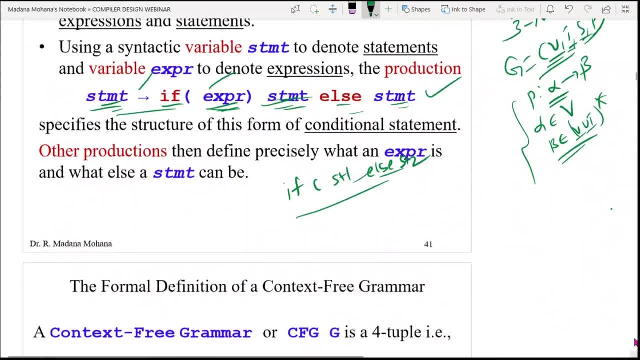 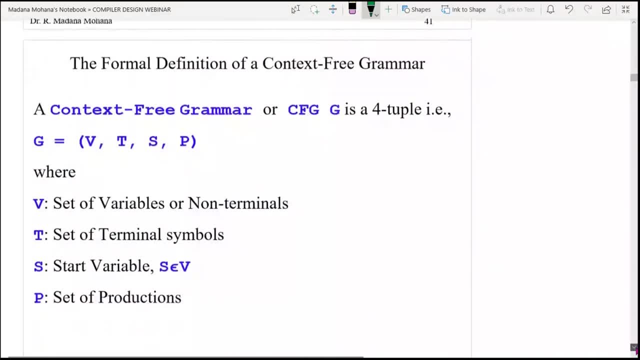 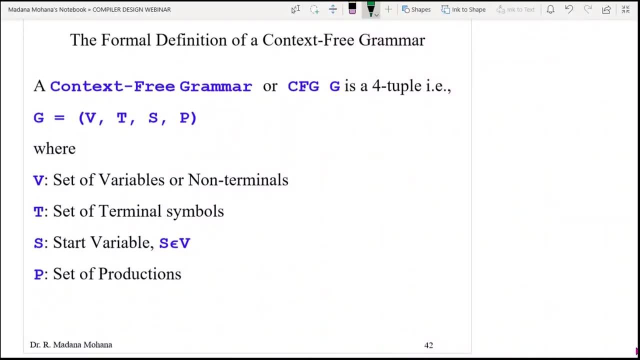 in our compiler design, even in semantic analysis also, we will use one standard grammar, that is arithmetic expression grammar. recently we have constructed the first e derives e plus e, e minus e e into e. that means standard grammar used. here is the definition what I explained here. just review once, because you 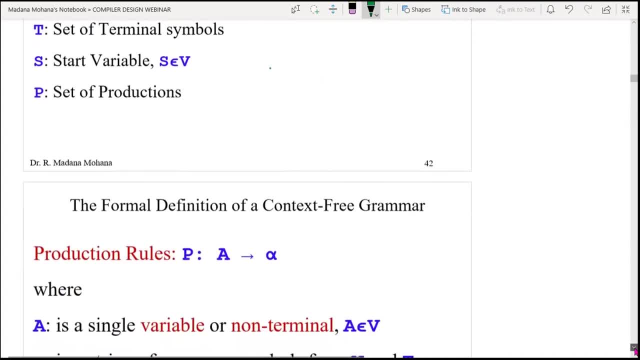 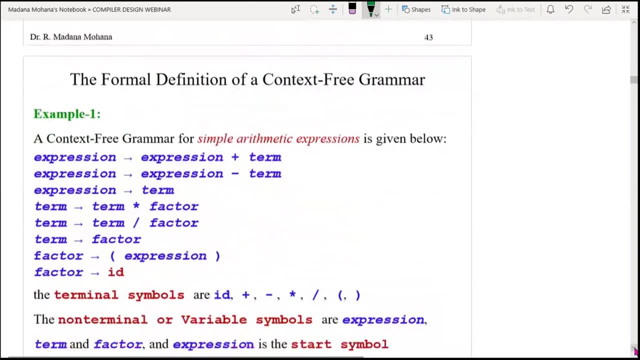 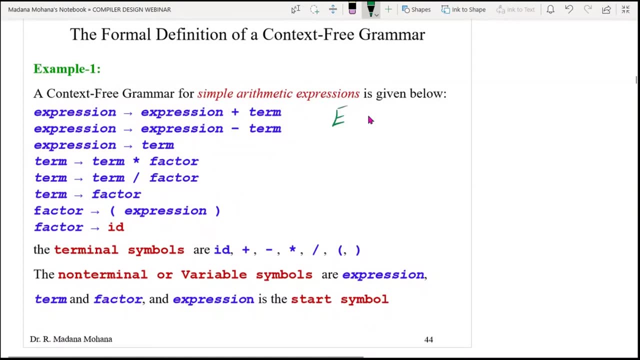 always studied in formal language, and automata theory again in syntax analysis. it is very important. so then, this is the arithmetic expression grammar. the same is given here, but for problems here, directly expression, we will use capital E. term we'll use capital T and factor, we use capital F. now, by converting these, 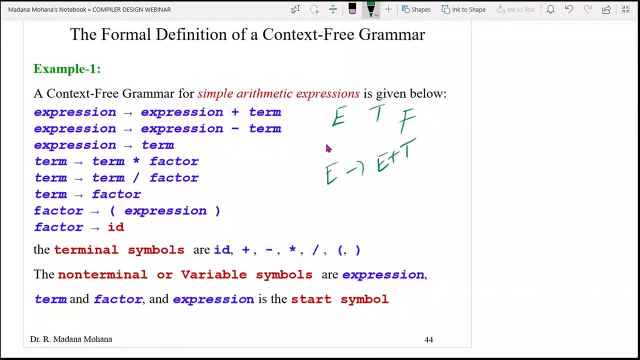 let us see what is this one: e derives E plus t, the first two production, then the second production: e derives e minus t, then third one: he derives t, then fourth one: t derives t into F, then next one: te derives T by F, then next one: te derives f and next one. 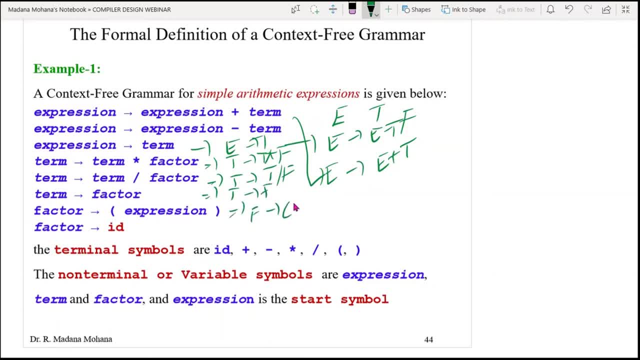 F. the next one, F, derives expression within parentheses. the next one, F, derives identifier. In this you can see in the grammar G equal to VTSP. just identify what are the variables here. here the variables are E, T, F, expression term factor. then the terminals are all the. 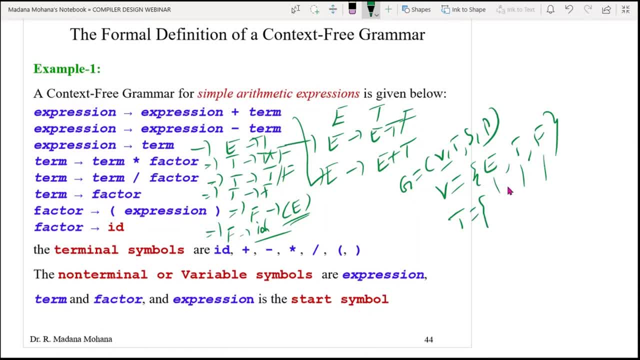 operators and bold face characters also. we are having plus, minus into divide, left parenthesis, right parenthesis ID. this ID is bold face character. so these are all terminals. then what is the starting variable in whatever the first production, left hand side, whatever? 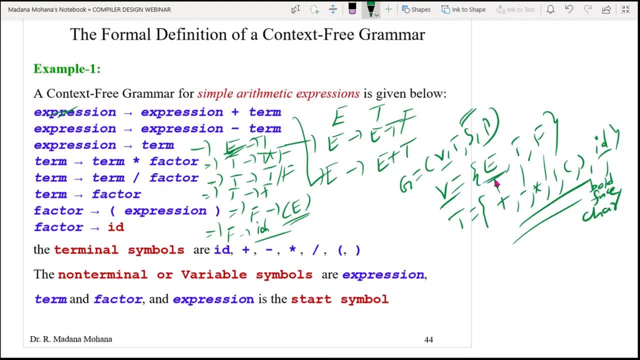 the variable, that is the starting variable. so E is the starting variable, S equal to E, right parenthesis. so then the productions are. these are all the productions. So, like in the given grammar, we have to know what are the identifiers, I mean what are the. 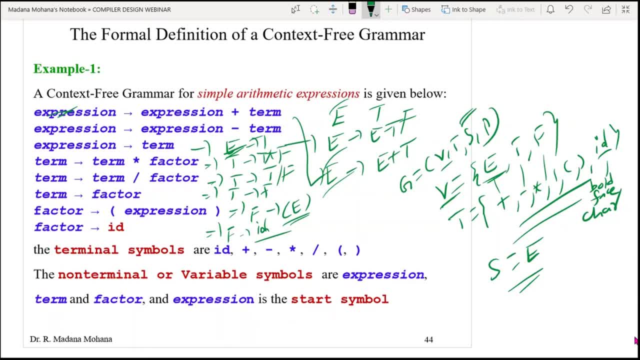 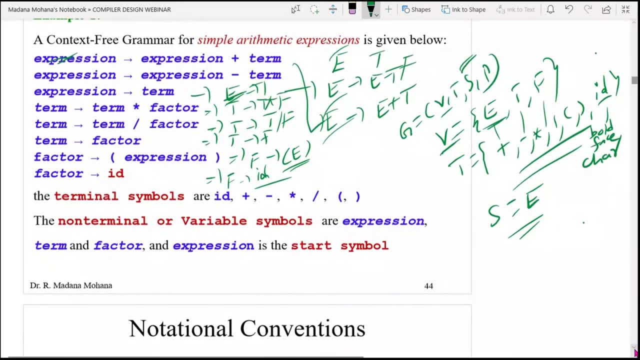 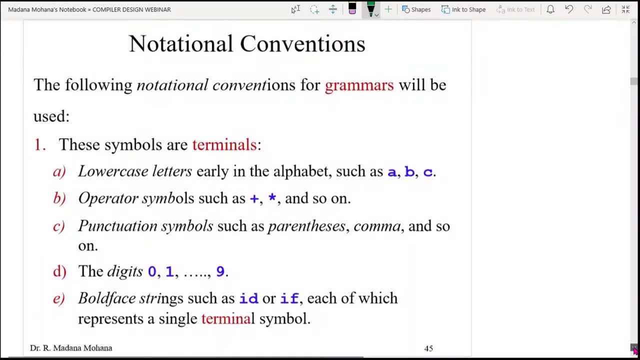 variables. what are the terminals then? what is the starting variable? you need to identify then the production. So any grammar, it contains only one starting variable, only only one starting variable. In the notations, all the terminals are denoted with lower case letters, then operator symbols: 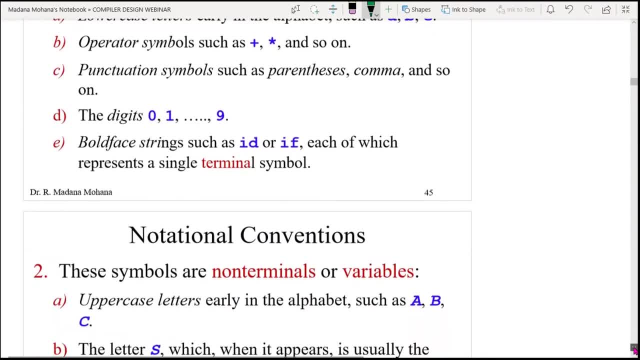 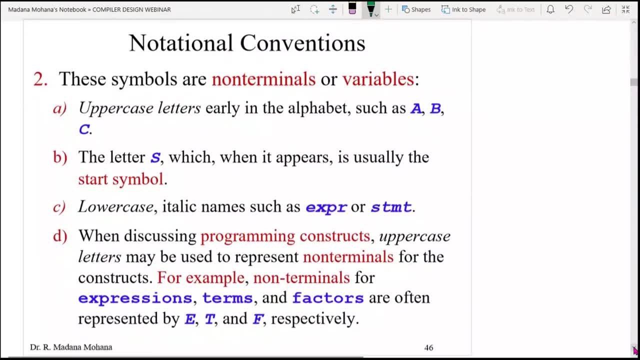 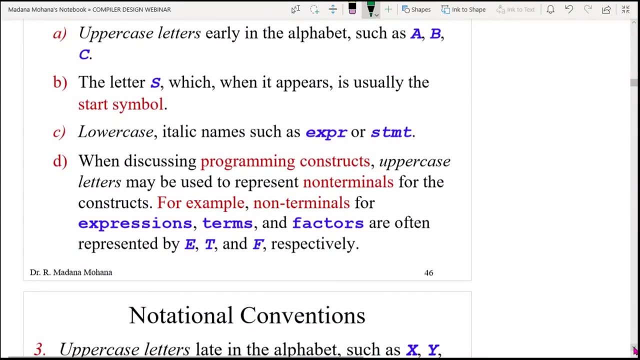 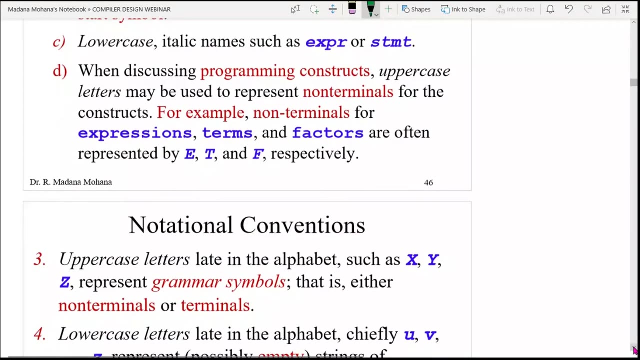 some punctuation, parenthesis, comma, etc. then digits 0 to 9, then bold face characters, ID, if, etc. then non terminals or variables are represented with upper case letters, capital A to capital Z, then using some italic names, lower case strings, like expression statement, then using some special greek letters, also alpha, beta, gamma, etc. these are all some notational. 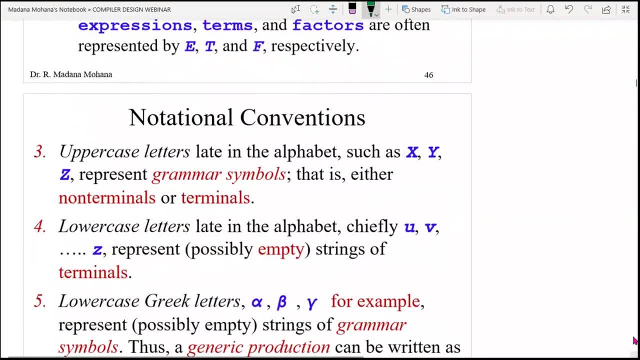 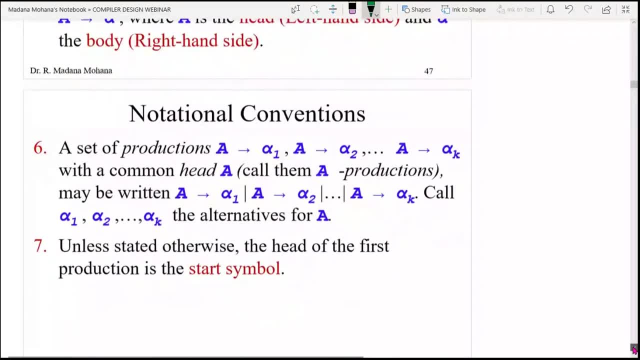 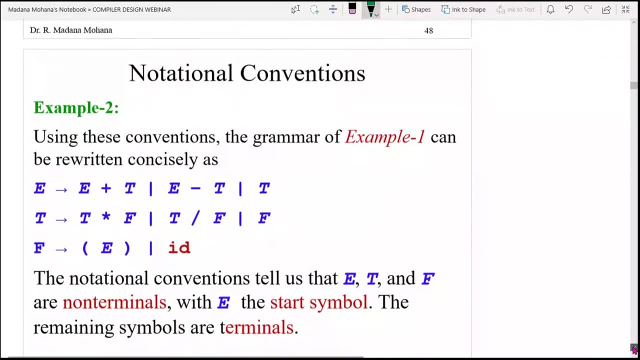 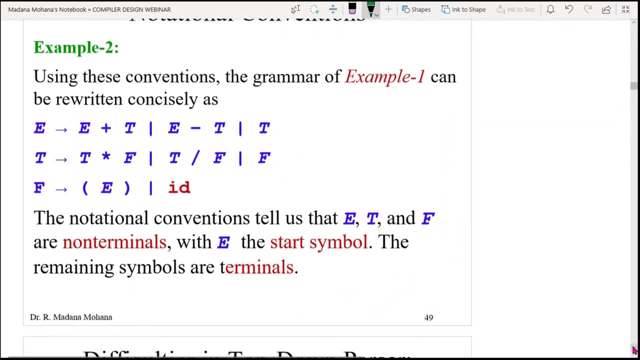 conventions used for variables and terminals. these are all the various notational or greek letters also used for the variables. then all the productions in the form of alpha derives: beta alpha. left hand side: it contains only single variable. right hand side: it contains variable followed by terminal, or only variable, or only terminal including null also. so this: 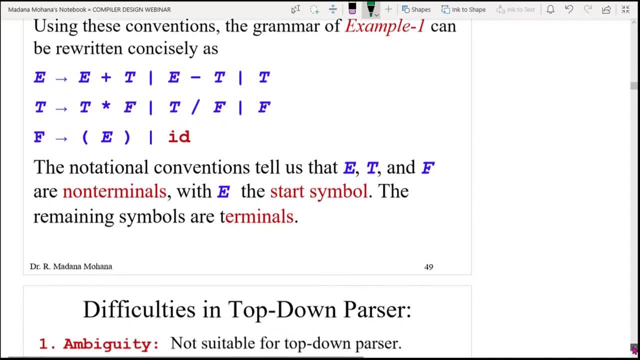 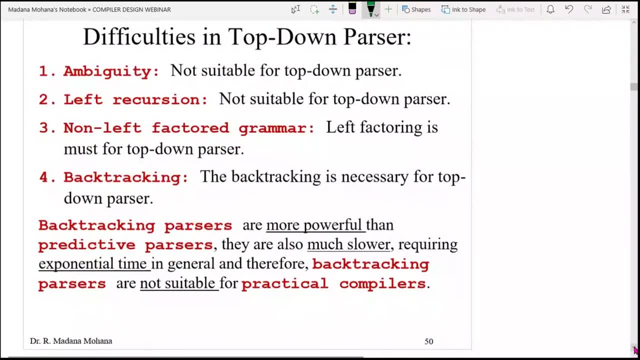 is the grammar, what I explained here in simplified form: automatic. So this is the grammar, what I explained here in simplified form: automatic. Ok now, whenever we are moving to top down parser first, there are some drawbacks or difficulties in top down parser. so we have to overcome all these difficulties whenever you are implementing. 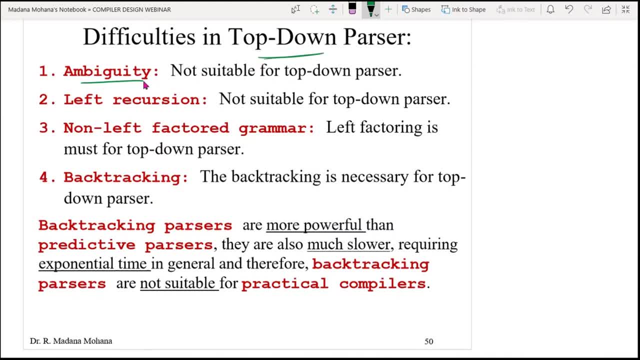 the top down parser. So the first difficulty in top down parser: ambiguity. so what is ambiguity in context with grammar? how can you define ambiguity for at least one string if there exist two left most derivations or two right most derivations or two derivation trees or parse trees? for 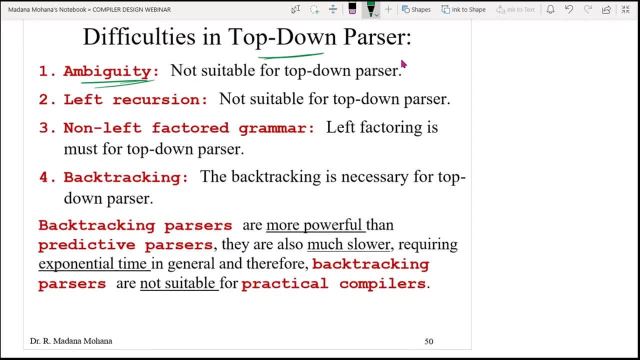 at least one string, then the grammar is said to be ambiguous grammar. So then, how to eliminate ambiguity? also, you are having, in the portion you already studied, so using this ambiguity rule, in case of if, then else grammar, then in case of automatic expression, grammar, So you are using precedence and associativity of operator, these two methods which are used 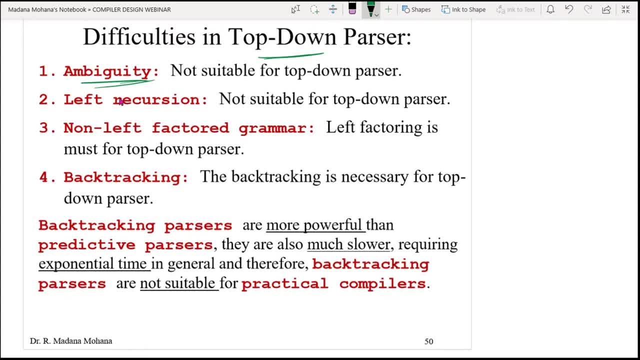 to eliminate ambiguity. that is one difficulty, then another one: left recursion. So if any grammar is left recursion which is not suitable for top down parser, you have to remove left recursion. this is one important concept: how to remove left recursion. one example problem: I will explain. 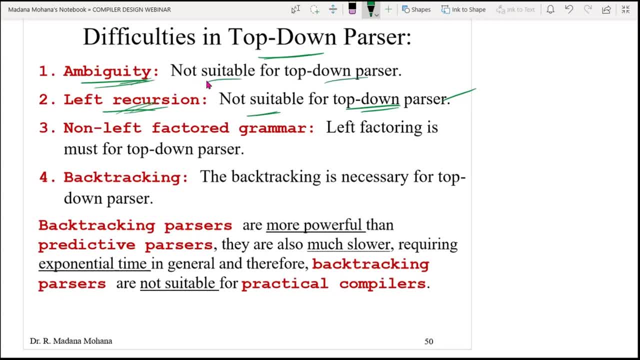 Then any grammar having ambiguity not suitable for top down parser: remove ambiguity. then non left factored grammar. so that means left factoring is must for top down parser. so how to remove the left factor? that means in the right hand side of the production. wherever the common values are, there prefixes starting right hand side left, most more than one production. 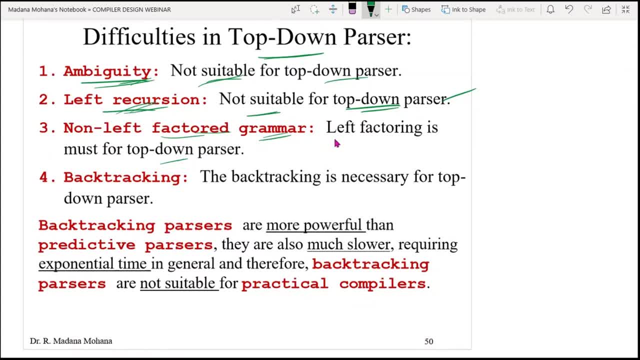 having common prefix, those can be taken as factoring out. so then that can be now non left factored grammar. So this is very important in top down parser. then backtracking. so backtracking is also necessary for top down parser. suppose in one production you substituted for deriving your string, so 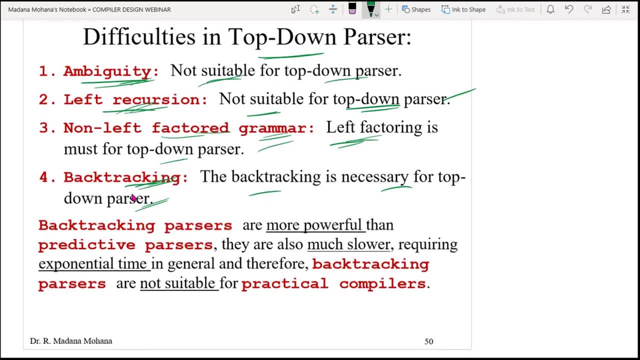 in that way your string is not derived. at that time you can go back and check: is there any alternative substitution for the same variable? so at that time you can go back and substitute alternative production. that going back is backtracking action. so without backtracking every time. 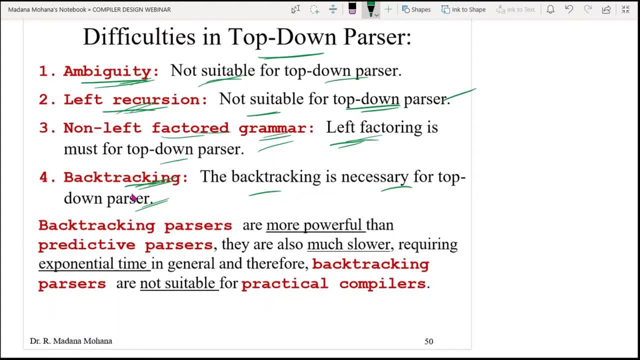 So you get our required strings. so backtracking parsers are more powerful than predictive parsers. they are also much slower, requires more time. therefore, backtracking parsers are not suitable for practical compilers. these are the difficulties in top down parser. now, whenever you, if you want to construct predictive parser, the grammar should satisfy all this. 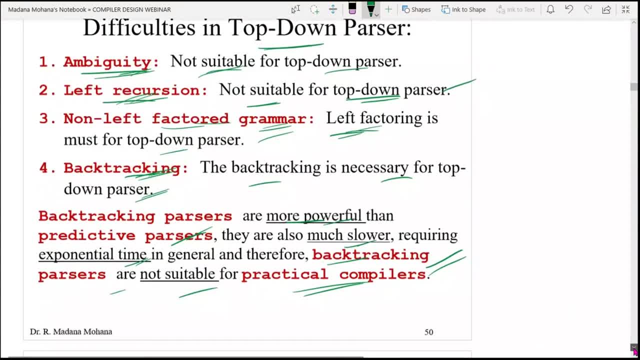 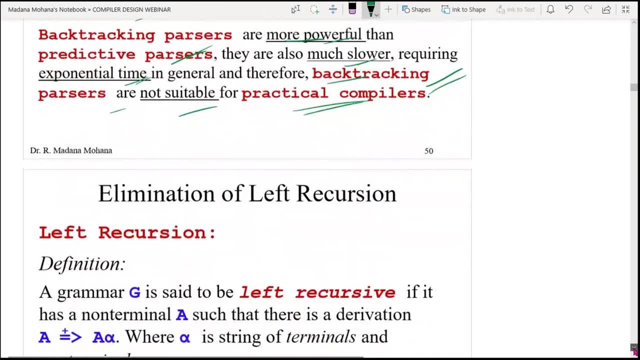 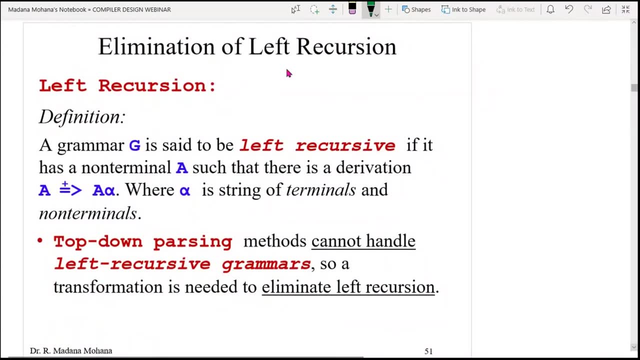 that means grammar does not contains ambiguity. So this is very important. Grammar does not have left recursion. Grammar should be left factored. so all should be satisfied. then only you can start constructing predictive parser. Now let us see the elimination of left recursion. sometimes in examination you will get one. 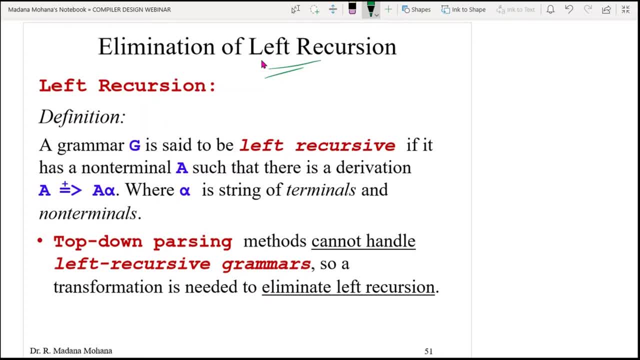 question for the given grammar. eliminate the left recursion, like this important concept. so a grammar G is said to be left recursive if it has a non terminal A such that there is a derivation. is of the form A, derives A alpha here why you use it less so compulsory. 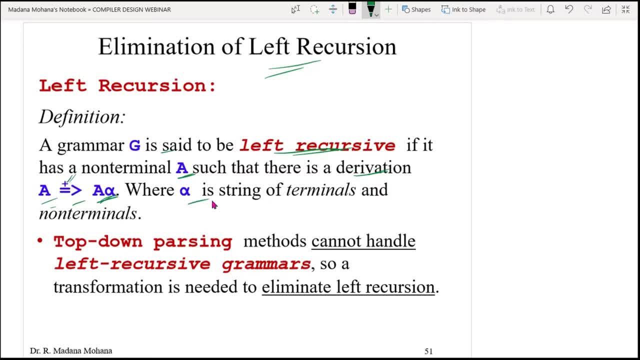 one or more productions are used to derive this one where alpha is string of terminals and non terminals. if you can draw its derivation tree for this, for example, your production is A derives A alpha. actually, if you can draw its derivation tree, this is the root right hand side- you can connect A alpha all the symbols in the right hand side, left to right. 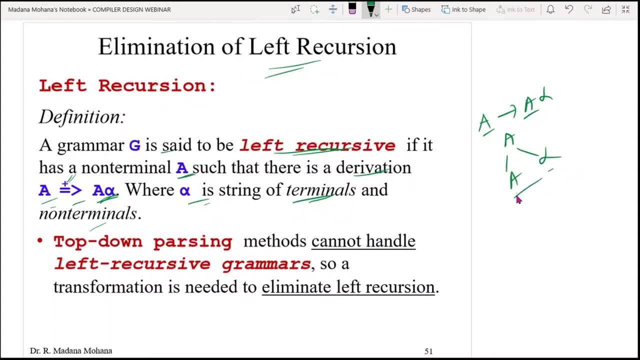 you can connect Again A. you are having substitution. what you are having again? A alpha, again A. you are having A alpha again you are having A alpha here. you can see this is the root left side. you can see the left. most the same variable is repeated. this is called actually immediate. 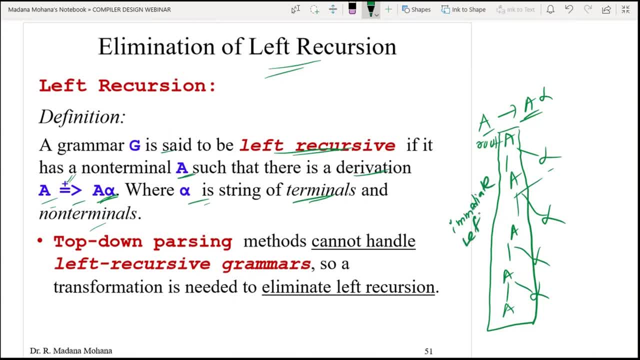 left recursion. this is called as immediate left recursion. The left hand side variable and the right hand side left most variable should be same. if any grammar is like this, then you can say it is in the form of left recursion. this is not allowed in the top down cursor. we have to remove this. so how to remove this? let us: 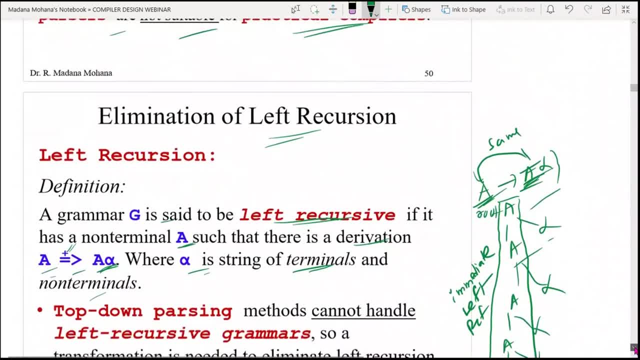 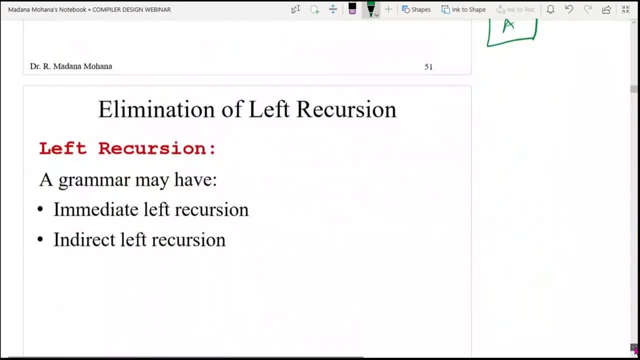 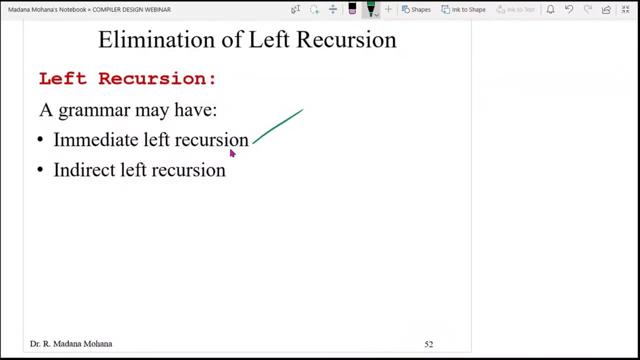 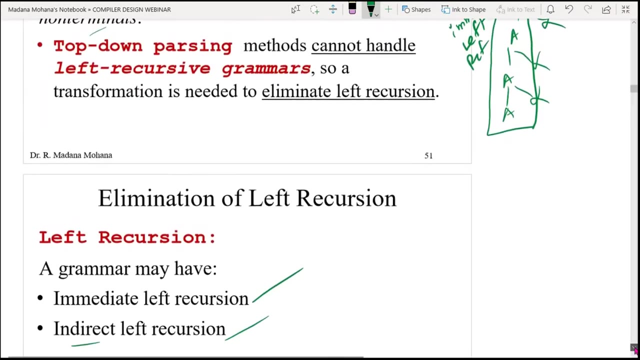 see you are having indirect left recursion. also, by substituting some productions at that time you may get left recursion. that is indirect left recursion. So the grammar is having immediate left recursion, the previous diagram, what we described then indirect left recursion during the process of derivation you may get this one that is: 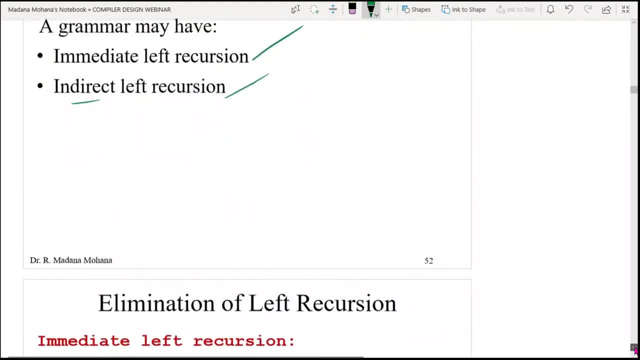 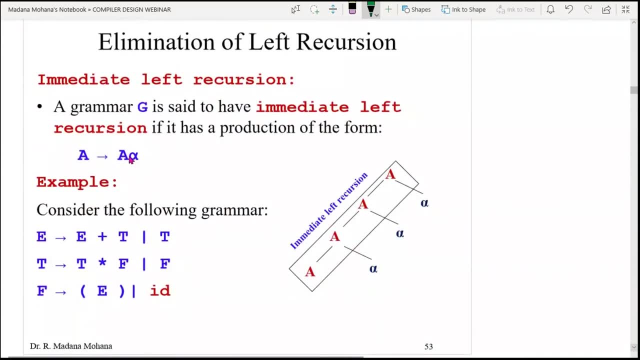 indirect left recursion. So, but our concentration is on only immediate left recursion. the given original grammar: immediately. when ever there is left recursion, you have to remove. see what I explained. A derives alpha, the diagrammatic representation. this is immediate left recursion, for example here: Here you can identify which are the productions having this left recursion here: E derives. 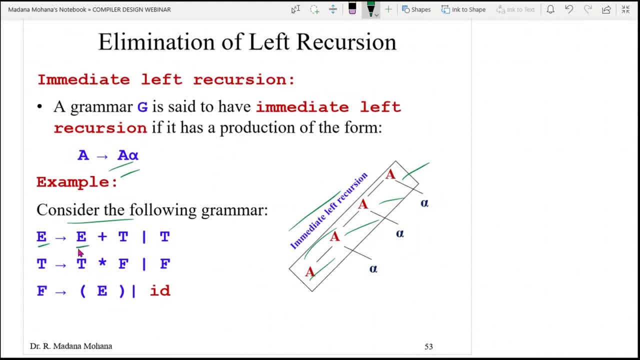 E plus T or T, at least any one in the right hand side having the prefix same as left hand side variable. these two are same, so it has left recursion and T derives T into F or F here T, T, so it is same, it has left recursion but F derives. it is starting with pedances. 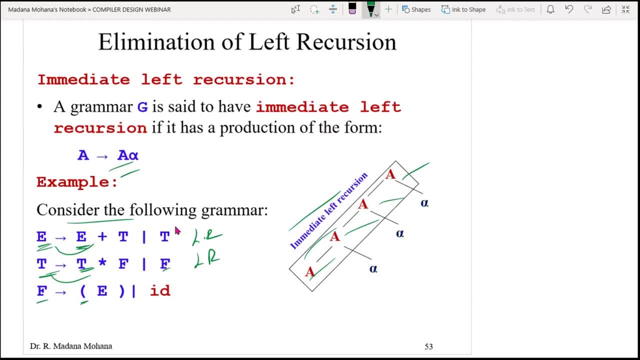 so, but indirect left recursion is there, but here our constant is null and immediate. so here no left recursion. production wise, we have to check in the given grammar. production wise, we have to check whichever the production having left recursion. so you have to eliminate. 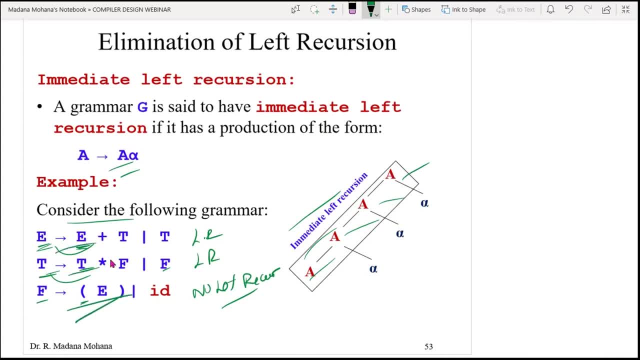 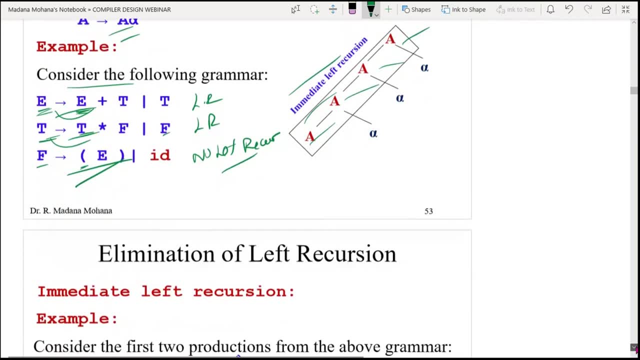 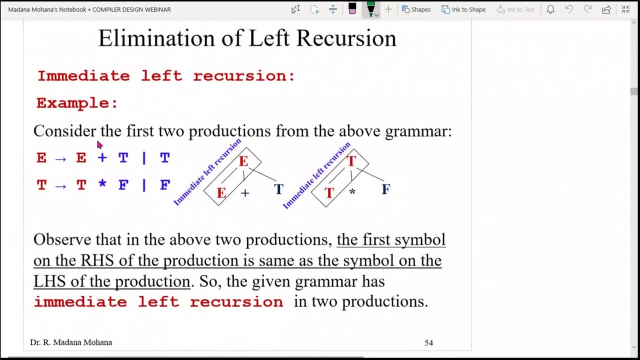 the left recursion, then how to eliminate left recursion for these two. so, as per the procedure, we are having some rules for elimination of left recursion. so let us see the rules here. See the above example diagrammatically represented. here you can see E derives E plus T E E. 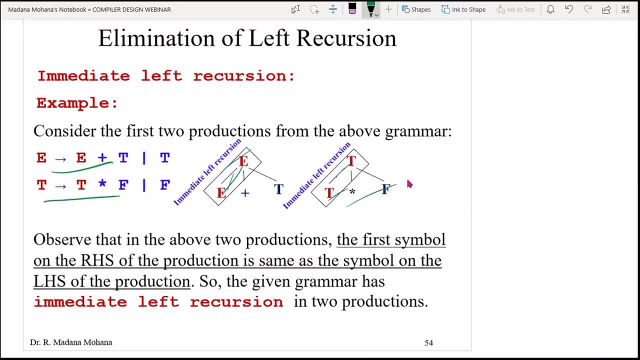 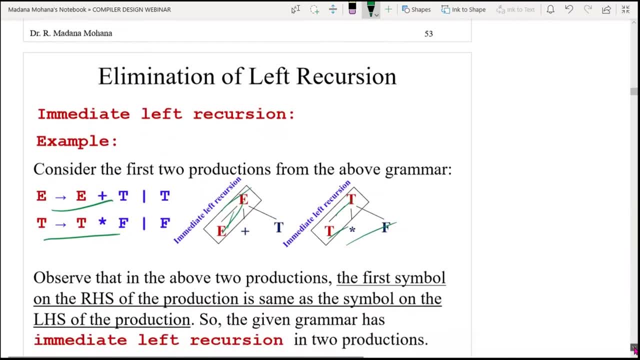 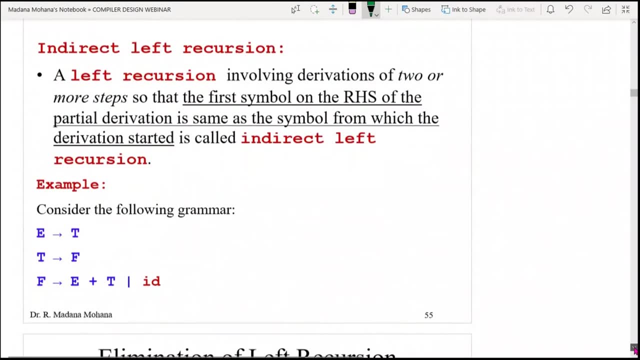 immediate left recursion is there. T derives T into F, T, T. so immediate left recursion is there Now. F derives E. within parenthesis, we are not having immediate left recursion, that is indirect left recursion. Okay now what are the rules for elimination of left recursion? we will see. 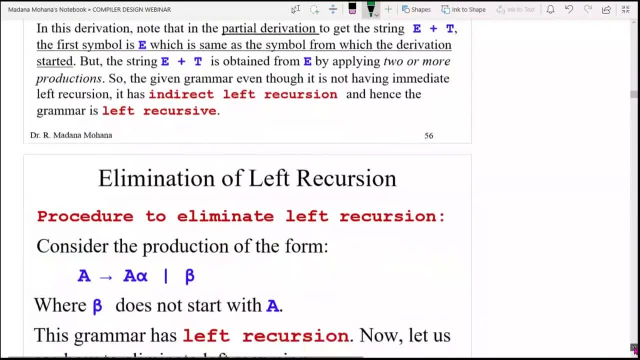 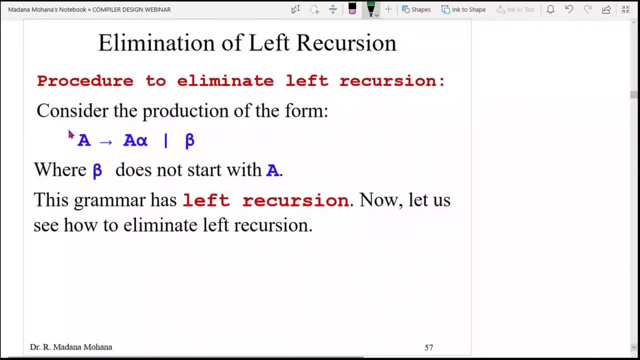 Only immediate left recursion. we will eliminate here. now you can see if any grammar is in the form. this is the general form of left recursion. grammar A derives A alpha or beta. here capital A is a variable, alpha and beta are string of variables or terminals, whatever. 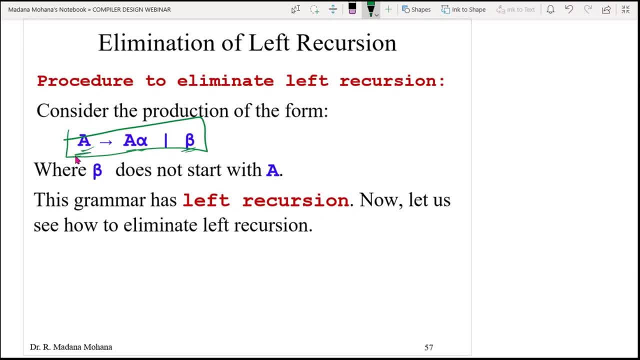 but only our intention is left hand side starting variable. Right hand side left most anyone matching with left hand side, then it has left recursion. then whatever the alpha beta values, do not bother about it. but here beta does not start with the variable A, because already here A alpha is there. if you are having one more, 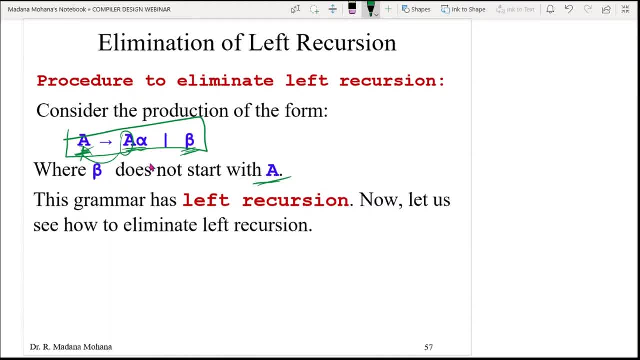 variable starting with A that comes under this one only: A alpha 1 or A alpha 2 and so on. like this: for n productions, Beta does not start with A. This grammar has left recursion. Now how to eliminate the left recursion for this? 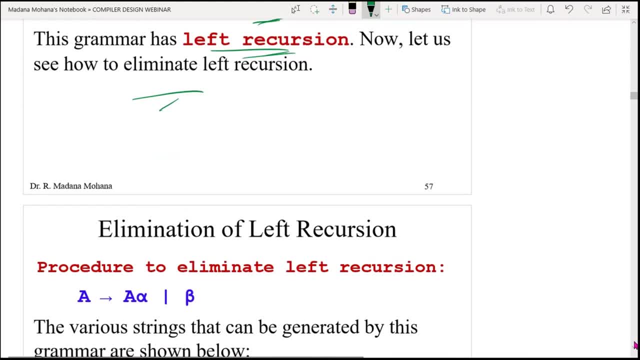 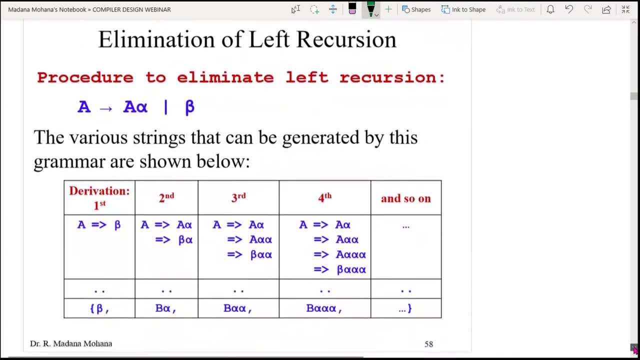 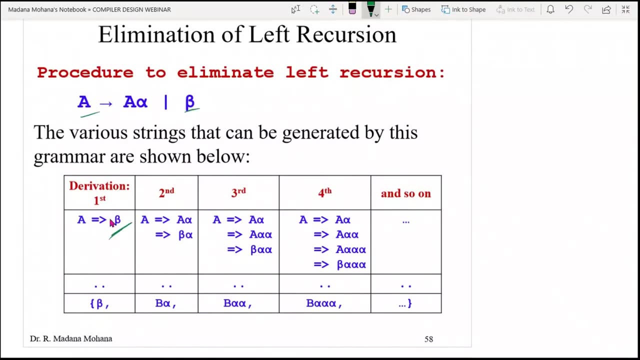 So again you can see the general for n productions. are there how the left recursion grammar will be Before that? first let us see whenever you can apply the derivation First. we have taken A derives beta, so here only the string beta, only derived further. 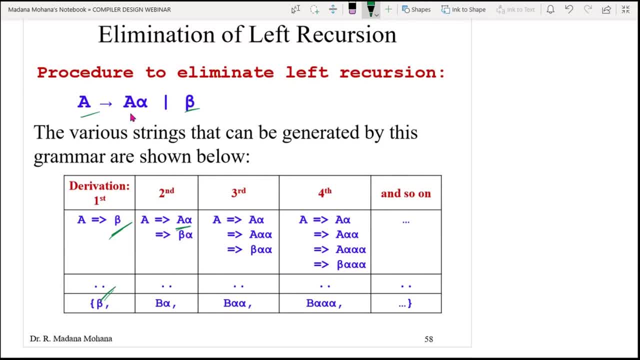 what beta, we do not know. then if you can take A alpha first production A, we are having, substitution, A we are having. what are the possibilities? you may substitute again A alpha or beta. suppose, if you can substitute beta, alpha here you will get this thing: beta. 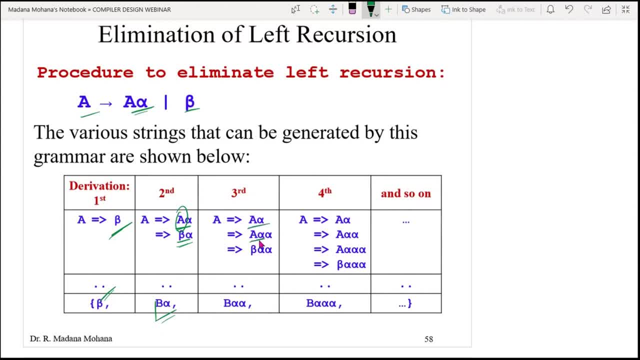 alpha. Next time A alpha A is substituted, again A alpha, next A is substituted: beta, beta, alpha, alpha, this thing next time, for example, repeated A alpha n times plus beta, alpha, beta is substituted, and so on. So these are all the things you will get here for this left recursive grammar. 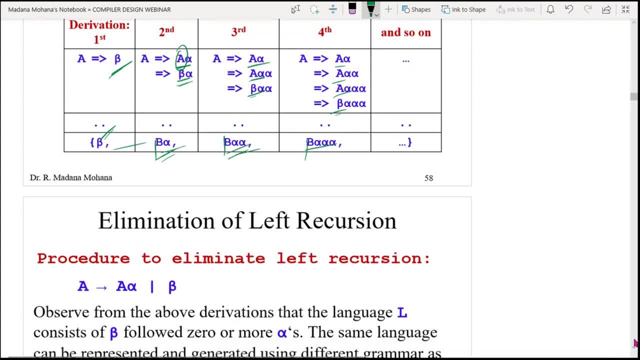 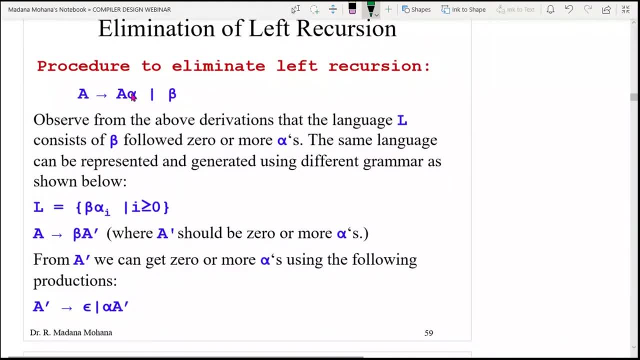 Like this: if you are having n productions which are in the form of left recursive form, that also we will see First for these two. what are the rules for elimination of left recursion? So the language is like this every time it is: start with beta. 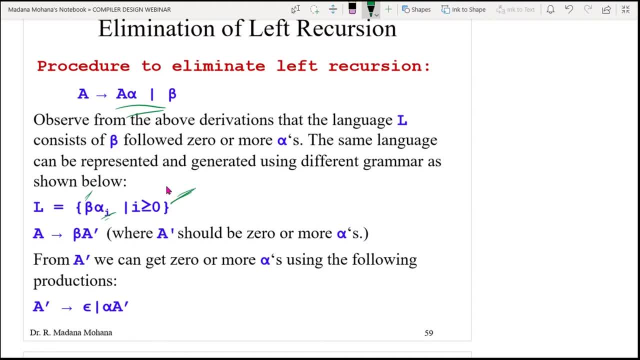 Followed by alpha i greater than or equal to 0.. So now you can write the productions like this: A derives beta A dash. A dash should be 0 or more alphas here. Here this alpha is substituted with A dash. 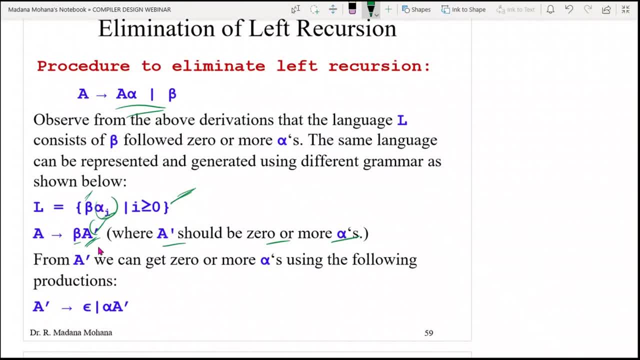 Ok, now what is A dash? what A dash contains? It may contains null or alpha, followed by A dash may be repeated. Now you can see A derives, A alpha. The equivalent productions are like this. So these productions, after eliminating left recursion, the first rule is A derives beta. 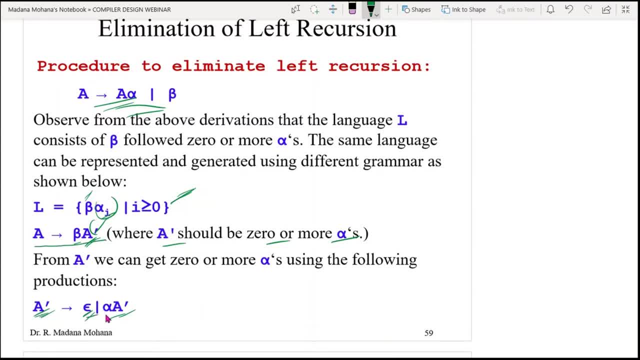 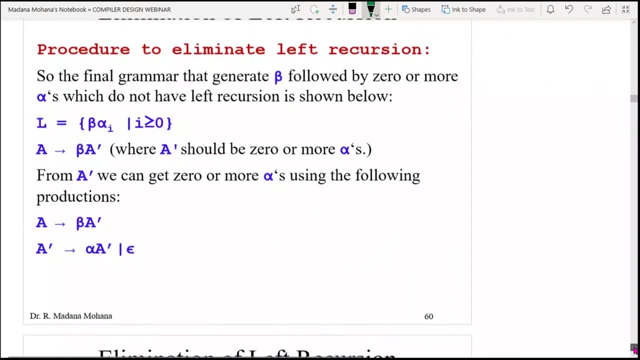 A dash, Then what is A dash? derives alpha, epsilon or alpha A dash? these are all the two rules actually, So any grammar is in this form. you can apply these two rules for elimination of left recursion. Ok now, A derives beta A dash, then A dash. derives alpha A dash, then A dash derives. 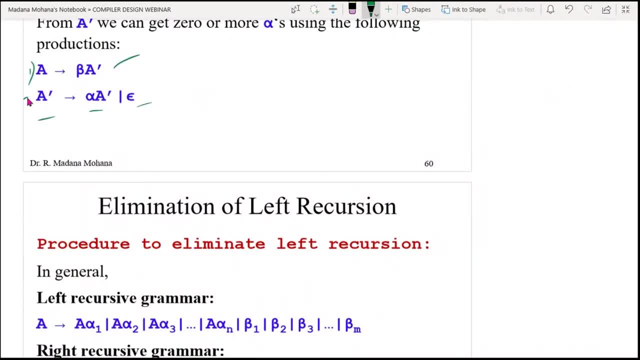 alpha, A dash. Ok, So these two rules are null. These two rules you can remember. If any production is in the form of A derives, A alpha or beta, non-left recursive grammar rules: A derives start with beta. then new variable, A dash, is introduced. 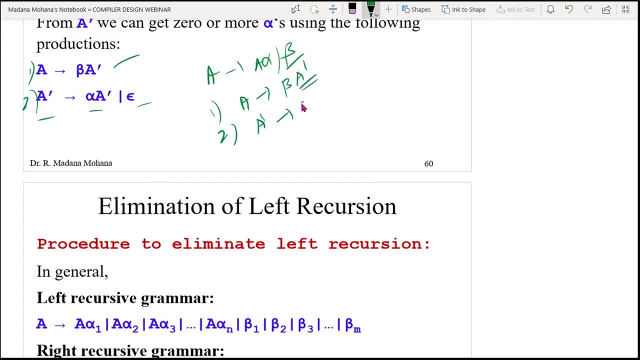 Now what is A dash? It is null or alpha A dash, These two rules. Now you can see here: A derives beta A dash, There is no left recursion. A dash is null, then A dash derives alpha- No left recursion. 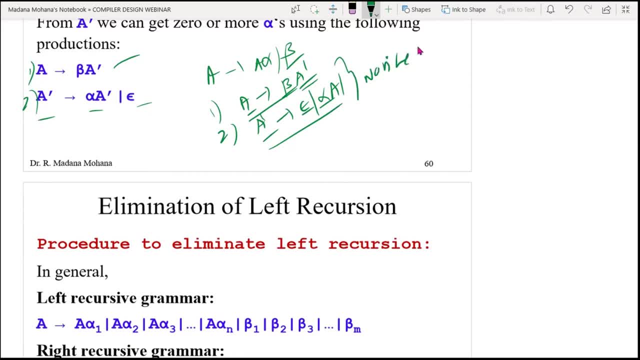 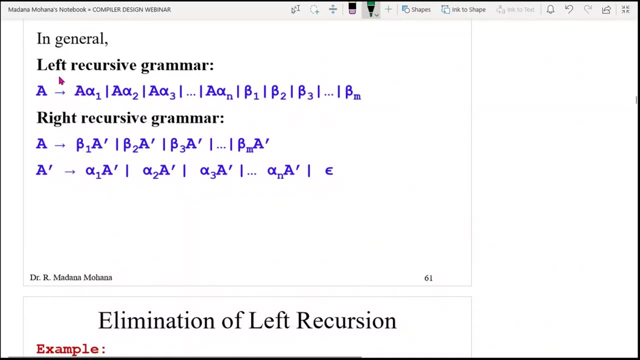 This is A dash. Ok, Non-left recursive grammar- You may consider it as formula, for any grammar- is in this form: These two rules you can apply. Then that grammar is converted into non-left recursive format Like this: if you are having n productions, this is C. if you are having n productions, 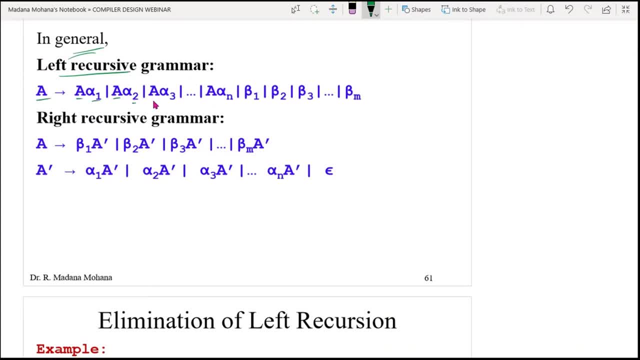 in general, A derives A alpha 1, A alpha 2 or A alpha 3, and so on. A alpha n. Here A is common. The prefix is repeated every time, Then followed by alpha 1,, alpha 2, whatever you want. 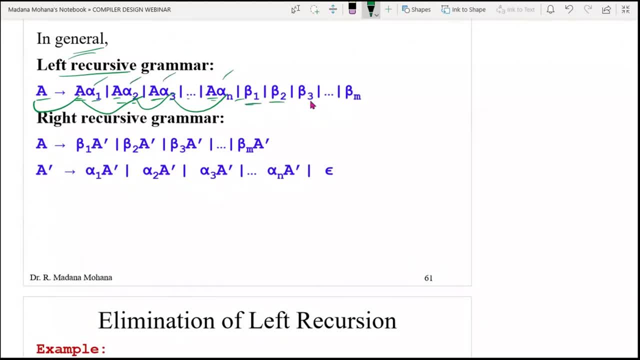 Or next beta 1 or beta 2 and so on, beta n. Here you can see, beta does not start with A. So in this, the general form, what we use here, A derives A alpha or beta. The first rule: A derives beta, A dash. 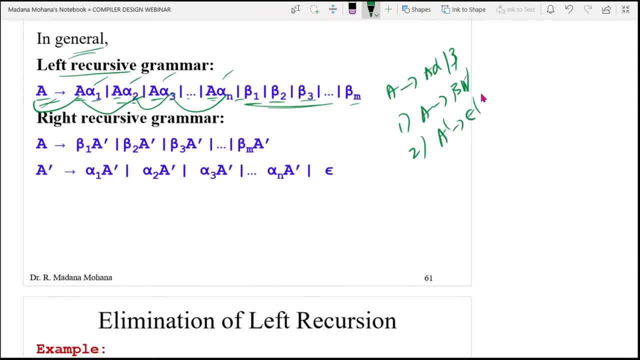 The second rule A dash derives epsilon alpha A dash. Substitute these values. As for rule 1, A derives beta A dash. It means beta 1 A dash or beta 2 A dash, or beta 3 A dash or beta n. Why? 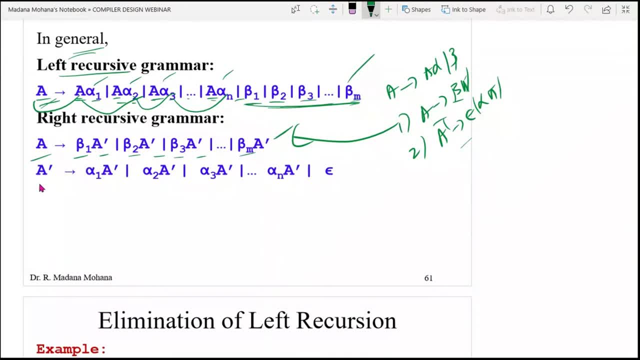 Because beta is repeated every time. Similarly. next rule: A dash derives null or alpha A dash. We are having alpha repeated n times: Alpha 1 A dash, or alpha 2 A dash, And so on: alpha n A dash. This you can make it as formal substitute. 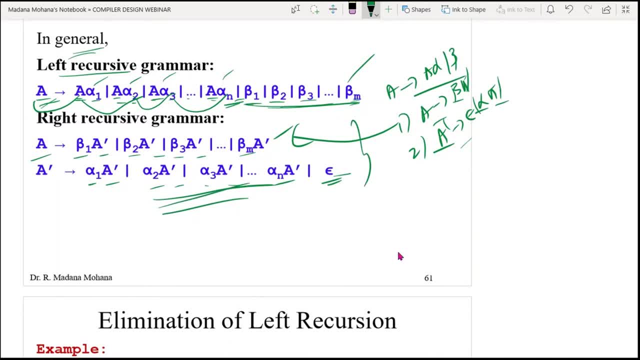 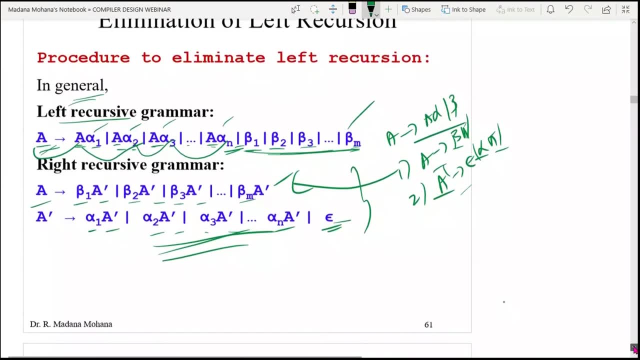 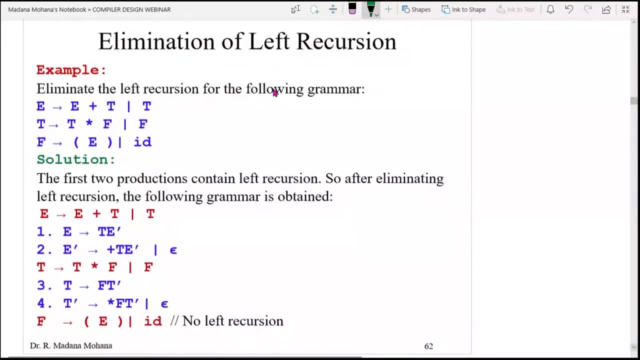 Any position with any number of. Here you can see It also- having a dash derives alpha, a dash are null. so using rule one you can substitute this one. so what? you will get this one. so here a means e derives, beta means t. now a dash means here e dash. 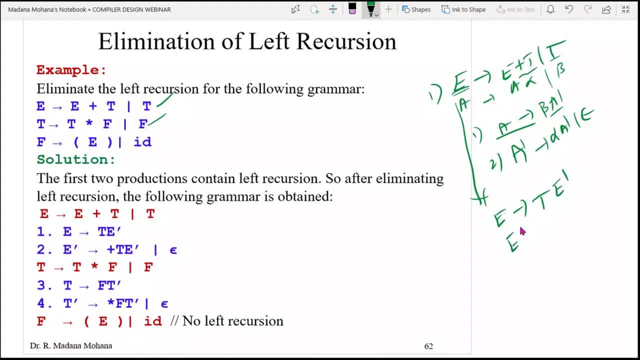 now next one: a dash equal to means t dash. using rule two, e dash derives alpha, alpha means plus t. so then plus t dash, here you can see e derives t dash, e dash. there is plus t dash, or lambda. which law then? similarly, t derives t into f. here you can see same t. 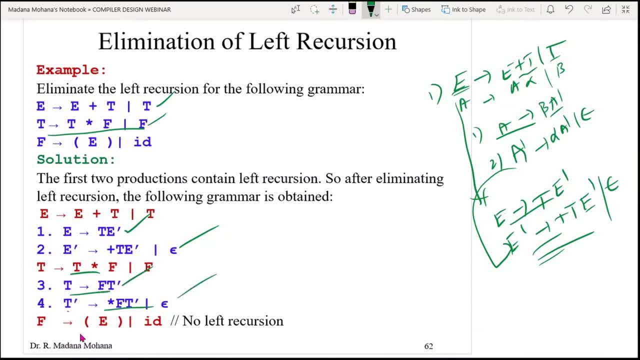 derives f, t dash, then t dash. there is star. f, t, dash are null, but f derives e, within parenthesis id: no left recursion. Now this is the grammar after removing left recursion: production: one, two, three, four, then five total the five productions. so like this, any given grammar, you can remove the left. 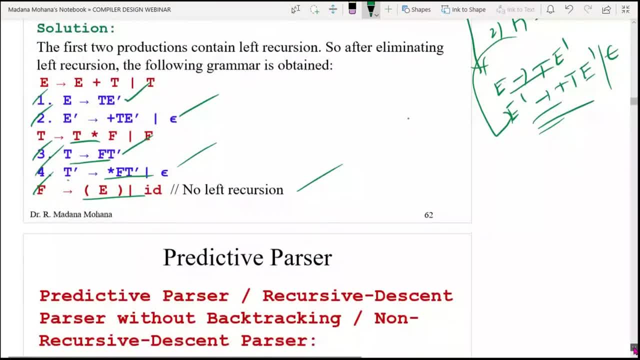 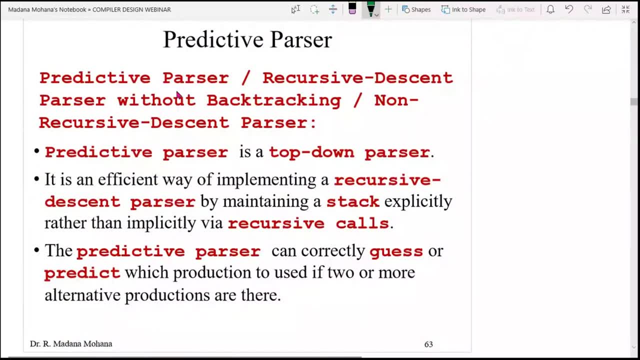 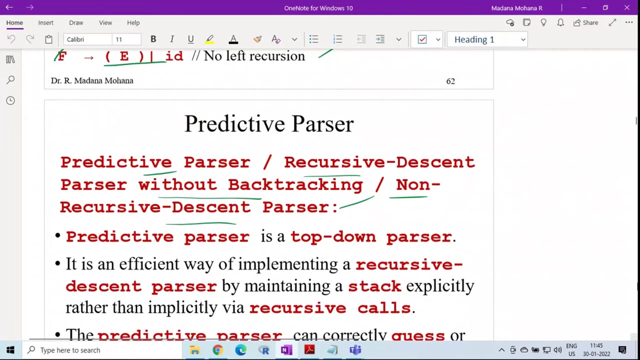 recursion. so that is the example problem. so then, coming to our predictive parser, why we discussed left recursion means for predictive parser is the prerequisite. Predictive parser is also called as recursive descent parser without backtracking or non recursive descent parser. now we will see predictive parser. so for predictive parser, what are? 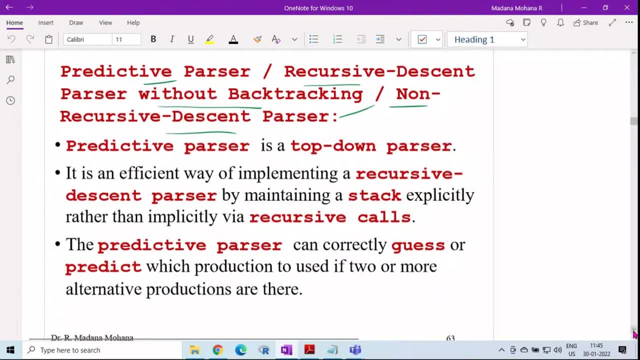 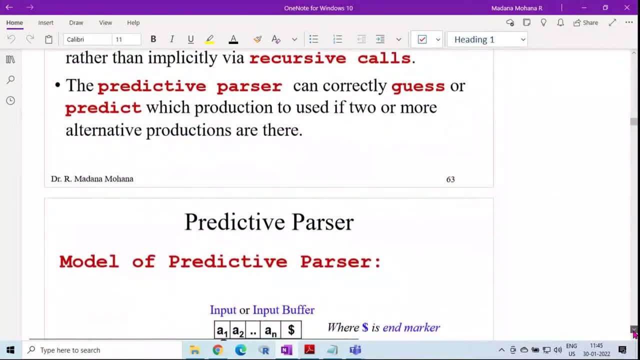 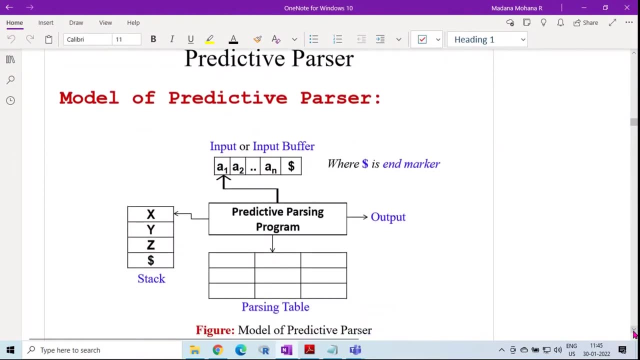 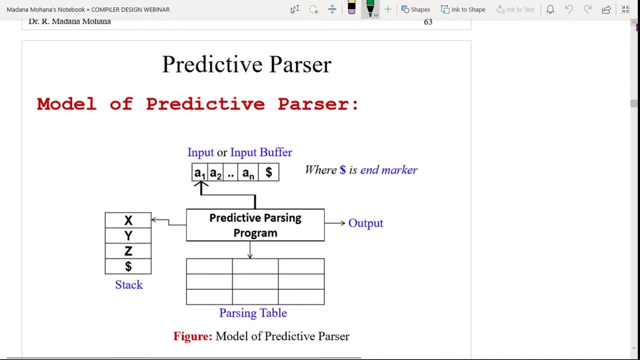 the difficulties in top down parser. any grammar that does not allows all that means. we have to remove ambiguity, we have to remove left recursion, Then non left factoring, etcetera. all needs to be addressed so you can see the model of the predictive parser. so sometimes theoretically you will get question. explain the predictive. 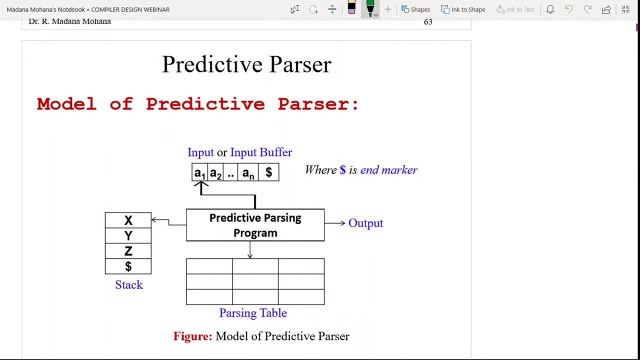 parser with block diagram or working of predictive parser, etcetera. this is the diagram, so model of predictive parser, mainly it consisting of the components. predictive parsing program is the main component. What it contains? It contains Output component, parsing table component. then it contains input or input buffer. then 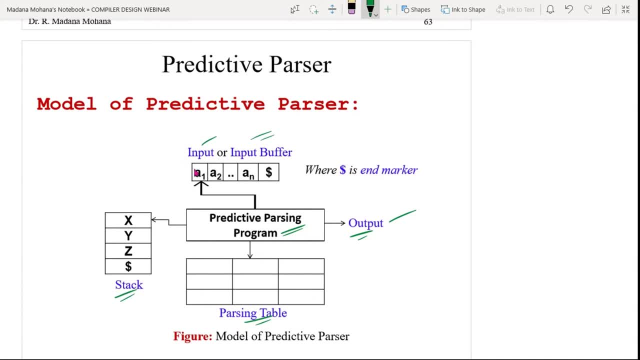 it contains stack also. so what input or input buffer contains? the input or the source program is stored, or the string is stored in input buffer ended with an end marker. so dollar- we will call it as dollar- is the end marker. now the string is stored in the tape. what is? 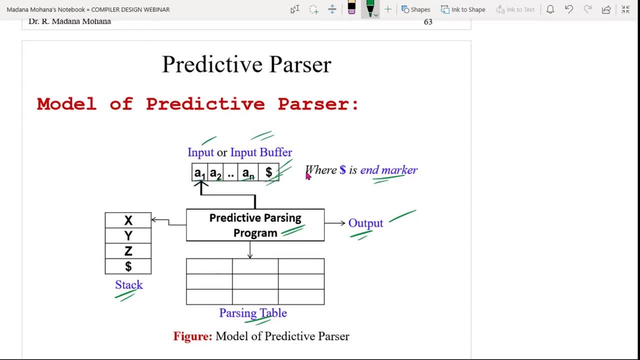 stored in the tape. one symbol in one cell only: stack A1, A2 and so on, A, L. then what stack contains? initially it contains the end marker. there is the empty of the stack. empty symbol of the stack. then some grammar symbols: x, y, z. always the predictive parser sees the top. 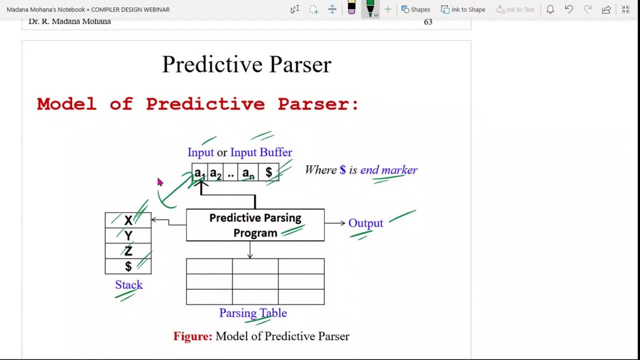 of the stack and the current input symbol. these two, based on this, actions are defined actions. so top of the stack and current input symbol. Then it produces output accordingly. what is the output here? parsing then successfully, successfully or not? the output is parsing successful, parsing not successful. so how this? 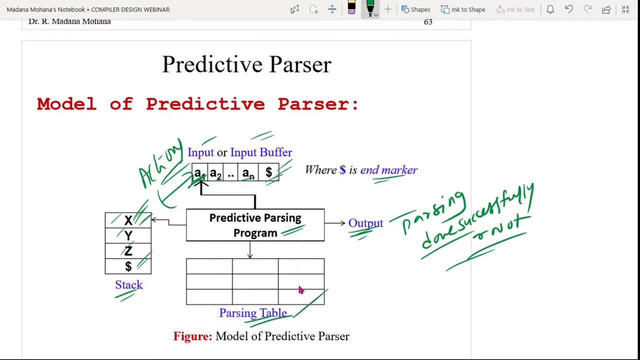 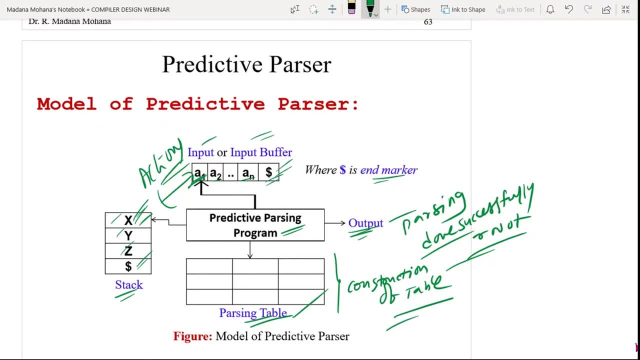 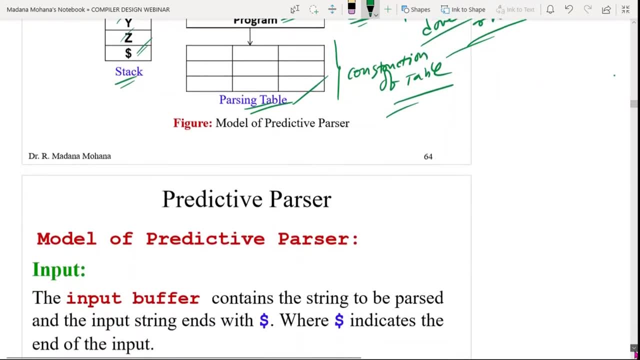 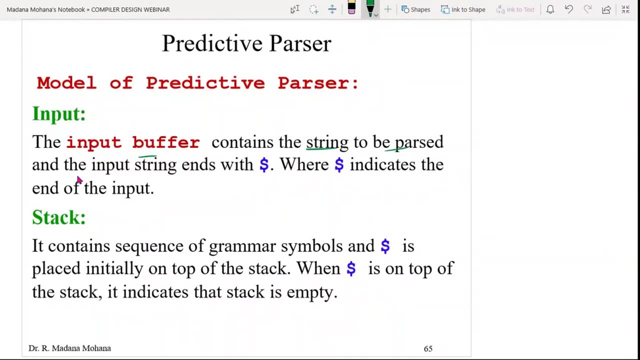 Construct the table. Construct the table. Construct the table. This is not a complete model of predictive parser, So briefly, let us see the description of all the components. I have already explained the same only given here. So the input or the input buffer contains the string to be parsed on the input string. 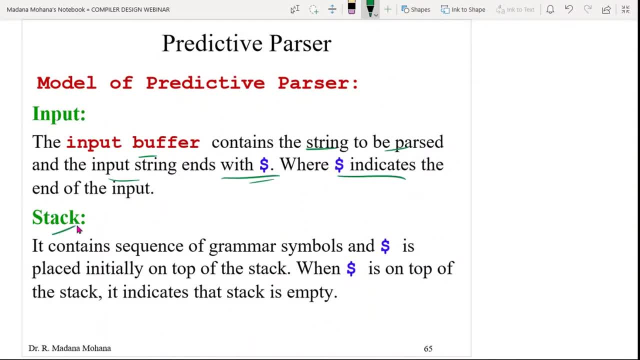 ends with dollar, where the dollar indicates end of the input and the stack contains sequence of grammar symbols and dollar is placed on attachment table And in the duration of the order of the data an out of foreign input other data is seen, is placed initially on the top of the stack. when dollar is on top of the stack, then what? 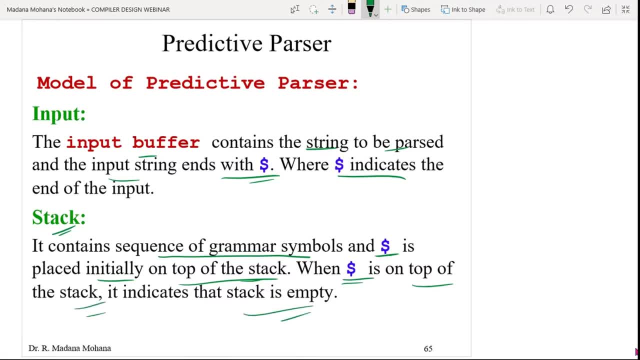 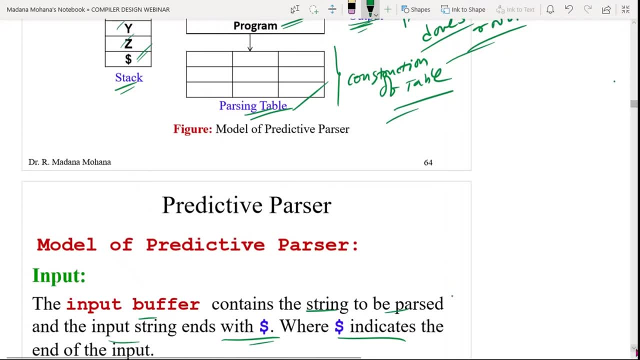 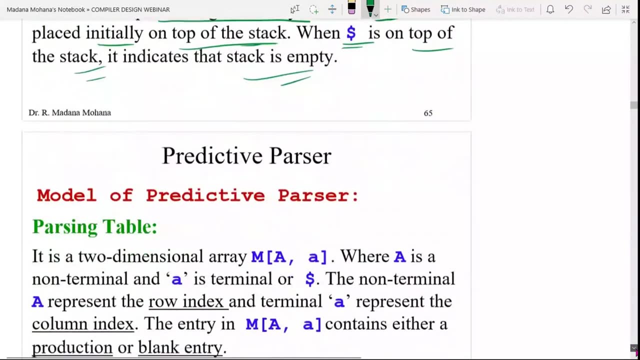 indicates stack is empty. normally in our data structures we may call it as z or z0, so here dollar is used. the meaning is same, whatever the symbol. so whenever the empty symbol that should be on top, then it indicates the stack is empty. then another important component. 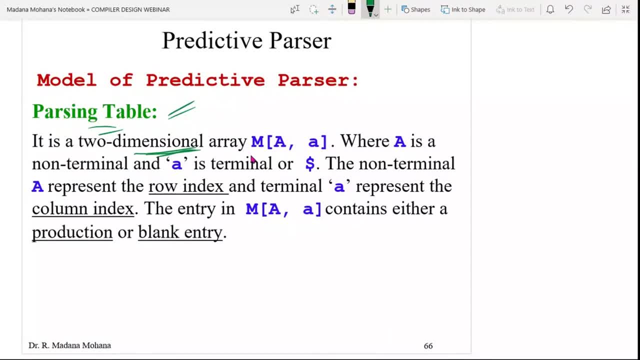 parsing table, which is a two-dimensional array, denoted with m, of a comma a. so here, where m is, we will call it as the model parsing model. so here, two-dimensional array. first it contains the grammar variable, followed by a terminal, terminal or dollar. also here you can see the entry. also it will be like this. so all the. 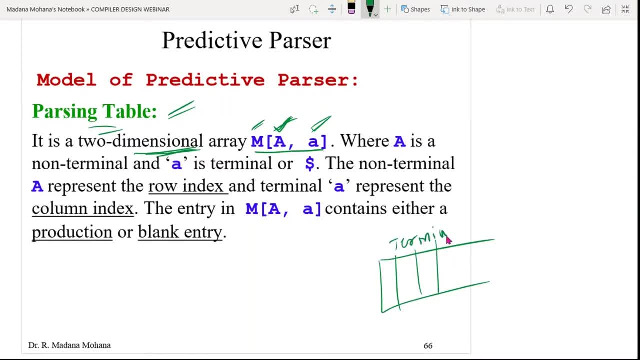 columns are terminals plus dollar, then all the rows grammar variables, so m of a comma a here this is a. here capital a. the entry variable a on terminal a. what is this value? the entries in the table are combination of the productions. only then, if any entry is. 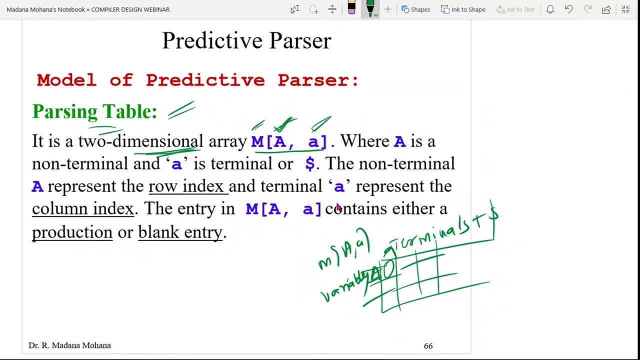 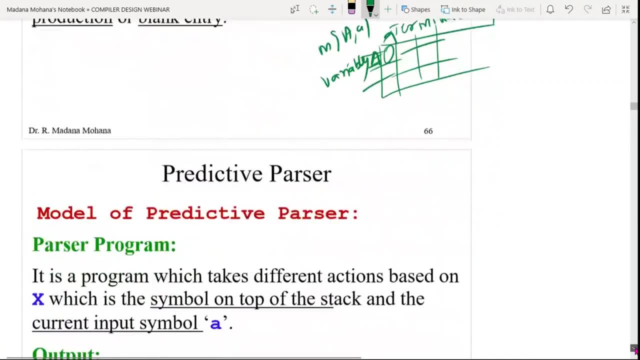 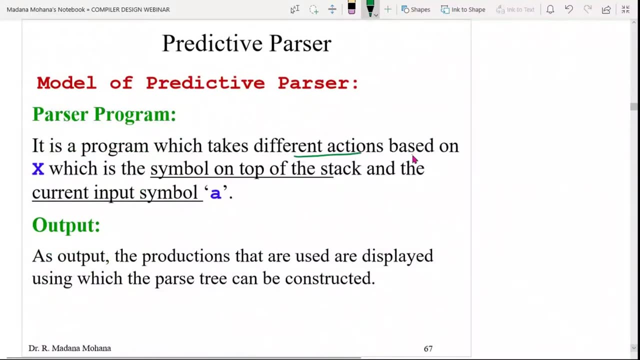 blank, so that indicates error. so this is the structure of predictive parsing table. then how to construct this table, that is our problem. then parser program: what is the role of boxer program, which takes different actions based on x, which is the symbol on top of the stack, and current input symbol? 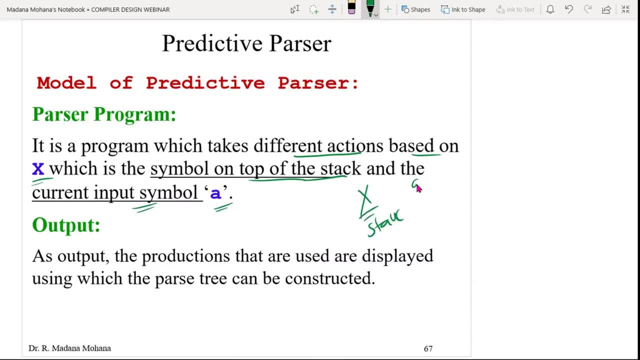 so here, x is the stack top symbol, a is the current input on input buffer. based on this, the actions. the actions means whether you have to simplify or move. then finally our sing is derived. then you can say parsing is completed or not, as the output, the productions that are used, are displayed, using which is the parse tree can. 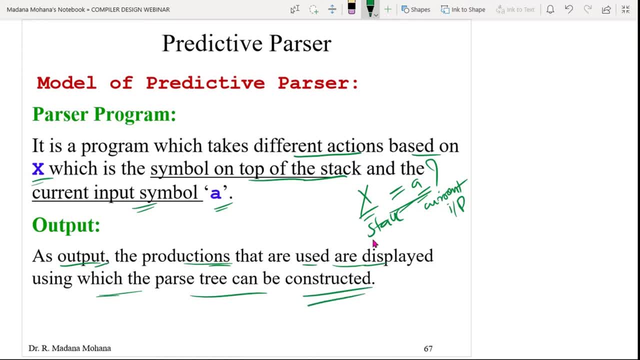 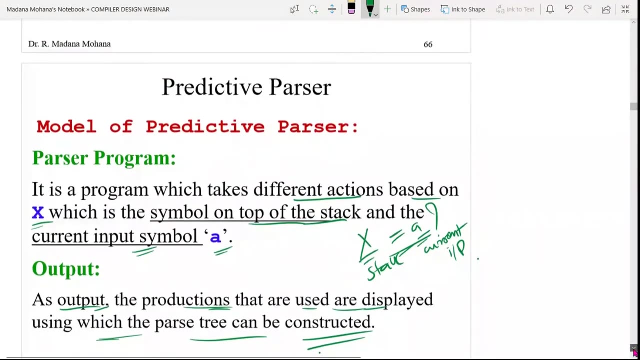 be constructed like in parse tree, whatever the productions we will use, to derive a string in top down parsing, starting with root here also. so finally our string is derived, then you can say the parsing is successfully. suppose if your string is not derived, you can say the parsing is not successful. like that, the same scenario here also we will use, but automatically. 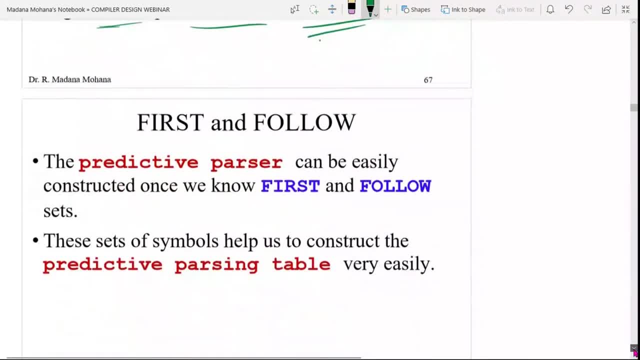 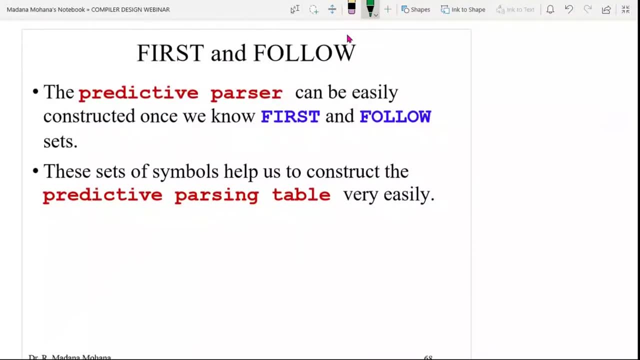 whenever you can implement this predictive parser, you can use this predictive parser using this algorithm, so it performs. okay, now for construction of predictive parsing table. the two prerequisite values are required: first values and follow values. so even in examination sometimes you will get question for the given grammar: find first and follow values. as a 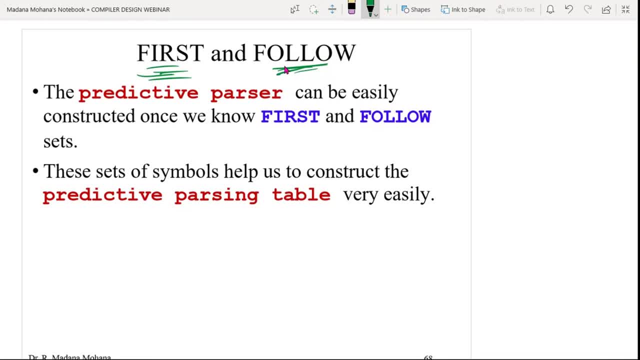 two more questions or even long answer, part a or part b, something like: or write the algorithm or rules for calculation of first and follow values. so these are all very important for predictive parser. with this only we will construct, so the predictive parser can be easily constructed once we know first and follow sets. these are: 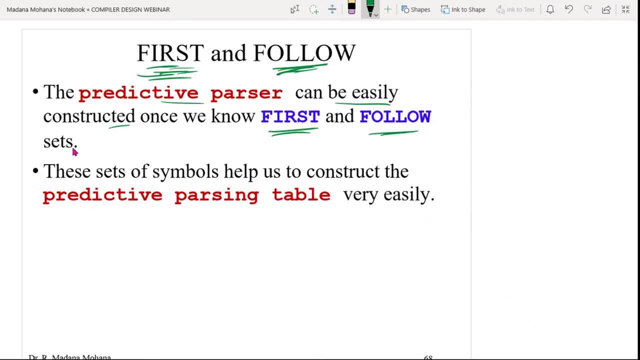 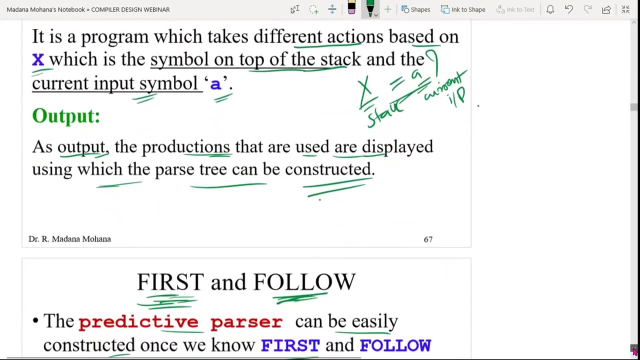 not single values. actually, more values are there. that's why we will call it as sets. so these sets of symbols help us to construct predictive parsing table very easily. okay, now let us see how to construct this with examples. briefly, we will explain then, followed by how to construct the predictive parsing table. once you know these values easily, you 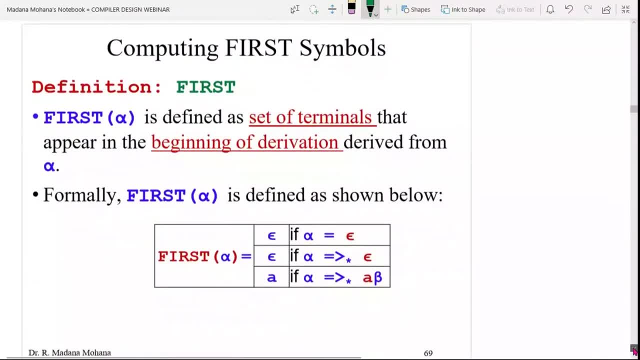 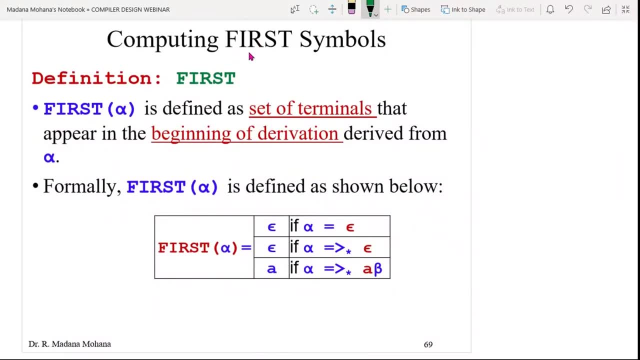 can construct the predictive parsing table using the algorithm. now you can see the first value is very easy how to compute first value. so even for first and follow, we are having certain rules. simply by following the rules easily you can construct first how to compute first values. if you can see the definition of first, for example, first half alpha, first. 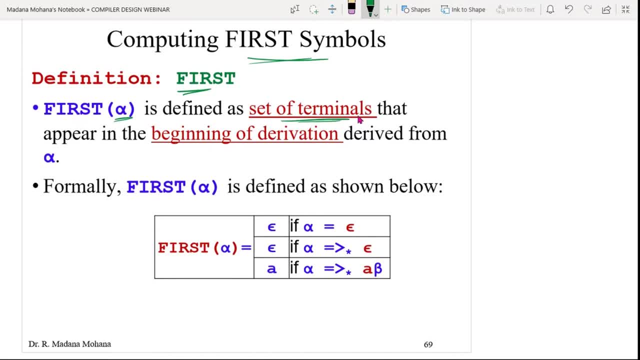 half alpha is defined as set of terminals that appear in the beginning of the derivation derived from alpha. suppose alpha derives something in the derivation beginning of the derivation, any terminal is there that terminal or set of terminals are called as first values. formally, let us say this can be defined as shown below: first half alpha equal to suppose if alpha 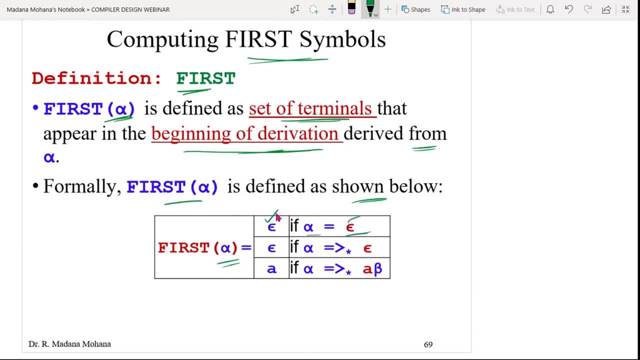 here you can see: by default null is there means first half null equal to null. only then alpha derives null, also using derivation so directly. for example, alpha derives null, then what is first half alpha? null, then alpha derives null. by substituting you are getting null. so again the first half alpha is null. only then, if you are having derivation like this, 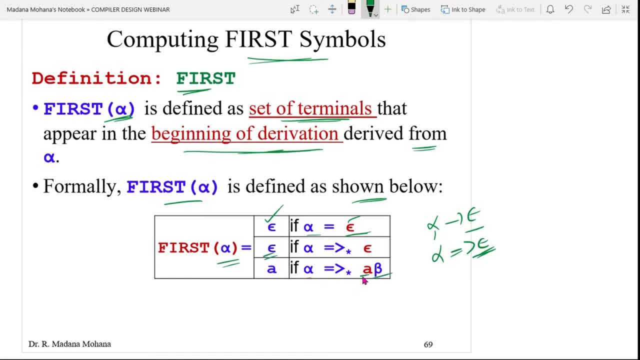 alpha derives terminal a beta. in the derivation beginning you are getting the first half alpha. this is the beginning. what you are having: a terminal a. now a is first half alpha, like this. so the first values are combination of terminals, including null, also in the direct production. if you are having a terminal in the right hand side of the beginning, take, 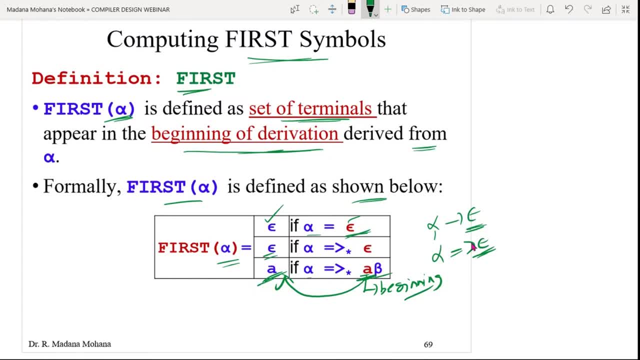 the terminal directly number. you can take the null at the first value. so but you do not have direct terminal, direct null, but you are having substitutions after first half. After substitution you may get in the derivation is of the form terminal, followed by something At the beginning. terminal means directly. you can take terminal as the first value. 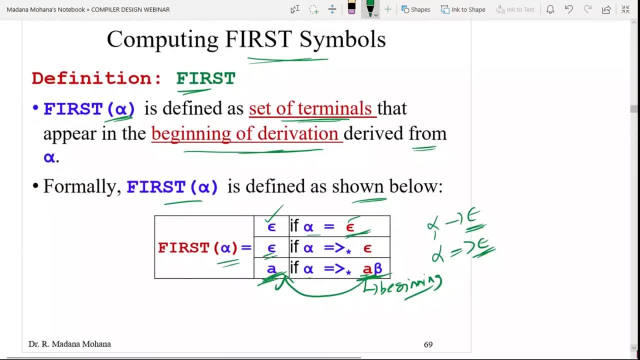 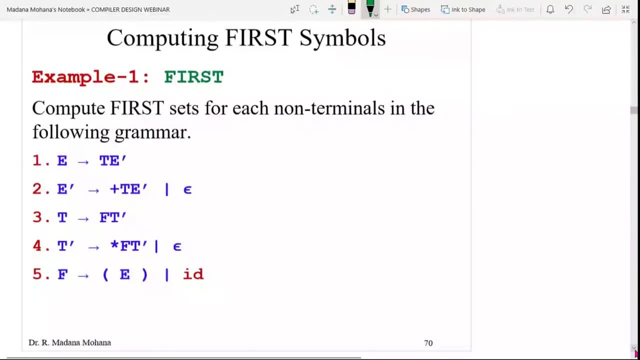 That is the definition here. Okay, now let us see the one example, followed by what are the various rules for computing? first value, For example, the grammar is like this: See the first sets for each non-terminal in the following grammar: we need to compute: 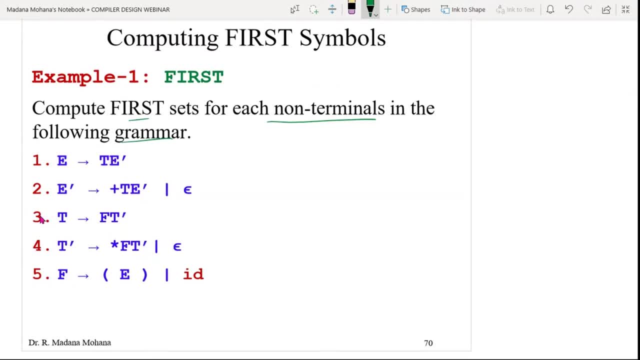 In the left hand side of the production. whatever the variable or non-terminals for those, we have to construct first values. So e, dash, t dash. we have to compute here first of e the left hand side, one That depends on the right hand side production. 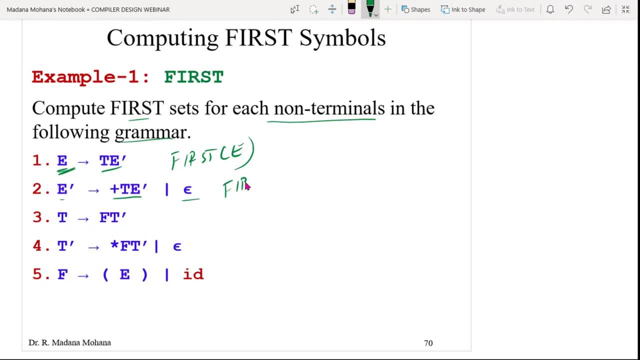 Here e dash dash plus t dash are null. We have to compute here first of the variable e dash, this one, t dash f t dash. here we have to compute First of t. then here t dash dash star. f t dash are null. here we have to compute first of t dash. here f dash is e within parenthesis, or id compute first of f. 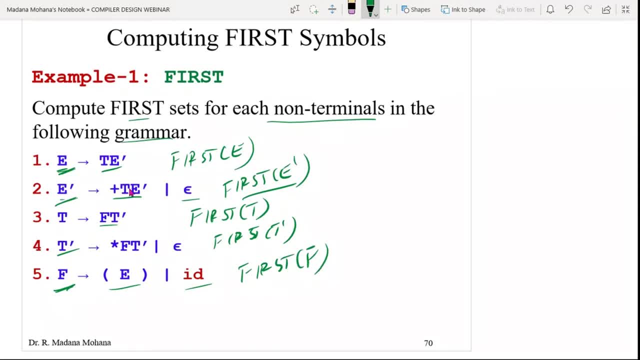 So here, by using right hand side productions, if directly you are having terminal value, you can take directly those values. If not a terminal, if you are having variable, then again you can find first of those variables in the derivation. Okay, 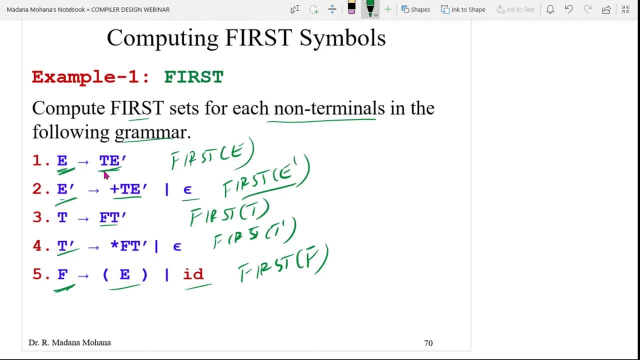 Like that Here: e dash, t dash directly. you do not have terminal First, you need to find out first of t. Then, whenever, if you want first of t coming to t dash, f, t dash, you need to find out first of f. 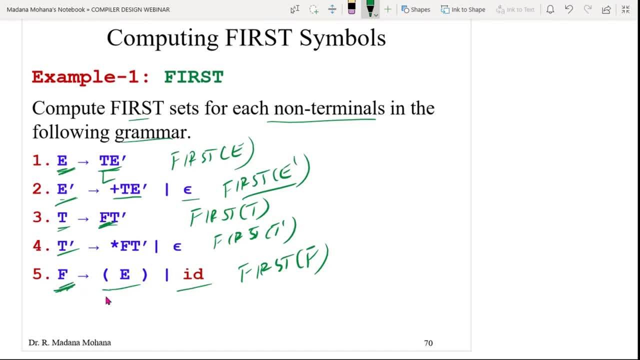 Again, coming to f, first of f, you can find from this Here, you can see here: this is the production. you are having terminal In the beginning, we are having terminal left parenthesis. Or you are having terminal id. id is also terminal. 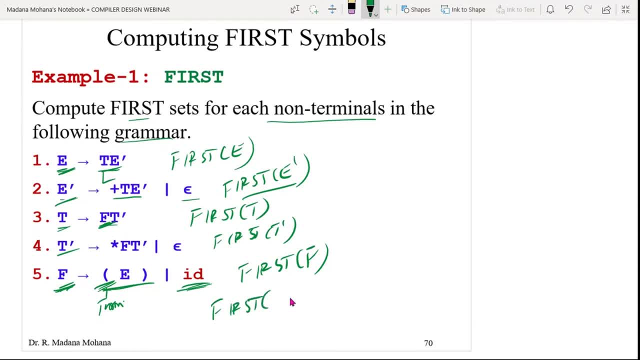 So Here, first you can find easily first of f, equal to actually this, you can write first of left parenthesis e, right parenthesis The first one. only you are having only terminal at the beginning, only take the first terminal. only If you are having two terminals, also only first terminal, you can consider: 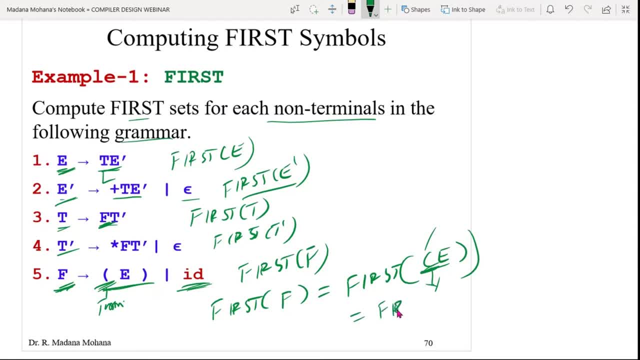 So this is the first value. So here you will get first of left parenthesis equal to left parenthesis. Then another production You are having: first of id- Id is a terminal, So first of id equal to id. only Now combine all these. 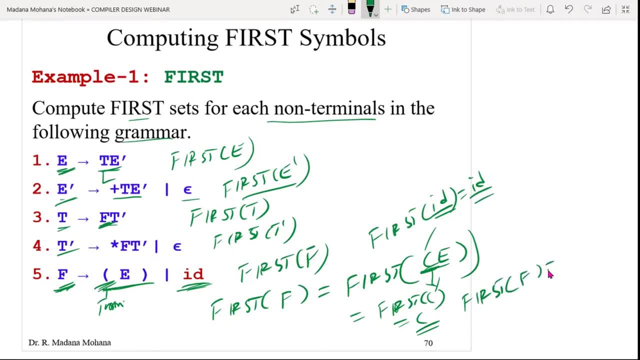 Therefore, first of f, equal to left parenthesis, comma id. These are all first values. So once you know the first values, Now here, first of e, we are finding this one, E equal to substitute. what is the production First of t, e dash. 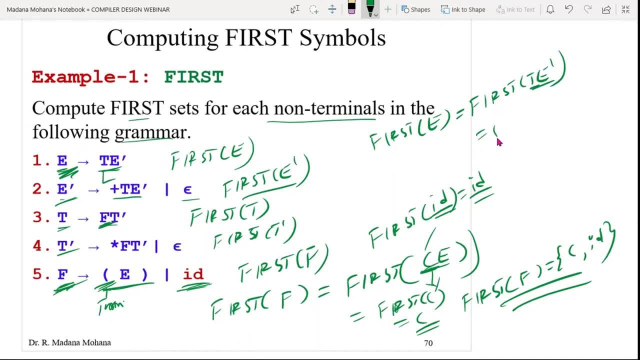 Now, first of t. e dash means first of t. this is equal to first of t. Now, what is first of t? t derives ft dash. This is equal to first of ft dash. Again, first of ft dash means first of f. you can find out. 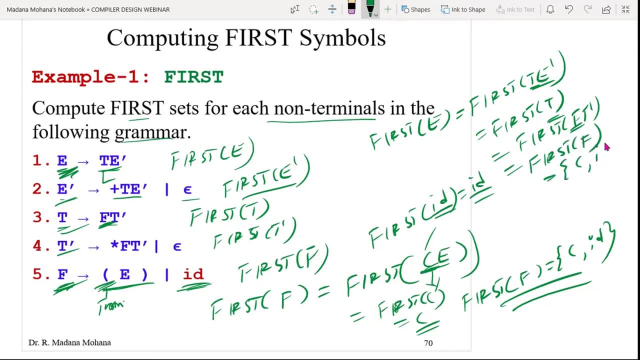 First of f equal to: here already we calculated left parenthesis comma id. Therefore, first of e, equal to left parenthesis comma id. First of e, once you know, Then first of t. also, First of t is also left parenthesis comma id. Once you know first of t, then first of f. already we calculated. 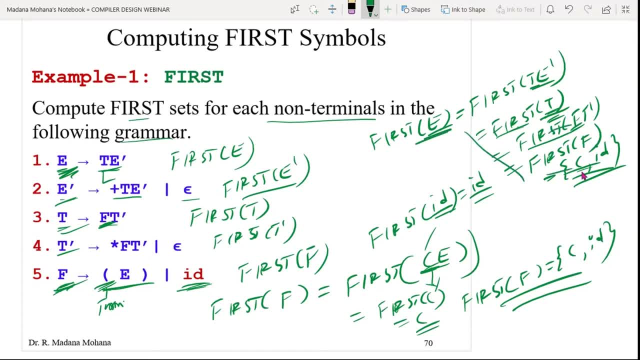 So now, first of e, first of t, first of f. all three are same. Left parenthesis comma id: This is equal to left parenthesis comma id. First of t is also left parenthesis comma id. Then first of f, equal to left parenthesis comma id. 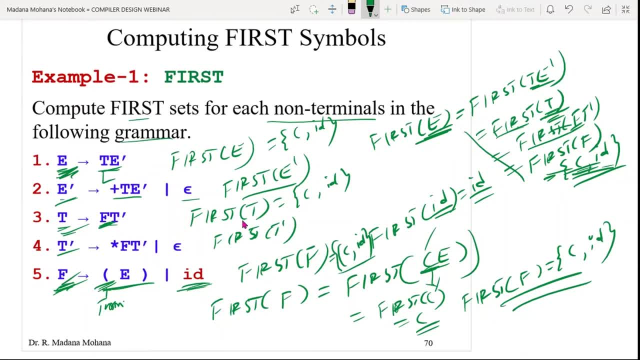 Okay, Now e, t, F values are calculated. Then coming to e dash. So e dash derives plus t dash, Already, starting with terminal. So first of terminal, followed by anything Terminal only you can take. This is the first value. 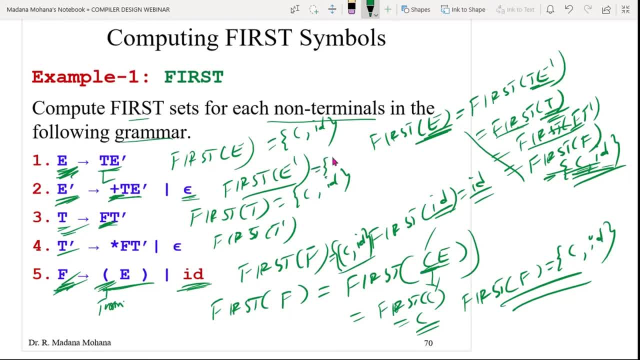 First of null equal to null. Therefore, first of e dash, what you will get Plus comma null. Then, similarly, first of t dash star, ft dash Star is terminal, Directly terminal or direct null. First of t dash equal to star, comma null. 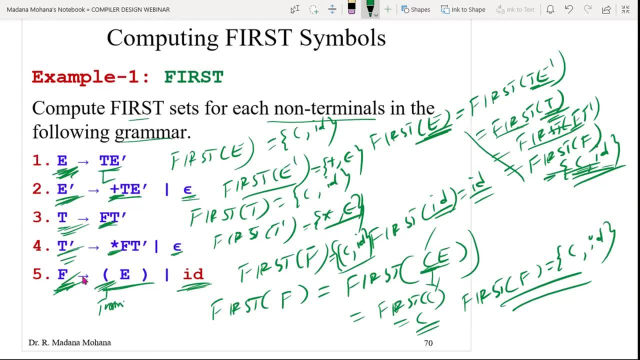 Now you can see First of e, first of e dash, first of t, first of t dash, first of t dash directly. we calculate it So. but we are having rules here to calculate all this. So suppose in the right hand side all variables derives null. 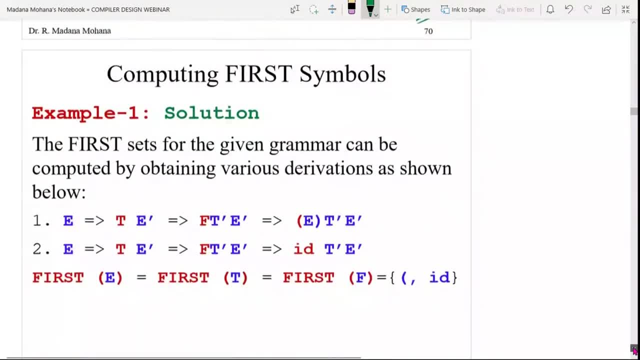 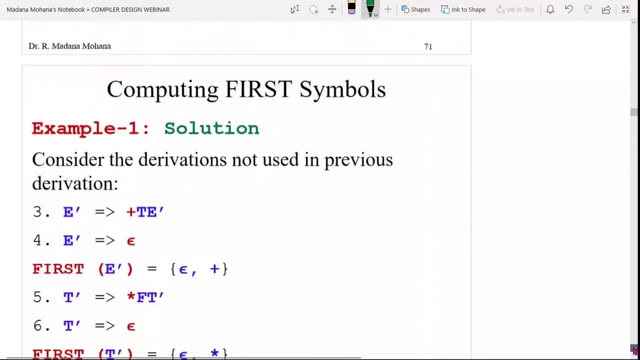 At that time, how to compute first value, Or, after substituting a variable by null, how to calculate Like. all this comes under the rules. So whatever I explain, the same is shown here. Then directly we will move to the 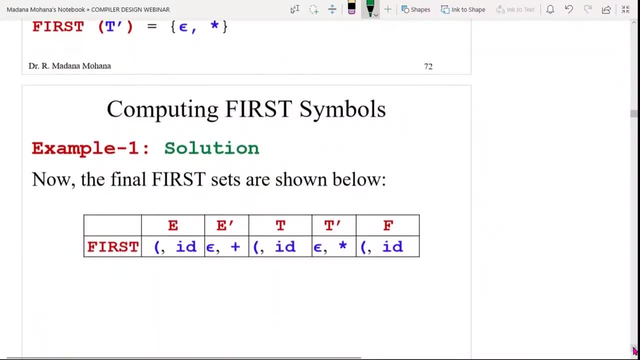 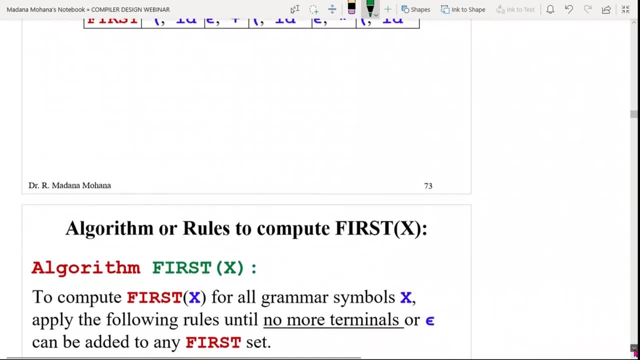 Rules for computing all the first values. This is the table. The final first values for all the variables are non-terminals. In the algorithm you will get all the possible rules for finding first values In examination. sometimes they will ask this algorithm also. 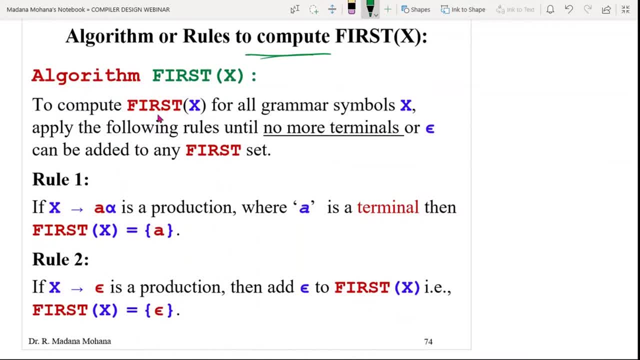 Or rules for computing first value. All these rules you have to write, So to compute first of x. x is the grammar symbol variable, Applying the following rules: until no more terminals are null, Can be added to any First set value. 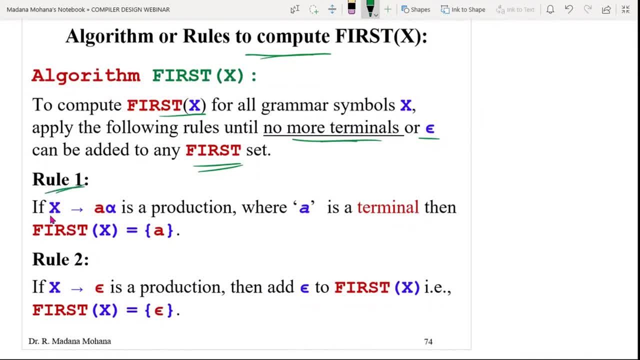 Rule 1. If the production is of this form, x derives a. alpha is a production. Here, right hand side, small a is a terminal. Then first of x equal to directly terminal, you can take Direct terminal value. That is rule 1.. 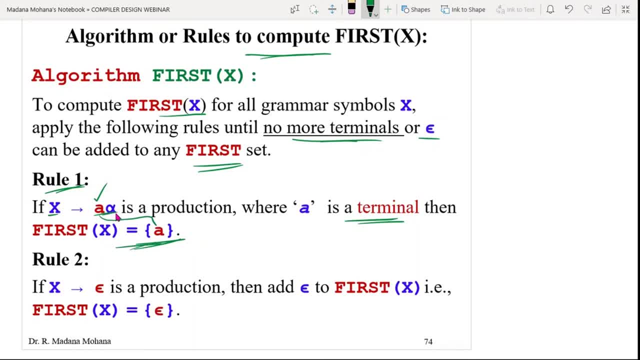 It is very simple: If any production, starting with terminal in the right hand side, are null, The null is in the second rule. x derives, null is a production, Then directly, This null is added to first of x. Therefore, add epsilon to first of x. 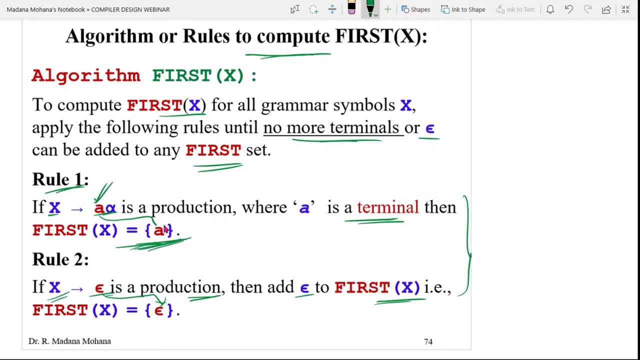 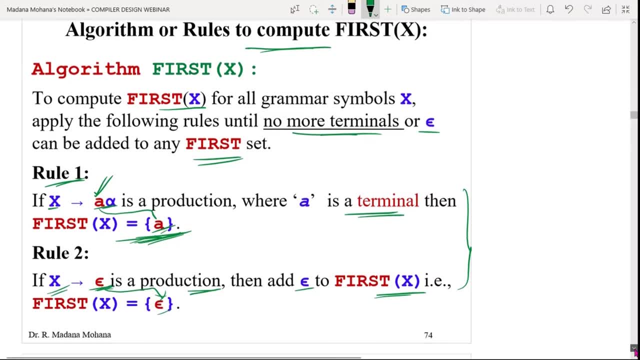 First rules are very simple. Right hand side direct: a terminal. That is added to first. Right hand side direct: null value. That value is added to first of x. So if it is not the rule 1 and 2 form, The productions are of the form. 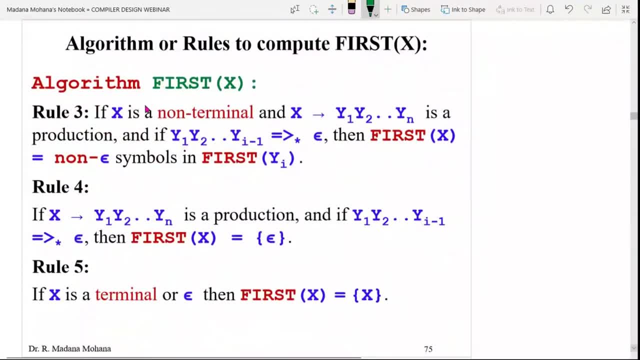 Like this you can see the rule 3. Rule 3. Same. the production is of the form: x derives y1, y2, and so on yn. Here. Here y1 to yn are the grammar variables. directly, no terminals are. there is a production. let us assume the right hand side: all y1 to yn derives a null. here you can see then what you have to do. suppose here y1 derives null, next y2 derives null, and so on, yn derives null. right hand side: all the variables. 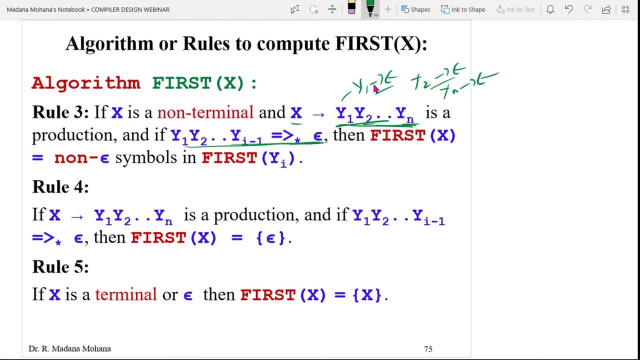 Contains a null production, Then what you have to do, You can add Whatever the variable you are finding, if it is first of y1, first of y2, and so on, first of yn, suppose first of y1, and so on. first of yn. 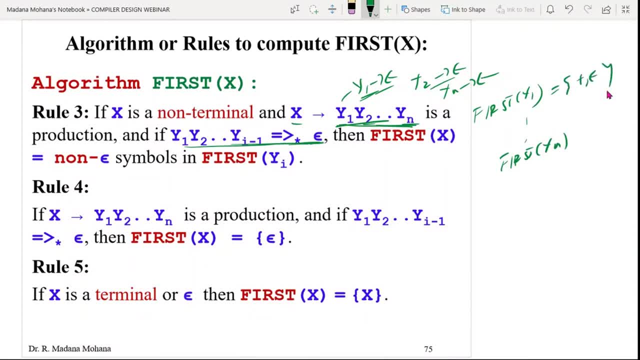 So it is having some plus comma null First of y1.. Then what is the left hand side? first of x, First of x equal to First of y1 minus null Non epsilon Values. first value should be added to first of x here. 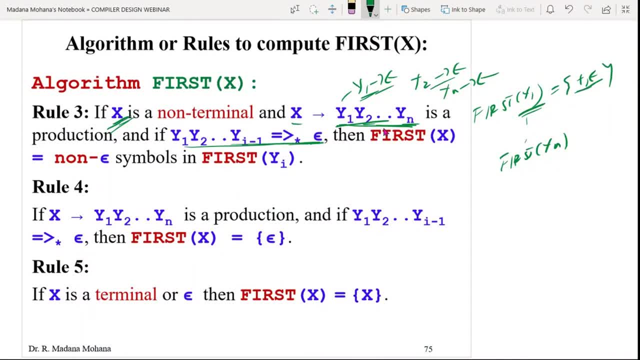 So now here you will get. only plus is the first of x the same. here you can see: x derives y1 to yn is a production, then if y1 to yn and so on Derives null, that means either any one contains null, Whenever you are finding first of its value. if y1 contains null, 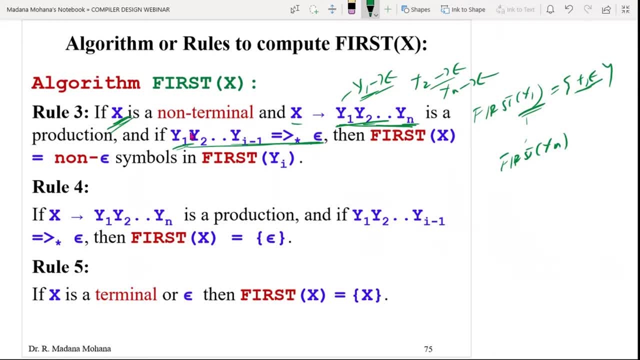 That means Derives null, But y1 contains other than null, also as a first value, Then non null values, Non non null first values of y1 can be added to first of x, Then first of x equal to non epsilon symbols in first of yi. 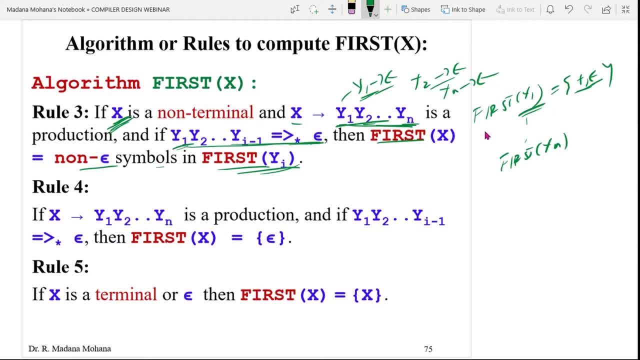 In your examples also we will see. Then you will get clarity. That is rule 3.. Whereas in rule 4, almost similar, but entire right hand side is null. Here you can see The rule is written similar fashion, But entire right hand side is null. 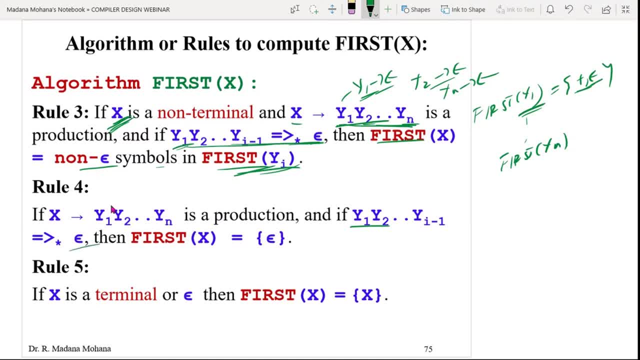 Then what is the first of x? also, X derives y1 to yn is a production Entire. right hand side derives null Means y1 null, y2 null, and so on. yi minus 1, all are null. Then entire right hand side value is null. 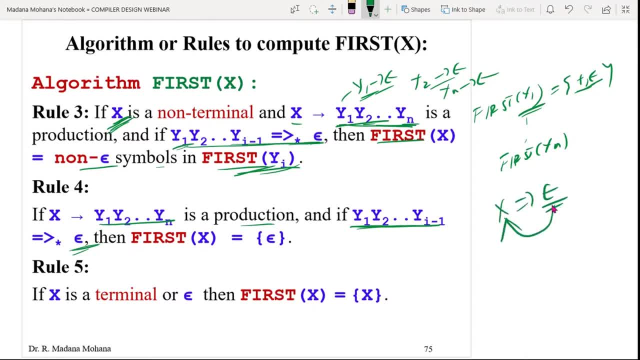 That is x derives null In rule 3, sir. Yeah, tell me, In rule 3, entire right hand side is also null. no, sir, No, no, no. actually that is the derivation actually. So if any one, If any one is, for example see, y1 is null, then you have to consider y2. suppose y2 is not null. 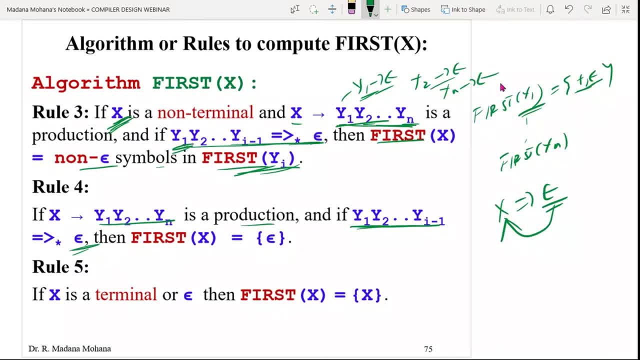 At that time non epsilon symbols of first of y2. you can add: That is the intention actually, If any non terminal exists in right hand side. Right hand side, see, for example, y1 is not null, Let us assume So y1 contains direct terminal. 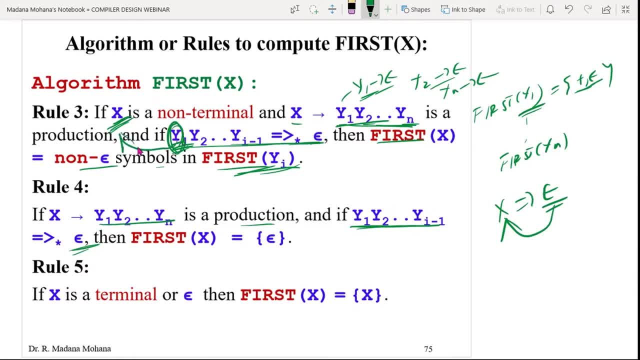 So then direct terminal is added to First of x, like previous rule. Suppose y1 also contains null, Means the production like this: y derives null. Now you can substitute y as null, Then what you will get? this will be eliminated, then coming to y2.. 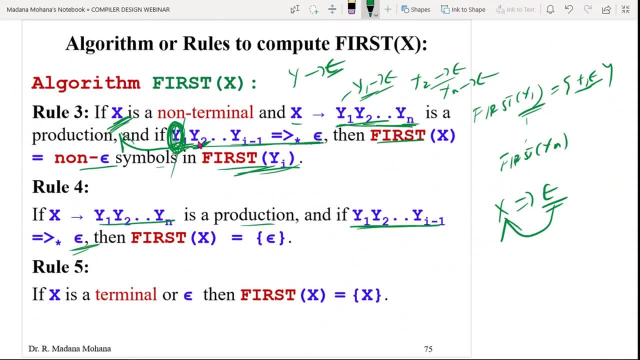 Then we will come to y2 variable. actually, If y2 contains null or a terminal, So other than null, you can add to x like this, Like this: Not all: The first one null, Then go for second one. If second one not null, then directly take this value. 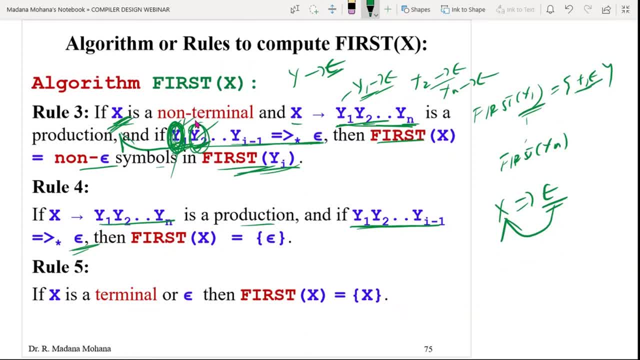 If first one, not null, directly, take first variable, First value, is only like this. Anyway, in the example I have given, clearly you will know: Whereas rule 4, complete right hand side, is null, But in the production I have written similar. But the intention is like this: here all are not null. 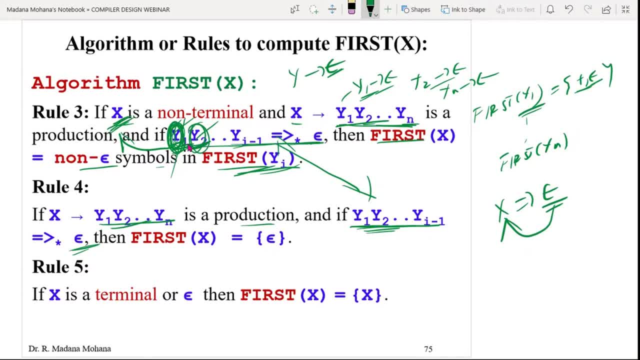 If any one in the right hand side. If first one is null, Then second one we have to consider. Second is null, third one we have to consider. At that time non epsilon symbols needs to be added like this, Whereas rule 4- it is not like all the variables in the right hand side are null. 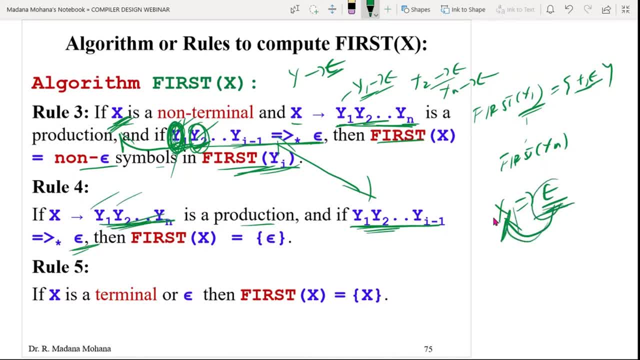 Complete, you will get null value. Then null is added to first of x. That is like rule 2.. Rule 2: what we are having: x derives null, Then null is in first of x like this. Then rule 5: direct terminal or null value. 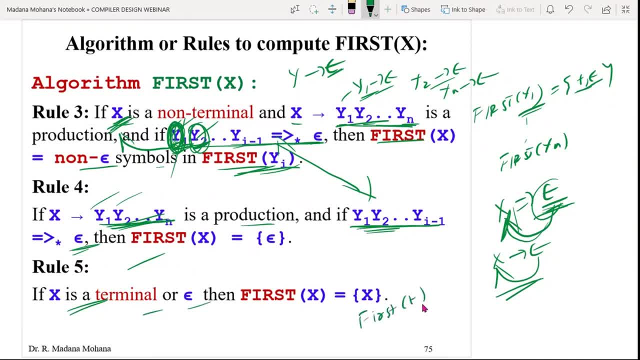 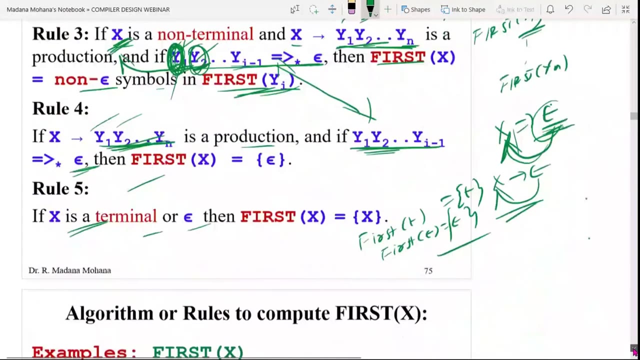 For example, you are having first of terminal, First of null, Direct value only. you can take Terminal, only null only, like this. Anyway, now rule wise, let us see the examples. Now we will get more clarity. If right hand side, if any variable derives null. 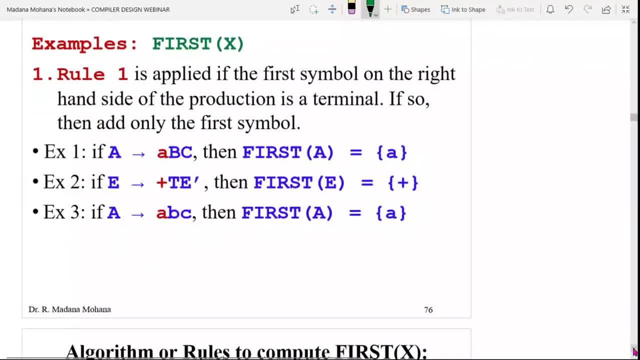 Then only you can go for rule 3 and rule 4.. Otherwise, by using rule 1 and 2 directly, you can find, For example, rule 1. let us see what is rule 1.. The productions are in the form of a derives terminal, followed by any. 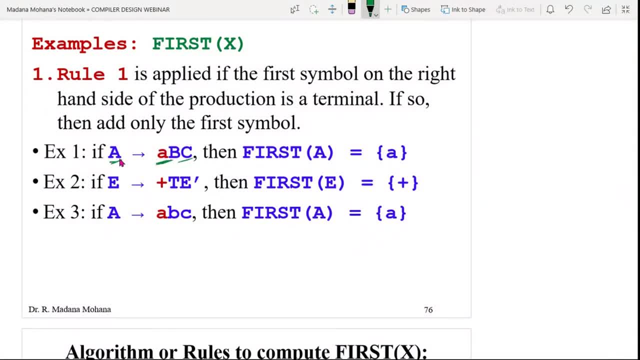 So starting right hand side, terminal means direct terminal is the first value, First of terminal a, b, c. Direct terminal is there First of a. equal to terminal a, e derives plus t, e, def. Plus is direct terminal. Now, plus is the first of u value. 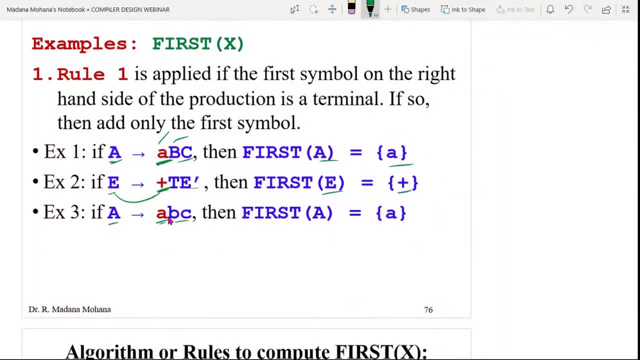 Then a derives terminal, a. Three terminals are there, But here you can consider only Starting terminal only. don't consider second third terminal, only starting terminal. First of a equal to small, a, only that is rule 1.. Similarly rule 2, when you can use rule 2 only. 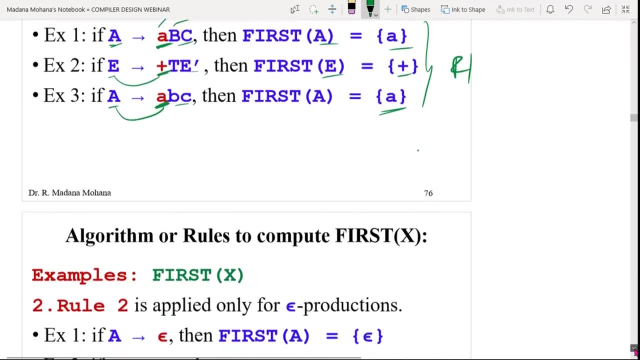 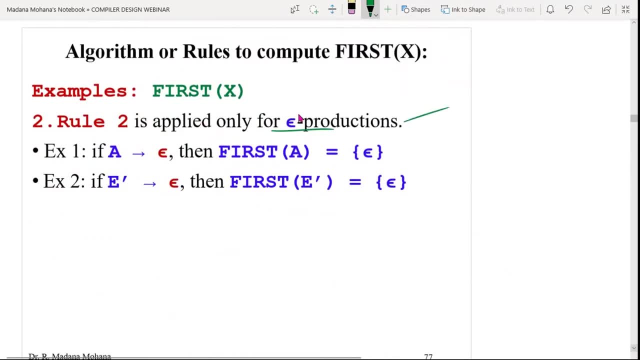 Direct null value is there If any production Contains epsilon- right hand side directly. Now you can see Is applied only for epsilon productions. a derives epsilon, Direct epsilon is the first of a. Then e dash derives epsilon. Epsilon is the first of e dash. 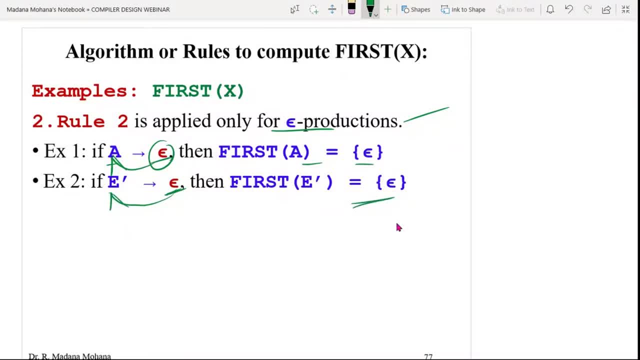 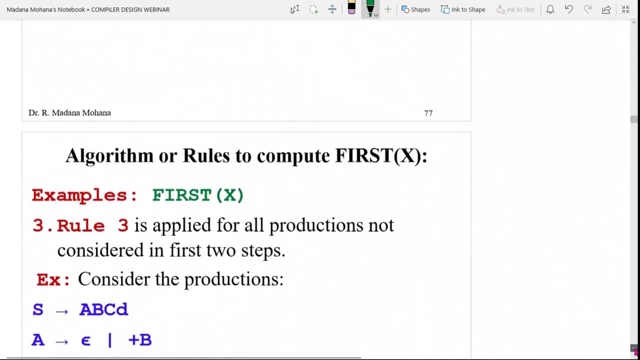 So rule 1 and rule 2. rule 1 is only for terminal in the right hand side, Then rule 2 only epsilon in the right hand side. If more than one terminal is there in the right hand side, Only first terminal needs to be considered. 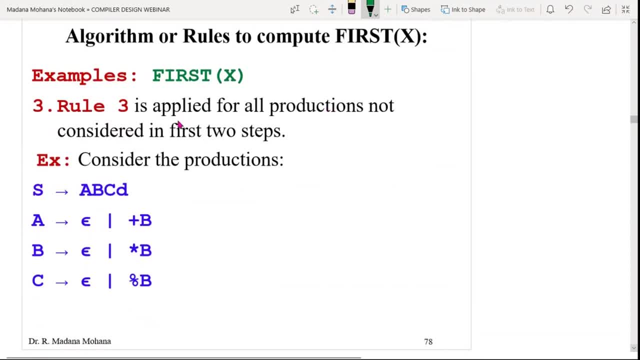 Now let us see the rule 3.. So rule 3 is applied for all the productions not considered in the above two steps. The production is like this: now you can check S derives variable a, variable b, variable c, Followed by terminal. 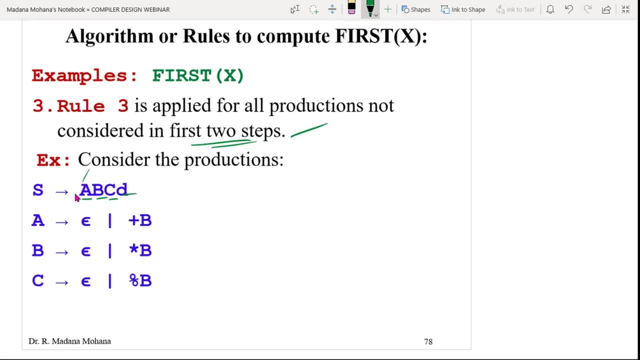 So If capital, a First value, you can find out Directly, you are having Non epsilon first values, then you can add to first of you, But you first of a contains null, At that time What will happen? let us see here. then you can consider the second variable also. 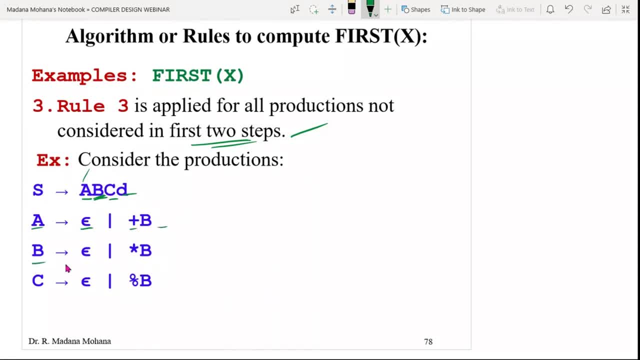 Now, a productions contains null, followed by plus b. B productions contains null, followed by into b, C productions. So for this, directly using rule 1 and 2, you can find out By rule 1.. First of a equal to, You will get plus only. 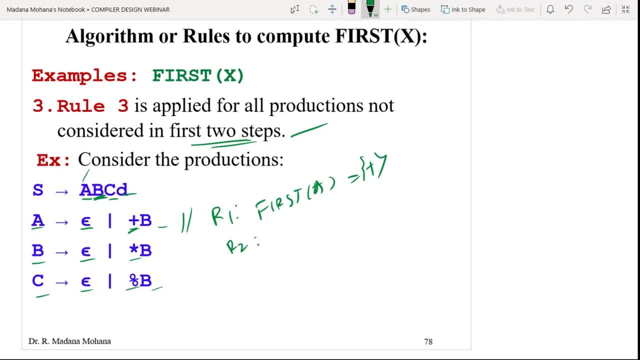 Because it is starting terminal. Then for rule 2.. First of null. First of a equal to null. only By combining these two Plus comma, null. These are all First of A values. Similarly, First of b, equal to. 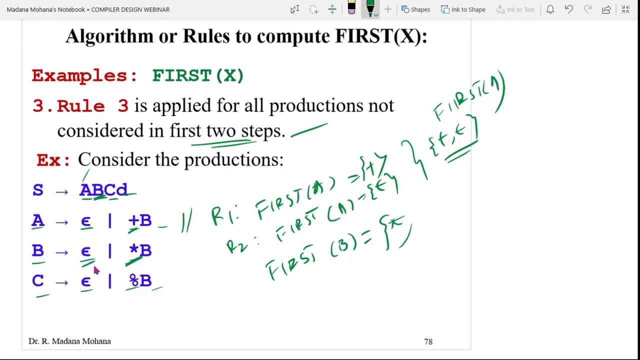 By rule 2, rule 1, into: By rule 2, null. Then first of C equal to By rule 1. Percentage Comma: by rule 2: null. Ok, This a, b, c directly We obtained using rule 1 and 2.. 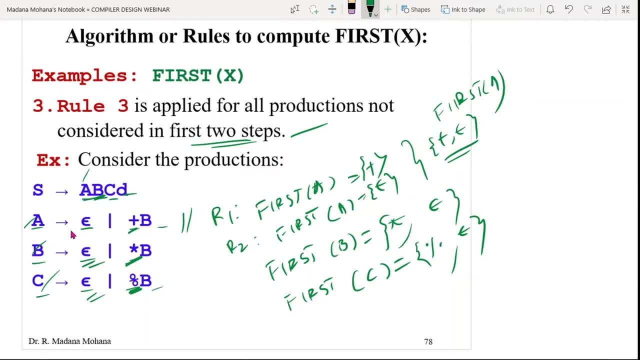 But The starting production is not in the form of Rule 1 and 2.. These are all in the form of Rule 3 actually. First, what you have to do First of a. you can see What is first of a actually. 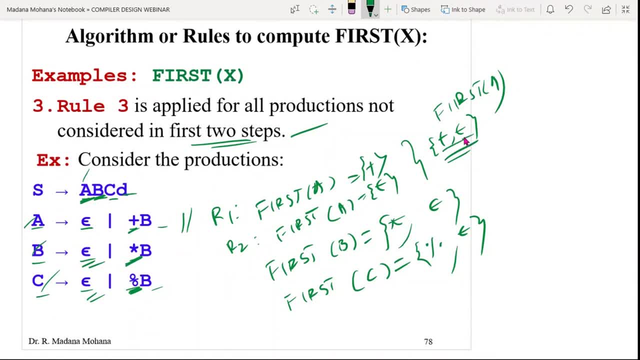 Plus comma null. So here It contains plus comma null And also a derives null. At that time Non epsilon First values should be added to First of s. So here you will get First of s equal to First of a. 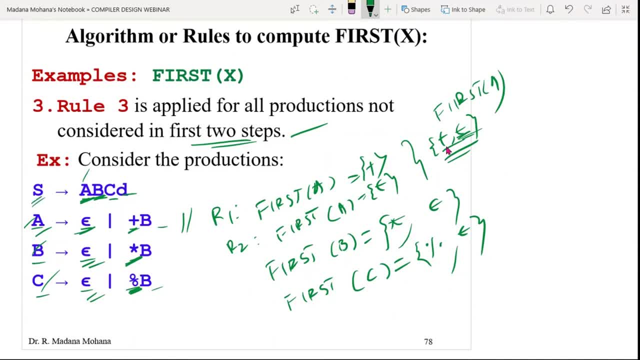 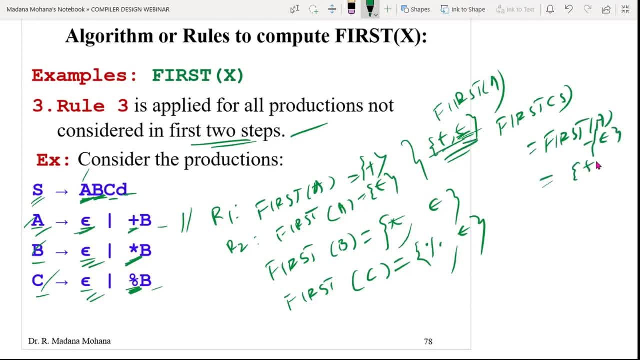 Minus undelt. wow, What you will get First of a actually Plus and null. You will get Plus only Why you Have to Consider This one actually. Yeah, Contains null production, Suppose if a does not contain. 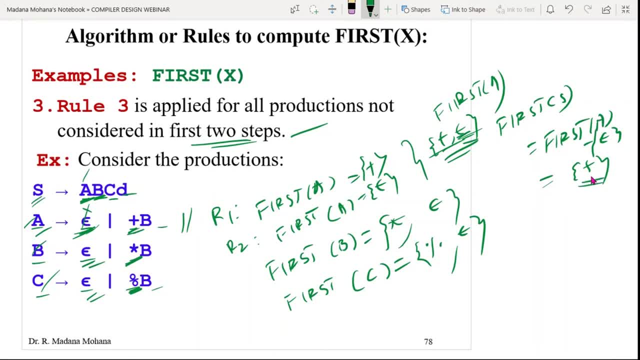 My production, This is not there. Then First of y Equal to 1. Place At that Time, Directly, First of a Equals, You will get Guess. so. So whenever a contains Now, Then 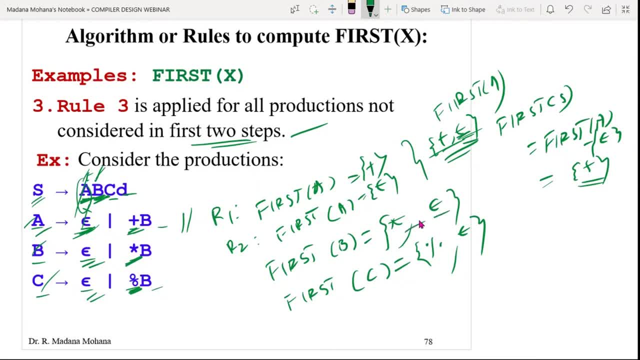 So what is first of B actually into comma? null, So, and also B derives null. So that is why first of S equal to first of B minus null. Now star Star will be added. If B does not contains null. let us assume only star B is there. This is not there, Then first of S equal to first of star only. 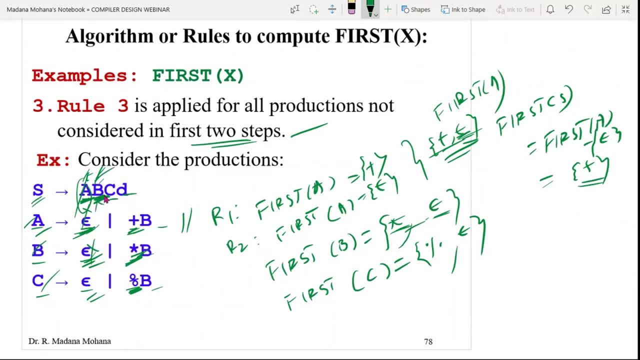 Now, if B contains null, we substitute null. Now we will get A. B are null. Next variable is C. Now you can continue with C. First of C equal to null comma percentage. So why? because C derives null Non-epsilon symbols, that is, percentage is added to first of S. If first of C not contains null, then only percentage will come. Then we cannot proceed with next symbol. 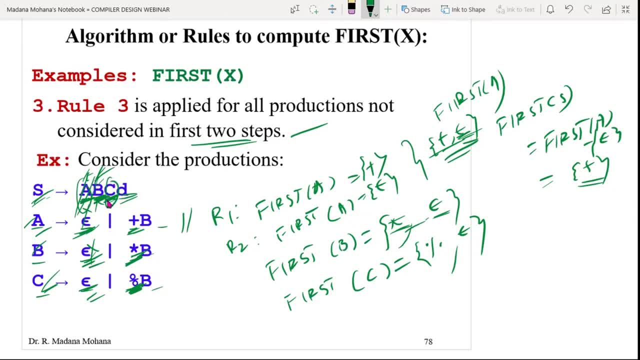 But C also derives null. If we substitute A, B, C as null, Now what you will get is C derives only terminal D By rule 1, D is also first of S. In this case first of S equal to what you will get. plus into percentage D. All values comes under first of S. 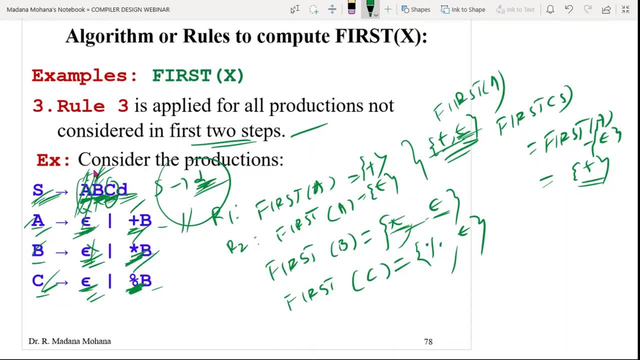 Suppose here next rule 4, right hand side, all are null. That means here D is not there, A, B, C, Now all are null. Now means right hand side compulsory S denies null. then this also added to first of yes along with plus into percentage null. 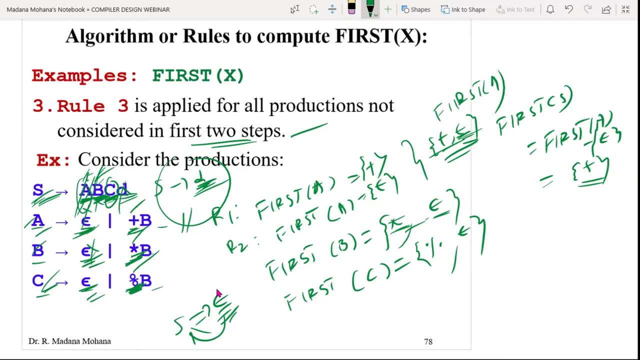 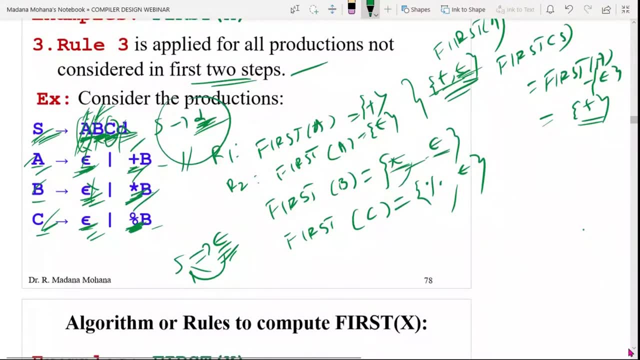 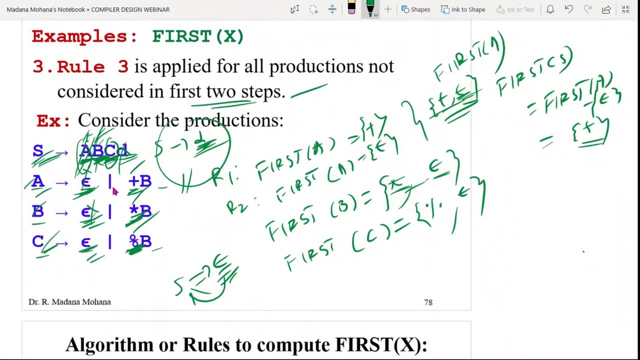 is also added. that is rule 4. now you will get clarity, the difference between rule 3 and rule 4. so, sir, now, according to rule 3, yeah, first of yes. first of yes is plus star percentage and d and epsilon. no, sir, epsilon won't come here. why? because yes, right hand. 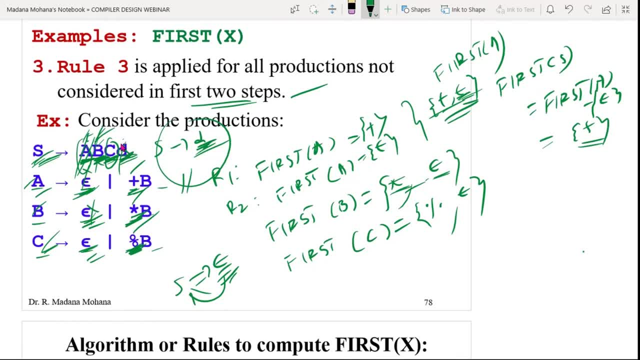 sir, completely does not contains null. here d terminal is there, it is not null. even by keeping a, b, c, null d remains same. so, right hand, sir, you won't get null now. first of s is first of d, sir, first of s, equal to first case. first of a minus epsilon, then first of 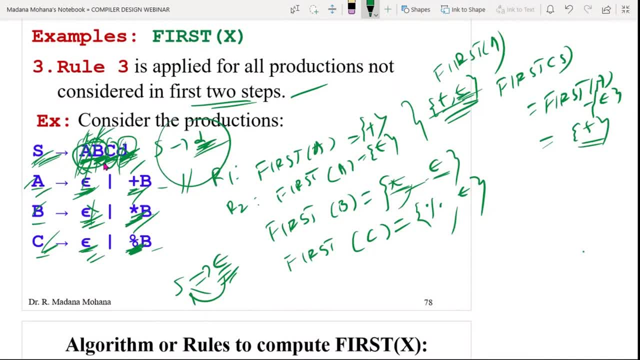 b minus epsilon, first of c minus epsilon, then first of terminal, all the four we have to consider. okay, what is the final answer, sir? final answer: plus comma into comma, percentage comma, terminal d, according to rule 3, first of yes. okay, so now rule 4. now you can see, you will get null. 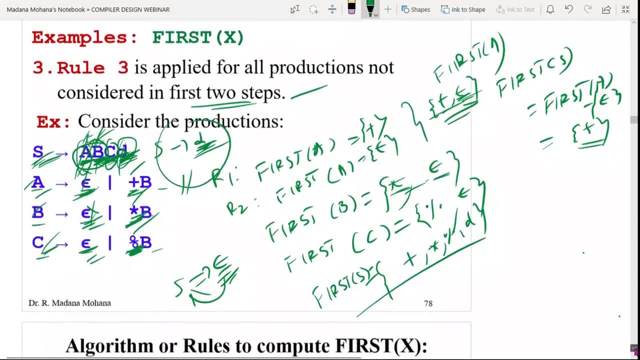 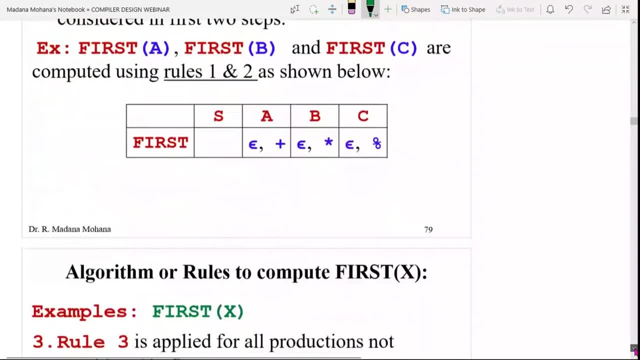 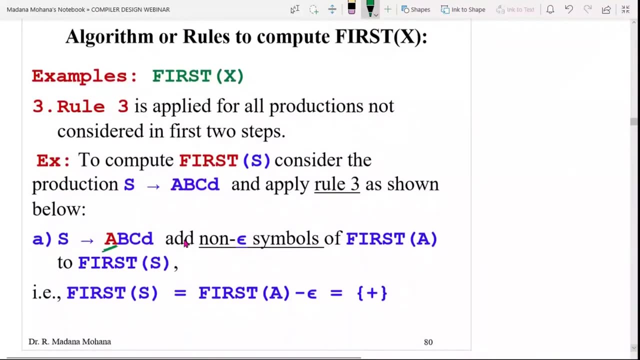 also let us see the rule 4 example. here you can see step by step. whatever i explain, the same is shown here. so first two, here you can see: first would have considered first variable. so a contains null production. that's why non epsilon symbols of first of a added to first of s, first of. 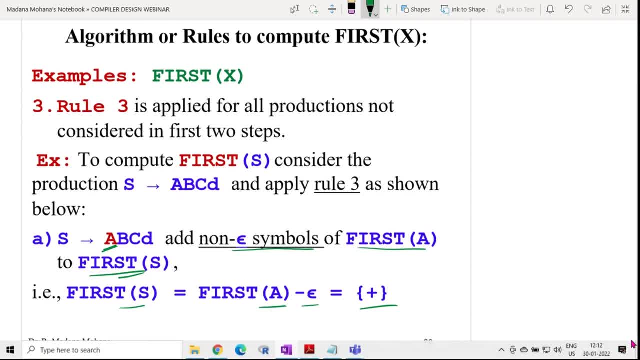 s equal to first of a minus null. here plus is added a. suppose now here: s derives a, b, c, d. this is production. now you can substitute a derivational here. what will happen? s derives b, c, d. this is a new variation of a. you can see a derivative of a here. so the first three: 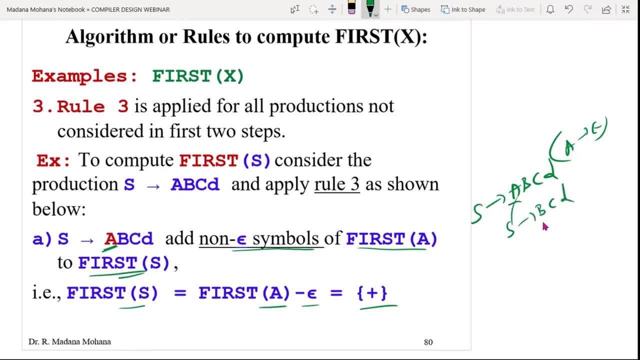 Role. What will happen after that? first of a minus null. here plus s is added. here a is added. it's not a normal thing, it's an expression of a. this is different way of is it is called. So this is removed. now B is the first. that is why, again, after substituting B as null, 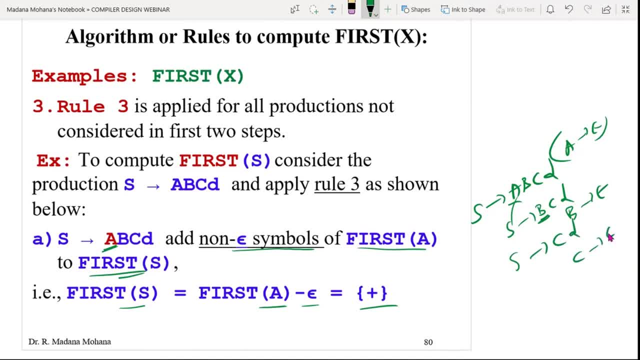 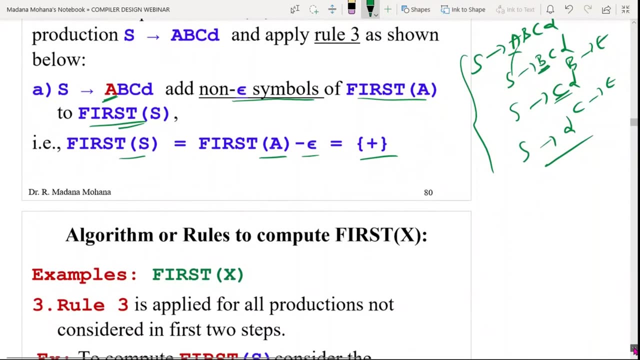 what you will get first of C, D. next, we are having null production for C. by substituting C as null, you will get it D. like this: by combining all this, you will get all these values. even a small d is not there, right hand side, only up to A, B, C. now all are null. then epsilon. 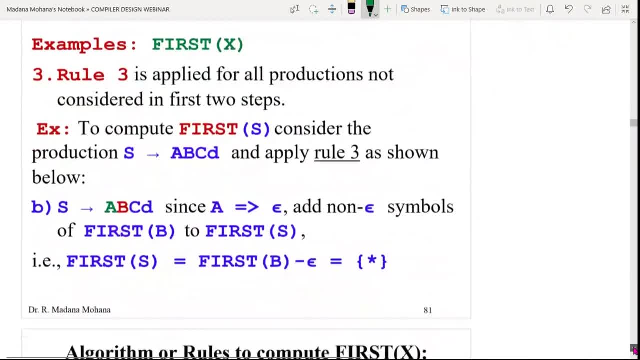 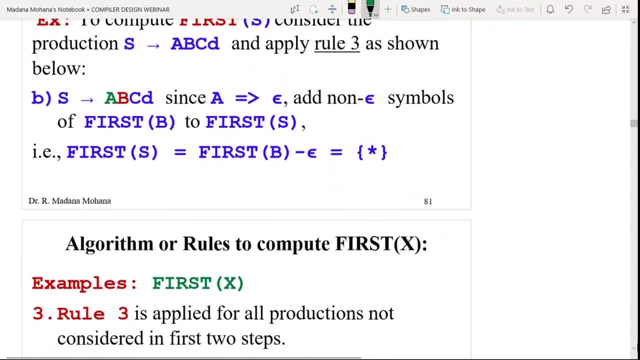 is also added here, that is, if A is null. now, second case: here A derives null. then we are coming to the variable B. if A derives null, add non epsilon symbols of first of B, this one red one, to first of S, equal to first of B minus null. then B derives null. why? because 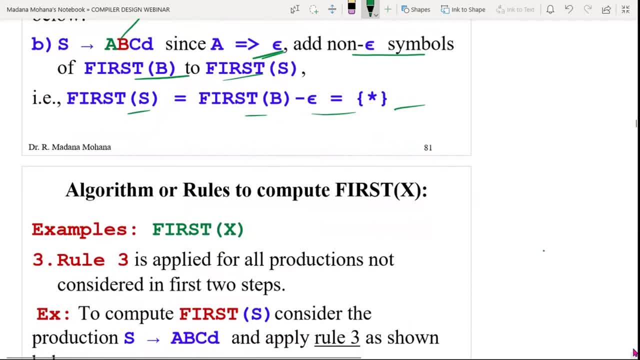 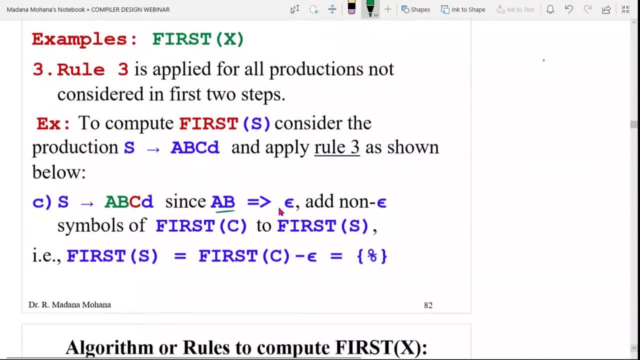 we are having null production for B. substitute B as null, then both A B are null. then we will come to the variable C. Actually this is the intention. A, B derives null. first to second derives null. null is substituted, then your starting variable is C here. so first of C, non epsilon symbols you can add to first. 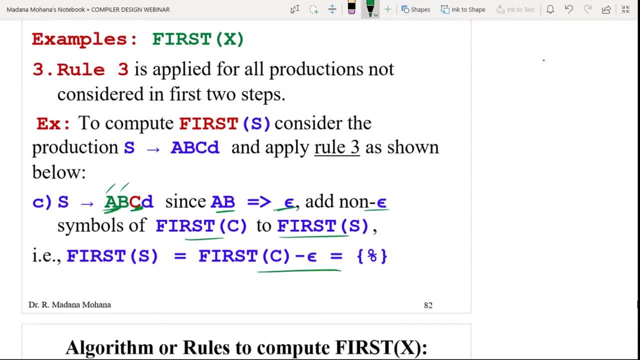 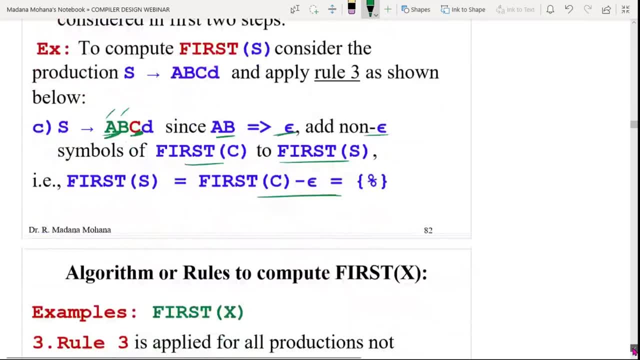 of S, now C is also derives null. that means Y 1, Y, 2, Y, 3 derives null. now, first of A, B, C means that is null. after three, null what you are having, D you are having now you can see here: A, B, C are null. 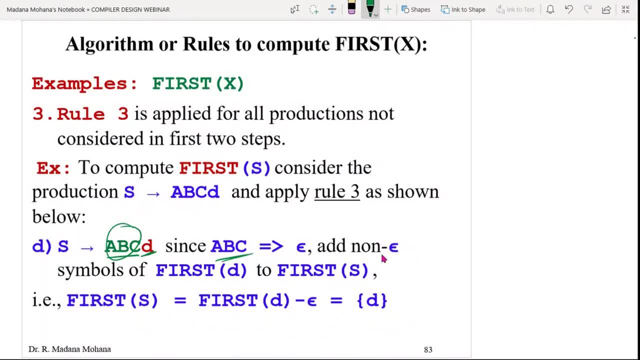 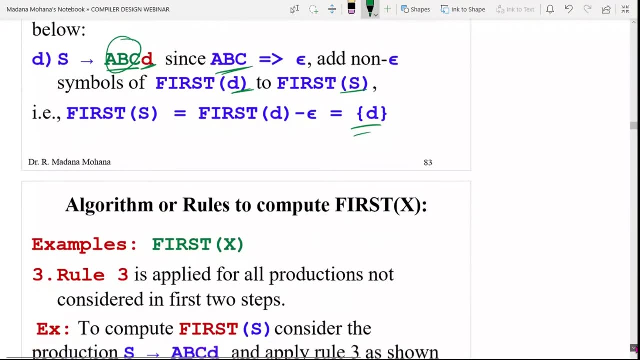 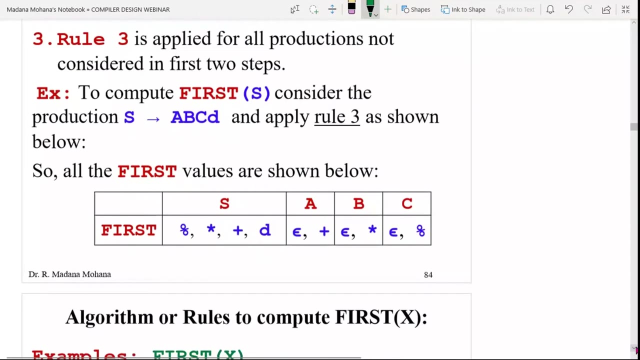 By keeping all are null, you are having terminal D, the non epsilon symbols of first of D. in a way this is direct terminal by rule one. so D is added. Now, finally, what are the first values of S? by considering all the cases plus into percentage terminal D here you can see these are all the first of S values. then coming to rule, 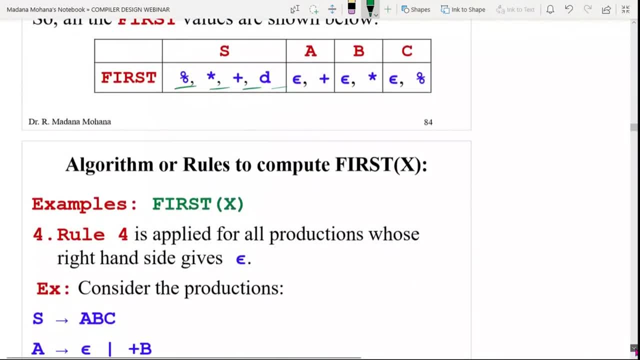 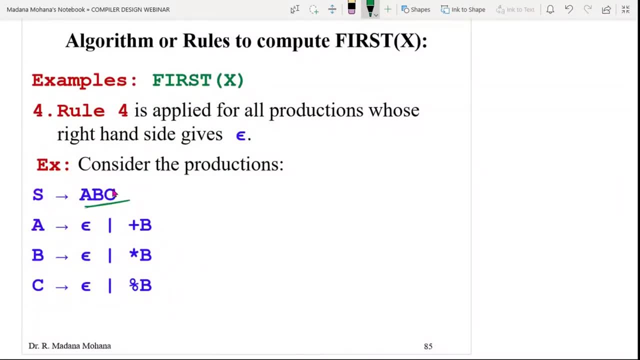 four: This is almost same right hand side: all are null. so the production consider like this: we did not consider terminal, here S derives A, B, C. the same example now: A derives null, B derives null, C derives null. here you can see same as rule three. it will come first. 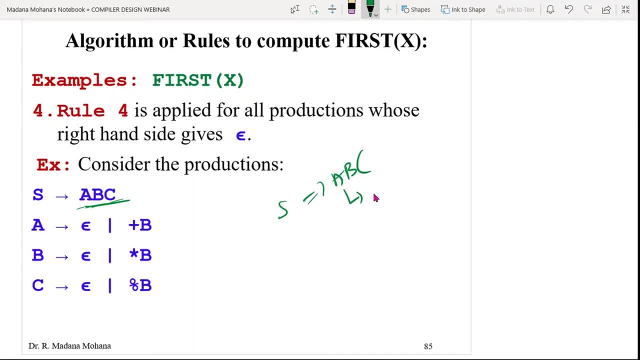 S derives A, B C from here. first of A minus epsilon will be added from here first of A. B minus epsilon is added from here. first of C minus epsilon is added by rule three. this, then rule four, is also applicable. why? because here A B C both derives null. here see A derives. 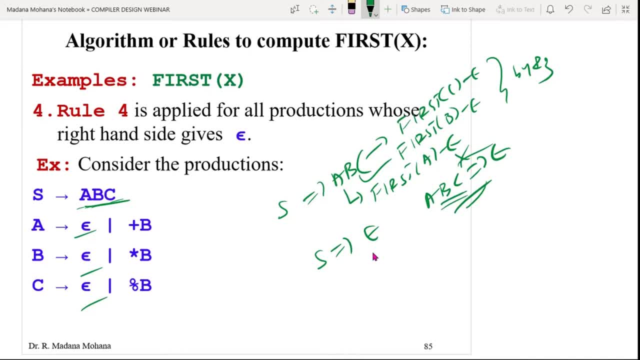 null. B derives null. C derives null. right hand side: completely null. here null means first of S equal to null. this is by rule four, Remaining are by rule three. So this is by rule four. So this is by rule four. So therefore here first of S equal to plus comma into comma, percentage comma: null also. 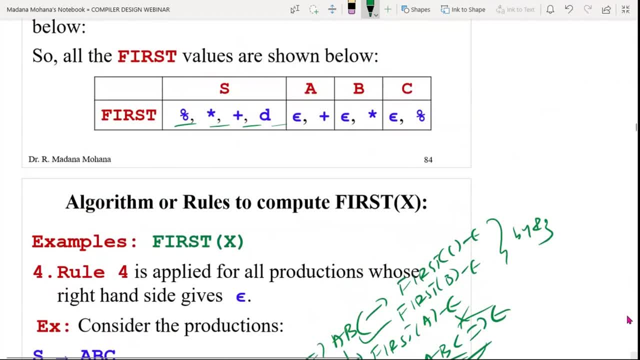 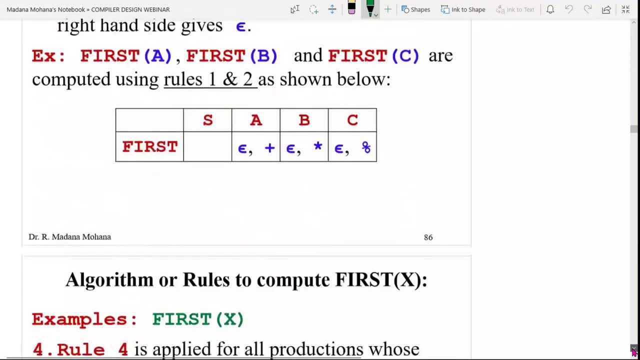 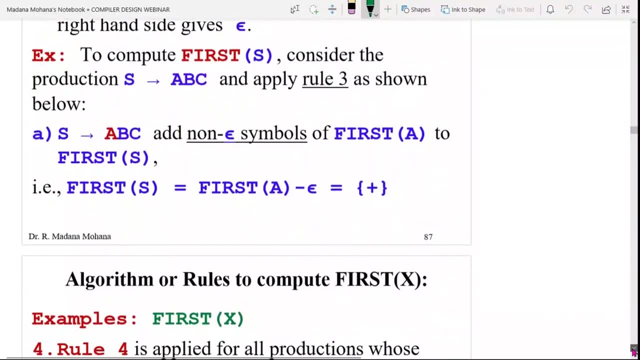 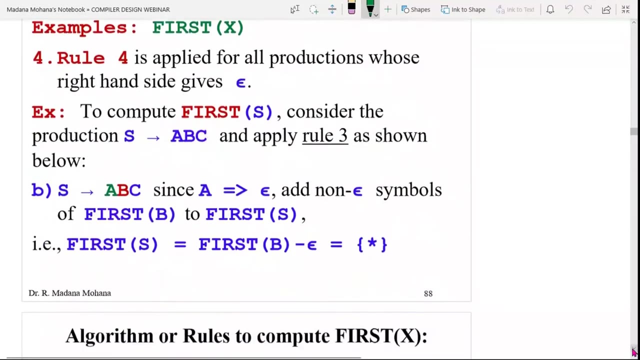 that is the only difference. right hand side. if all contains null, the same is shown here, same as rule three, only the last step. right hand side. if all are null, this is first of A. If A derives null, So non epsilon symbols of first of A is added to first of S, then here, whenever A contains 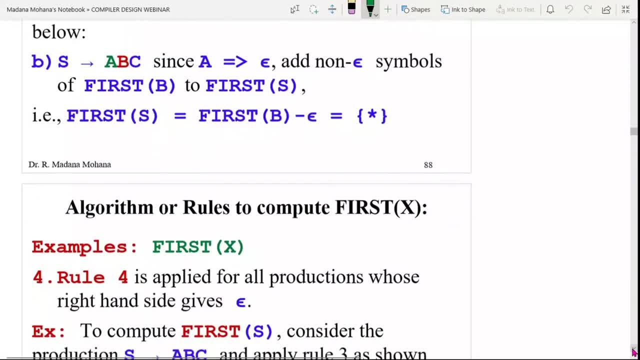 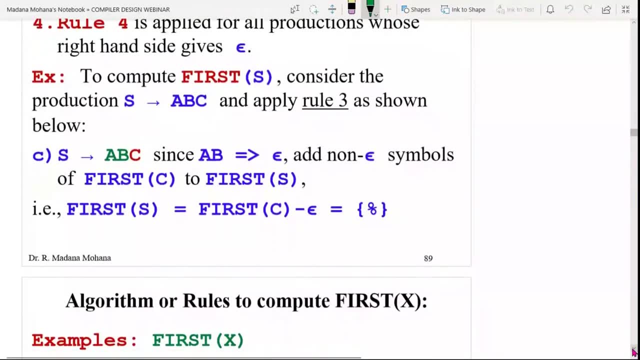 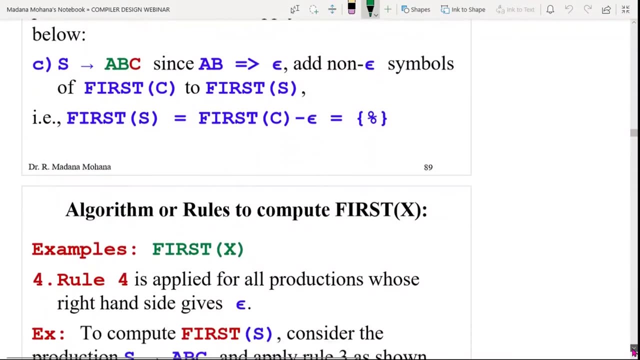 epsilon. then coming to B, non epsilon symbols of first of B added to first of S. then take two combination: A- B derives null. A- B derives null means then your next variable is C first of C, non epsilon symbols added to first of S. then next case: A, B, C derives null, all three. 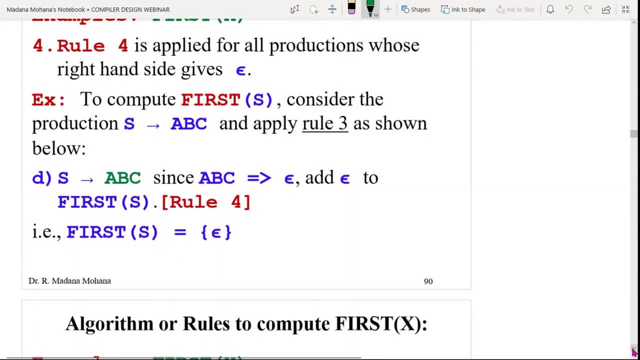 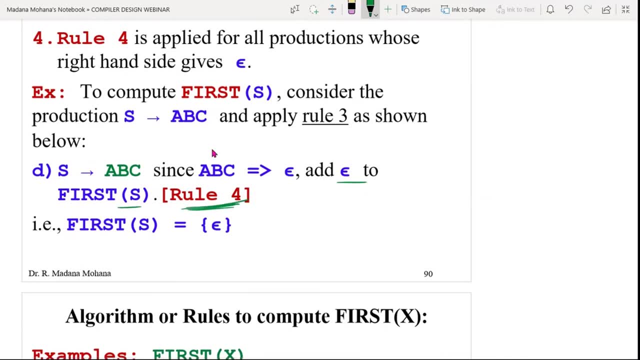 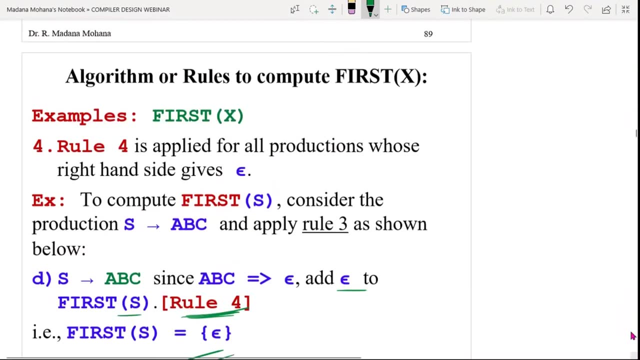 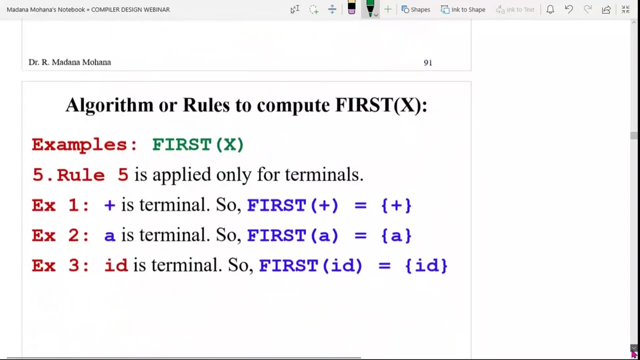 variables null, then what you are having: right hand side, only null value is there. then add epsilon to first of S. only this is the rule four. remaining all are rule three. only now, by combining all, you will get all the first values, So like that you can find out the first values. then rule four. that is direct if it is a terminal. 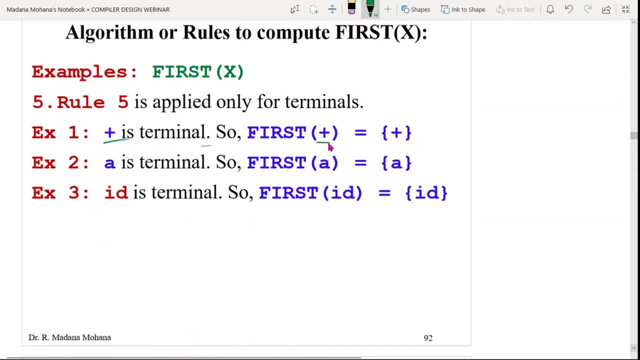 first of terminal equal to terminal, For example. first of terminal equal to terminal, For example, plus is a terminal. first of plus plus small a is a terminal. first of a equal to a. id is a terminal. first of id equal to id, direct terminal. now, this is the computation. 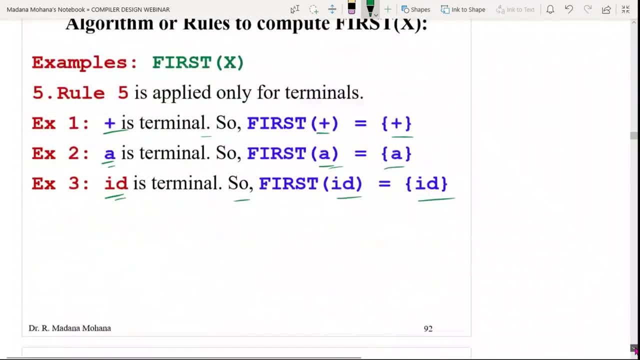 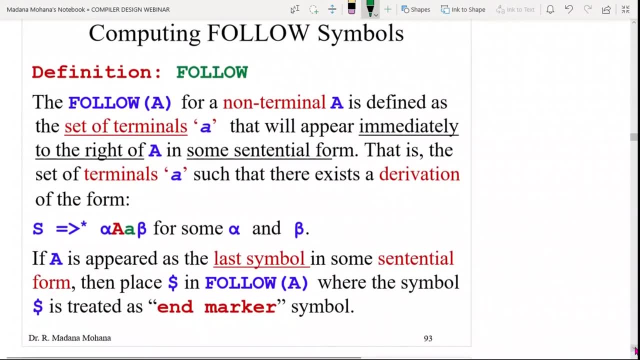 of first set values. then coming to follow the follow is somewhat difficult and you may get confusion also. So carefully you have to follow, So follow. we are having some certain rules here also. but follow value can be calculated. the variable that should be occurred in the right hand side. first value means the variable. 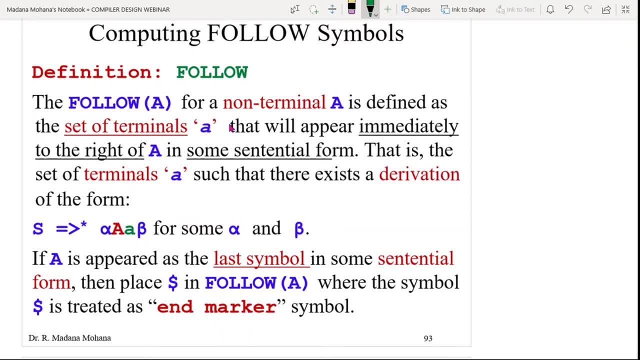 that occur in the left hand side of the production. for that variable first value is calculated but follow value is not like that in the right hand side, in the sentential form, wherever variable is there. So after the variable, whatever the values followed, but that follow value should be terminals. 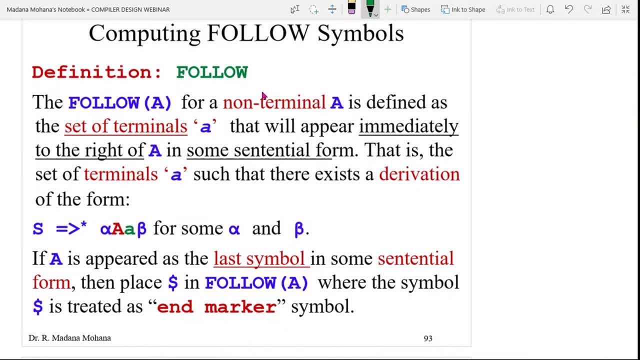 only not variable values, your first values, also only terminal values combinations. the follow of, for example, variable a: a is the non terminal or variable is different as set of terminals, small a that will appear immediately to the right of a right of the variable in some sentential form. 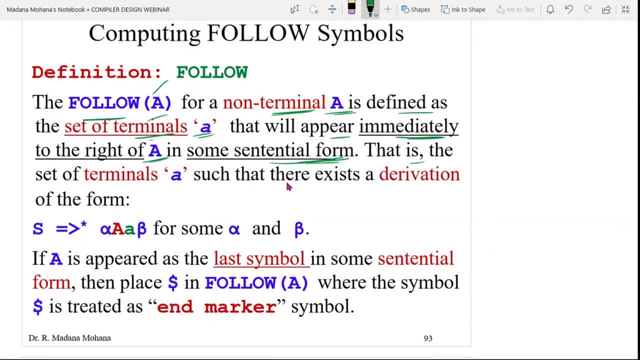 That means in the right hand side somewhere. so that is the set of terminals, a such that there exist. a derivation is of the form. this is the derivation s derives: alpha variable, a terminal, a beta. now for this we can find out: follow, follow of a equal to, after a, whatever. 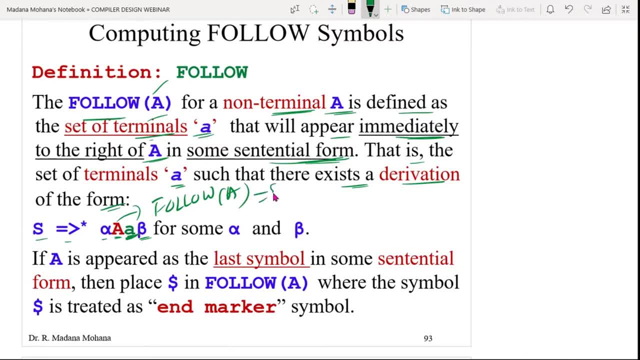 the terminal. So this is the follow value actually, but directly we cannot write. we are having some rules here. ok, now here, alpha beta, some values, any values. we are concentrating only a in the right hand side, where a is occurred after a. what is there if it is terminal or something? 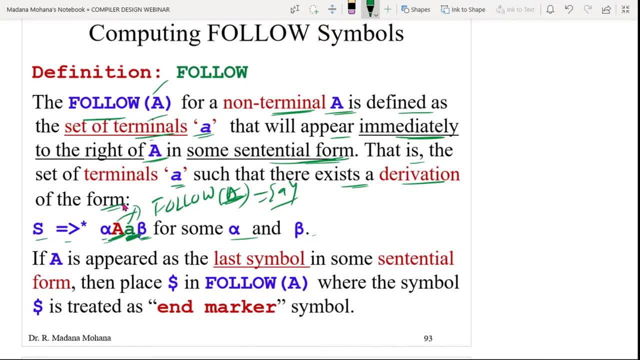 null. based on that, the follow of a, values are calculated. suppose a is occurred in the last symbol of the sentential form. that means here a is occurred right hand side after a. actually, what is there here? null, actually. So in this case dollar by default. 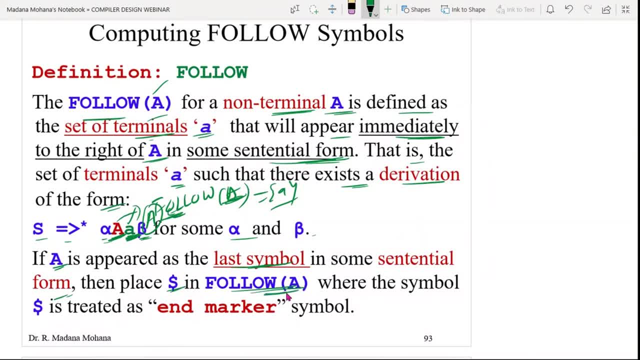 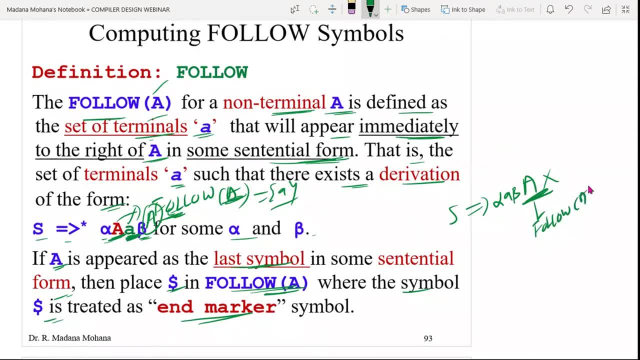 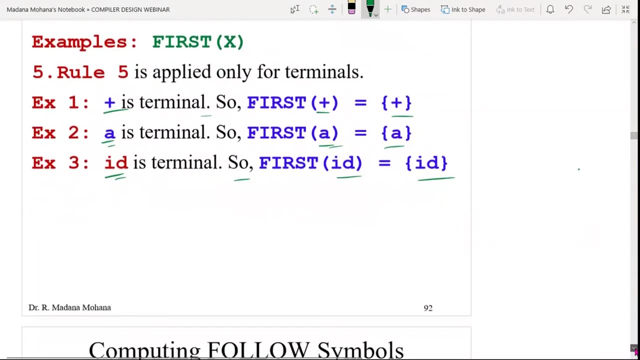 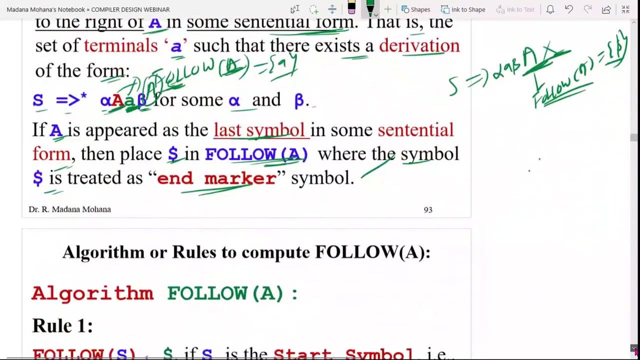 follow of a, the end marker will be added by default dollar. So this is the definition of follow value. so here, directly after follow of a variable variable, whatever the value we can't add, we are having the rules here strictly. we have to follow the rules here. so according to rule, so we can write the follow values now there. 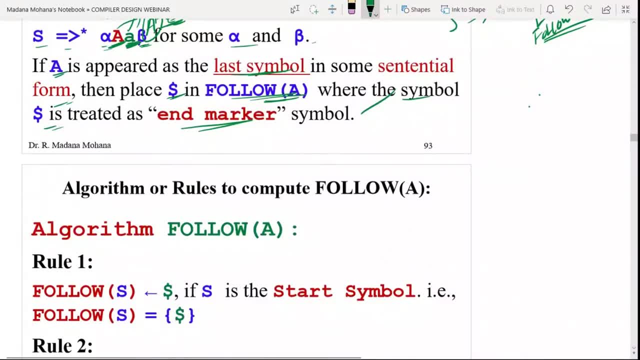 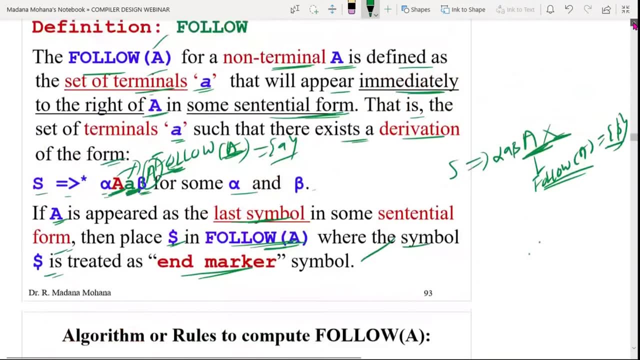 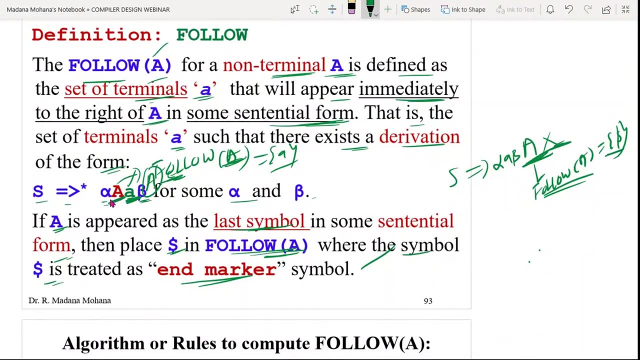 one doubt say yeah. yeah, if we take the same expression s tends to above one, sir, which you written, s tends to alpha a, beta, capital, a in that expression. if first of a means, what is the answer, sir? first of a? see here directly. you can't if there is no other productions. 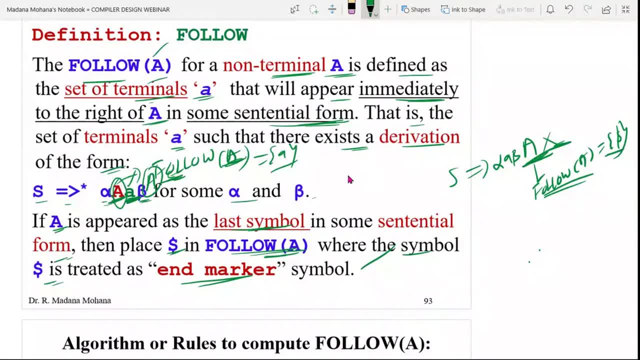 means only that is the production. then, at that case, what is the first of a? can you tell what is the production of s? there is alpha, a, a beta, same, this one, no sir, same, no, no, alpha, a beta capital, a, a yes, same production. so you want this value? yes, first of a. what is a? there is no further. 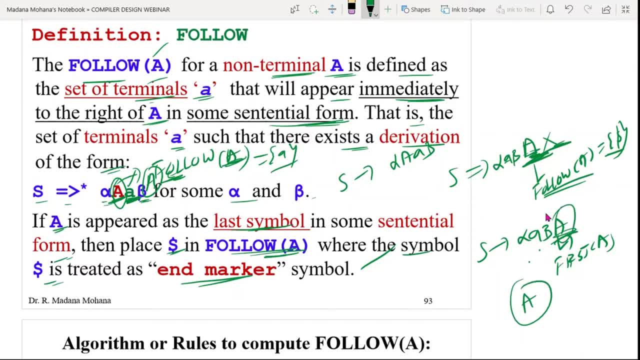 productions to a. ah, yes, then we can't find first value because no productions. if a contains something, then then from this you can find first value. okay, in this case, first of a is nothing, sir. yeah, first of a is undefined because there are- let's find these are productions for you. compulsory first value means: okay, it contains. 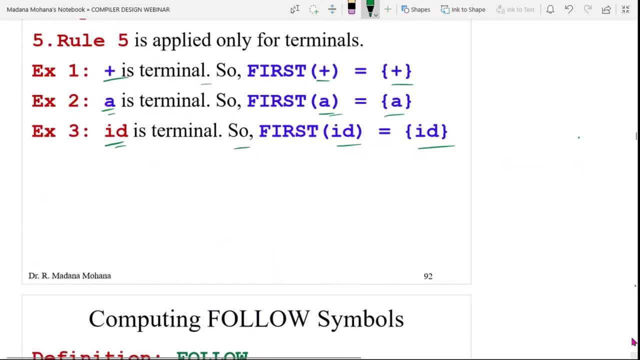 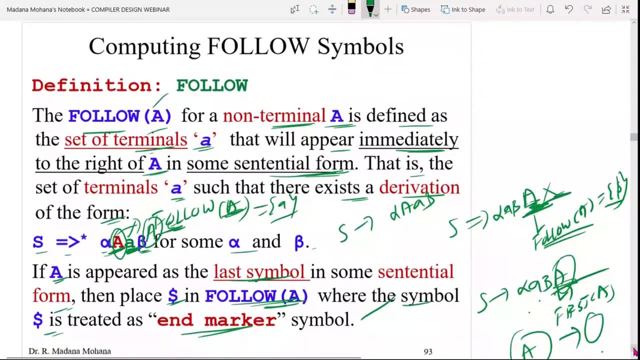 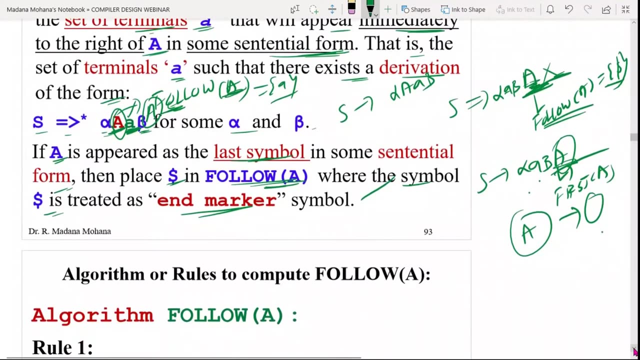 a production for that variable. based on that and you can find what follow value you can find after a nothing is there? no, in that case we can't write that sign, sir. yeah, in that undefined case we can't write epsilon as answer. no for first two. we don't have that chance. okay, sir. a contains output. why? because in the first rules anyone can do this. yes, do you find that is it may be useful, the other reasonable to do the follow up idea which is better? no, implies that it will be easier to. why is it? yeah, cumbersome. does that explain that up to? 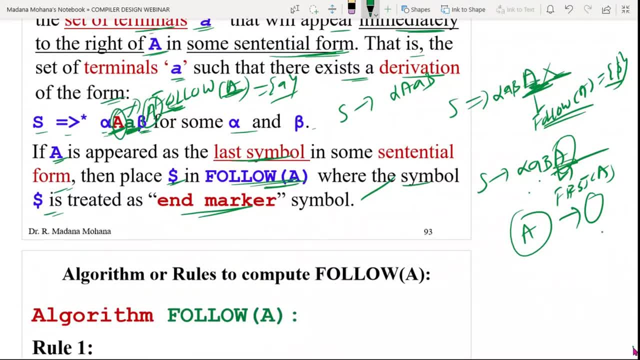 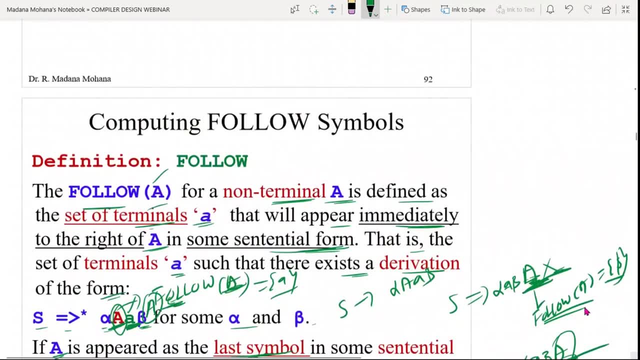 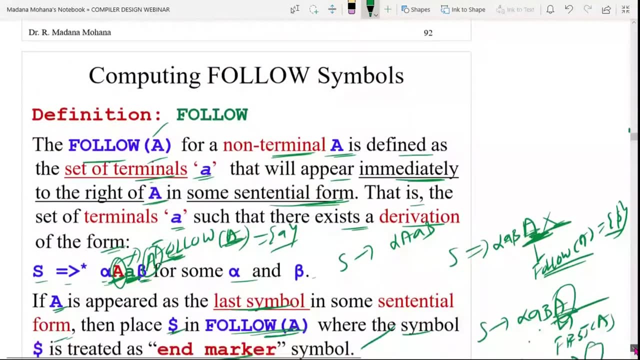 a box f soul koska, in that case it is the form l. then, first of a says: how much will p? very first rules, the five rules you can see. do you have any such case? no, sir, that's why we can't use that, but follow it is possible. now let us see the rules for follow. so these rules, 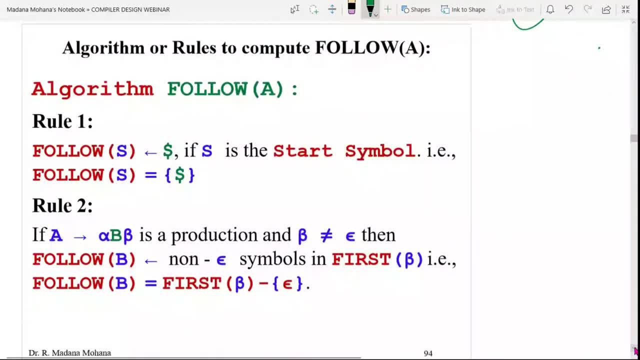 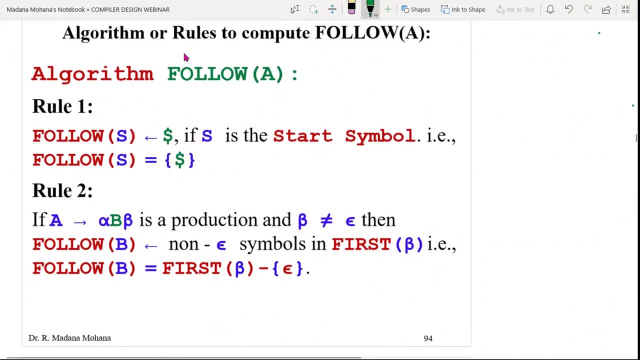 also called as algorithm for computing, follow values. so the first rule, so all of you, before doing any problem, whatever the procedure rules, we have to follow those. you have to remember and practice. then only you can start doing the problem. the first one in our given grammar, if you are. 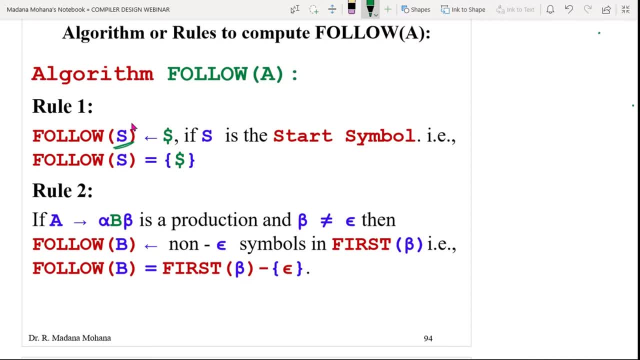 having a starting variable. let us assume s is the starting variable, s derives something. s is the start symbol. then follow of s equal to dollar is added by default rule rule one. suppose in our grammar e derives e plus t or t, t derives t into f or something. here e the first production, s equal to e. here. 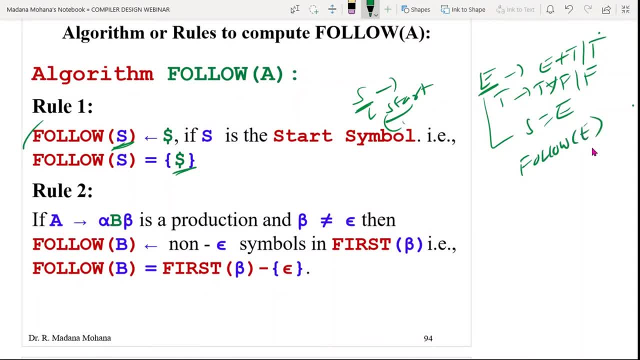 then follow of e equal to dollar. default. this value will be added according to rule one: follow of s equal to dollar. if s is the start symbol, that is, follow of s equal to dollar. then the second rule: if the production is of the form a, derives alpha, a, variable b. beta is a production beta not equal to null. beta contains something. so then you. 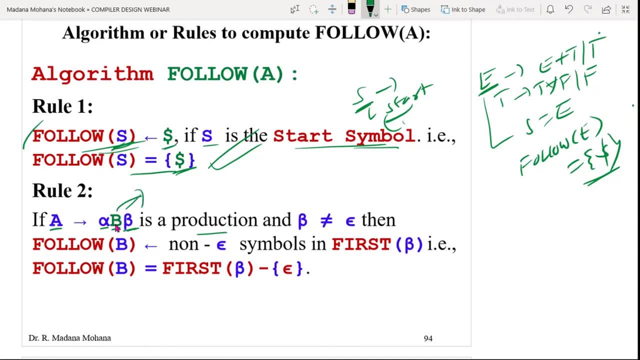 need to find out follow of b. so follow values is not like first value. first value you can find only for left hand side variables using the right hand side production, but follow value directly. we can't find left hand side variables in the right hand side. wherever the variable after the variable. 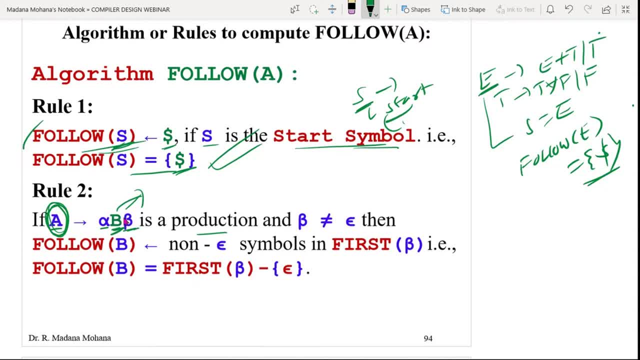 whatever the value. based on that, we can't find the left hand side variable. in the right hand side we can find follow of b like this: now the production is of the form a derives alpha variable b beta. now you need to find out follow of B here. how to find your beta is not null. the 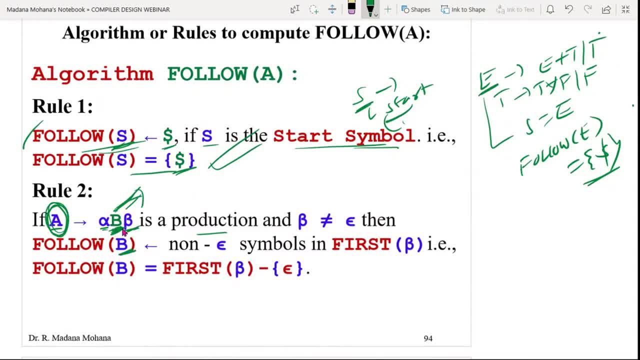 rule is your fall of b equal to this: 1 non epsilon symbol soft for stop beta, non epsilon symbols in first of beta, that is for stop beta minus, For example here for stop beta equal a plus comma epsilon. let us assume then non epsilon symbols means only plus will be added. 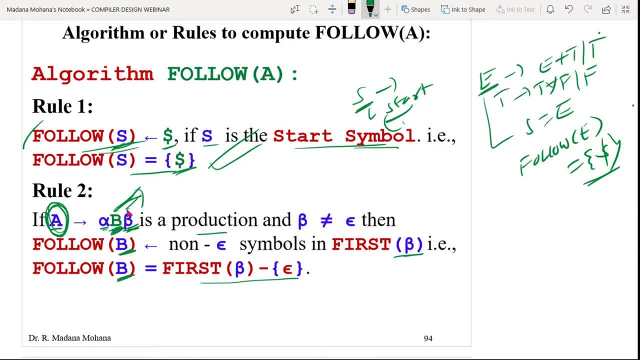 to the fall of b like this. so here beta equal to not null beta. something should be there at that time. fall of b equal to first of beta minus null. this is rule two. this is the in anyway. in examples we will see clearly. so that is rule two. fall of b can be five if 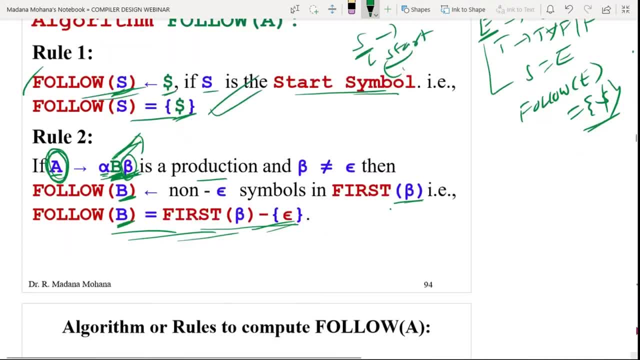 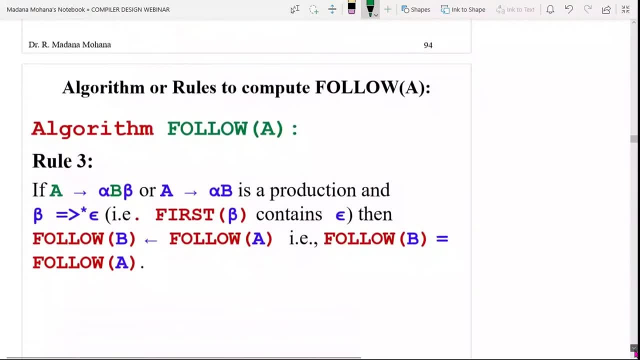 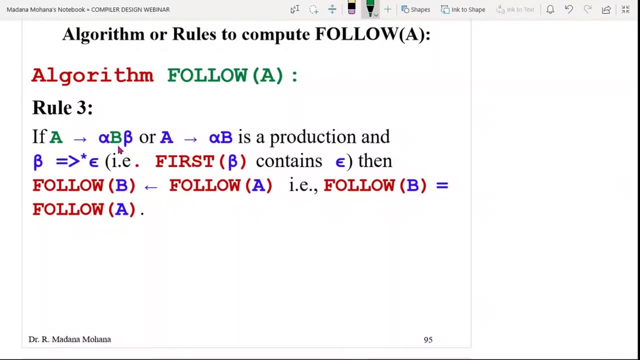 beta equal to null. what will happen? there is a next rule. let us see then rule three in follow. we are having only three rules. no problem, very simple. rule three, almost similar to second rule, but beta contains null. so the productions are of the form alpha. a derives. 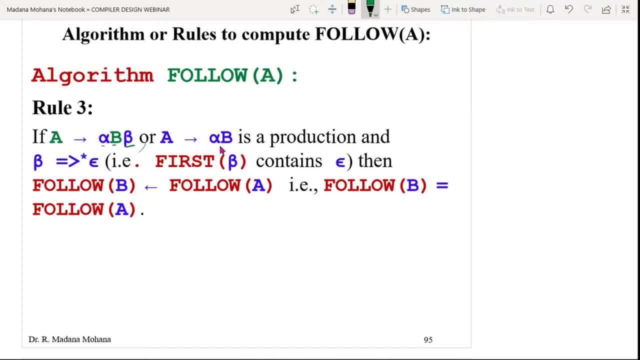 alpha b, beta, or if beta equal to null means only alpha b is a production. here beta derives null first of beta contains epsilon. then what you have to do here actually fall of b. we need to find out. fall of b. what was the fall of b value? same values for fall of a. 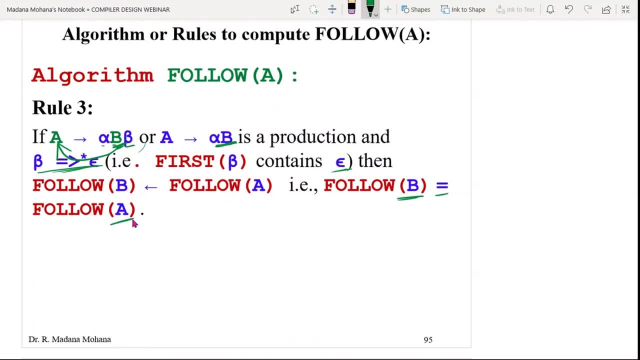 also, therefore fall of b equal to fall of u. suppose earlier you already calculated somewhere in fall of a, then fall of b, the same a values you can substitute here follow by b equal to fall of u. So, following rule three, what you will do already, existing fall of values will be useful. 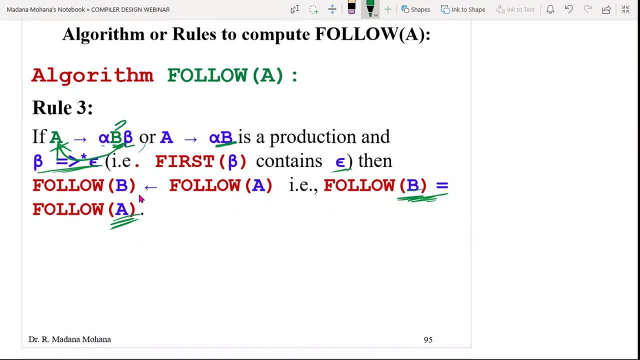 for the current variable fall of value, whereas rule two you will get after variable, whatever the values. if that value is not null, non epsilon values, the terminal values will be added there in rule two. like that rule two, rule three you can apply for all productions by considering: 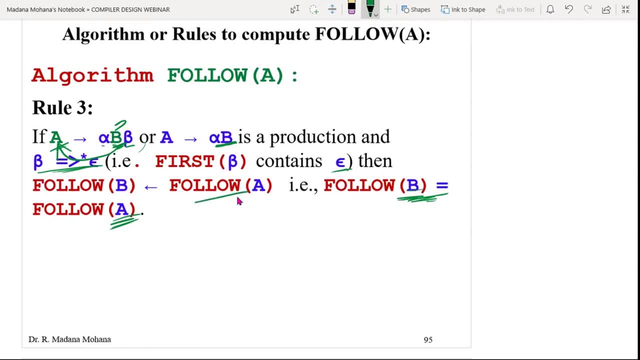 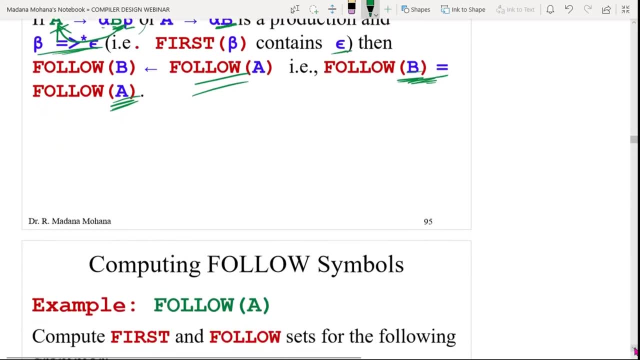 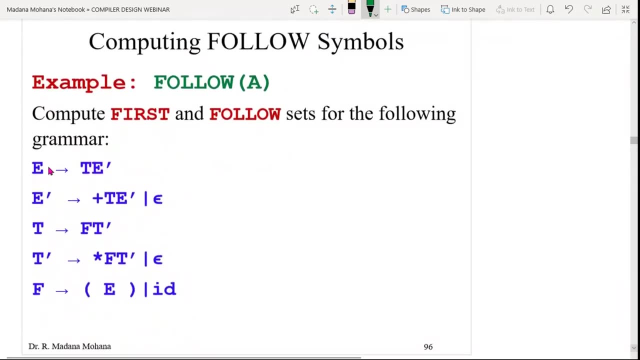 beta not null, And beta null, the two cases. now you can see some examples on this, then you will get more clarity. now the same problem. let us consider. this is the problem: e derives t dash. e dash dash plus t dash are null. t derives f t dash. t dash dash star. f t dash are null. f derives. 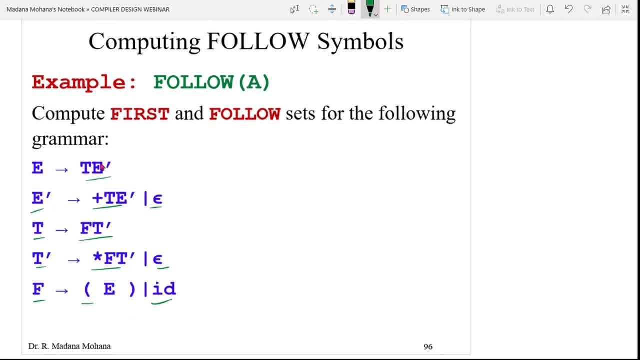 e within parenthesis, already for the same problem. first values we already calculated, So now For follow compulsory first values required. why? because in the follow rules first values also used. Okay, now, as usual, you can write down first values first, then apply the follow rules. 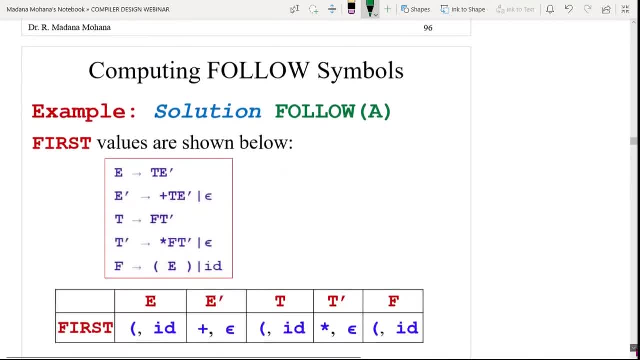 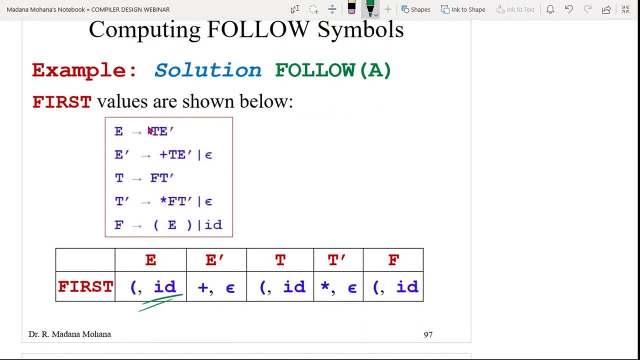 Now let us see the first values directly. I have taken why? because previously we already did the same example: first of e, equal to actually first of t. what is first of t first of f? what is first of f? First of t equal to first of f, first of f. we already calculated left parenthesis, id. then 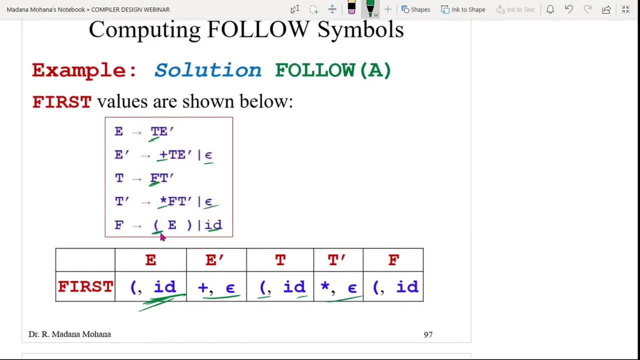 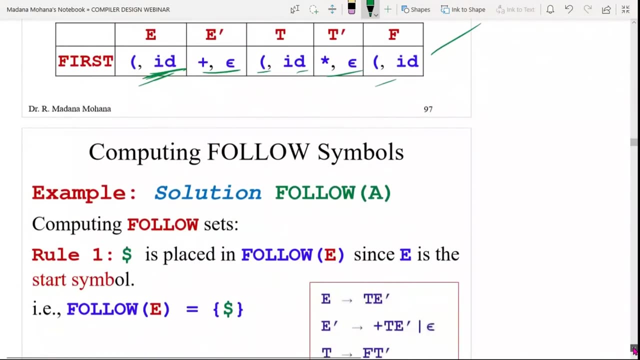 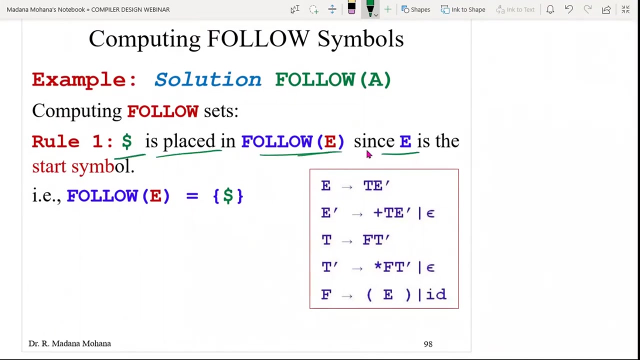 first of t, dash star comma null. then first of f, left parenthesis comma id. these values directly written in the previous we already did. now coming to the follow values: In follow value, rule one for starting variable: follow of the starting variable equal to dollar. Here you can see rule one: dollar is placed in follow of e, since e is the starting variable. 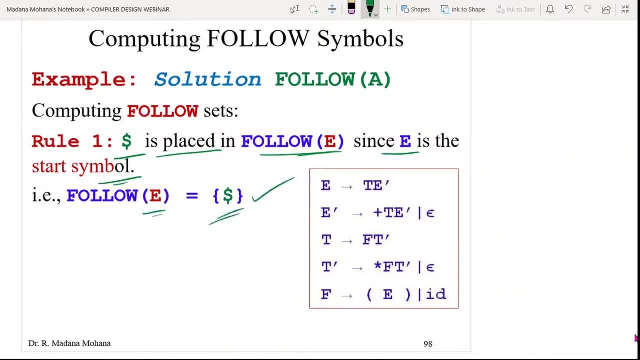 therefore follow of e equal to dollar. So then you can apply rule two and rule three for the variables wherever right hand side variables are there for t dash, here also t dash f, t dash, f, t dash, e. so for all these, both rule two and rule two, you can apply whichever applicable. 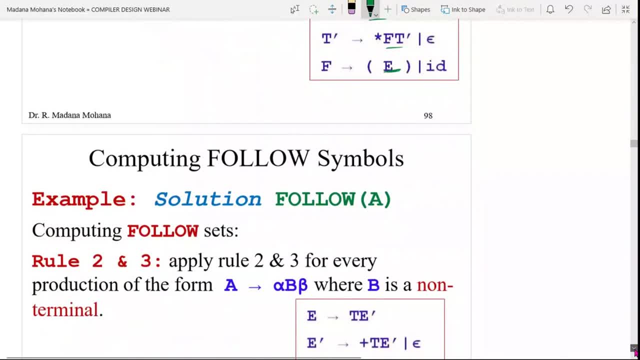 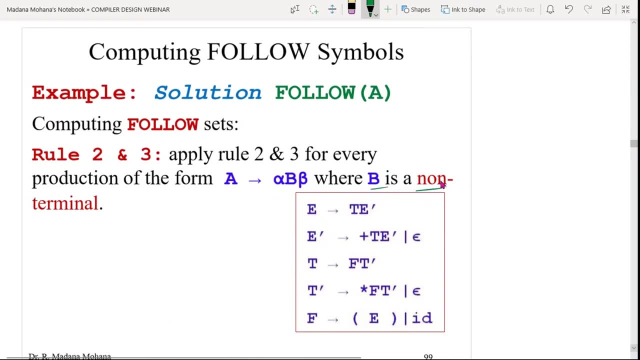 Then coming to rule two, So rule two and three apply for every production of the form a derives alpha, b, beta where b is non terminal. So rule two: you can apply whenever beta e is not null. then rule two, rule three, you can apply whenever beta e is null. 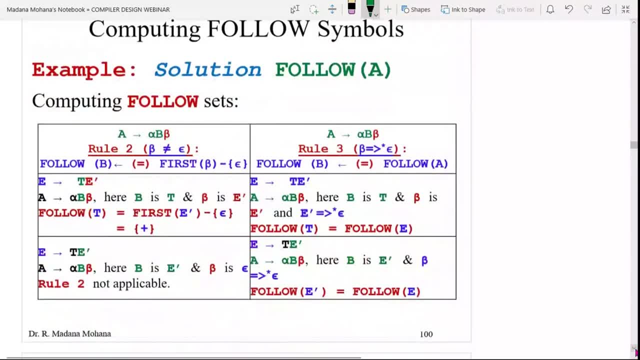 Now you can see in the tabular format all I have listed at one place carefully. you can observe Here rule two in first column, rule three in second column. so rule two is the general format. a derives alpha b, beta, beta not equal to null, whereas rule three alpha b, beta, beta, direct. 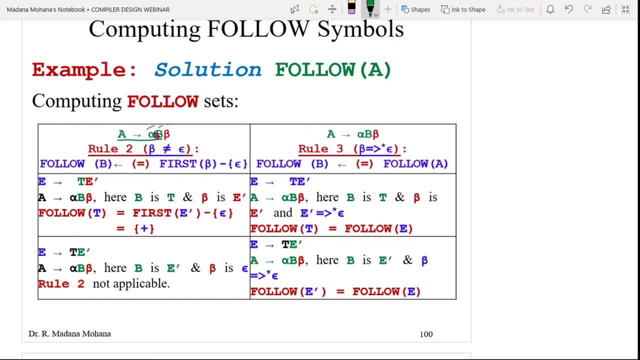 beta null or beta derives null. So in rule two case here follow of b equal to first of beta minus null. in rule three case, follow of b equal to follow a. now you can see: take all the productions, the same production, apply rule two, rule three also. so then you can see: first a derives t e dash. 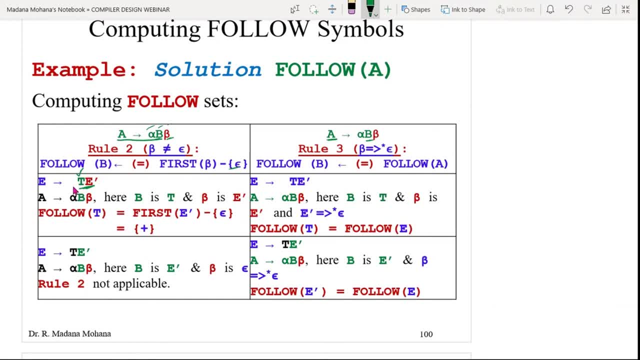 now you are finding all of t here. why? because it is in the form of alpha, b, beta. here, alpha is null. ok, now b equal to t, now beta equal to e dash now. now beta, not null. it is a variable, e dash. it is a, not null. then here, b is t, beta is e dash. now, as per rule two, what you have, 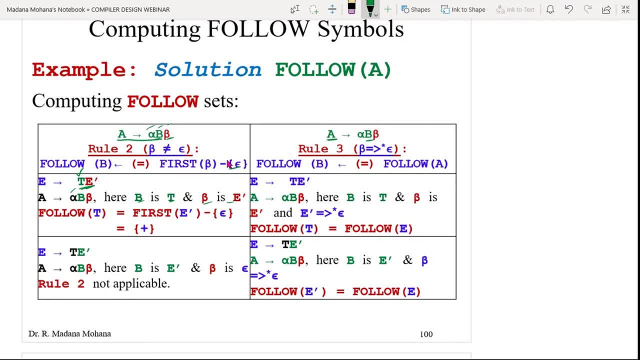 to do. First of e dash minus null will be added to all of b. their fall of be mean. therefore, fall of t equal to first of e dash minus null. What is first of e dash actually we are having in the table we already listed, first of t equal to plus comma null, so excluding null. 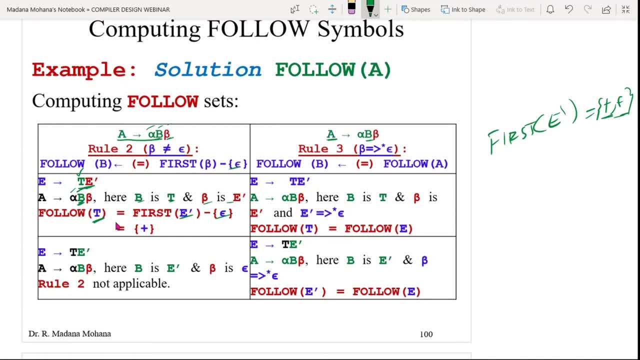 what is first of it as place. plus is added to all of e. therefore all of t equal to first of e. dash minus null, e is added. Ok, the same. you can apply for rule 3 here again: alpha, null, alpha, whatever, even null, also you. 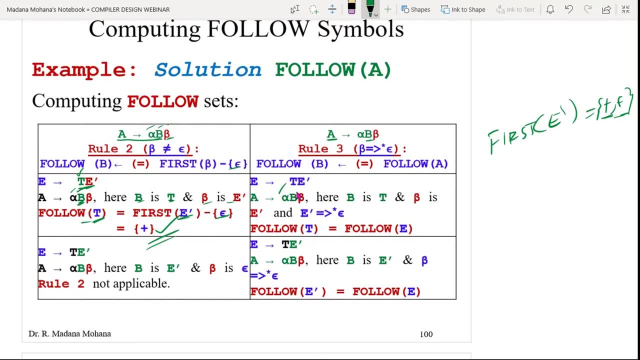 can consider our concentration. is b beta always. we can consider b beta. rule 2 beta is not null. rule 3 beta is null. now alpha b beta. b is t, now e dash. that is the beta. ok, now here beta derives null. why? because we are having the production. e dash derives null. 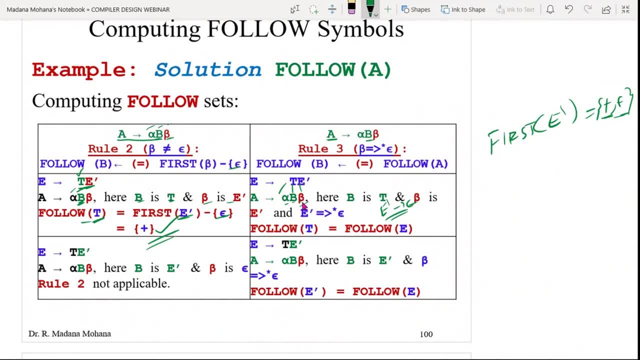 so, whenever you can substitute this, what you will get: beta is null here. now you will get only b after b. nothing is there. then what the rule we have written? fall of t equal to fall of e. as per this, fall of b equal to fall of e. therefore, fall of t equal to fall of. 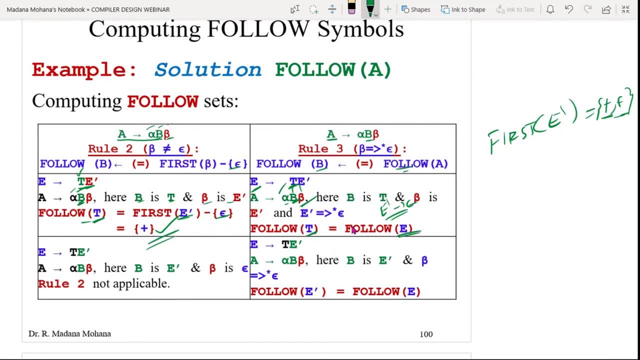 e, but initially we do not know fall of e. keep this relation. later, once we obtain fall of e, then automatically t will come like that, then coming to the same, in second case, that follow of t equal to follow of e. dash, no, sir, there, no, no, no, not this one. 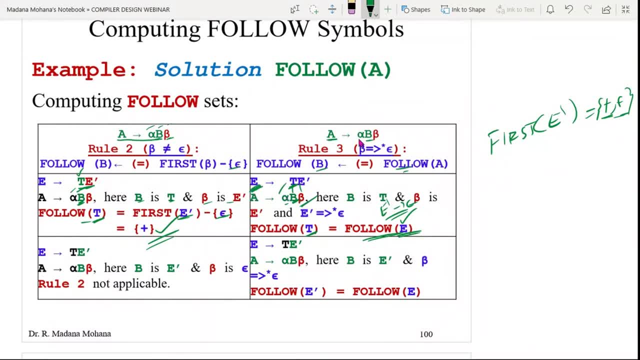 left hand side. here rule you can see: a derives alpha, b, beta. if beta e is null, fall of b equal to fall of a, this one. why? because if beta is null, nothing is there now after b. then we are depending on the fall of a values. that is the rule. the rule as it is i have written. 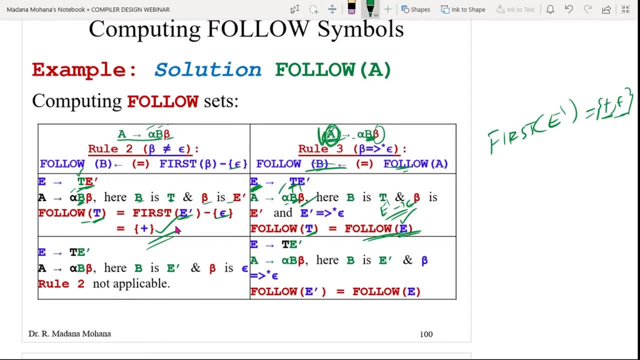 let us see this one. we are following simply the rule. then coming to suppose, now you can change the alpha, beta, alpha b beta values, let us check what will happen. suppose you derives t e dash. now i assumed alpha as a tb as e dash. now beta is null here. beta is null means rule two is not. 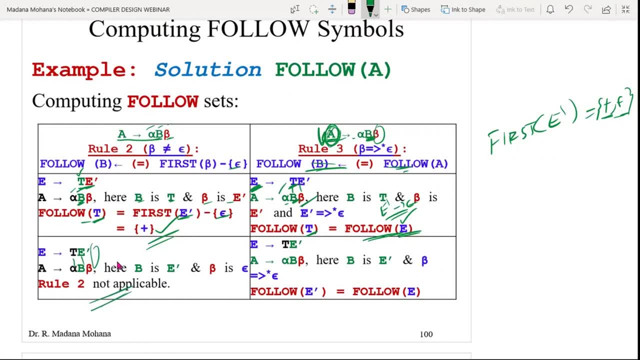 applicable. beta not equal to null, only rule two is applicable. then say we can apply for rule three: is e dash, beta is null. now, ok, now here. as per this rule, fall of e dash equal to fall of e vr. all this relations further useful after calculating other fall of values using 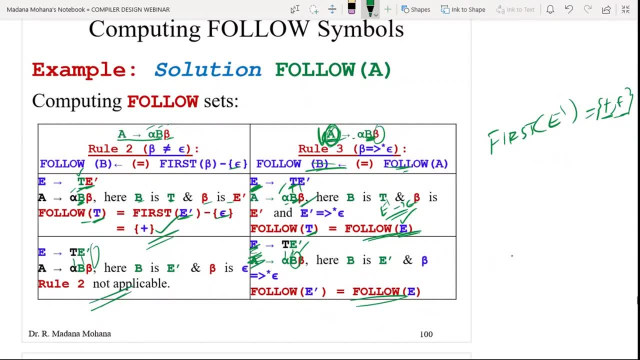 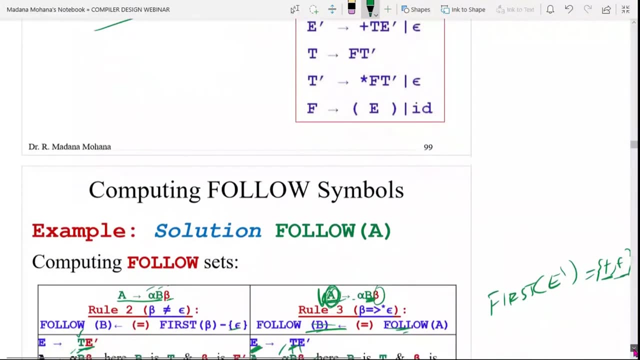 rule two. ok, now that is for e dash, t dash production only. till now we applied two times. so rule two or two times, or rule three: two times we apply by changing alpha beta values. then, coming to next production, let us see what will happen. so first you can write down. 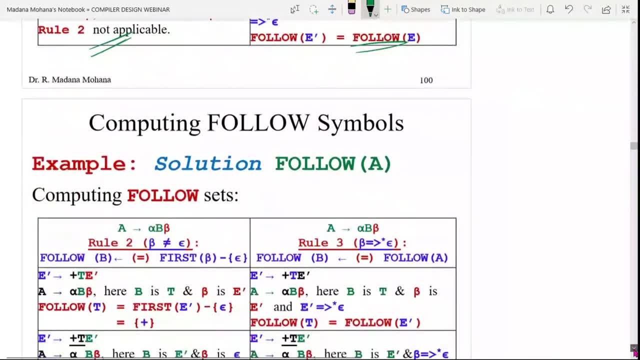 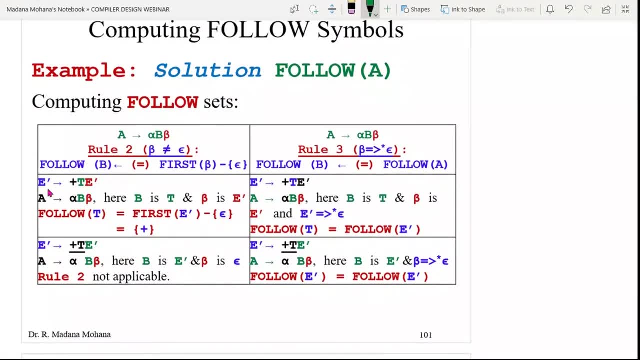 the rule and you can substitute the values. then you would not get any confusion. as per the rules, then next to production: e dash, dh plus t dash we have taken now apply rule two for this. now alpha is plus b is total. So e dash, d dash is null. 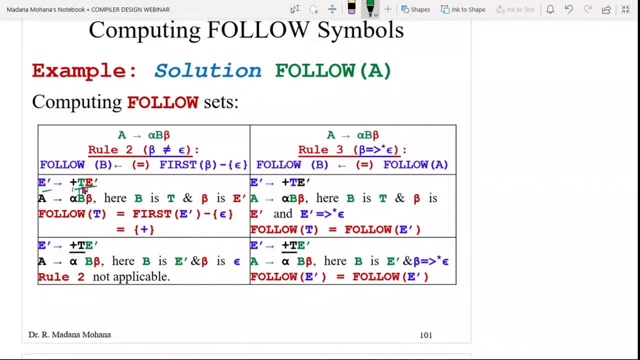 t beta is e dash beta, not null. why? because e dash is variable, is there? so now your fall of t equal to first of e dash minus null. so your fall of t you will get plus here then same. you can apply for rule three. then what you will get here: e dash derives null. then 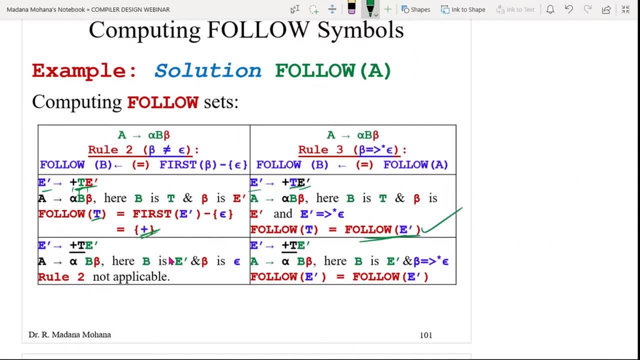 fall of t equal to fall of e dash. one relation you will get similarly for same production. apply rule two by changing alpha value. suppose plus t as alpha b as e dash, beta is null. beta null means not applicable. now same you can apply here. now. fall of e dash, after e dash. 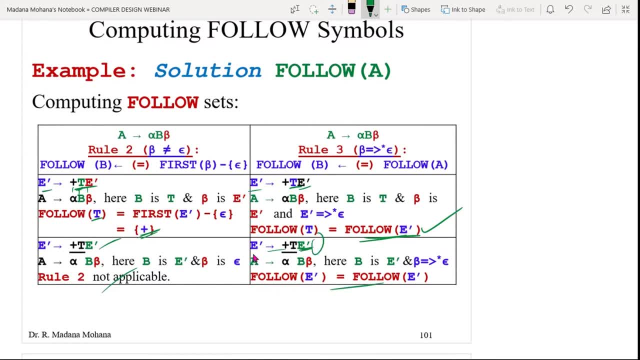 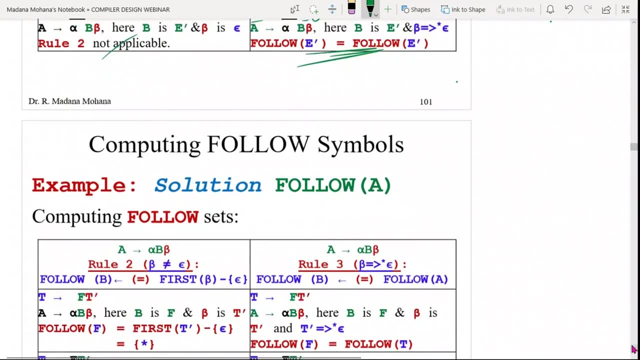 null. is there fall of e dash here? no meaning why? because e dash, e dash, same. you are getting ok like that. sometimes you there may be chance of having some values. if you can apply e dash, rule two, rule three, for all possibilities, then we wont miss the values actually. then 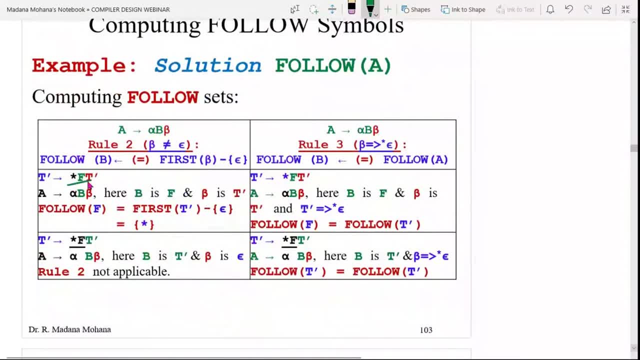 coming to t dash production: t dash derives star f. t dash, fall of f equal to first of t dash minus null. here you will get star same. you can apply rule three: t dash derives null, then fall of f equal to fall of t dash. then for this, by changing alpha values, rule two: 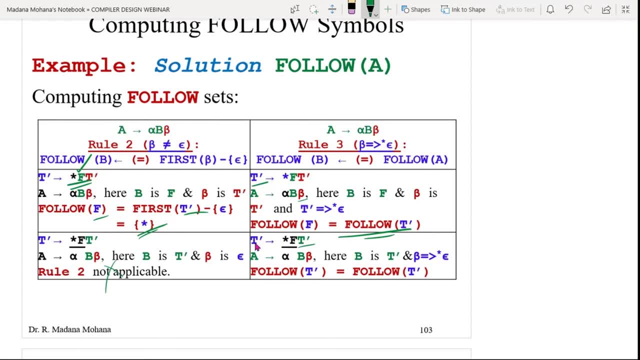 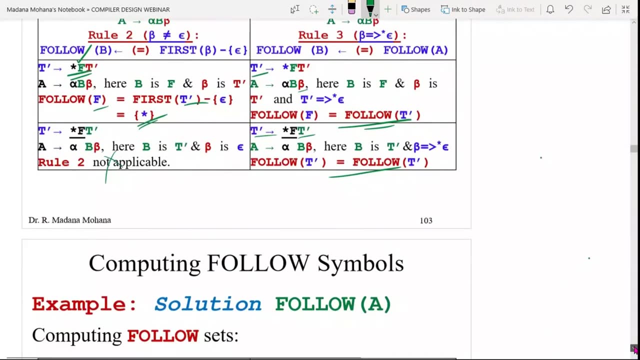 not applicable, then here also, by changing alpha value, here also same value. you are getting now. finally, you can combine all the values. whatever the fall of values, you will get all fall of e, all fall of f, all fall of t. you can combine then the last production, f derives e within. 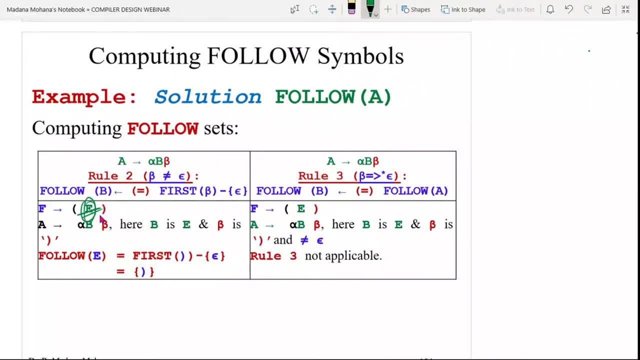 parentheses. now e this fall of values. you need to find out. beta, not null, first of beta, first of right parentheses. first of terminal t, first of right parentheses, first of right parentheses. you will get- and here you can apply rule three for this. here rule three is not applicable actually, here beta is not null, it is a terminal. now e value. 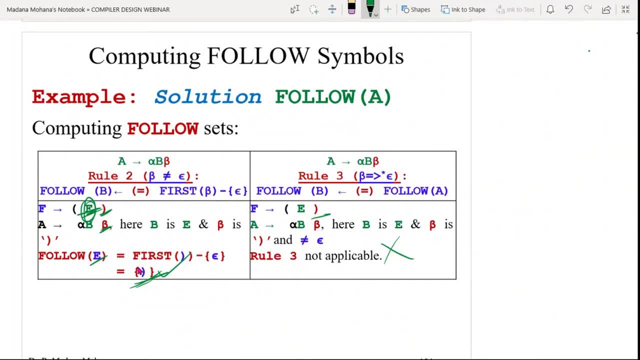 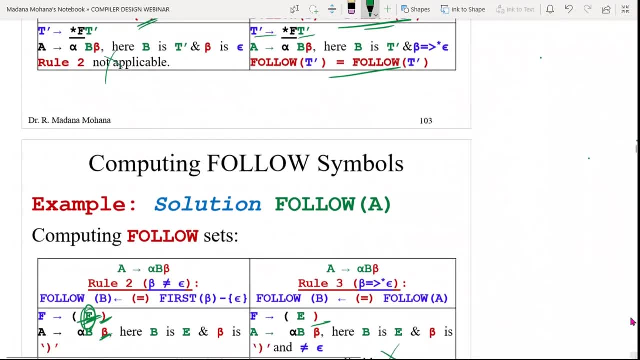 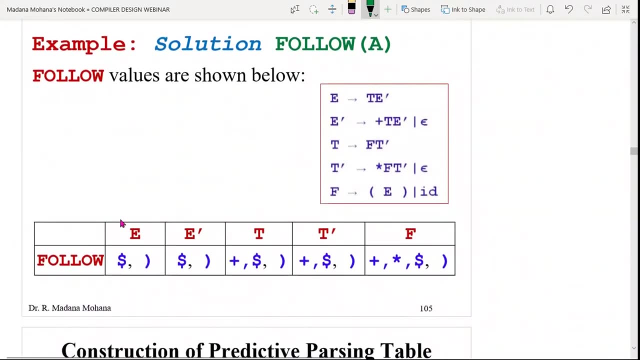 previously we got one value here. we got one value and we got dollar also. now all combined fall of e values. once you know fall of e value, then according to rule three we got some e values, also equivalence values. now you can see fall of e by default dollar we got. then write parentheses: 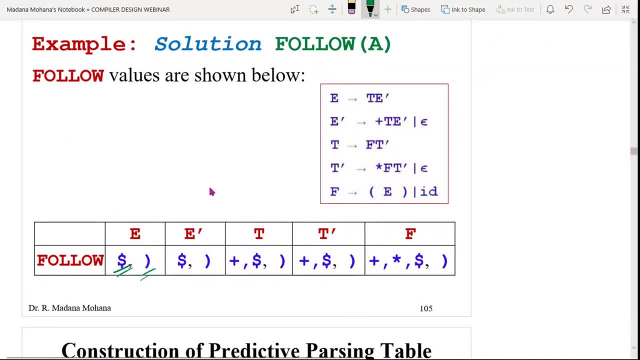 so then we are having the relation fall of e equal to fall of e dash, so this one. then fall of t. we got one value, then fall of t equal to. we are having fall of e relation, then dollar. write parentheses also: added plus is direct value. we got then e value also. 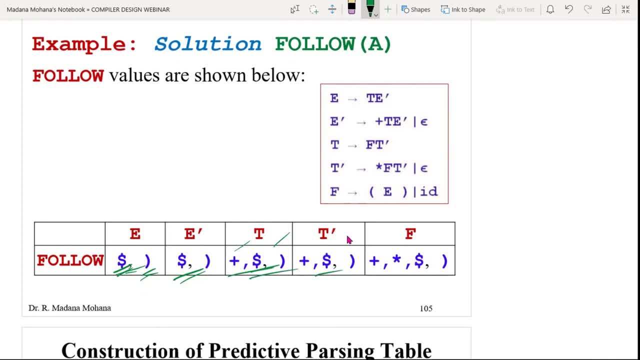 then fall of t dash equal to fall of t as per the rule three relation we are writing. then fall of f: here what we got previously, we got some star value. then fall of f equal to fall of t or t dash is there earlier. so all values are added like this: 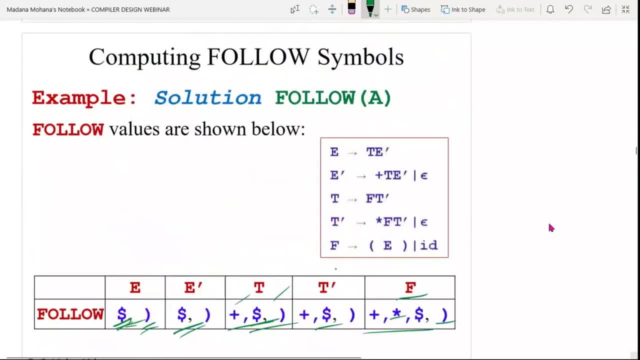 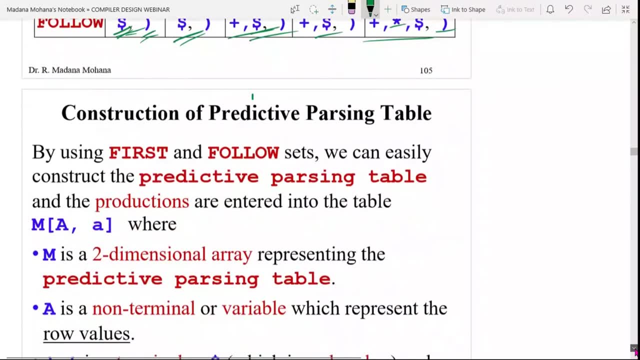 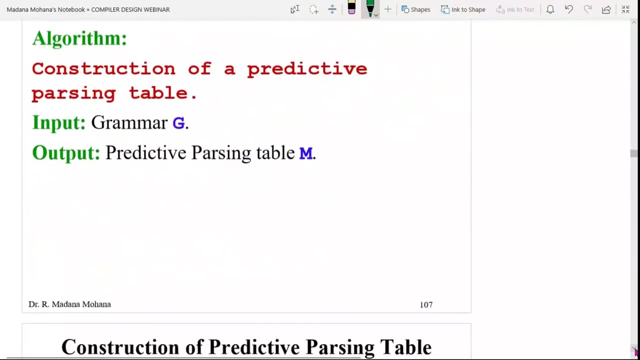 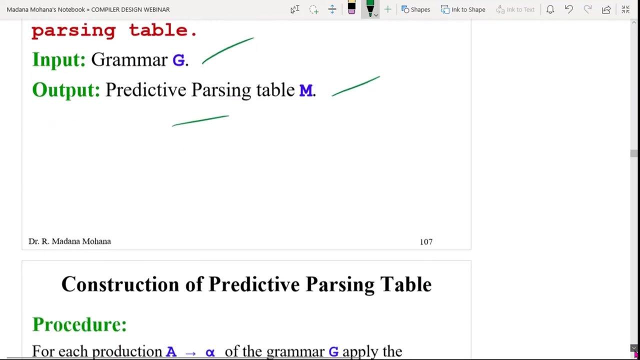 You can go back and check all these values. ok, now, once you know the first and follow values, then you can construct the predictive parsing table easily. we are having one algorithm, the predictive parsing table. we already discussed in the model coming to the algorithm. so for this input is grammar, the output is predictive parsing table. what is the procedure? the rule. 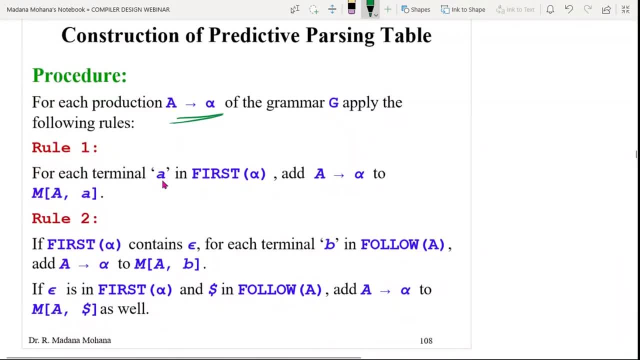 for each production is of the form: a derives alpha for each terminal in first of alpha for each terminal in first of alpha, first of right hand side, whatever the terminal value in the table a on this terminal at this production. see, the table is like this: this is terminal. 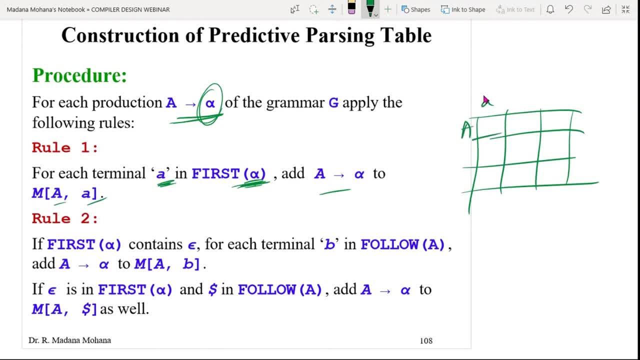 a. this is variable a. now you are finding first of a, actually having this terminal right hand side. This is the production: a derives alpha. first of alpha contains a terminal a, then the entry: a on terminal a, a on terminal a at this production, a derives alpha. in the table, the entries are: 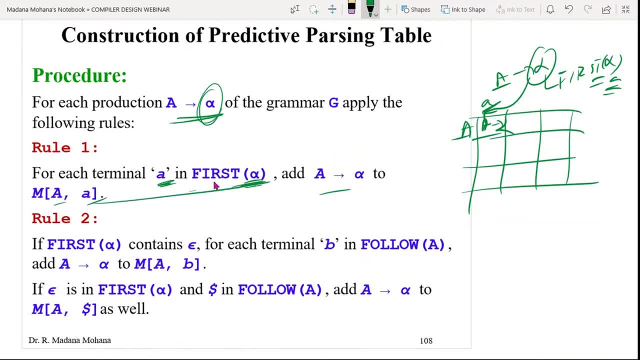 productions are blank entries. that is rule one for all terminals. you can apply rule one, then rule two: first of alpha contains epsilon. the right hand side, first value contains epsilon. then for each terminal b- what is b here? fall of a left hand side, follow value. so now you can find out fall of a fall. 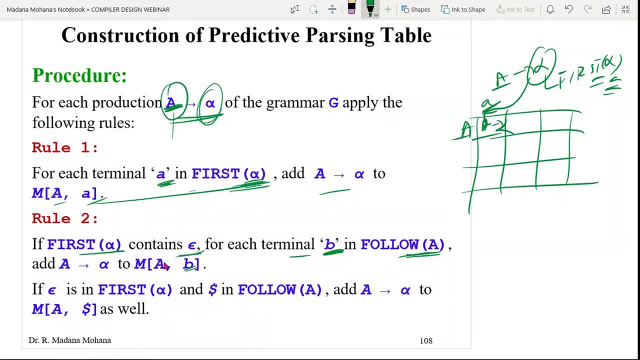 of a equal to, let us assume, b, then the entry a on b. you can add this production. if epsilon is in first of alpha, dollar is in fall of a, then in this case a derives. alpha is added to the entry m of a comma dollar in the table you can add dollar also dollar, also one dollar. 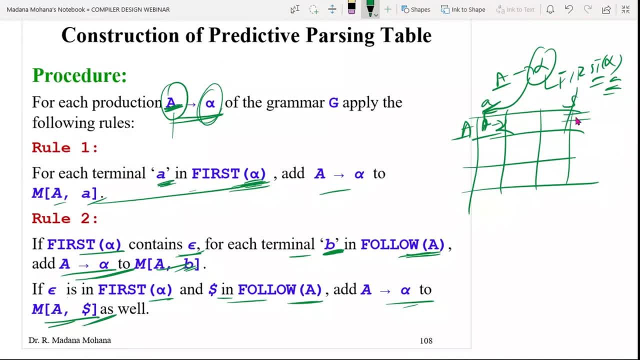 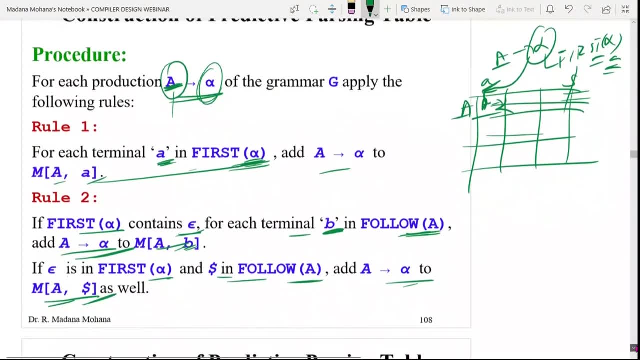 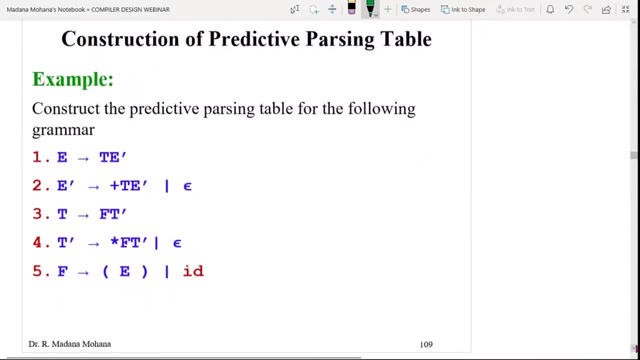 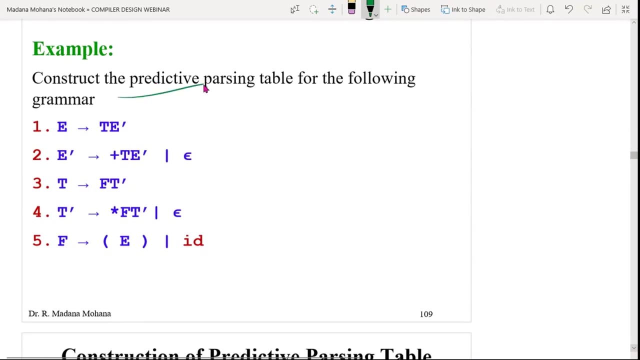 also one dollar. So this is the production, But this is the entry. there is rule two. Now let us see. or the same problem. only two rules we are having. one is the direct terminal, second case: none. So the question you will get examination like this is one important standard problem. 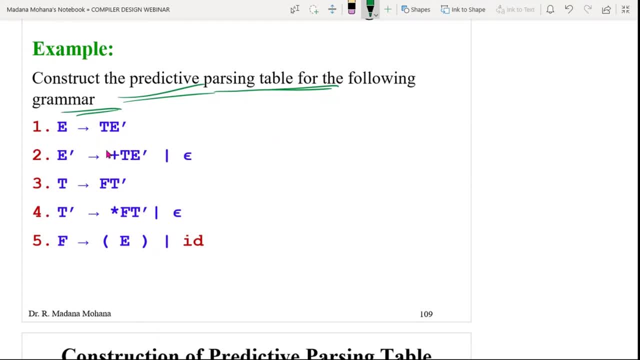 construct the predictive parsing table for the following grammar: t derives t dash, v dash derives k dash, t dash as plus t dash, so on. so see directly: sometimes they will use the grammar with left recursion. if any grammar having left recursion ambiguity, we cannot apply predictive parser. the difficulties: 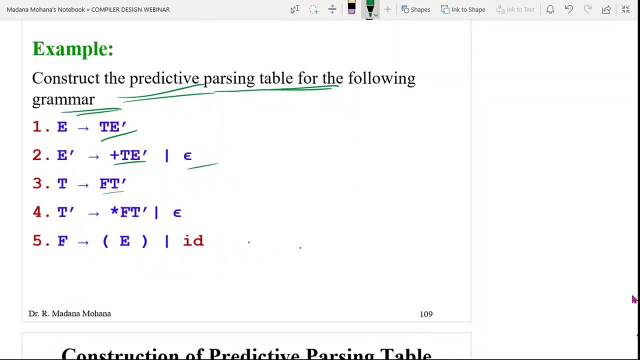 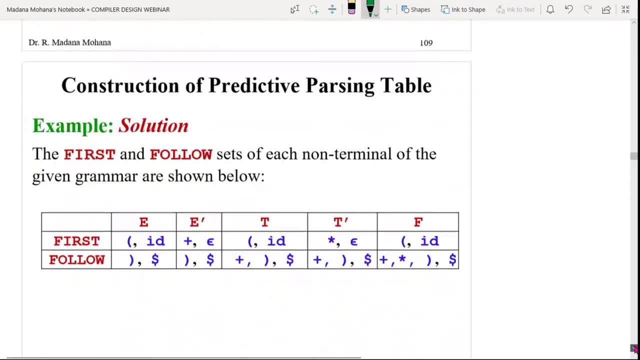 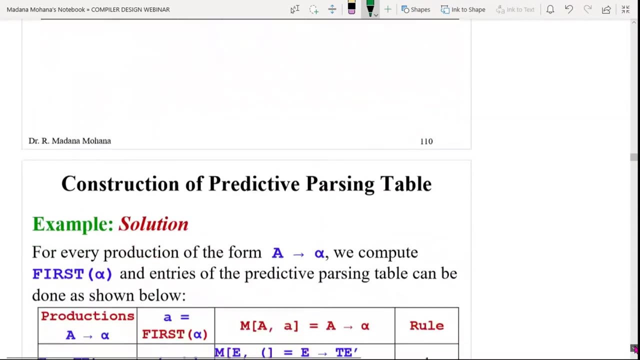 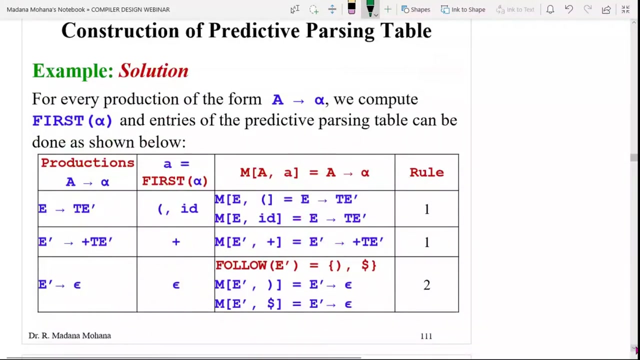 in predictive parser we already discussed. the grammar does not contains ambiguity. the grammar does not contains left recursion, then non left factored, all we have to consider. but this grammar is non left recursive grammar. only now you can see directly continuing with first and follow values. then the table first, the productions are of the form a derives. 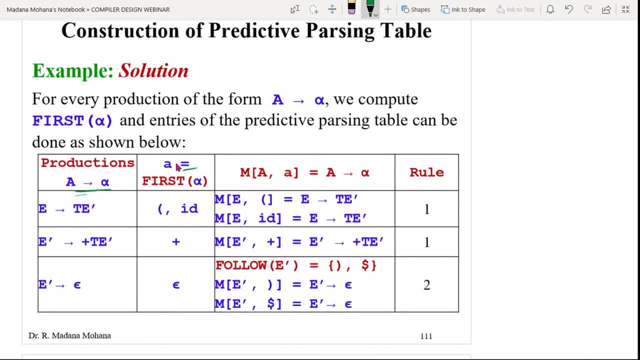 alpha. rule one: terminal: a derives first of alpha, a is the terminal. so now here, first of e, what is first of e first of e, left branch is id. now in the table, e on left branch is e on id. add this production. that is m means table name, m of e comma. left branch is: add this production. rule one: e derives. 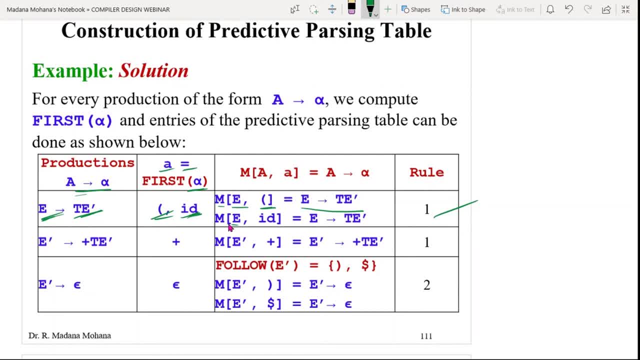 t dash, then id is next terminal: e m on e on id. e derives t dash. same rule one. the second production: e dash derives plus t dash. what is this first value, plus so m of e dash on, plus e dash plus d dash. rule one, that coming to rule two, right hand side, for null production. 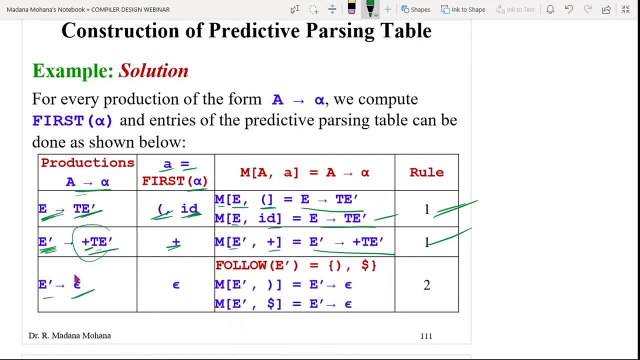 so we can apply rule two: e dash derives null. then for all of e dash- you have to find out for this- add this: null production for all of e dash, right branch is dollar. m of e dash and right branch is equal to e dash comma null e dash, that is null rule two. then m of 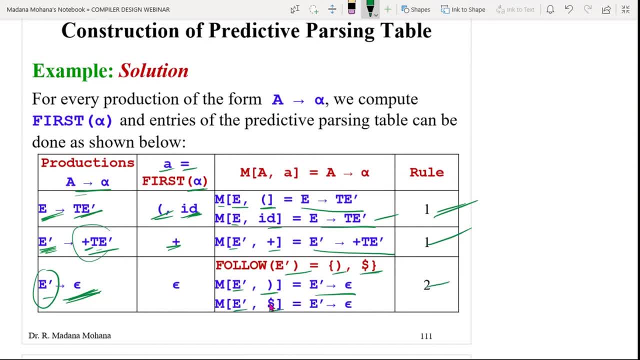 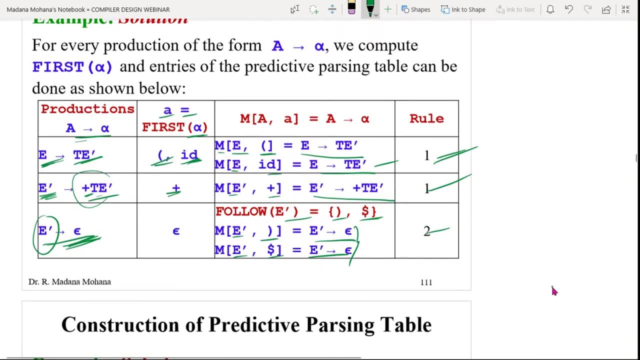 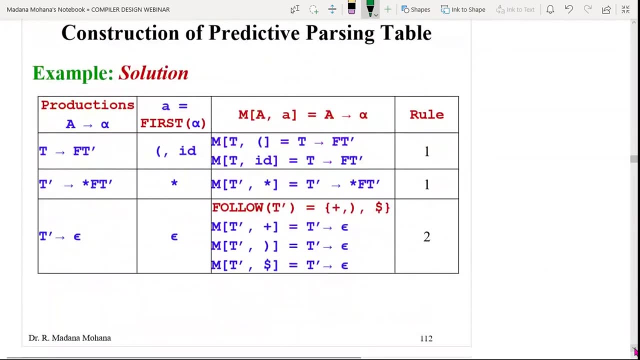 e dash comma dollar in the entry, at entry space. So in that case it has to be. that's is now two e dash on dollar. e dash there is null is added. so like that for all the productions you can apply rule one and rule two, rule one only for terminal, rule two only for epsilon. similarly, 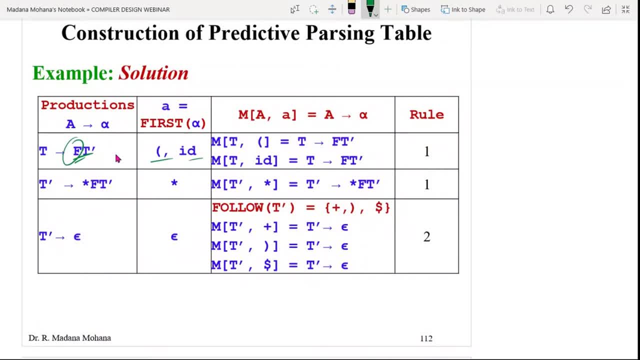 t dash ft dash. first of f, left parenthesis, id. then t on left parenthesis, t on id. add this production: t on left parenthesis. t dash ft dash. t on id. t dash ft dash, rule one. then t dash. derives star ft dash, your first of all, for first of star star. t dash on star. 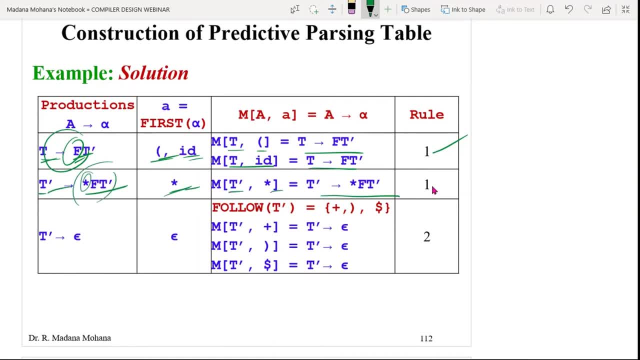 add this production at this production m of t dash, comma star, then t dash derives null. all of you can find out, all of you: das equals and dollar, all these entries, t dash on one place, and add this production: t dash dirives null by rule two. then what are the other productions? 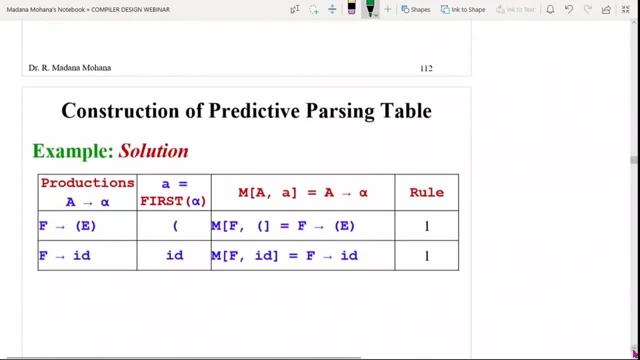 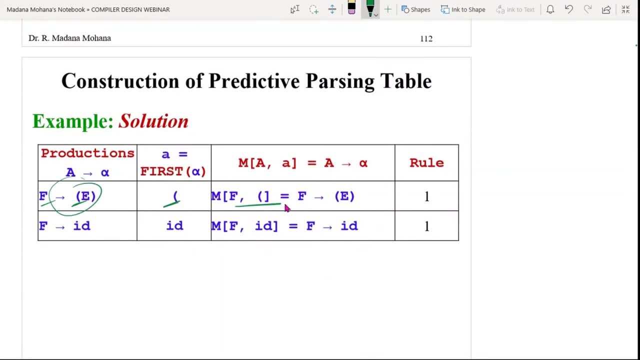 next step for f productions: f derives e. within parentheses: first half: alpha left parentheses f1 left parentheses. add this production rule one: f derives id. this is also terminal first half id id. f on id derives. f derives id is added here. rule 2 is not available. no, null production. 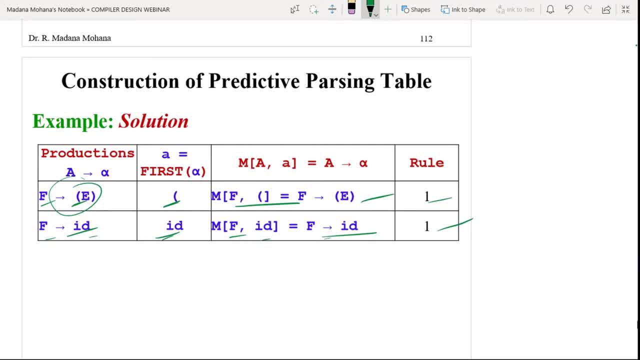 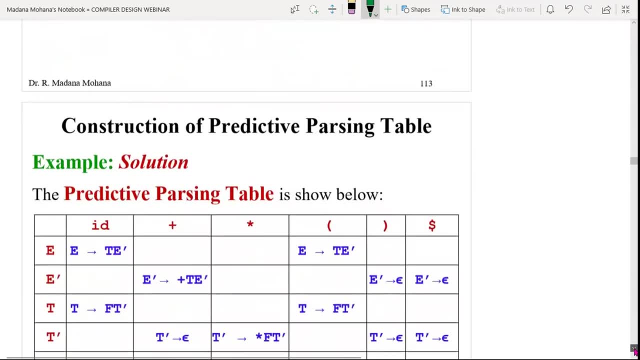 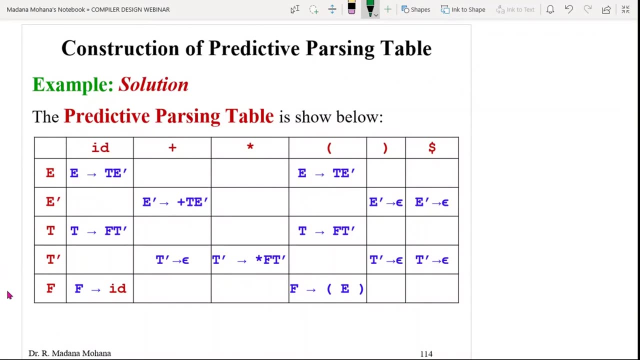 for f. now all these entries. now you can fill in the table. now how to take the table structure: all the columns, you can take all the terminals, followed by dollar, then all the rows, you can take all the variables in the grammar which can be occurred in the left hand side. this is the table. 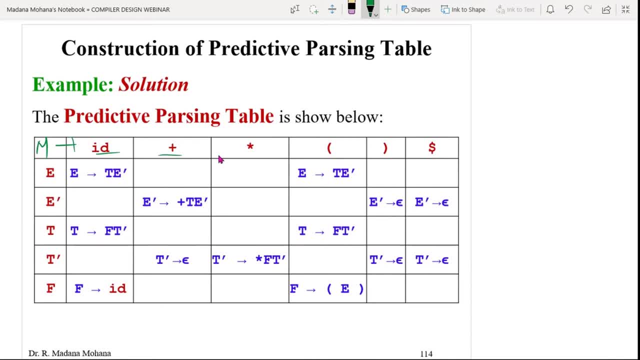 structure m. so row values: all are terminals, including dollar. dollar is default because this is the end marker. then all terminals in the grammar. you can add then row value, row values: all the variables in the grammar, your grammar having unique variables: e, e, dash, t, t, dash, f. now the entries in the above, whatever. 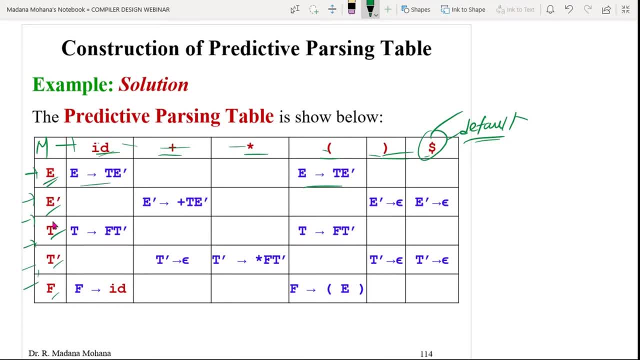 we calculated e and id, then e and left parentheses. unless he does and write for on the c doesn't dollar, etc. now all the blank entries denotes error here the entries in the predictive parsing table combination of a production or a blank entry to here. blank denotes error. this is the predictive. 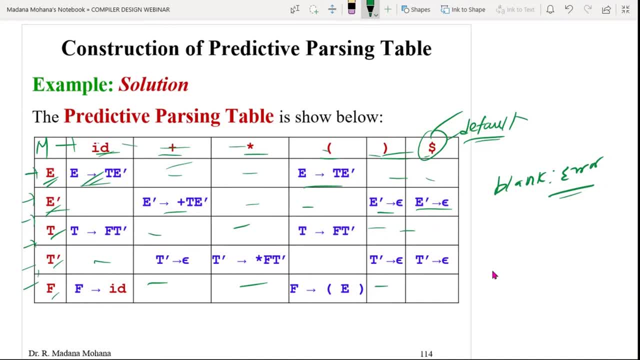 parsing table. Now, in this predictive parsing table you can define LL1.. What is LL1 parser actually Here? first, L stands for left to right scanning of the input. Second, L stands for left most derivation. One is the look ahead symbol. Look ahead, one input symbol. 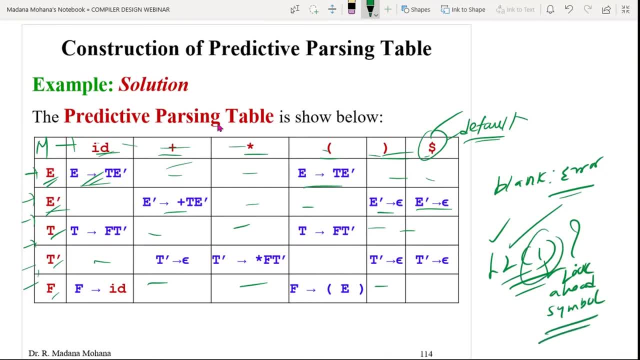 is considered So actually, when you can say a grammar is LL1 grammar by constructing the predictive parsing table. if the parsing table does not contains multiple entries, See all the entries consisting of a single production. here Single production, Suppose somewhere you are having, let us assume So here: T dash there is, Suppose T dash there is, null is. 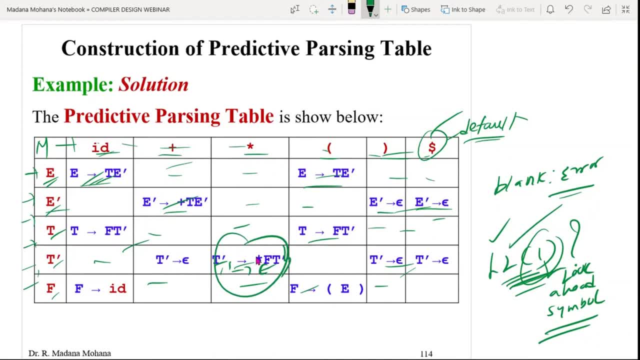 also Here, two entries. If any predictive parsing table like this, then we can say this is not LL1 parser. The LL1 parser means again, you need to construct the table like this by seeing multiple entries. If in at least one entry contains multiple entries, then this is not LL1 parser, But all. 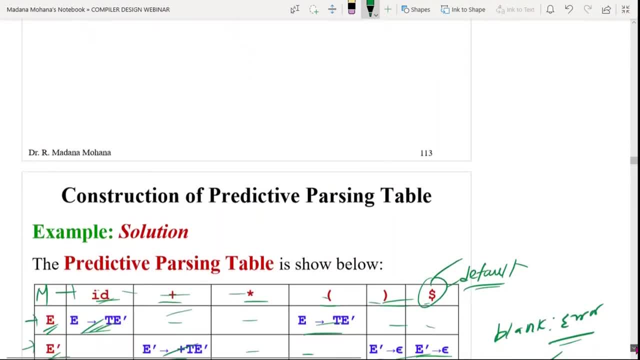 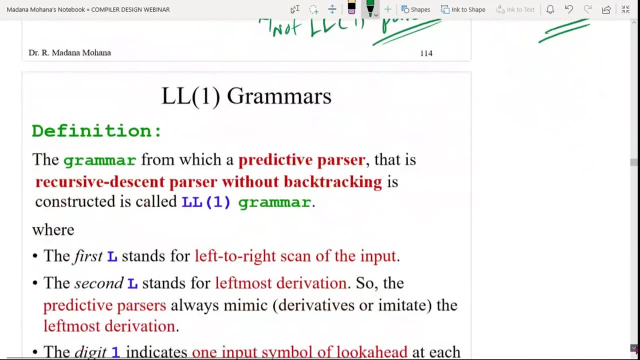 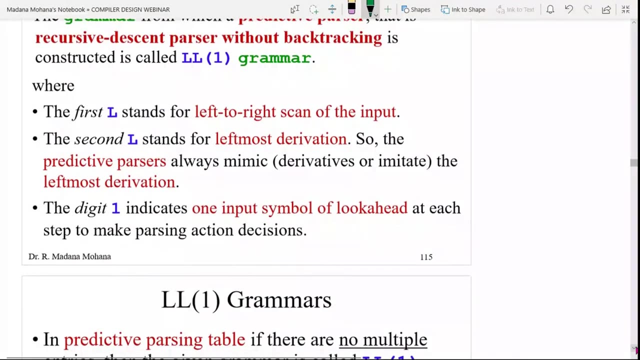 entries are unique, No multiple entries. then you can say: the predictive parser is also called as LL1 parser. by satisfying this condition, Here you can see, the same is given here. First, L stands for left to right scanning inputs. Second, L left most derivation. That digit one indicates the one input of look. 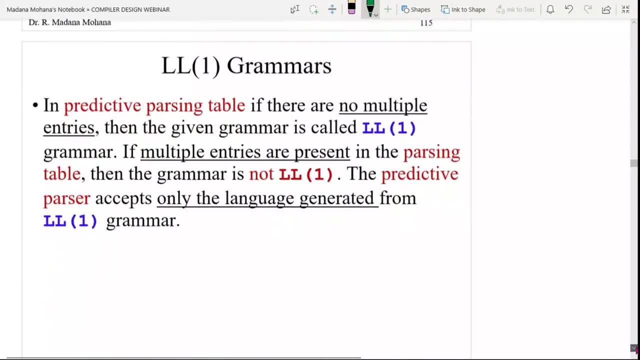 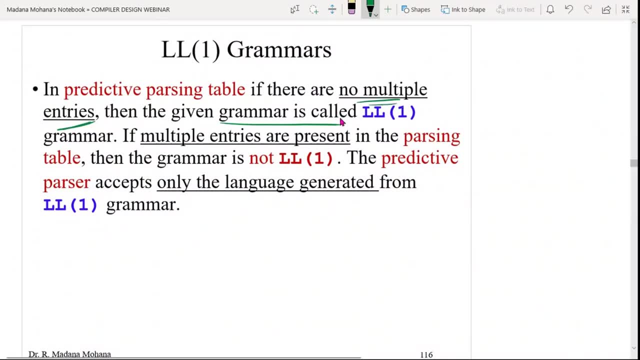 ahead. That is used to make parsing decisions using that input symbol In predictive parsing table. if there are no multiple entries, then the given grammar is called LL1 grammar. If multiple entries are presented in the parsing table, then the grammar is not LL1.. So this: 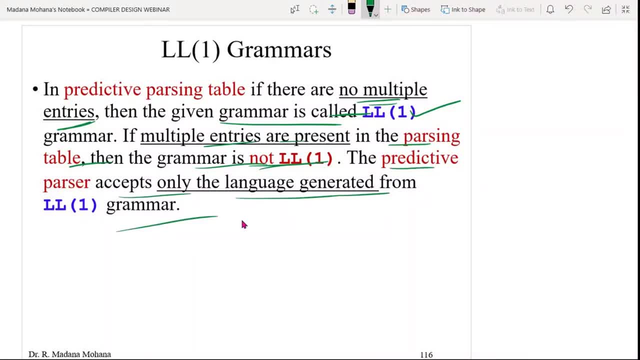 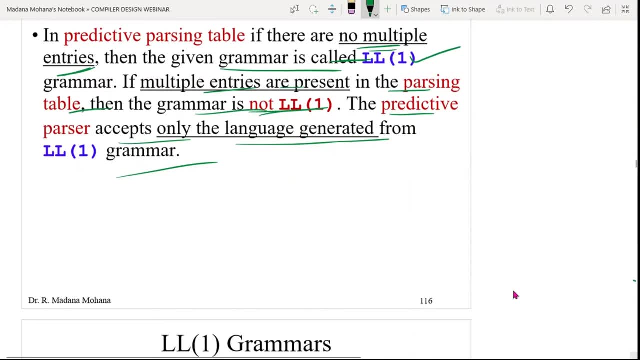 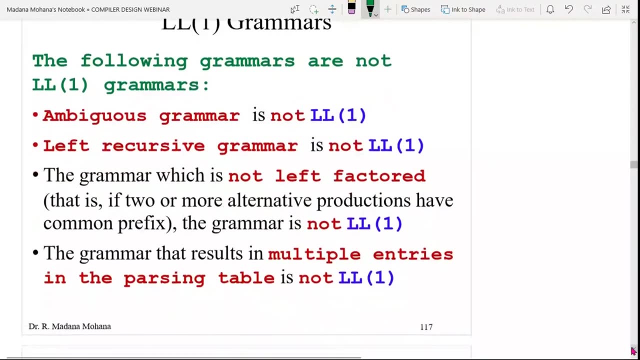 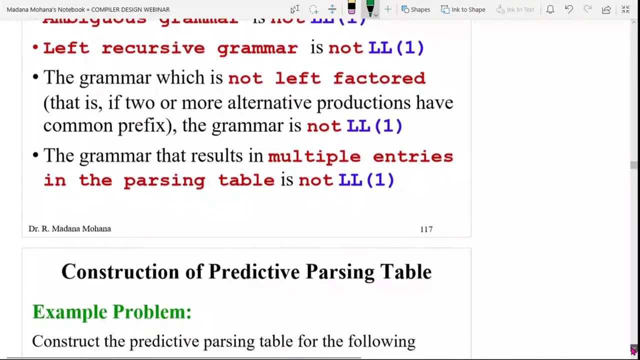 the predictive parser accepts only language generated by ll1 grammar. ok, now one more example problem. I have given here the same process and here some of the grammars are not ll1. any ambiguous is not ll1. any left recursive is not ll1 and non left factored also not. 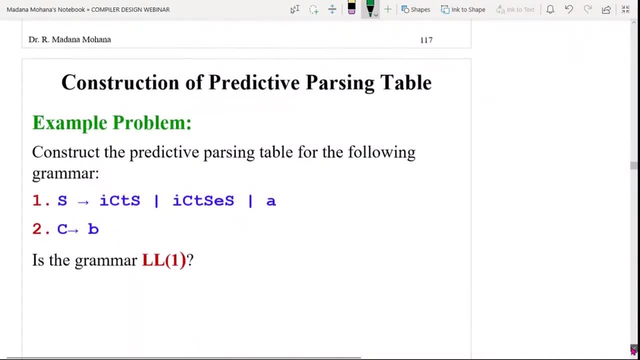 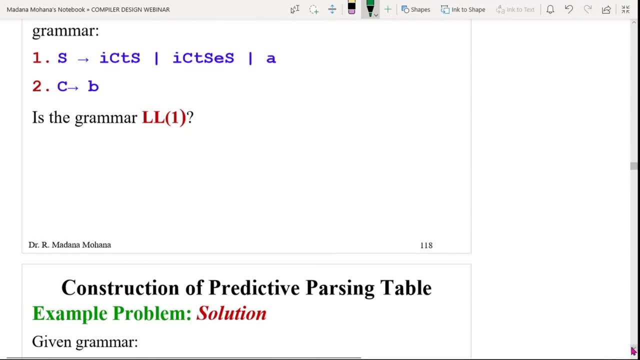 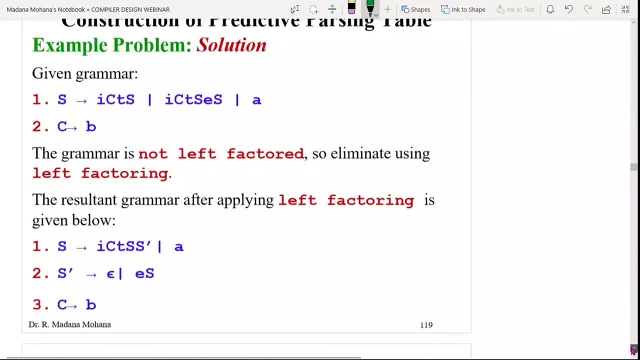 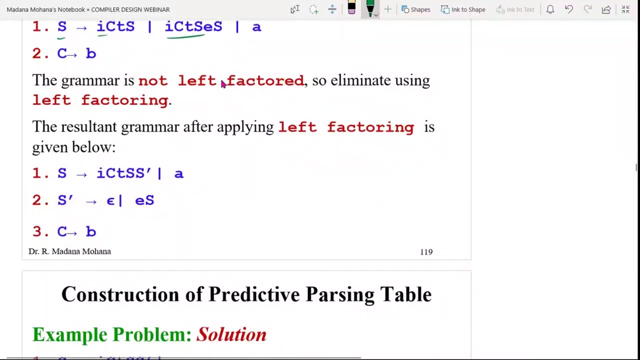 ll1. now the second example. this is also our standard question: S derives I C T S or I C T S, E S or A C derives B is the grammar ll1. the question will be given like this. so the same process. first you can see this grammar: actually S derives I C T S, I C T S here this: 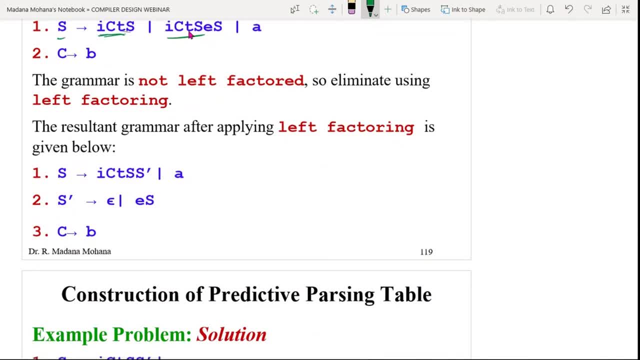 is not left factored I C T. yes, I C T, S is repeated, So common prefixes are there. we have to remove by applying left factoring. this is not left, not left factored grammar. eliminate left factoring by taking common I C T, S, S. 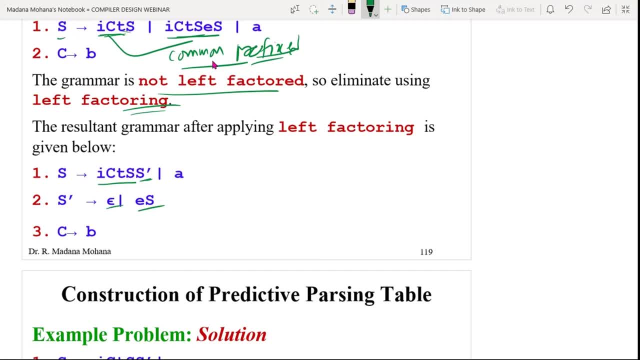 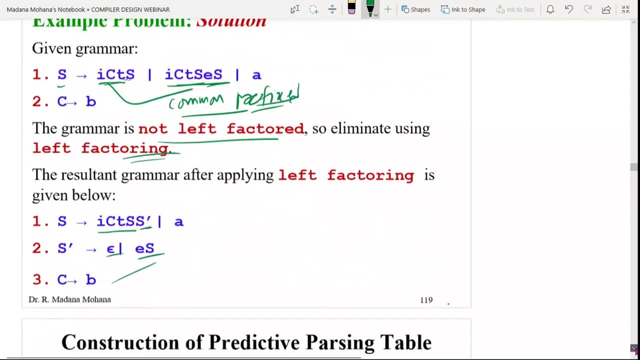 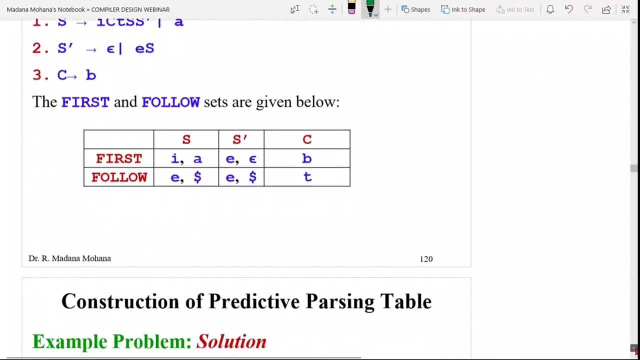 dash, S, dash, there is epsilon or yes. after this, whatever, this is the resultant grammar after eliminating the factoring. ok, now anyway, here left recursive is not there, Only left factoring we have to apply now. after that same, we can find out first and follow values. the same process first and follow values. are there, then the predictive parsing? 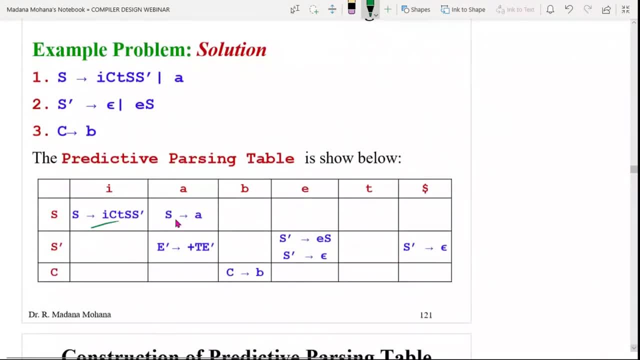 table directly. I have written here you can see now: is it ll1 grammar or not? how can you find? here you can see, we got two entries on the S dash on E, M of S dash on E. we got two entries. We got a regular comma, robot dot dot dash. but let us see now say H of S dash, undline. 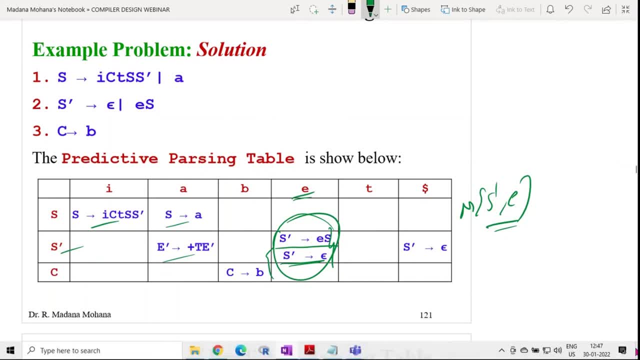 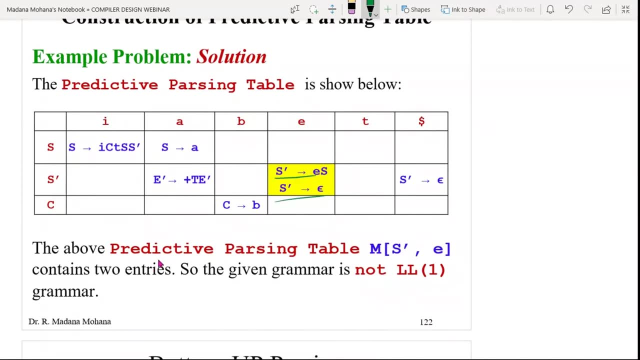 or we see에게 any one entry. if that context more than one value, then you can say that is not a ll1 grammar. here you can see above predictive parsing table M of M, of S, dash E and that is too empty. so the given grammar is not ll1 grammar, like that you can define. 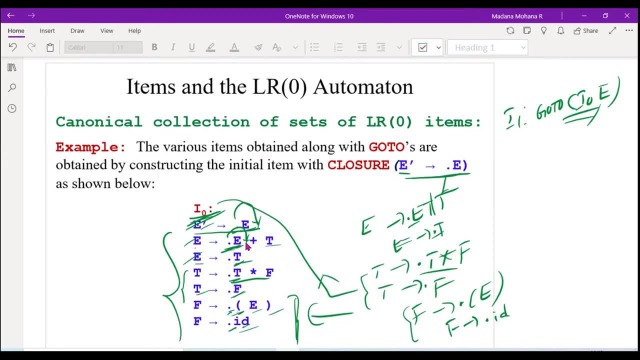 Number dot is moved after, dot will be a variable. is there then what you have to do? you can apply again closer function. You cannot apply again with thisometer. still, you cannot apply again with thismeter. as стrunnover stands好像 reply. not be there? yes, no think he said. 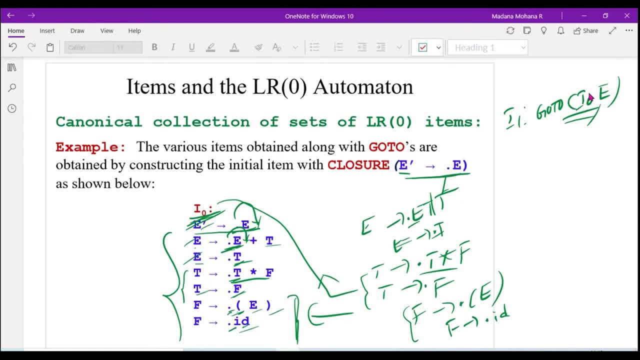 So like that go to function. we can apply over one grammar symbol at a time. only E means wherever dot is before E in all items you can shift after E. So this is one, Next another one: I2 again go to off from I0. only over E is over, then over T is also there. 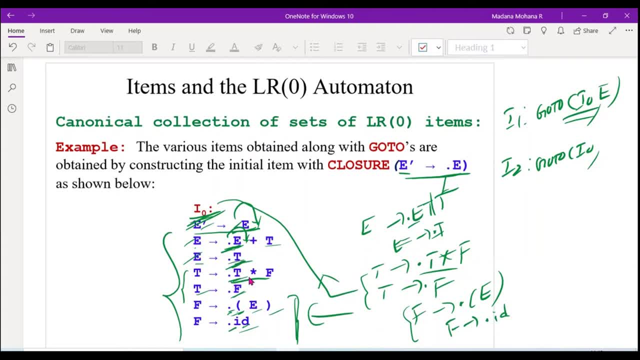 Over T. we are having two places: E direct dot T, T direct dot T into F. Now dot place after T. Now this will be next item. go to off I0 on T. here you can write and again you can apply closer rule, Then I3 again go to off I0 after T over, then after F. 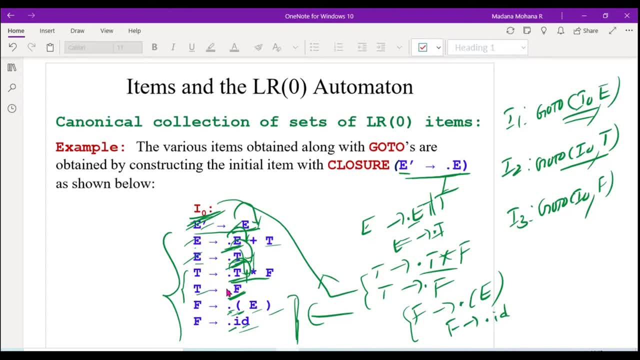 Dot is before F, now it moves after F. After F only one. you will get Then even terminals also you can take Then go to off. I0 on left parenthesis: Now dot moves after left parenthesis. Again, apply whenever dot is moved over a symbol. 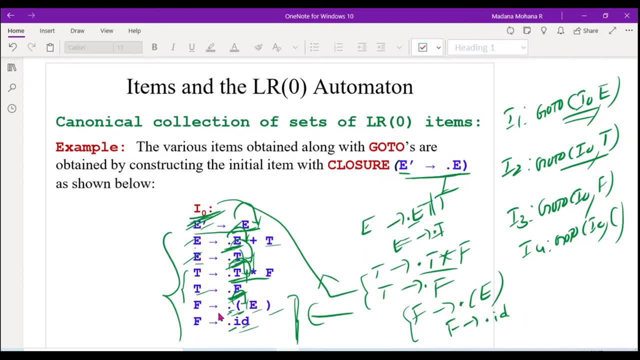 Compulsory. you have to apply closer rule. Then F derives dot ID. here dot moves over the terminal ID. go to off I0 on ID. See from I0 you are getting I1, I2, I3, I4, I5. these five new items are getting. 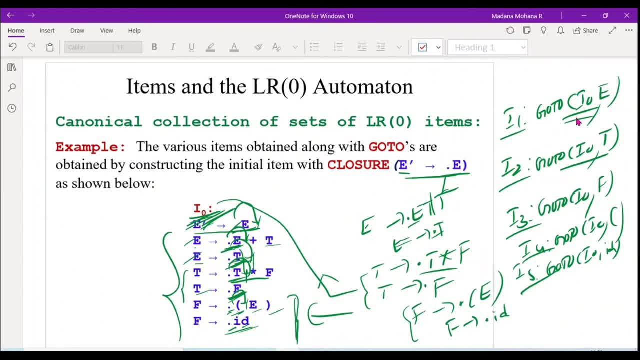 Again. you can continue with I1. wherever dot is there before a symbol, you can move again new item, then I2. also Like that. this process will be repeated till all the items should be completed items. what is meaning of completed item? dot should be placed at the right end. 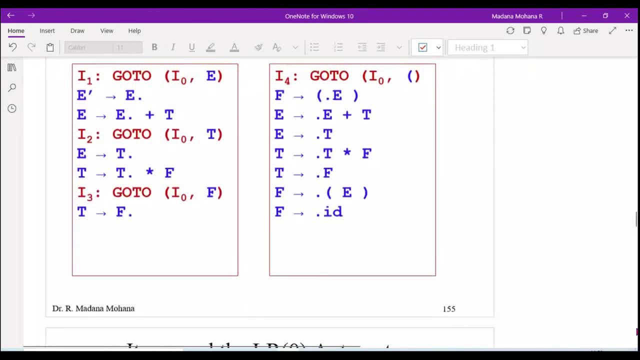 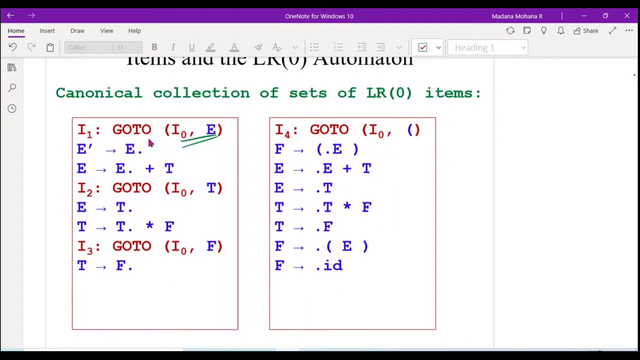 Dot should be placed at the right end in all items. till that we have to continue. Now you can see whatever I explained stepwise. so here I have given First I0 on E, That is I1 item. now dot moves after E. that means in I0 dot is there before E. 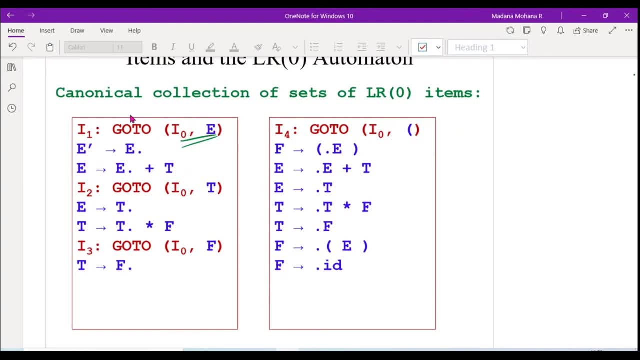 Now two places. we are having dot before E, now moving after E, E dash, there is dot E earlier, it is here now it moves over E Now. after that, nothing is there now. closer function is not applicable after dot. if a variable is there, then only closer function is applicable. 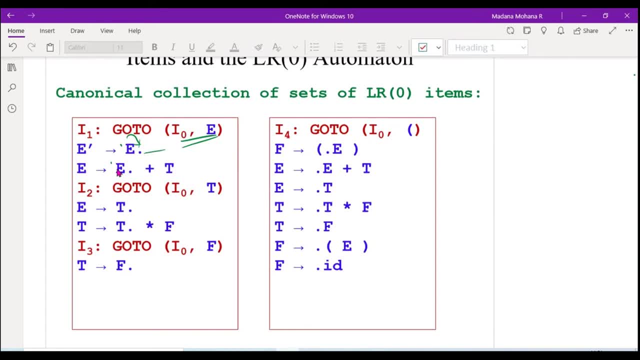 Then next one in this: before dot: here dot E plus T. Now moves after E: E, dot plus T after dot. we are having terminal. it is not a variable here. closer function is not applicable, only these items. further, no new items are added. This is called as I1 go to I0 on E. 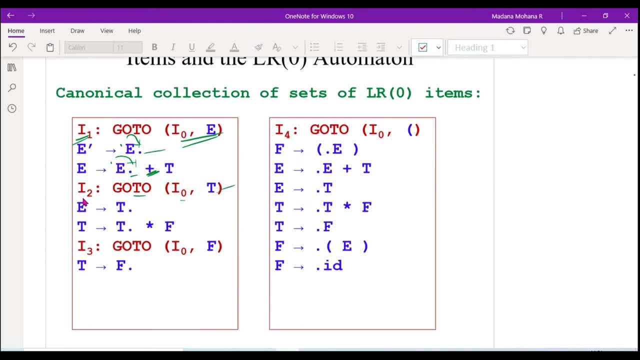 Similarly go to I0 on T, so that item we can name it as I2. previously we are having dot before T. now it moves here. after dot, nothing is there, no new items are added. Then T derives. previously we are having dot T into F. 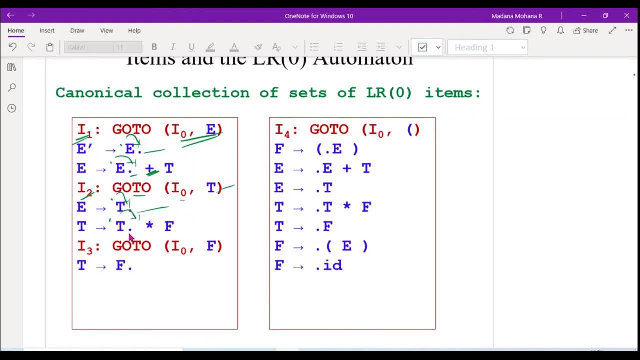 Now Dot moves after T. so now it will become T, dot star F. but after dot terminal. no new items are possible by using closer function. Similarly go to I0 on F. we are having previously T derives dot F. now dot moves after F. after F, nothing is there. now no new items are added. this is I3. this is completed item actually. further we can't apply the closer function, this one, wherever dot is there in the right hand side. 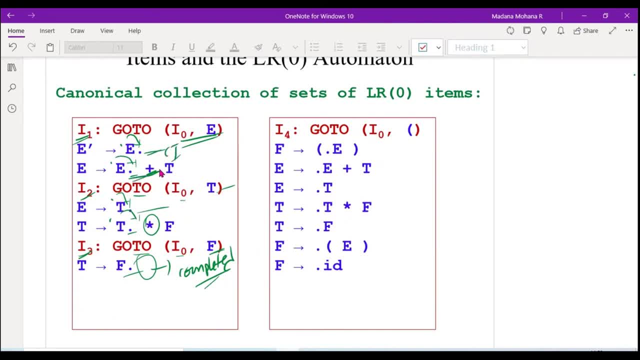 This is also completed item, but for this we have to apply again. this is completed item. again T, But for this we have to apply, because dot moves over star and over F, like that, but only one movement in one step only we have to do. Then similarly, I0 on terminal left parenthesis we are having earlier, F derives dot open brace E. dot is before the left parenthesis, now it moves after left parenthesis. 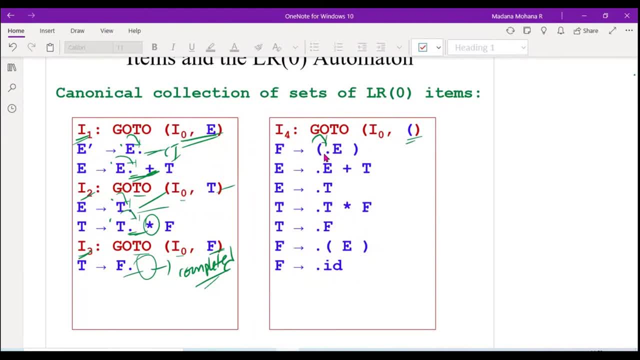 It moves here, passes it morespeed than the Left parenthesis. after that we are having in the left parenthesis This one also. again we are having a dependent momentum feature which moving dot over left parenthesis. we are having variable e again e items are added from the 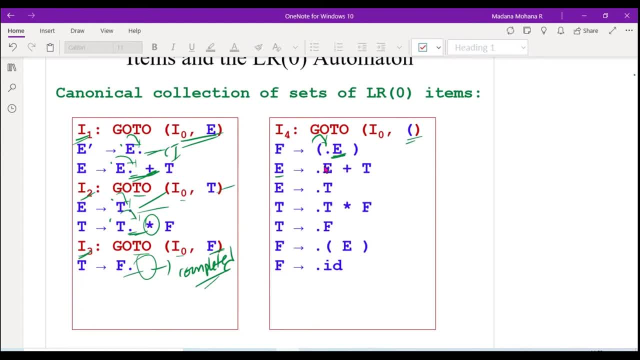 original grammar by putting dot in the right hand side, beginning now e directs dot e, plus t, e directs dot t. the same process repeated. now you can see dot e. all the items are there: dot t, now t items. you can add t directs dot t into f: t directs dot, f. again dot t, t items. 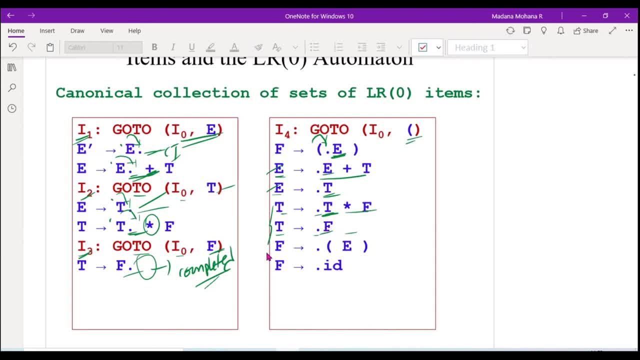 already there. now dot f, f items are not there. add f items: f directs dot left parenthesis e, right parenthesis f directs dot id but dot terminal. further no new items are added. this is i four, so i not on left parenthesis over next, i not on id. so previously we are. 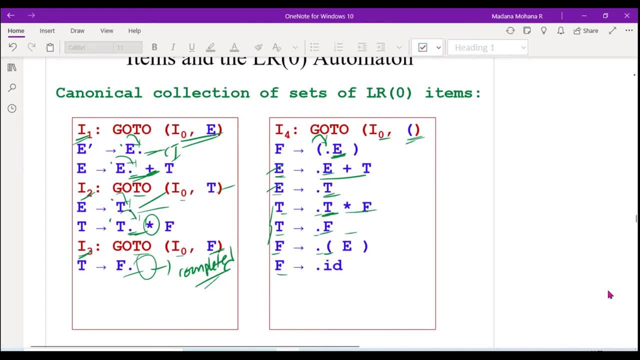 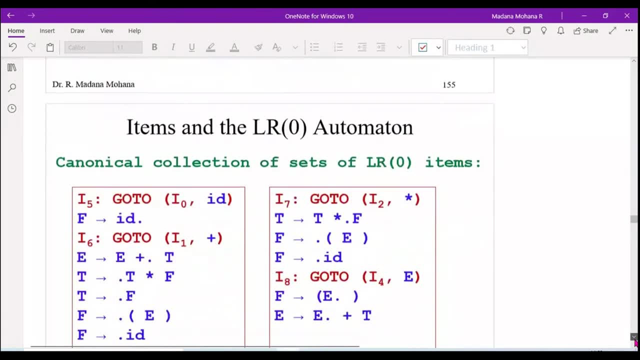 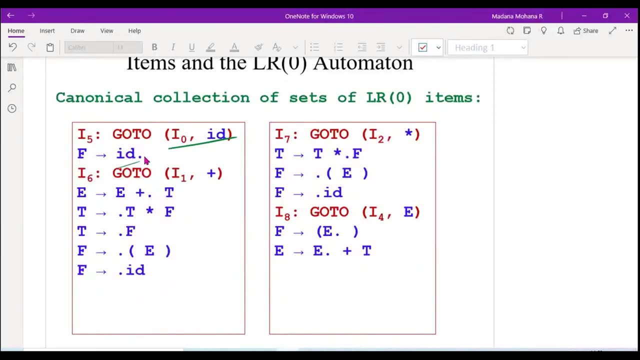 having in i not f directs dot id. now this will become f directs id dot. that case that you can name it as i five item here you can see. so go to off i, not on id. now dot moves after id. f directs id. further nothing is there. no new items are added. this is completed item. 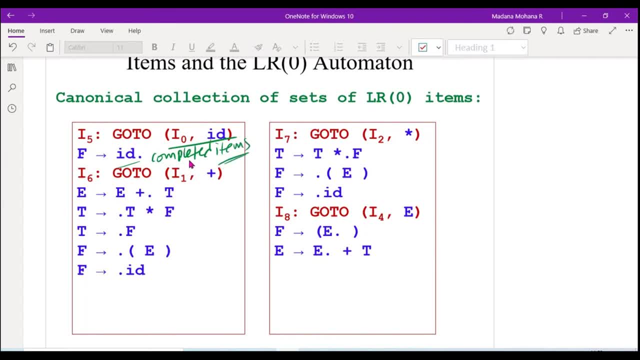 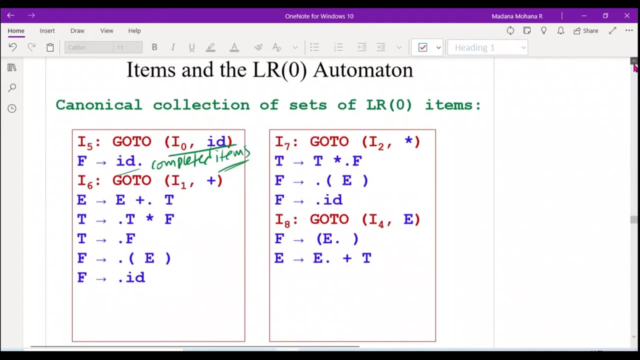 all completed items. further, we cannot apply the closer function or go to function once dot is moved to the right end. now i not is over. then go back and check. i one now, i one also, wherever incomplete items are there. for all again you can repeat the same process. 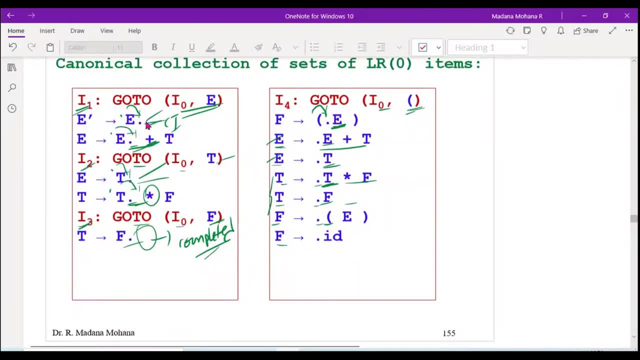 now you can see we are in i one. he does direct dot e completed item. but the e dot plus t is not completed item. so here you can see: e derives e dot plus t. it is incomplete item. this is in i one. now you can apply go. 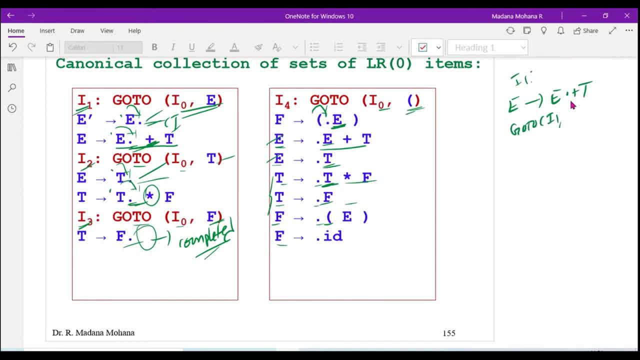 to function of i one on where dot moves over. plus this you can make it as a some. what is the number? i six or i seven, whatever, continue with the number. now. this is equal to f. all id dot plus t is complete item. but e dot plus t is not complete item. so here you can see. 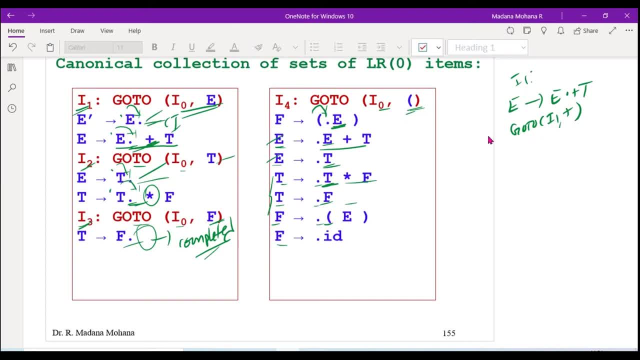 This is equal to go to off. this is some i6. let us check now here: e derives e plus dot t. dot moves after plus again after dot. variable t is there add t items. we are having t derives t into f by putting dot, then t derives f again. here you can see dot t already there, dot f. 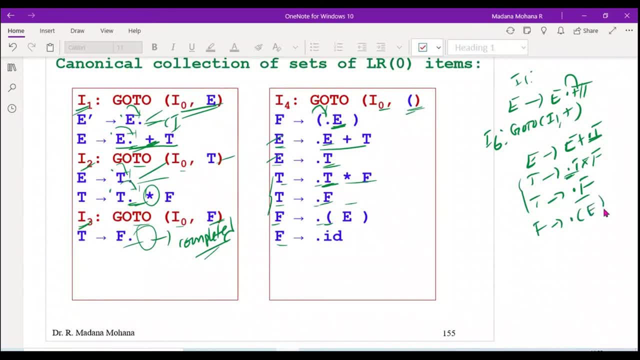 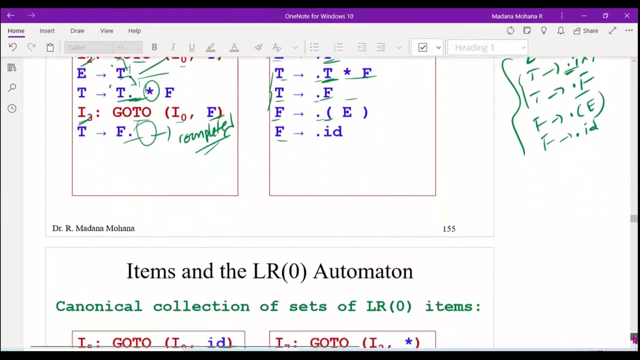 you can add to: f derives open break, then f derives dot id. now this is gotof i1 and plus, then from i1 only one. then coming to i2, from i2 you will get over star. so what is this item number where we stopped i0? let us see, continue the number. keep on repeating. 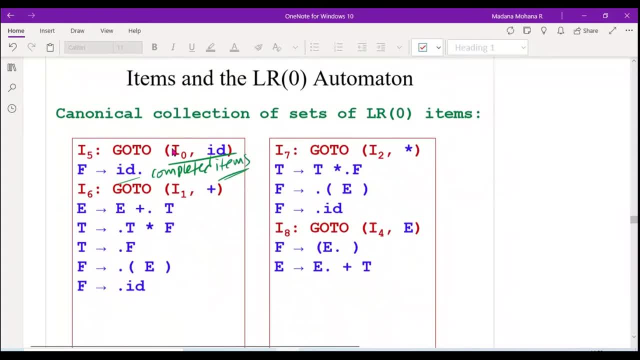 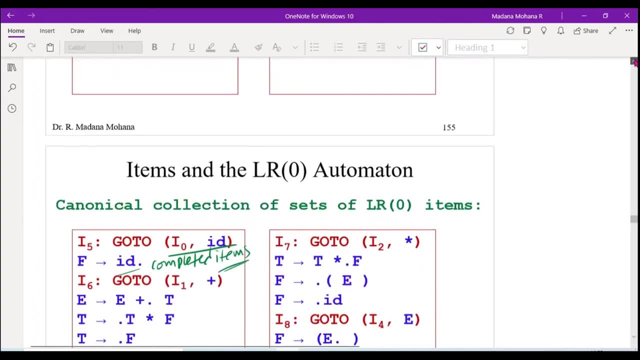 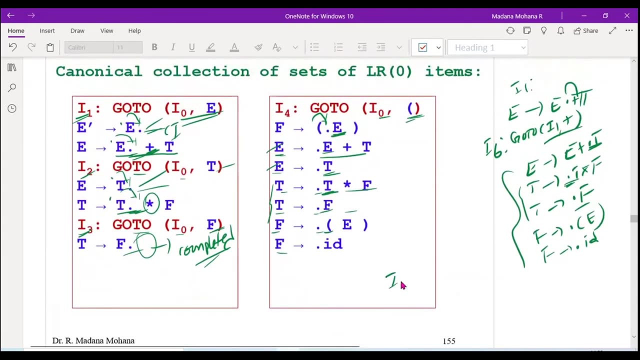 this process. items will be repeated Later. so now this is i6, what we went till now, next coming to i7. i7 from i2 item. we have to continue. so now i7 from i2, here goto off. i2 on the dot moves over star. now now this: 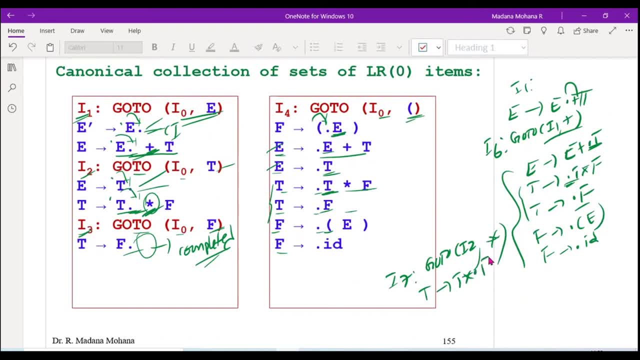 will becomes t. derives t dot star f, see after dot f is there variable Again, add it items by putting dot the f productions from the augmented grammar. now this is over i7, then coming to i3. this is completed item here. further known new items are there then? 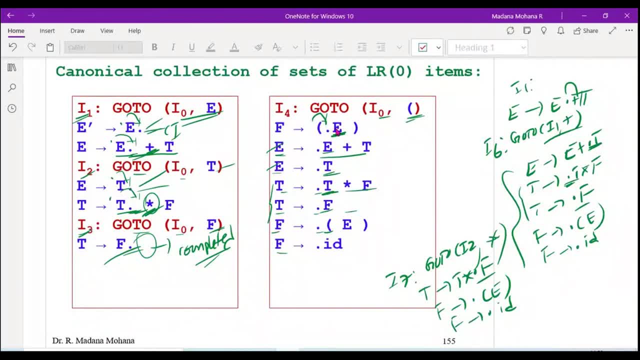 coming to i4 here, i4, many possibilities are there. why? because i4 on e is there. i4 on t is there? i4 on f? is there? i4 on left parenthesis: this item may be. you will get repeated one again. For example, let us see i8 from i4 goto off i4 on e. what you will get: dot moves after. 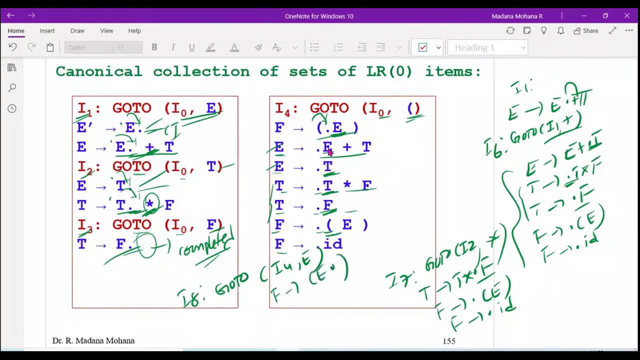 e, here you will get f derives t, dot, dot moves. after this: after dot at the terminal, no new items are there. then again here what you will get: e derives t, dot plus t. so after dot terminal, no new items are added. So only these two possibilities are there over e further no new items are added. this: 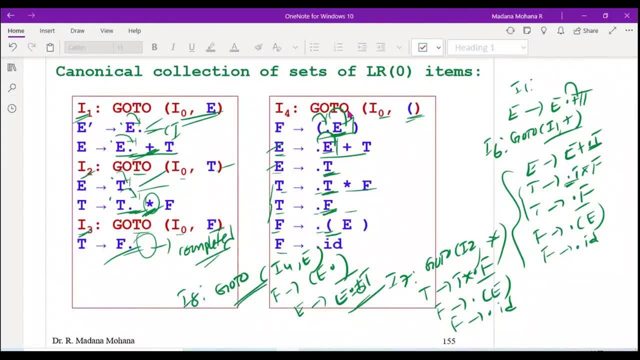 is i8. so then coming to i9 from i4, only over t you can take i9. goto off i4 on t. now dot moves here t dot, t dot star f. now you will get t derives t dot, then t derives t dot star f. 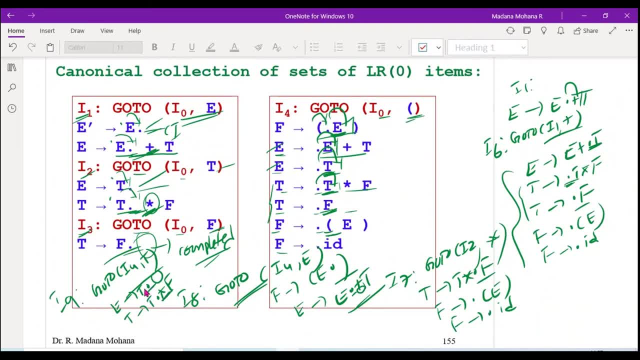 dot. nothing is there here after dot terminal. no new items are there then coming to i. 10. now over t is over, then over f. you can take here only one possibility is there now: t derives f dot. here you can see go to off i4 on f what you are getting. t derives f dot this item. 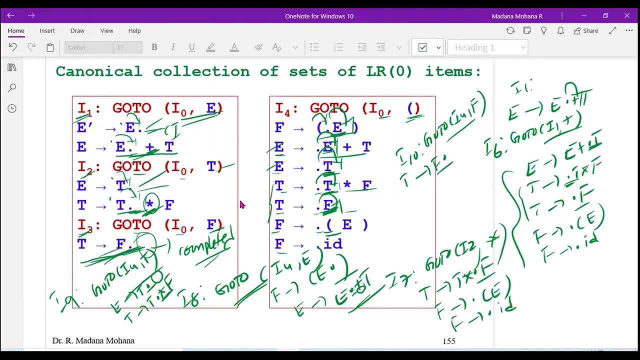 all over there. let us see: i3. t derives f dot. wherever repeated item is there, you can take the same name. what is the name here? i3 so, but in that table- slr parsing table- we can't consider i10. why? because this is same as i3. don't give number for this at the time of slr parsing table. 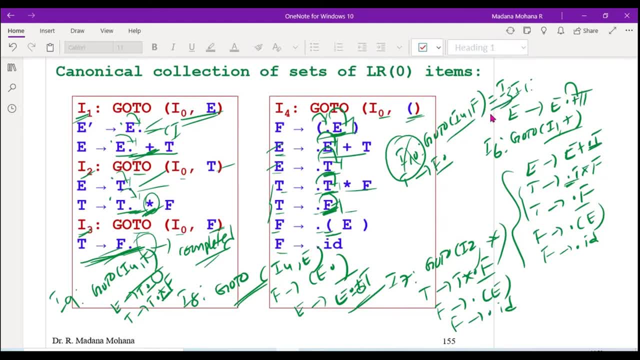 take only unique items. now go to off. i4 on f. you will get i3. only this is not a new item, already existing item. then over left parentheses here go to off. if it is new item, continue the item number. if it is repeated item, don't give the item number. i4 on left parentheses. let us see first what you will get: dot moves. 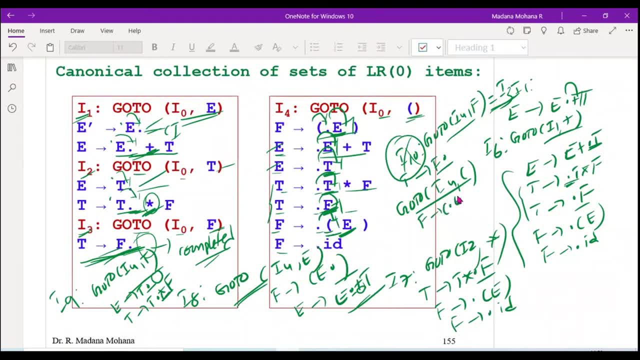 after e: f derives, left parentheses dot e. so dot e means again e items are added. so e derives dot e plus t. e derives dot t, again t derives. see again what is this one? you can see, this is same as i4, only we are getting here, you can see, you will continue. same as i4, so i4. 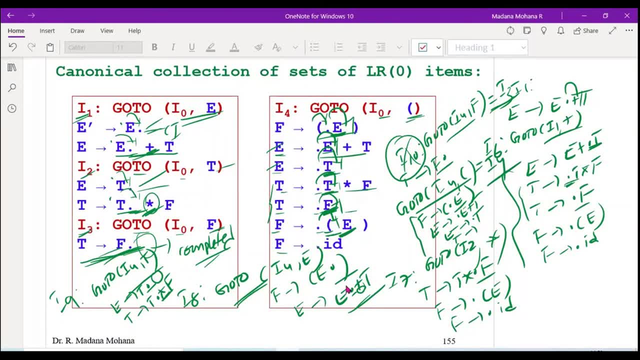 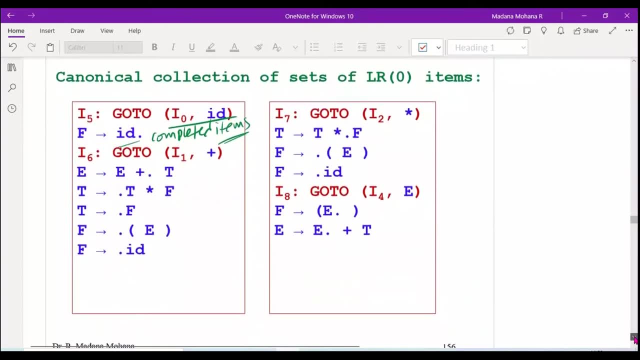 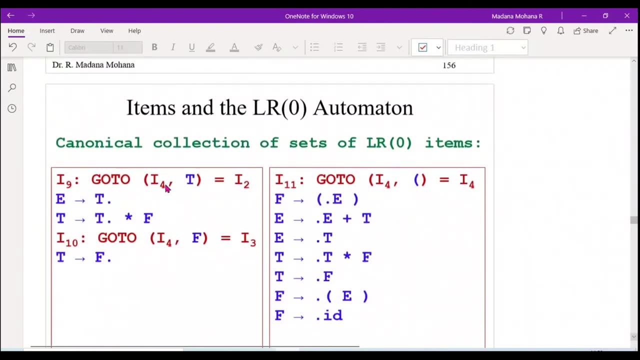 on left parentheses equal to i4. this is also repeated item, like that. you have to repeat this process for all the items wherever the dot is not at the right end. so finally what you will get, you can see whatever we explained. i4 on t. also, you are getting the same i4 on. 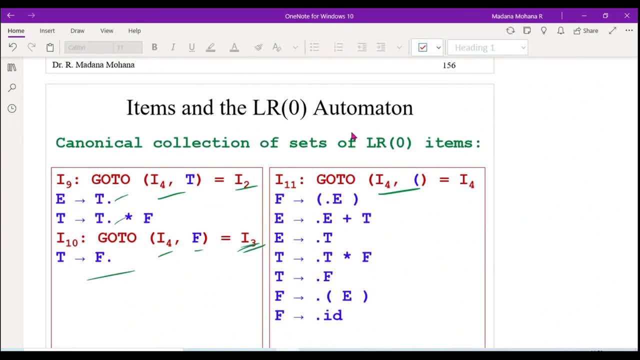 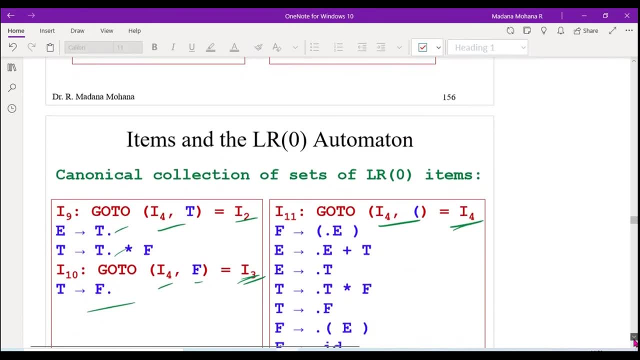 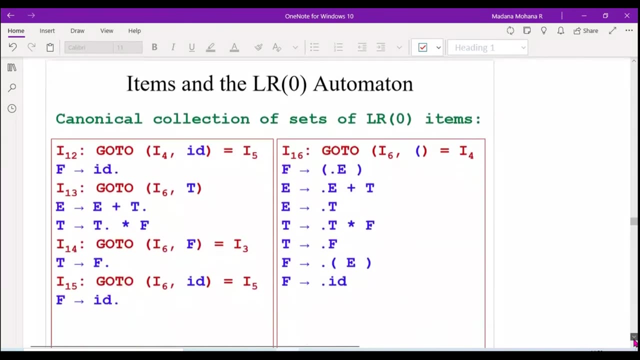 f. you are getting i3, i4 on left parentheses. just now we have seen we are getting the same i4. So here you can continue the item number. if it is repeated item, don't give the number why, because for slr parsing table we can take unique items for the construction. now you 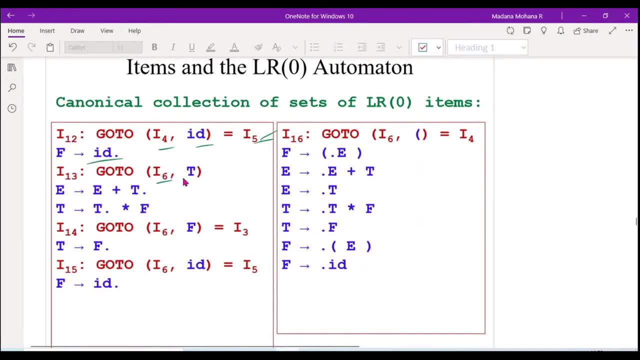 can see: i4 on id. we are getting same as i5, then i6 on t. this is new item actually, so you can continue the number. but here the numbers are continued, but table construction, these duplications you can remove now. i6 on t- this is a new item. 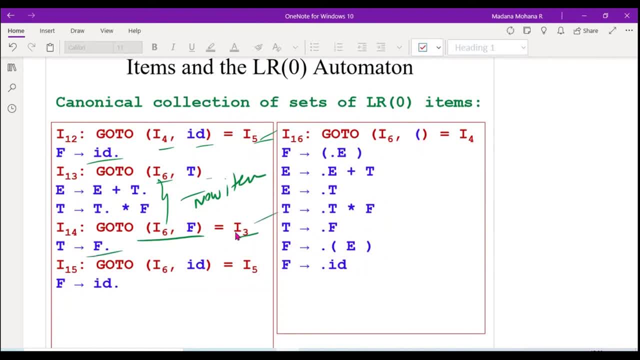 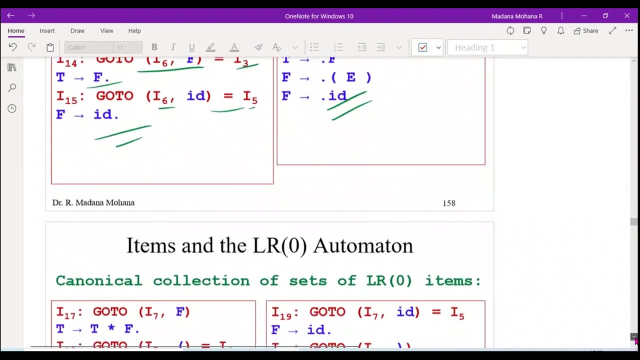 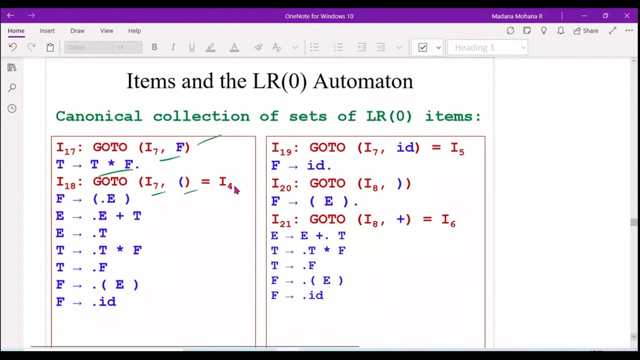 then i6 on f, you are getting i3, i6 on id, you are getting i5, then i6 on left parenthesis, you are getting as same as i4, only like that. this process you can repeat for all the items till dot is moved to the right end. now i7 on f, you are getting new item. i7 on left. 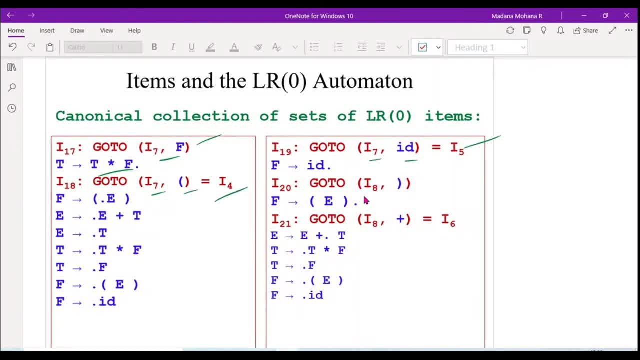 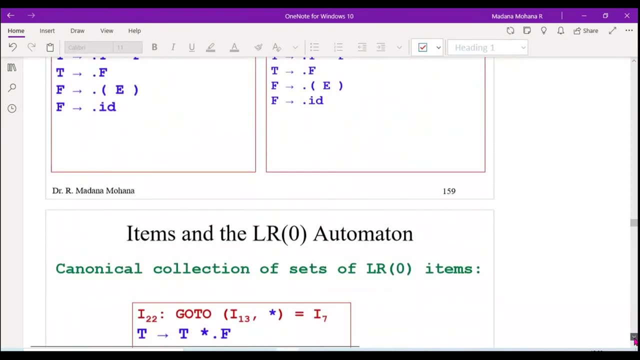 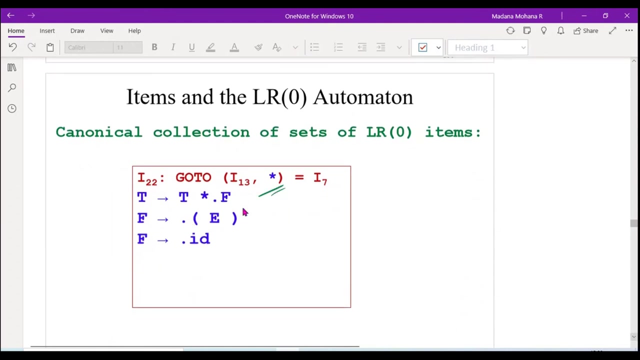 parenthesis, you are getting i4, then i7. on id, you are getting i5, i8 on right parenthesis. this is new item. i8 on plus, you are getting same as i6, like that you can repeat this process. then another one: i13 on star, you are getting the same as i7, with duplication. 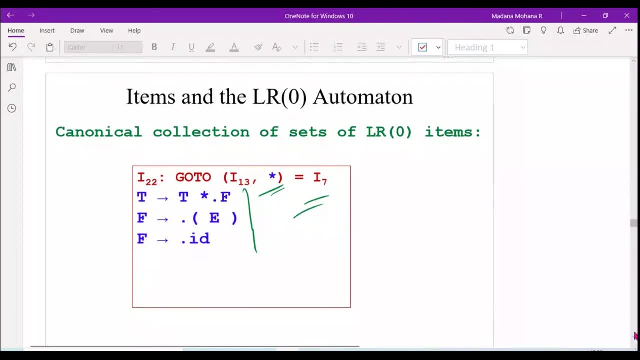 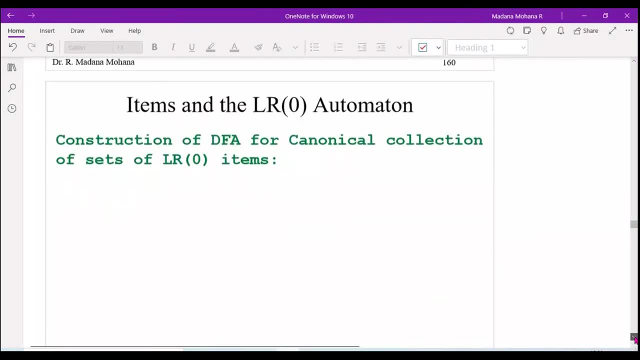 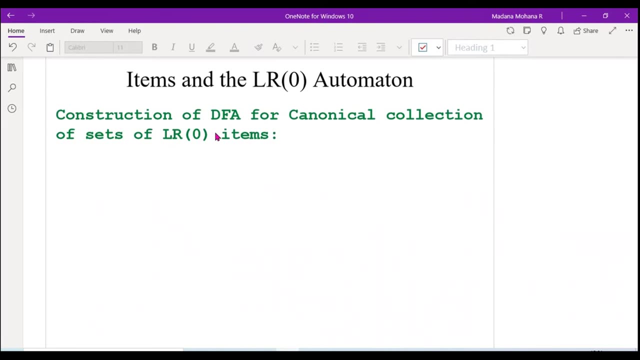 here total i02,, i22,, 23 items, By excluding duplication, the unique items that can be included in table construction, SLR parking once all the items are constructed. now you have to construct DFA. how to construct DFA for the canonical set of LR0 items. so the item i0, considered as the initial or start. 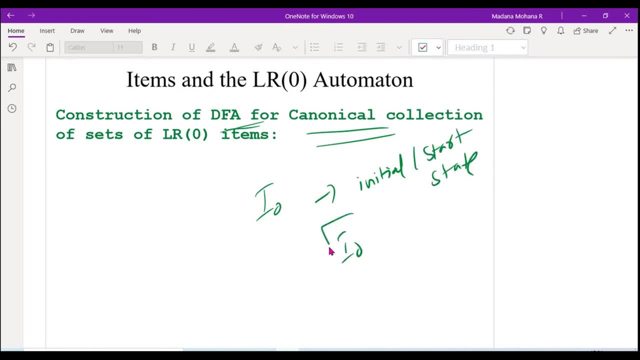 state you make it as this is one. Then go to functions. Go to function over all the grammar symbols, not only terminal over variable. also to go to of some i0 on e equal to some i1, let us assume So this is nothing but delta of i0 on e equal to i1, this is the transition, like this you. 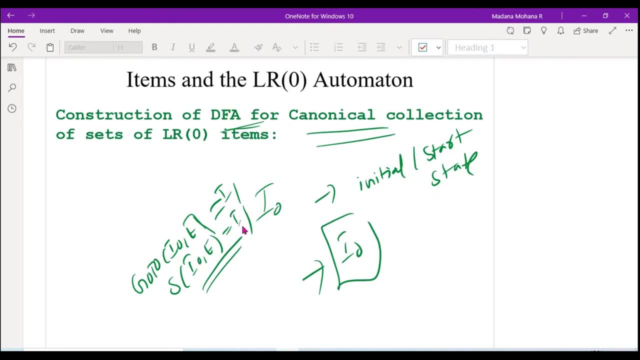 can write down the go to function. Now you can take: so this is i1,, i1 is the next new state. so here the same as transition diagram. So i0 on 0, similarly delta. then go to of i0 on t. this is some item 2.. 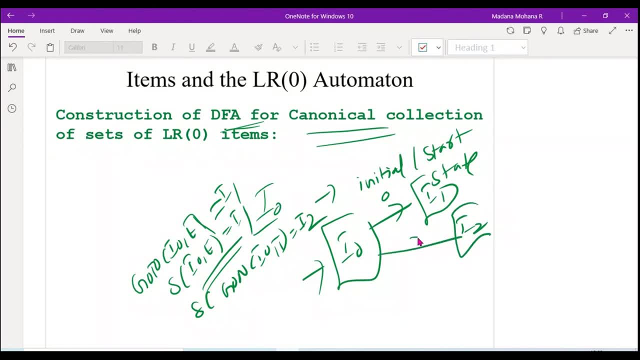 So then another one, i2, take here on input. what is the input here? the terminal t here do not think you know, automaton inputs are only sigma. but here in the LR0 automaton the items, I mean the inputs, are both variable as well as integral. So i2 take here. what is the input here? the terminal t Here, do not think in our automaton inputs are only sigma, But here in the LR0 automaton the items, I mean inputs, are both variable as well as. 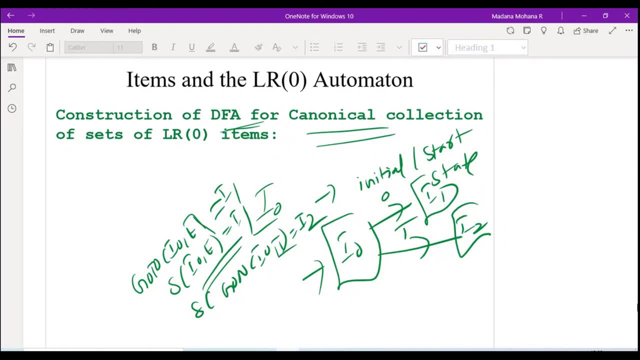 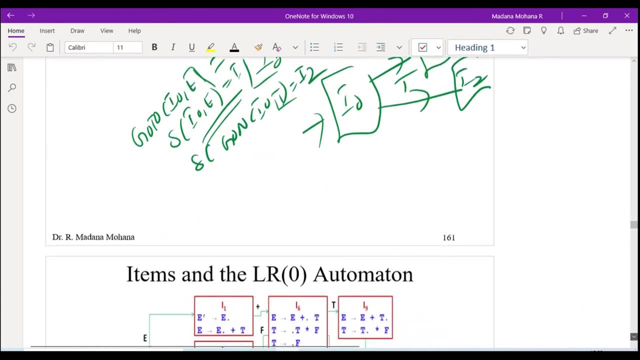 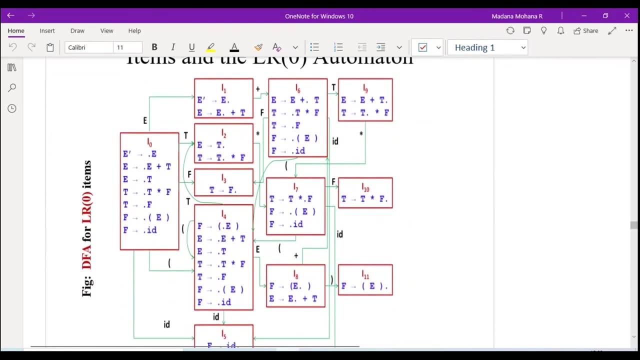 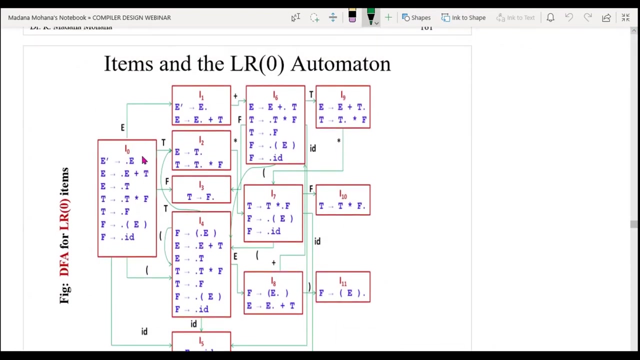 the terminal you need to consider here. So like that. now you can see the final DFA diagram shown here. So L R 0- automata. here you can see. So first initial item I naught we have considered at the initial. So here I naught, followed by all the items. also you can list. 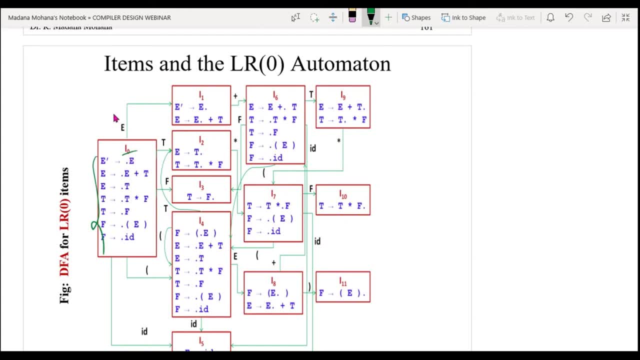 out Now. I naught on E. that means go to. this is nothing but go to of. I naught on E, equal to I 1. So here I naught on E. it is going to I 1.. Then go to of. I naught on T, it is. 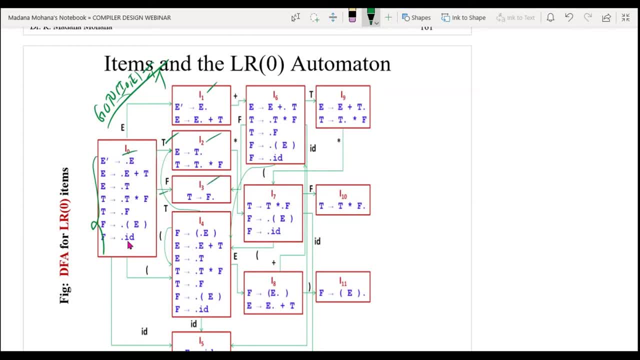 going to I 2. Go to of. I naught on F, it is going to I 3.. Then go to of. I naught on left parentheses, going to I 4.. Go to of. I naught on ID, it is going to I 5.. 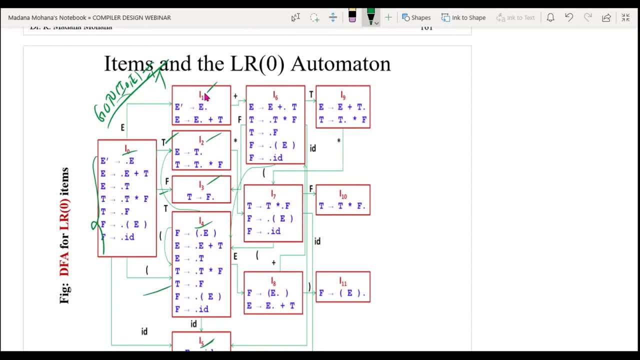 Then again from state 1, item 1. So go to of I 1 on plus equal to I 6. So then only one item is there. Then I 2 go to of I 2 on star, it is going to I 7.. Then here also only 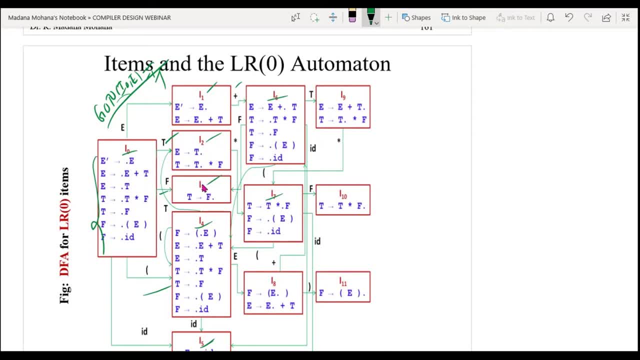 one is there. Then I 3 from I 3: this is completed item, no transition. Then I 4, I 4 on left parentheses: the same loop. Then I 4 on ID, it is going to I 5.. Then I 4 on E, it is going to I 8.. So like that same. 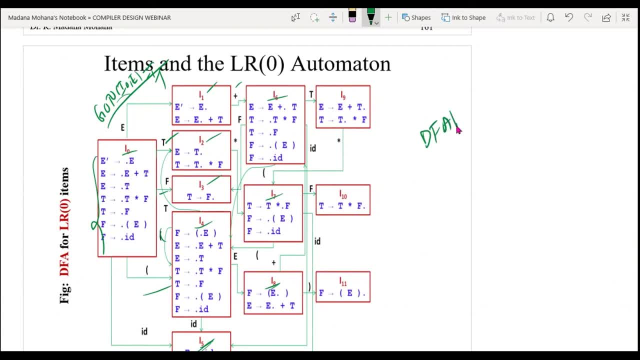 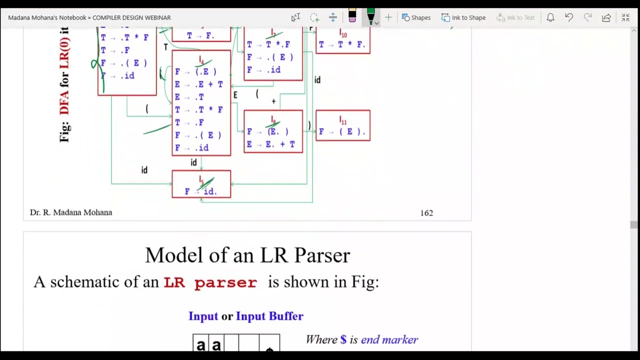 as our DFA automata. How to construct a transition diagram, Transition table. not included here. only transition diagram used for L R 0 items. Like this we can construct the DFA automaton for L R 0. it means Now with these items, Now. 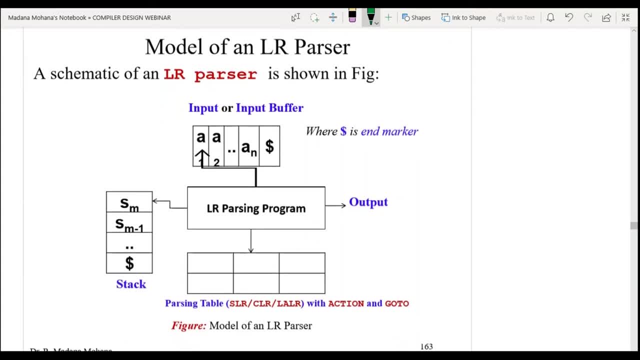 How to construct our SLR parser. Before that, this is a common model of L R parser, either symbol L R or canonical L R or look ahead L R. Same say model we have to follow For only parsing table. SLR, CLL Or LL With action Go to this parsing table having 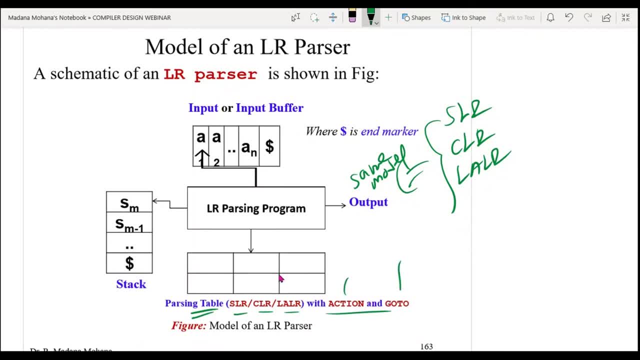 2 parts: Action part. Go to part. Okay, we will see about this also. this is the model. you can see the predictive parsing model similar to that. there we are having predictive parsing table here, LR parsing table here also stack. 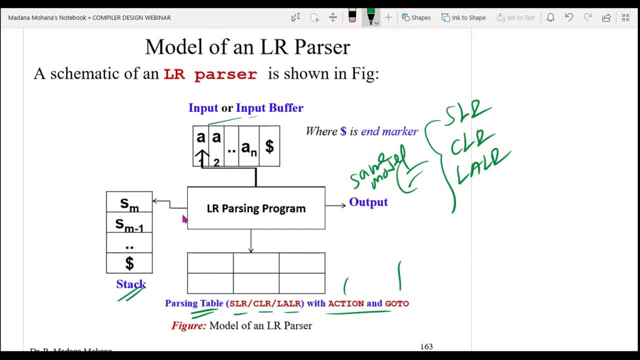 is there input or input buffer? is there here stack symbols? but these are all states, whereas in a predictive parser what stack contains grammar symbols, but here it contains states. so state 1 to state n, that means item 1 to item n, 0 to n, the suffix values. 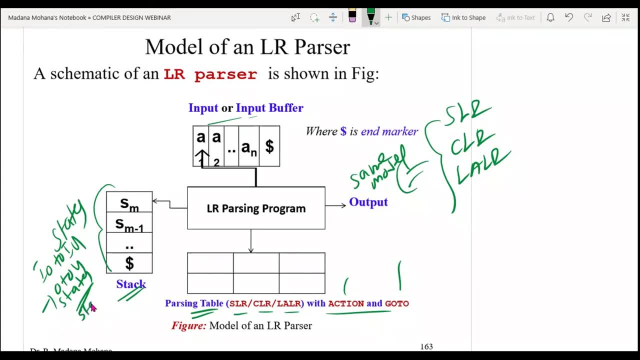 are states will be used here like state 0,- that is, S0, state 1, state 2 and so on. state n- these are all the state values. here input contains same as input symbols, only ended with dollar. that is n mark. here their predictive parsing program, here LR parsing. 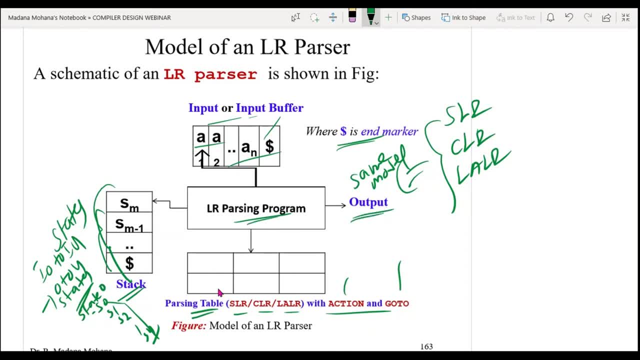 program here output Parsing is successful or not, then parsing table where predictive parser that is two dimensional. so here this table having two parts: action part and go to part. for all the three types of parsers, same action, go to values are there but the construction. 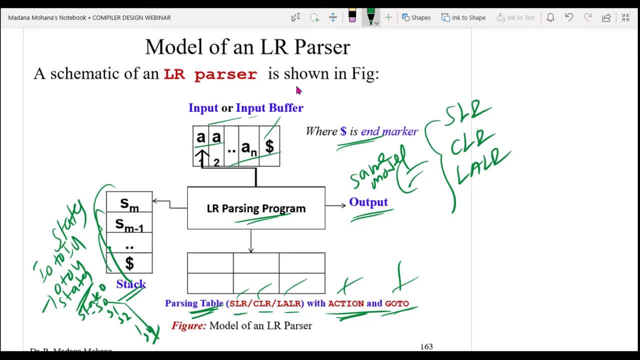 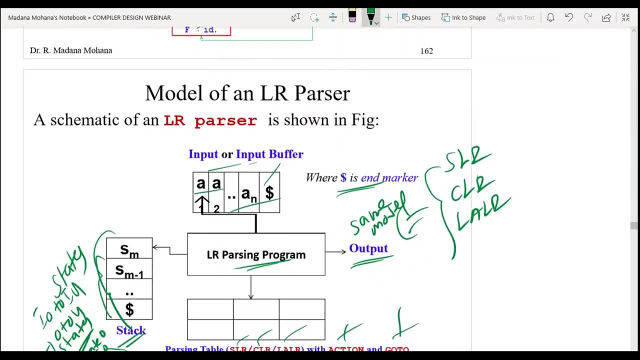 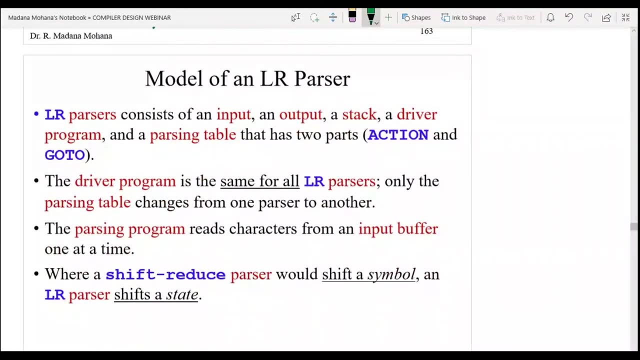 process is changed for all parsers. this is the common model. only parser to parser the table is different, but the table structure is also same. Same action and go to part. now you can see the LR parser consisting of input output stack, then parser program parsing table. it has two parts. action and go to the parser. 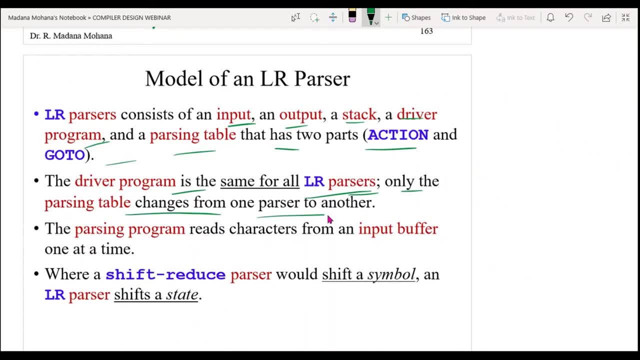 program same for all LR parser. only parsing table changes from one parser to another parser. the parsing program reads character from the input buffer, one at a time where shift, reduce parser. that means shift, action, reduce action. shift a symbol, then action go to part go. 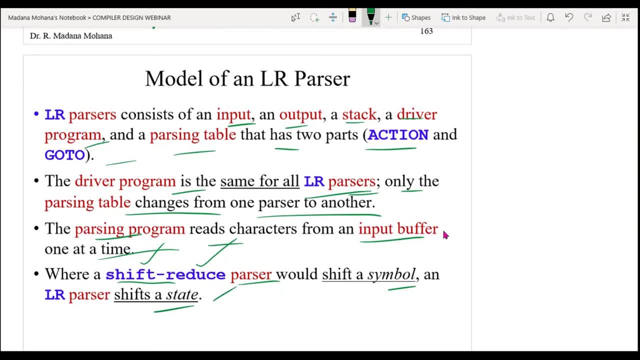 to the Sverer integration, then LR parser, and LR parser shifts a state, So shift will be denoted with s, followed by the suffix state number, which is state, for example, shift I. this can be written as s suffix: i shift i. santa can be written: as s one. so s means shift, suffix means state number. Then another value reduced denote with of value. this can be written as S 1, so you implement this in this example that is, hoy Derek class will. the tags now you can set. 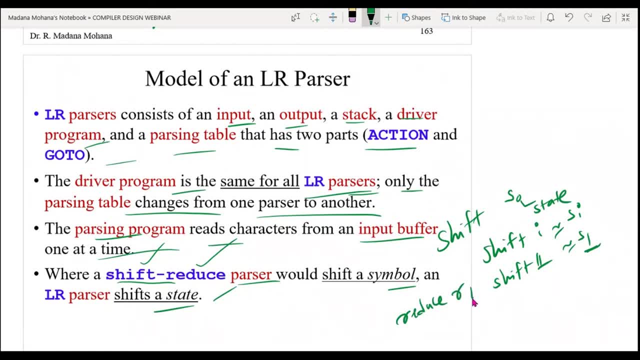 up these flags values at every time for each one right, double. familiarize this statement, correct. you integrate it. on the other hand, you are using the tags of: you write to�나 received R with production. for example, E derives E plus T, So actually reduce by this production. 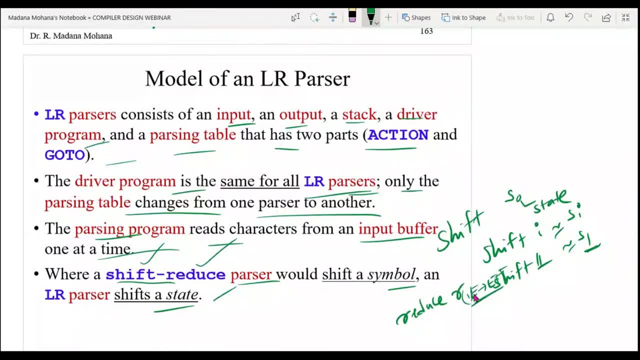 what is the number of this production? for example, in the given grammar, original grammar, whatever the production number, suppose R1. then reduce by second production, R2. reduce by third production, R3. reduce by fourth production, R2. these are all reduce value, these are all shift values. then text value accept. this can be denoted as AC text value error. this can. 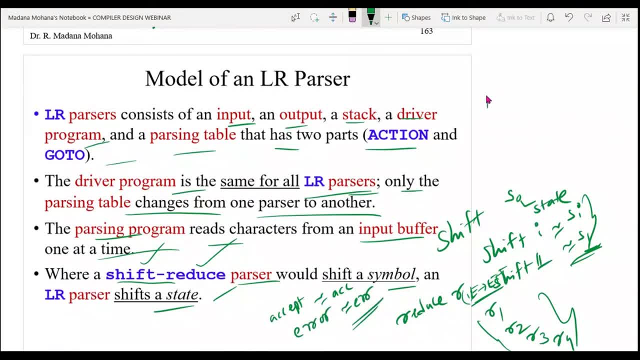 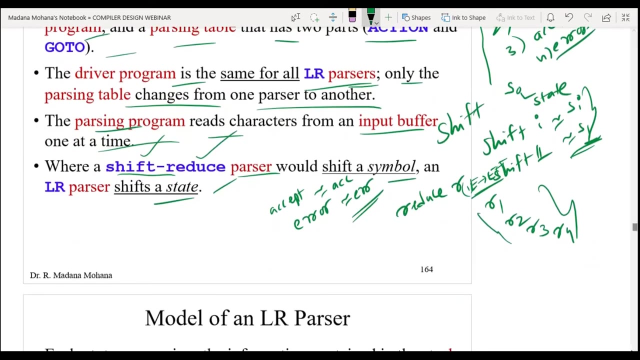 be denoted as ERR. So in the parsing table, first value is shift value, denoted with S suffix I. second value, reduce, denoted with R suffix state number. then third one, accept. fourth one error. Error means all the blank entries. So any any LR parsing table which is combination of these four values, only Now how to construct SLR. 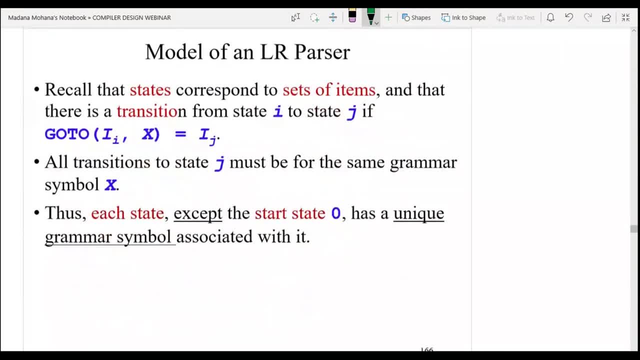 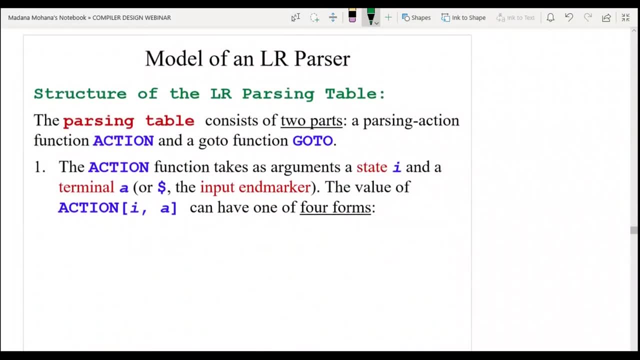 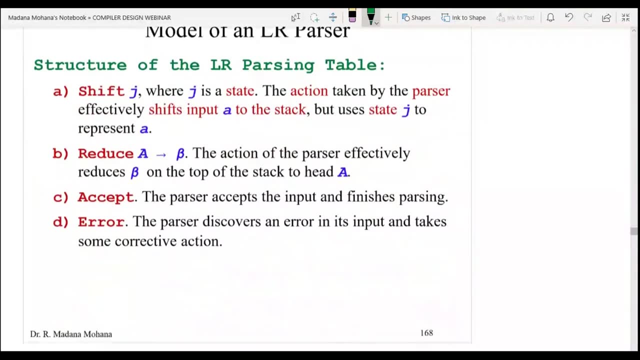 parsing table. let us see. First is the algorithm. The parsing table algorithm is also almost same. only in SLR parser LR0 items are there, whereas CLR, LALR, LR1 items are there. How to construct LR1 items: that we will see after completion of this SLR parser. 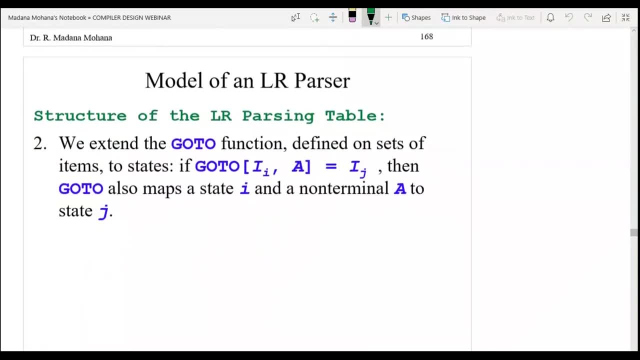 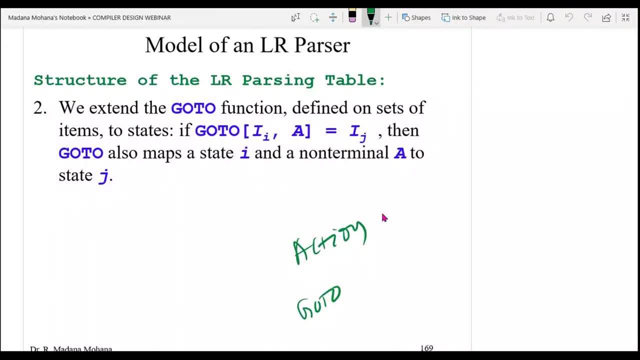 Now let us see how to construct LR0 items and how to construct SLR parser: LR1 items. Now the action part in the table: Action part go to part. Action part will contains terminals plus dollar. go to off, only variables, only variables. So action part contains the predictive parsing table, like 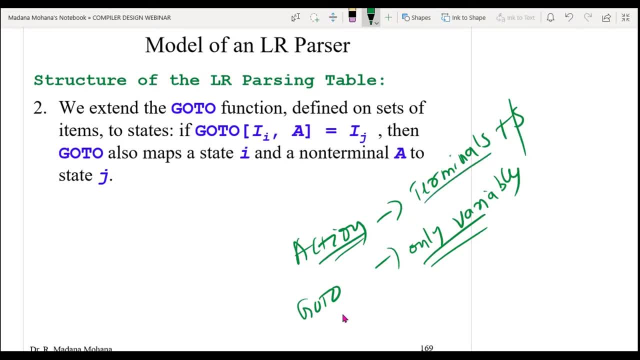 So variable combination, terminal combination, including dollar, whereas goto part only variables like delta: delta of q0 on 0 equal to q1, here goto of i0 on 0 equal to i1, so from state 0, this is the variable. let us assume 0 on e, the state is 1, in the table entry: 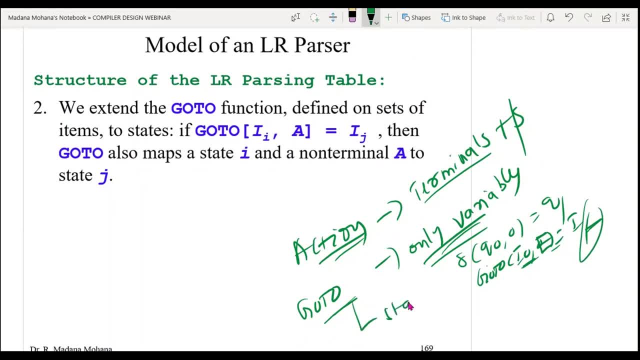 only the state numbers you can enter. goto values are states, then action part, the four values. what we discussed, that is, shift, reduce, accept error. these are all action values, goto values only state number. here you can see goto of ii comma, a equal to ij, only one. 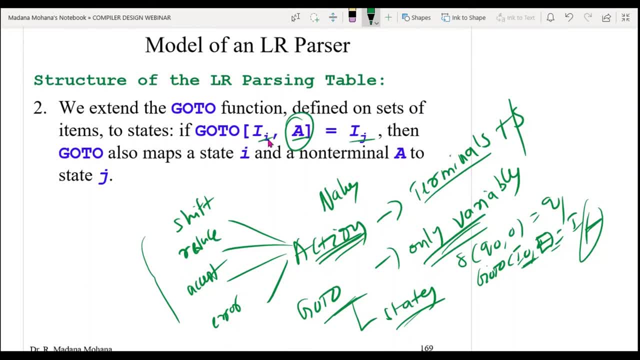 over variable. we have to consider not terminal in the table. that means from item number ii on the variable a it is going to item number j. that means suffix small i is the state i on variable a. it is going to state j. that value you can enter in the table. 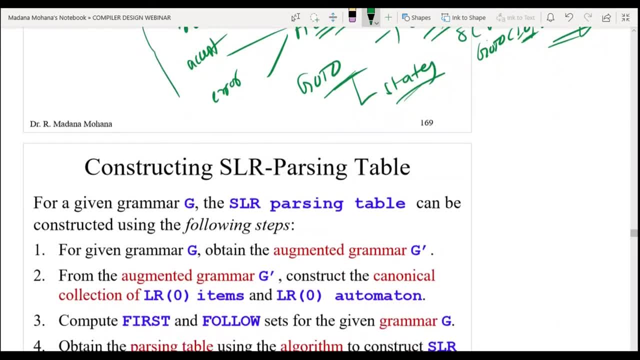 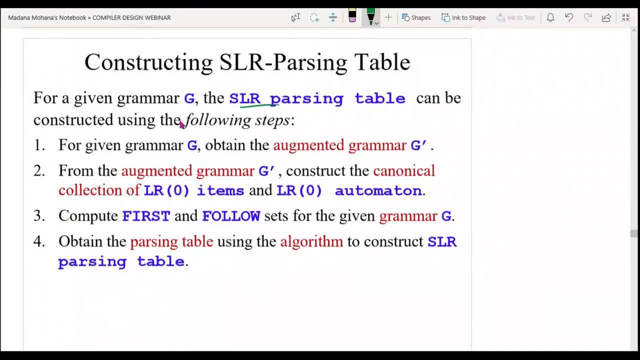 Now see the construction algorithm, then we will see with this LR0 items how to construct the table. Constructing SLR parsing table with the following steps: For the case of SLR parsing table For the given grammar: first, augmented grammar: you need to find out for the augmented grammar. 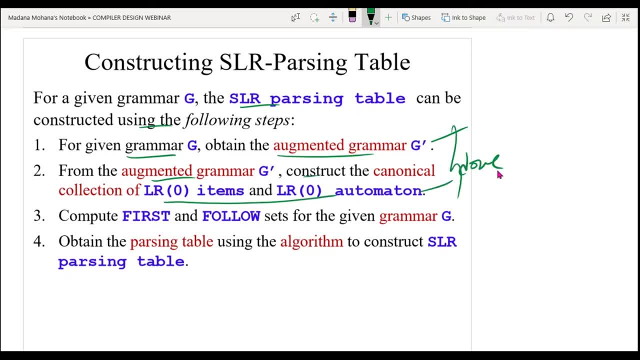 find out LR0 items. these two already done. goto then first and follow also in the predictive parser same process you can use: find out then parsing table using the algorithm. here you can see the fourth. the fourth point only we have to do now to construct SLR parsing. 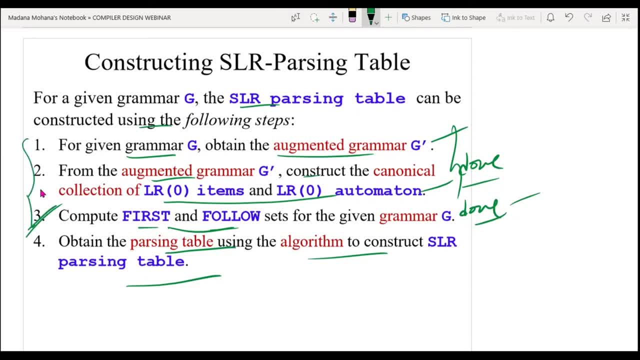 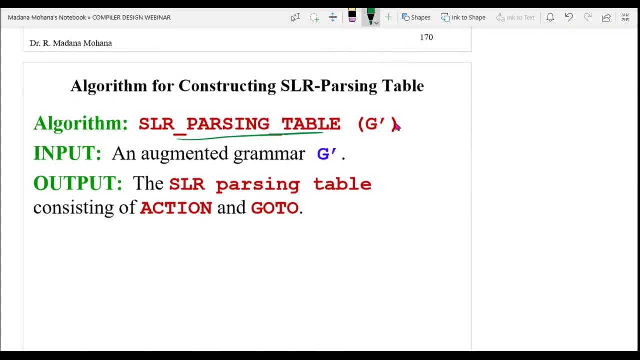 table previous three steps you need to perform. then finally use this one. now you can see the algorithm name: SLR parsing table for augmented grammar, GDEV. this is the input. then output: SLR parsing table with action and goto part. 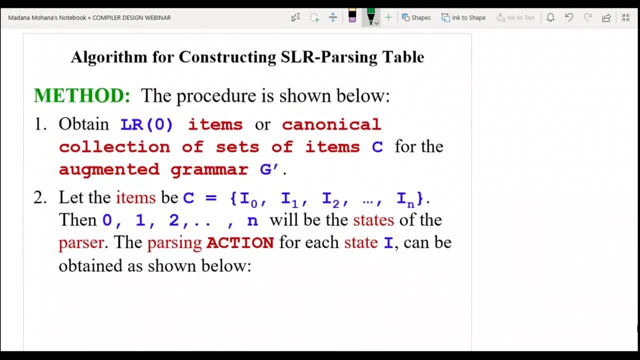 But in the parsing table production number should be from the original grammar, not from augmented grammar, Original grammar without introducing new starting variable. those numbers only we have to do in the reduction values. So first the procedure. step one: obtain LR0 items or canonical collection of sets of items. 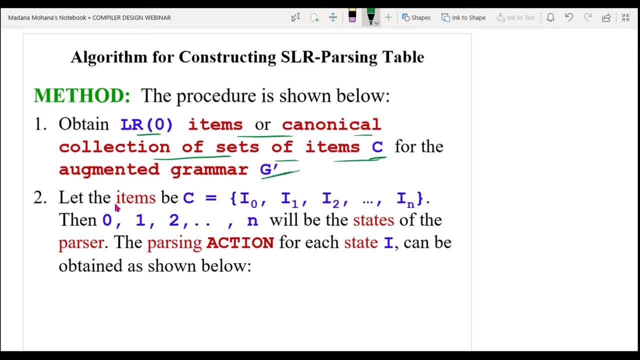 that can be stored in the variable C for the augmented grammar GDEV. let the items be C, equal to I0, I1 and so on IN these are all unique items. previously we got twenty three items. you can take only unique items. now the suffix values 0 to N, 0, 1 to N will 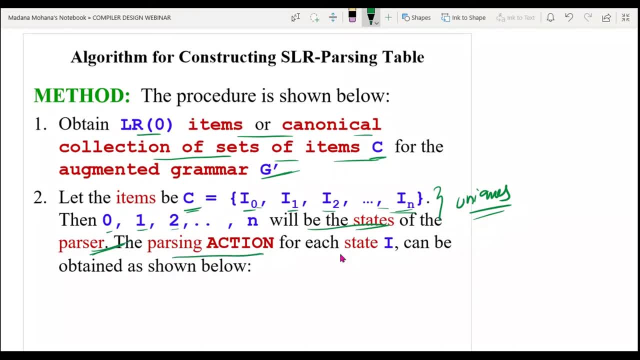 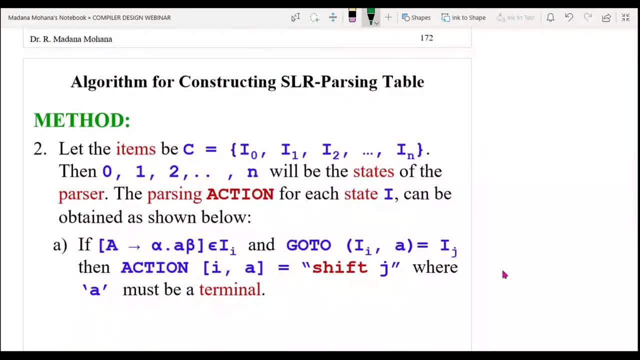 be the states of the parser. the parsing action for each state I can be obtained using the following rules. ok, Now the first rule. If the item is like this: A derives alpha dot terminal. A beta is in some item. number. I I here you can see, after dot, A terminal. is there then goto of I? I means this item. 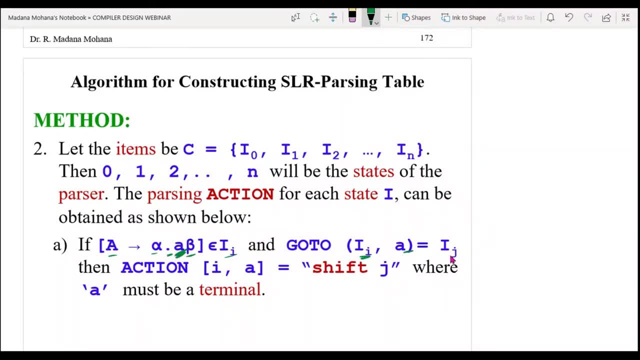 over A terminal A. it is going to which item some I J. now you can see the action value. how to fill carefully. you can observe from this goto function The action value. action of first value is state. second value is terminal or dollar. 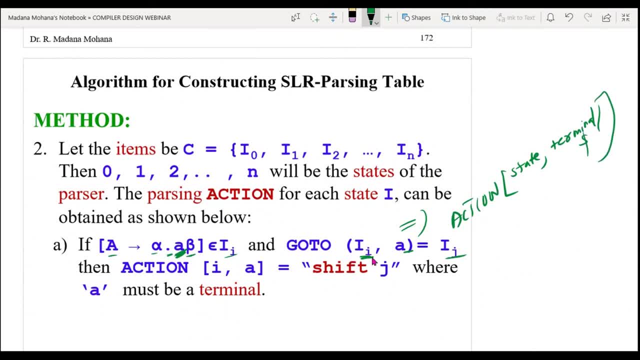 also Now in this: what is the state suffix value I, so action of small i. the terminal is A, here equal to here J. But here, what is this one state I. So here we have state J, state means we have to write shift J, nothing but S suffix J. 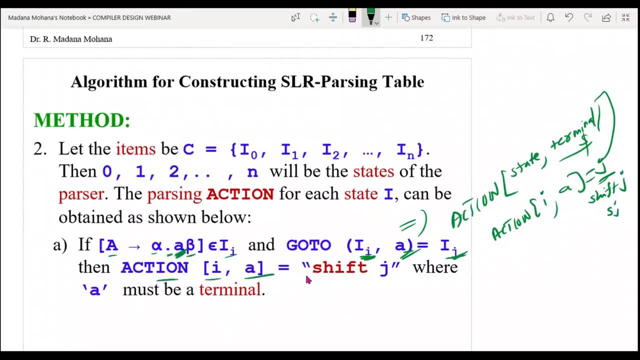 Now in the table let us see action of I on A shift J, where A must be a terminal, here, after dot A terminal. then only you can apply rule second step, first rule For all terminal combinations. you can apply this one here like this: you can fill the: 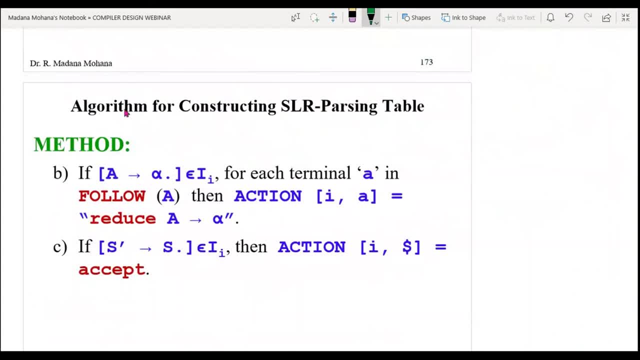 shift values Similarly. next, if item will be completed, item A derives alpha dot after dot, nothing will be. there is in some item number, then you have to find out follow of left hand side variable A. So that value should be. let us do small a, so small a in follow of A. so then action. 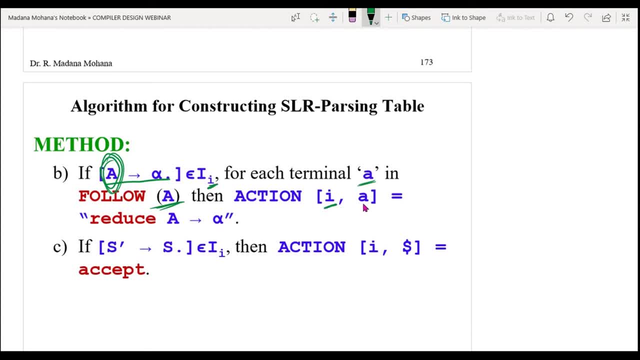 of the state suffix I comma. the terminal follow value equal to. here it is not a state. here we will get reduction For completed item. you will get reduced values. then the items where dot before terminal. you will get shift values. Now, here you can see action of I on terminal A reduced by this production. A derives alpha. 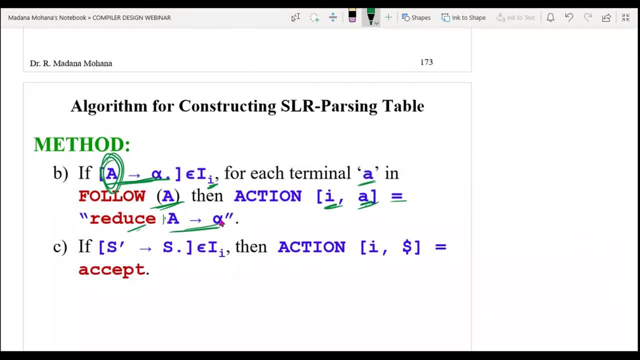 what is the production number actually that number you have to give. for example, this is 1.. So R1 you have to give in the table. that is the reduction value for completed items. So then the rule C in step 2, this is only for special item S, dash zero, S, dot for new. 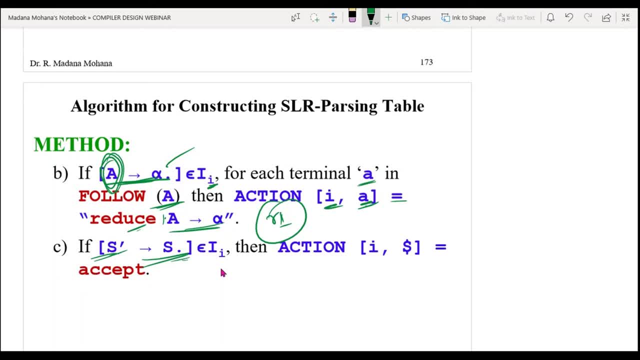 starting variable S dash. completed item is in some item number. Then I on look ahead symbol dollar you can take and do not take follow of S dash, because S dash zero S dot. so that is the default. n marker dollar is added. 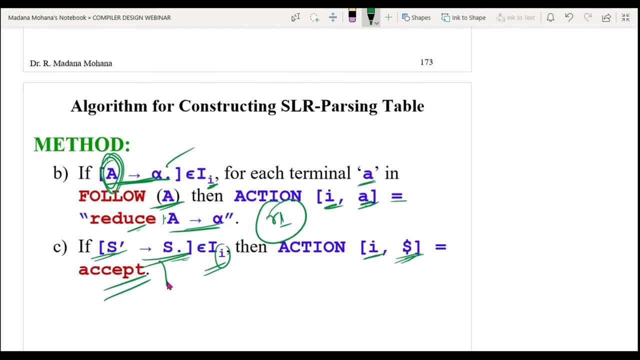 Now action of I comma dollar equal to zero. I comma dollar equal to I dot. so absolutely no trouble. accept for accept only only one time it occurs. this value occurs only in one time, only for this item. completed item that starting variable used for augmented grammar starting variable. 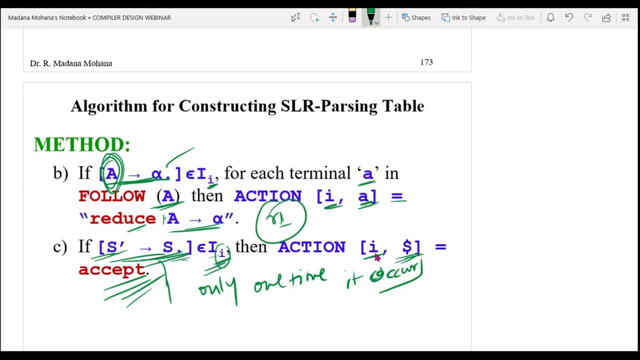 completed item s dash zero s dot. so here suffix i i the look ahead. dollar: default comma. action of i comma. dollar equal to accept. now shift value is over. reduce value is over. now accept value is over. after filling all these three values, all the blank entries, all the blank. 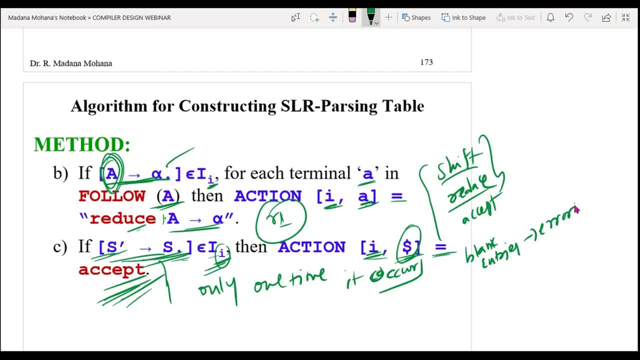 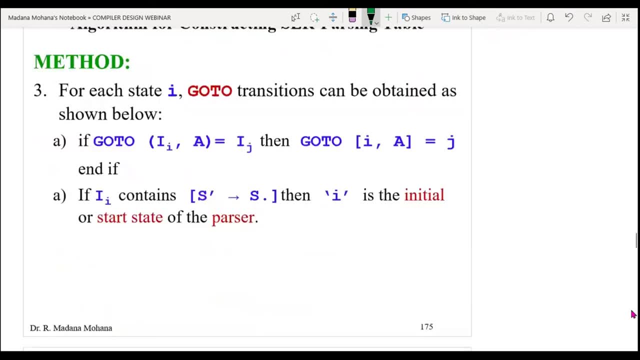 entries nothing but error. but specifically we won't mention error. we will keep it as blank only by default. blank means that denotes error only that is action part. then how to fill: go to part. just now i already explained: go to part starting. go to a transition like delta function. so 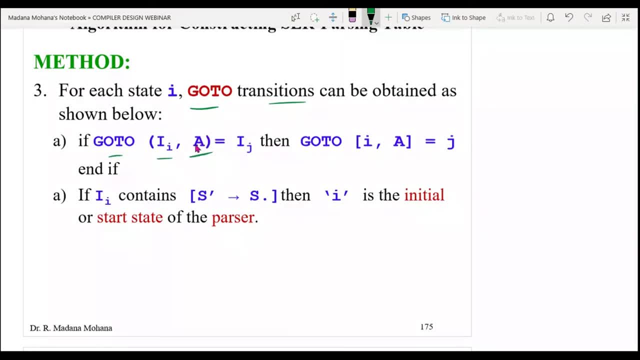 go to of i i comma variable for go to values. you can take only variable, not terminal combination. so go to of i i comma. a equal to i j, nothing but the suffix state i. on variable a. here you can see in the go to part: go to part only variables. it includes not terminals or look. 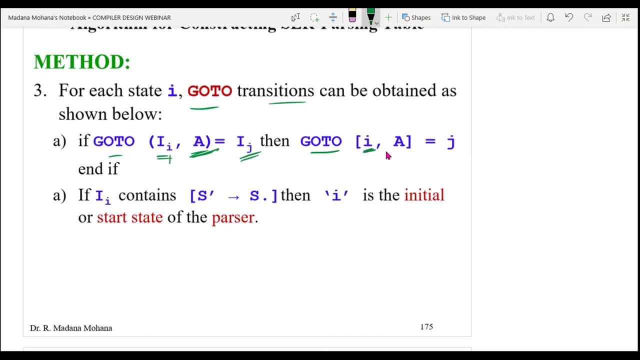 ahead. so now from i, from state i on variable a, the next state is j. so here don't use shift. j reduce accept only j, only you can include. for example, you are having the item like this: so go to of i, not on e, equal to some i one now in the table. 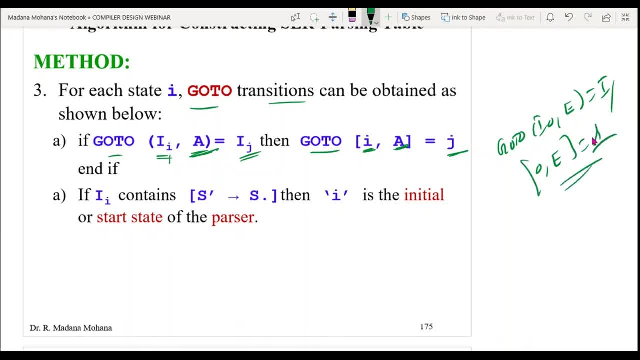 zero on e you can include the one only. don't include shift reduce, accept error only state number, suffix value only you can include in the go to part. so now a special item. if ii contains s dash zero s dot, then i is the initial or start state of the parser in the dfe of: 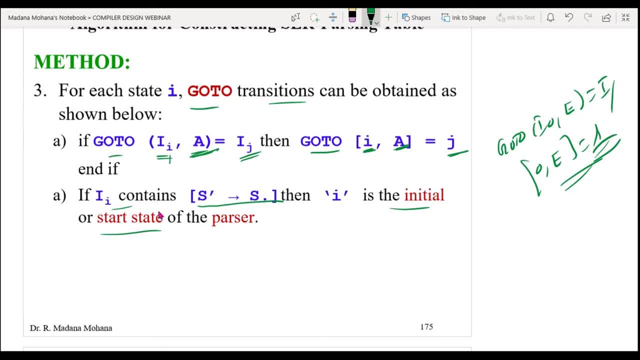 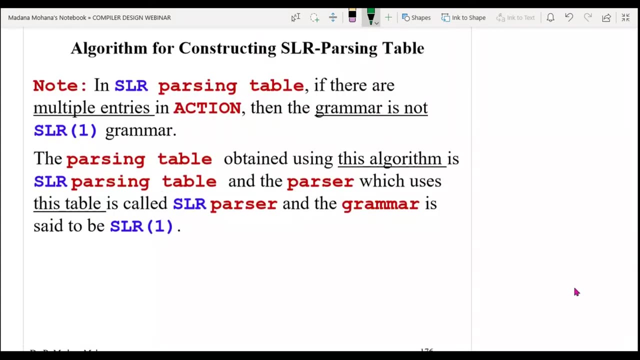 l? r zero items. we already discussed so how to identify the initial statement. if any item contains s dash, zero, s dot in a particular item number, then that will be treated as the initial or start state of the parser. ok, now, after constructing the slr parsing table: same. 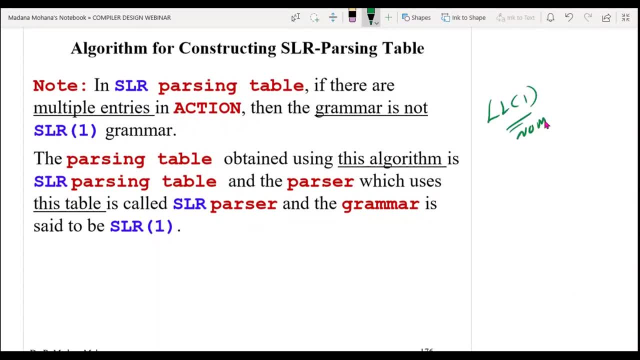 as ll one. no multiple entries in the parsing table. so now, after constructing the slr parsing table, no multiple entries in predictive parser, predictive parsing table. then that is ll one grammar or parser. similar rule applied for all the l r parsers in slr parsing table. if there are multiple entries in the action part, here you can consider only action part. 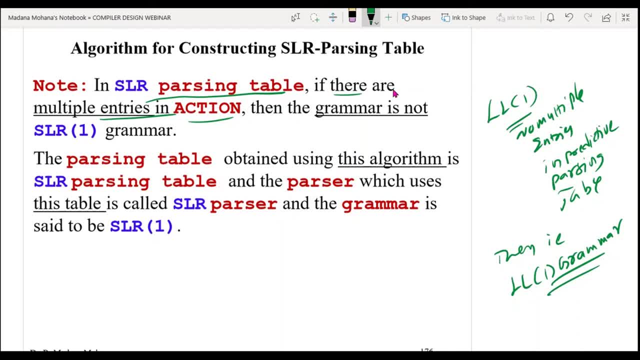 in the predictive parser we don't have a separate category, common values only. but in the l? r parsing two parts- action part- go to part in the action part. if there are multiple entries then the grammar is not slr one grammar if no multiple entries in the action part. 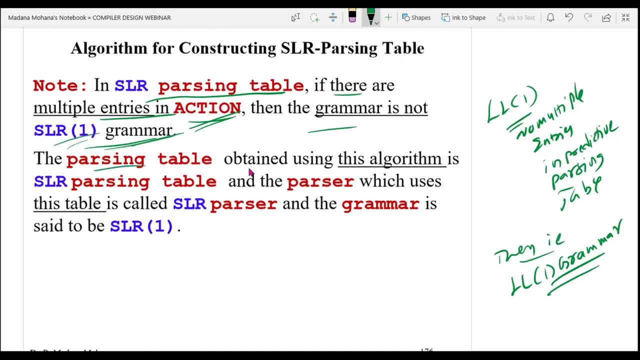 then that is called as slr parser and slr one grammar. the parsing table obtained using this algorithm is slr parsing table and the parser which uses this table slr parser. the grammar is said to be slr one parser, but if the table is not here, then the grammar is: 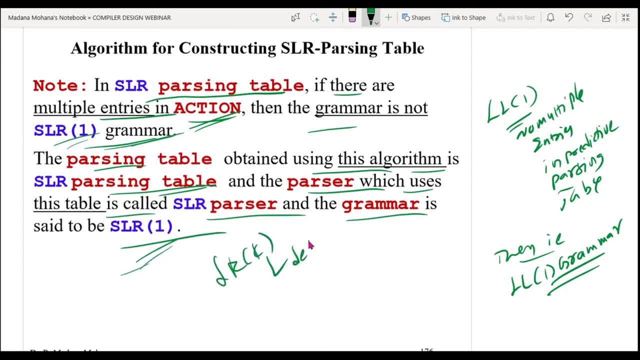 one parser. so how to identify the slr two category of letters is called one parsers default. so LRK default value is 1. default is 1. that means SLR 1 parser. CLR 1 parser. LALR 1 parser. similar definition applicable here: SLR parser. SLR parsing table. CLR parser. 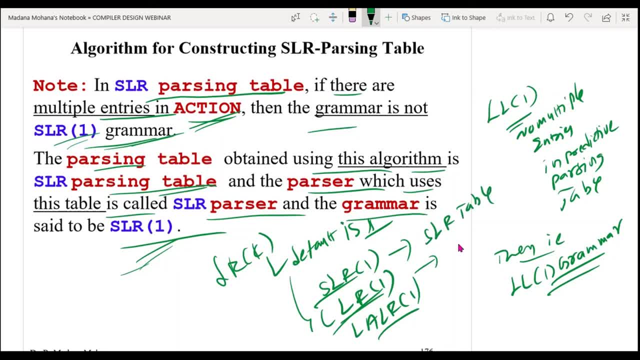 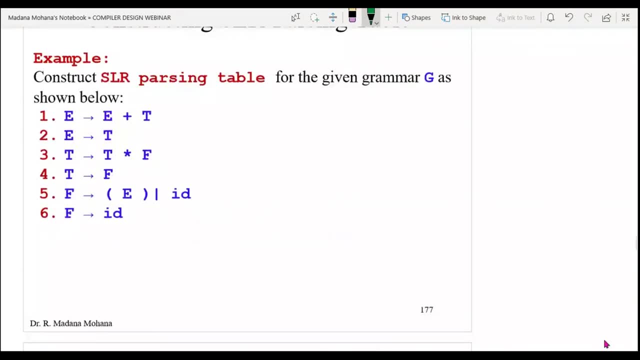 CLR parsing table. only the respective tables needs to be considered. LALR parser. LALR table needs to be considered now using this algorithm for this problem, let us see how to construct the table, so the question will be given in examination. like this: construct SLR parsing? 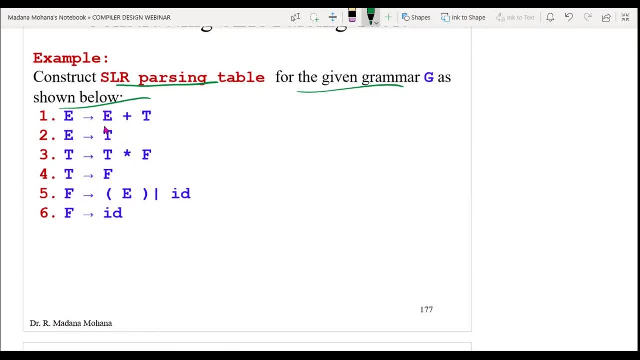 table for the given grammar directly. if you can see the starting variable doesn't occur anywhere in the right hand side, This means you can consider it as the augmented grammar. if at least one production in the right hand side starting variable occurred, then you can convert into augmented grammar. 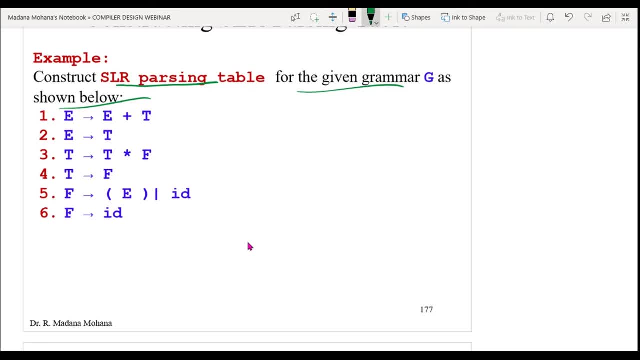 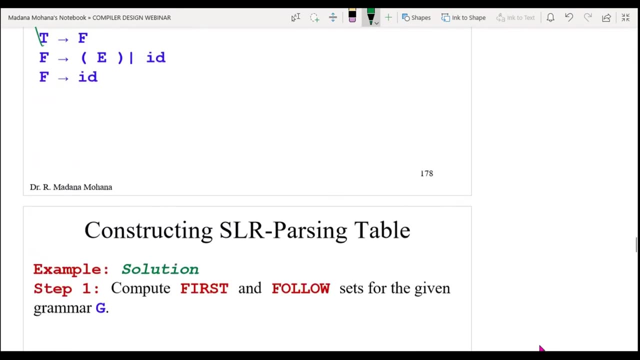 then that is not augmented grammar. now, here you can see, this is not augmented grammar. E occurred here, right hand side, first production, then F production also. so for this we already augmented grammar is constructed G dash by introducing new starting variable. then LR0 items are constructed. 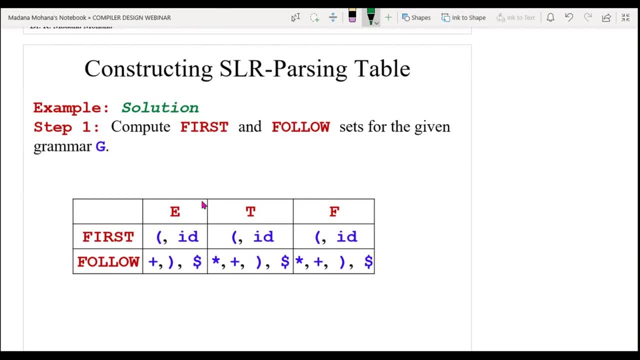 So here first and follow values you can find first of E, T, F. so this is even here. left recursion is there, because in bottom of parser we don't have restriction of. if it is not, I mean no left recursion, not ambiguity, I mean ambiguous, no restriction. so even whatever the given, 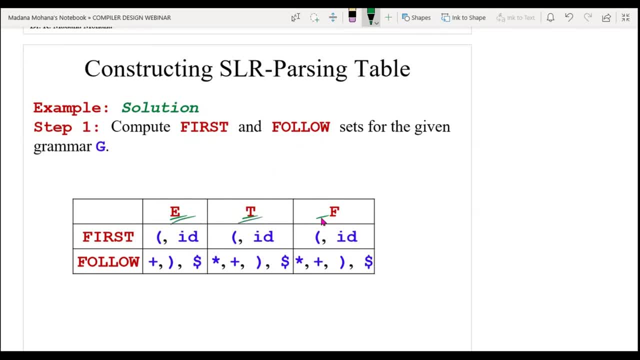 grammar. even having left recursion you can find out first and follow value only in predictive parser. we have to stick on the limitations of top down parsing. it doesn't aloud left recursion, then ambiguity, all you have to remove. but in bottom of parser there is no such restriction. 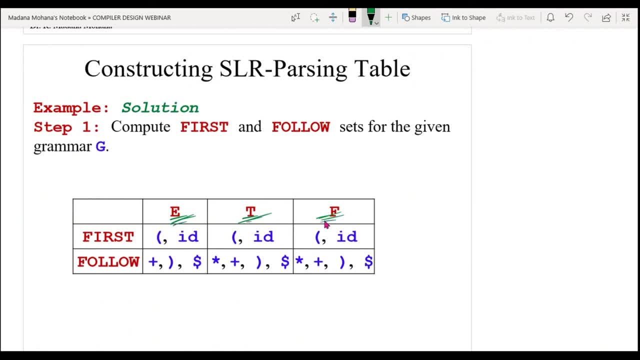 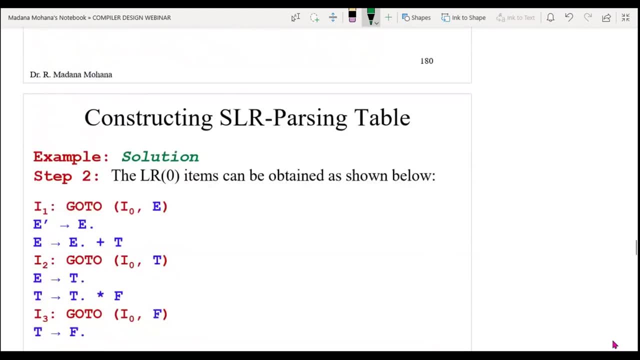 directly. we are finding first and follow values, E, T, F. so, first values, follow values, using the same rules. ok, now let us come to the LR0 items: I00, I22- we already constructed. now, from I0 to I22, we constructed the 1st filled with I0, we have already constructed. 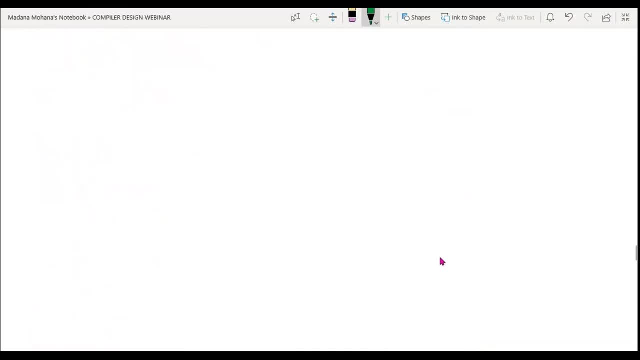 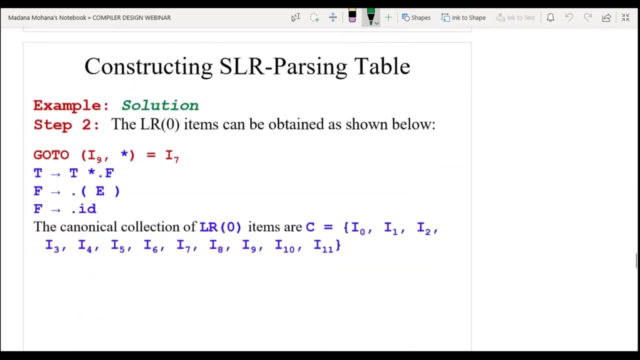 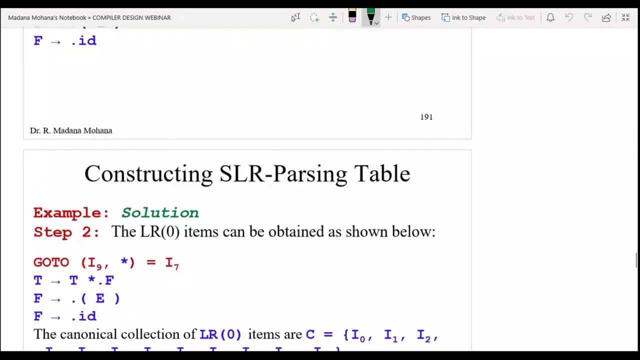 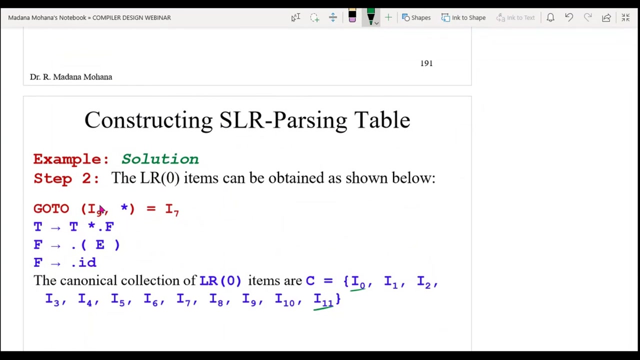 So that is already constructed. 22, the same I have listed here by repeating duplications. let us see the unique items by removing the duplicates here. you can see here we have listed: I naught to I: 11. 12 unique items are there from I naught to I: 22 after duplicate items removed. duplicate items removed. 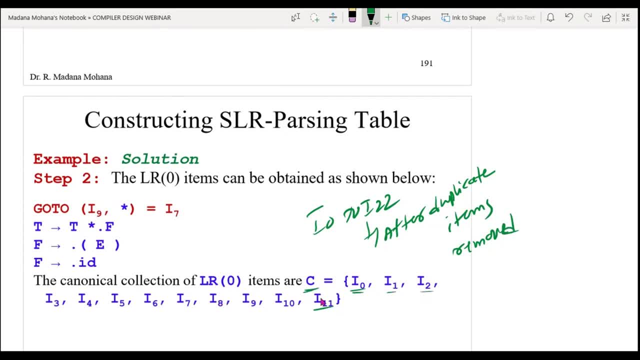 the unique items are stored in C. I naught I 1, I 2 and so on. I 11. now 0, 1, 2, 3 and so on. 11 are states of SLR parser. So this is the state of SLR parser. 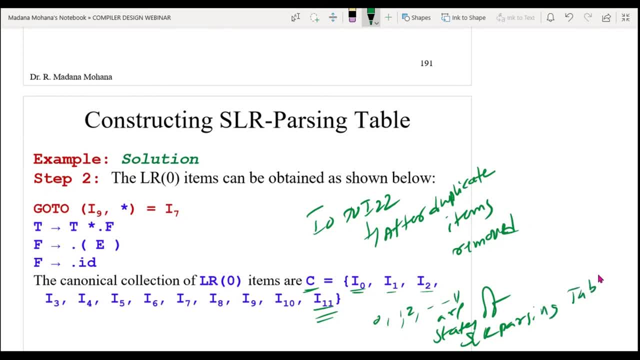 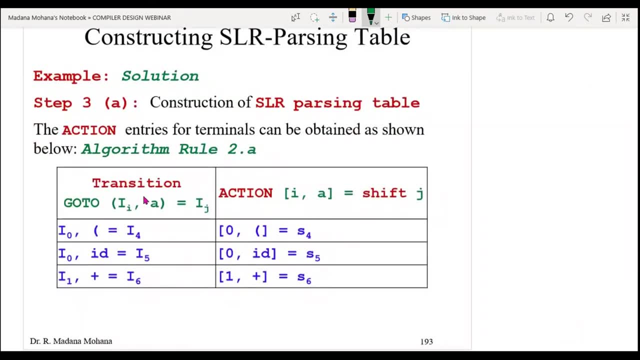 SLR parsing table. now the rules. now we will apply here 1 by 1. first step to rule A: if you are having goto function like this: goto of I I, comma A equal to I, J, that is dot is placed before terminal, then that is going to a particular item. then action of the suffix. 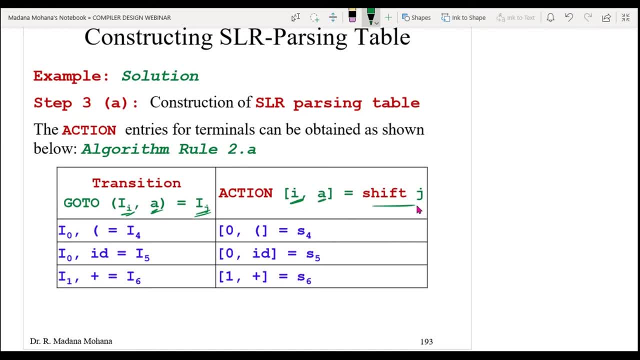 I comma the terminal A equal to shift J. Now we are having over terminal combination. only you can consider not variable here. A should be a terminal. now all the goto values we have taken like this direct values here already function is there goto of. I naught on left parenthesis it is going to I 4.. 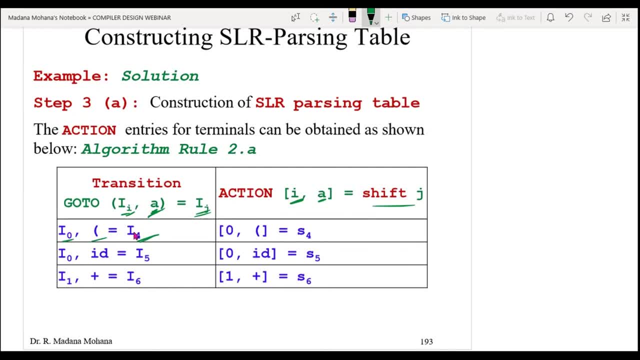 Now in the table, action of 0 comma left parenthesis equal to shift 4 means this is nothing but shift 4. that can be written in short form: S 4, 0 on left parenthesis. then I naught on I, D, I, 5.. 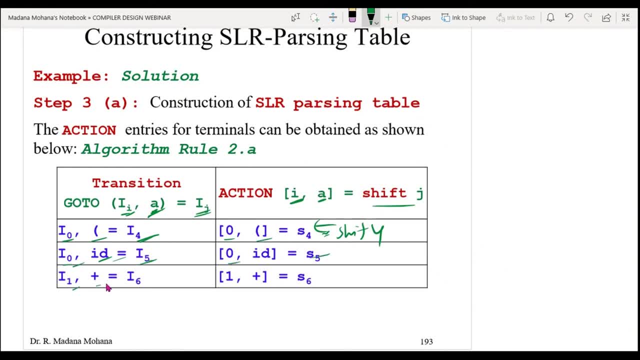 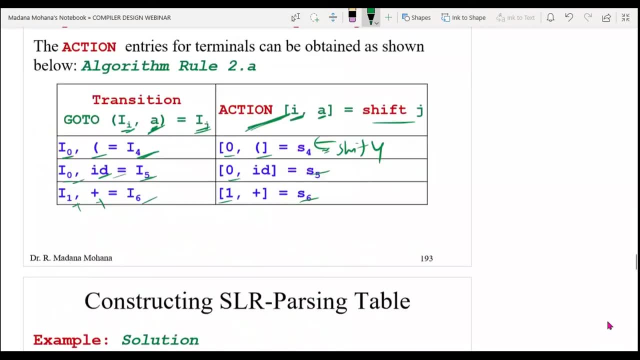 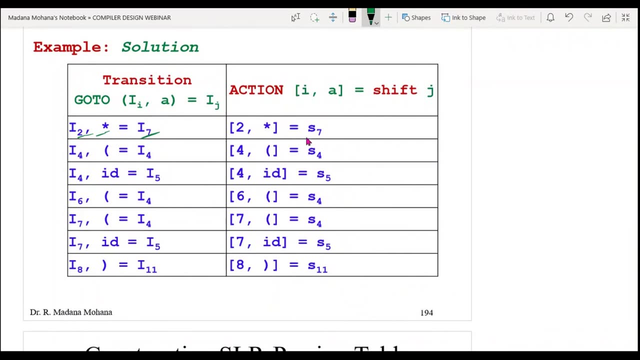 0, I D, equal to S 5. then I- I 1 on place I 6. 1 on place equal to S 6. these are all action values. we are filling action part of the table over terminal combination. first we are taking: then I- 2 on star- I 7. then 2 on star, equal to S 7, then 4, I 4 on left parenthesis: I 4. 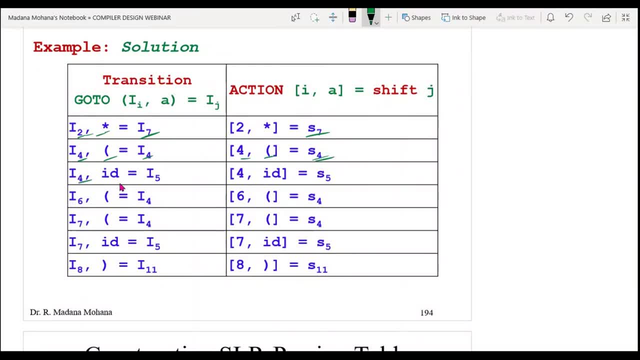 loop 4 on left parenthesis, S 4 then I 4 on I D, I 5- 4 on I D, S 5 then I 6 on left parenthesis. I 4- 6 on left parenthesis, S 5 then I 6 on left parenthesis. I 4- 6 on left parenthesis. 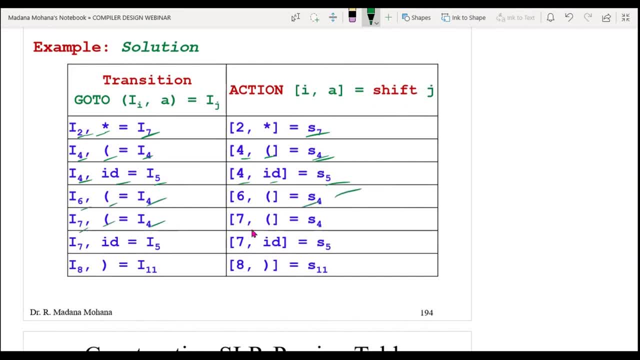 I, 4.. Then I, 7 on left parenthesis I 4. 7 on left parenthesis, S 4. see here even repeated items also. we have to consider here: so why? because in the automaton also self states occurred on particular input going to the same state. but item number should be unique, repeated. 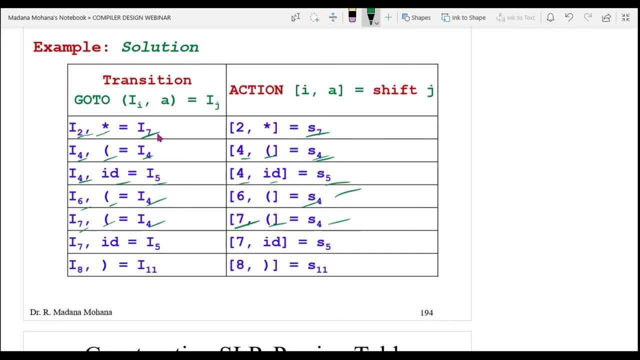 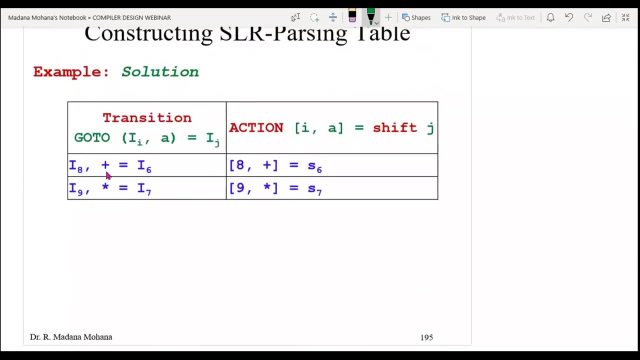 items without state number. whatever the repeated item number, that item we will take now similar I 7 on I D, I 5.. 7 on I D, S 5, 8 on right parenthesis, S 11. then similarly I 8. on place we are having 6, 8 on. 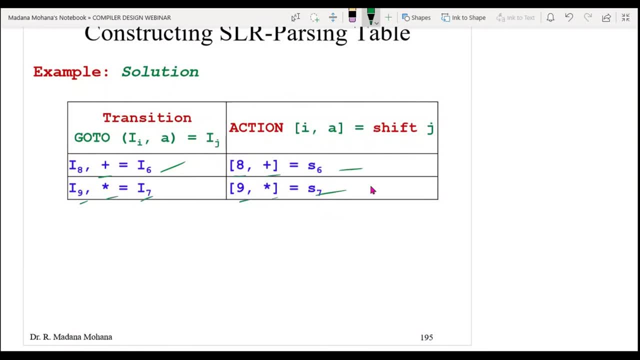 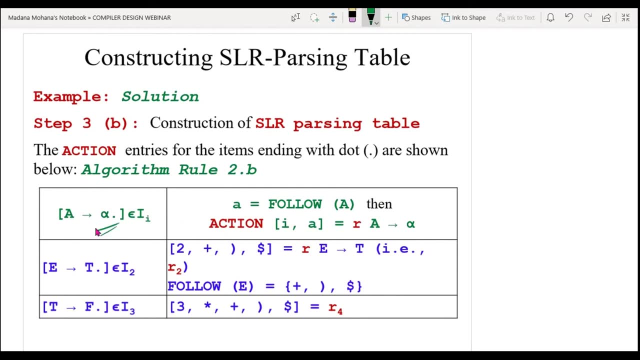 place S 6 I. 9 on star I 7. 9 on star S 7. that is rule 2 A. then coming to 2 B: 2 B is applicable for only completed item wherever dot will be in the right end in any item. for all you. 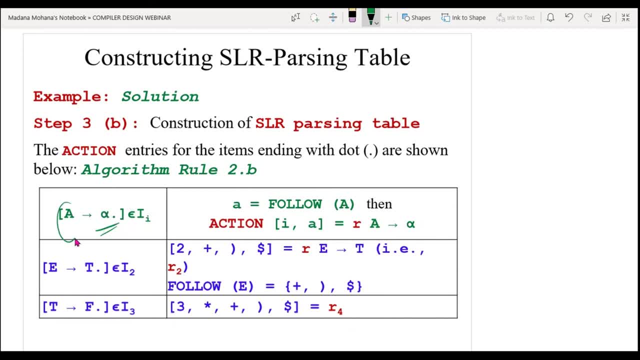 can apply rule 2 B. Now here what you have to do: fall of a: we have to find out here you can see, small a equal to fall of a. whatever a is not a single value. even you will get more than one value also. 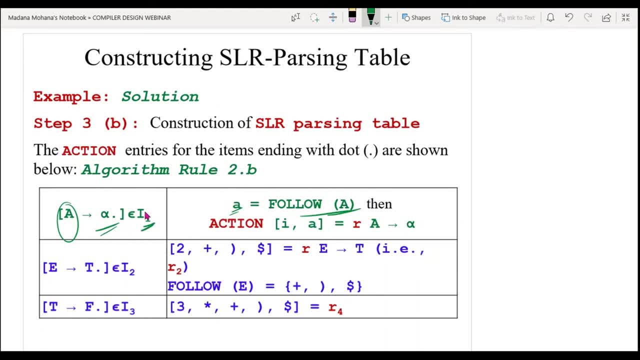 So a equal to fall of a. then what you have to do, whatever the item number, suffix: i, small i. action of i comma. the follow values: the same value. action of i on follow value. a equal to reduced for completed item. only reduced values will be generated, reduced by the production. 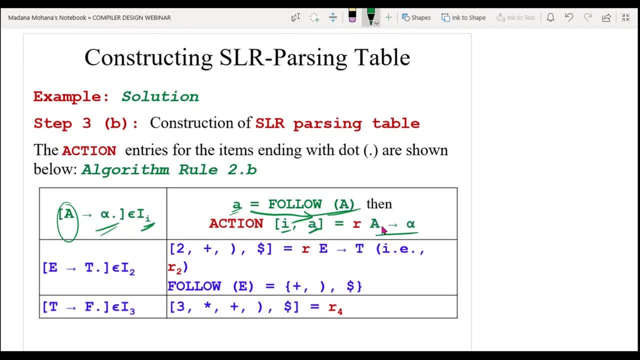 number name we have mentioned, but the table we can give the numbering of the production. the numbering will be given from the original grammar. that is not for augmented grammar. you are given original grammar by default. the original grammar itself is augmented grammar. then you can give the production numbers for the same if the given grammar is not augmented. 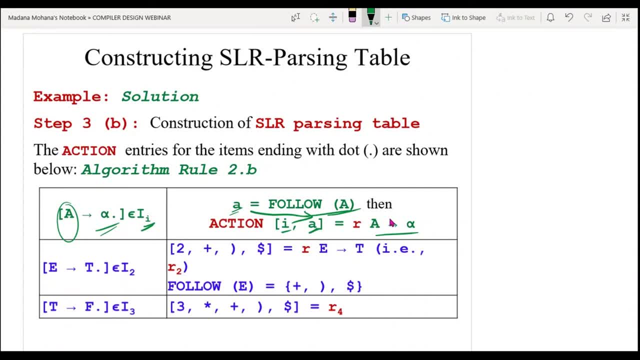 grammar. you need to find out new grammar by introducing new starting variable. but production numbers you can consider only for original grammar. Now here you can see The first completed item. e derives t dot in i2 item in i2. it is there in the above from. 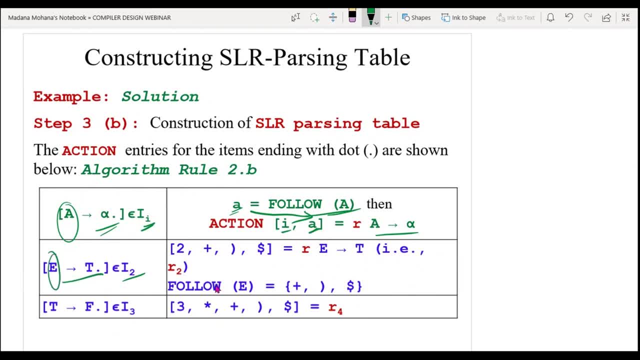 above. we are doing this one now fall of e. you can find out fall of e also. we listed plus right parenthesis dollar. now the action entry with the same state to on place on right parenthesis on dollar from the state. with three different terminals, the same production we can use. reduce e d e. e derives t. 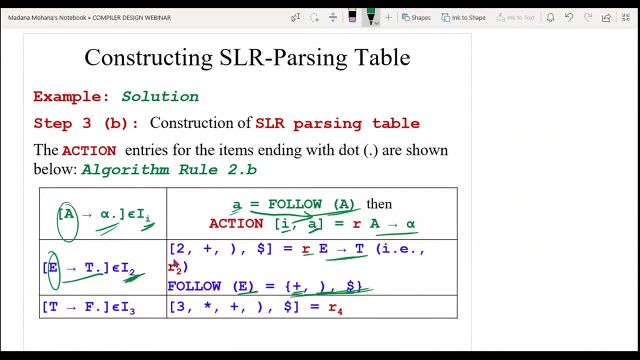 So this is what we have to do Now. you can see in the action, part two, state. this is state. then the terminal values including: look at two on place r: e derives t. two on right parenthesis: same production. two on dollar: same production. So e derives t. what is the production number? actually you are given original grammar e. 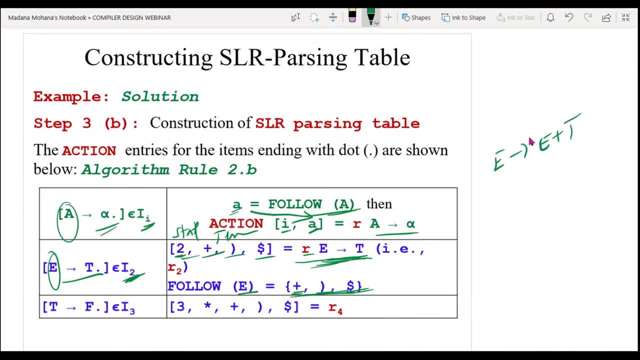 e derives t plus t, then e derives t, t derives t into f, t derives f. take all the production separately, even starting with same variable, also separately. you can list of the production numbers: one, two, three, four, five, six. now you can see e derives t. what is the number two? so r two is used here, r two similarly. 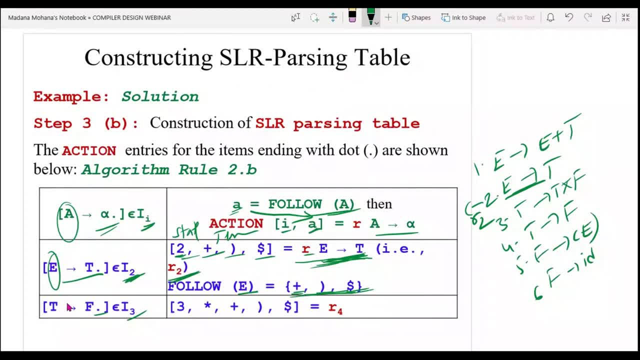 next, t derives f dot. e is in i3 item. what is fall of t to fall of t, equal to a. Similarly, next, t derives f dot using i3 item. what is follow of t? to follow of t equals equal to star plus right parenthesis dollar. now three on plus three on into three on plus. 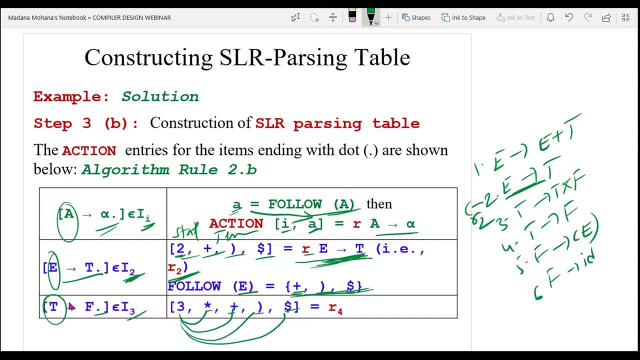 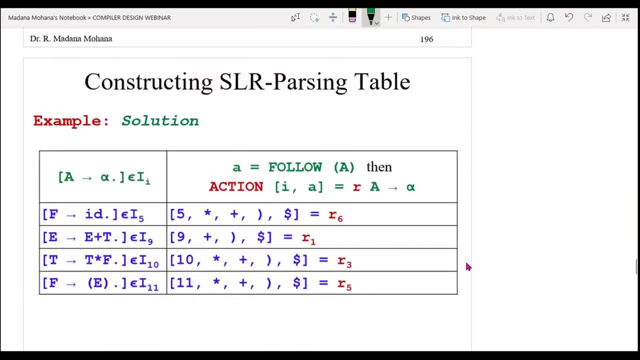 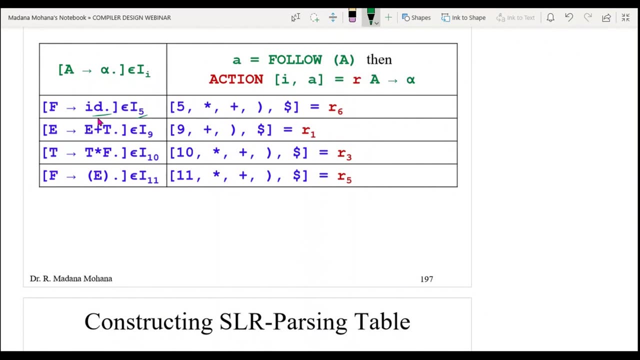 three on right parenthesis, three on dollar. so what is the production here? t derives f, t derives f equal to fourth production. so r4 you can use like this for all completed items. you can take the reduced values similarly. f derives id. dot is in i5 now fall of f plus. 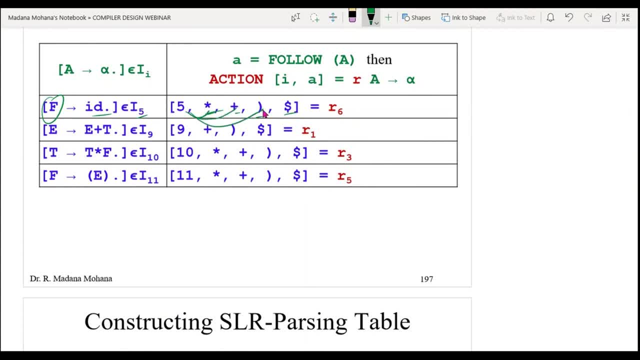 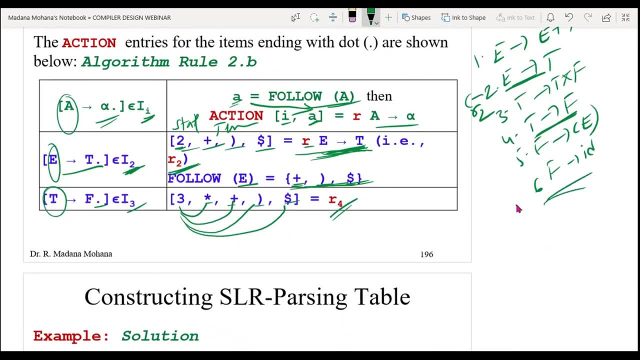 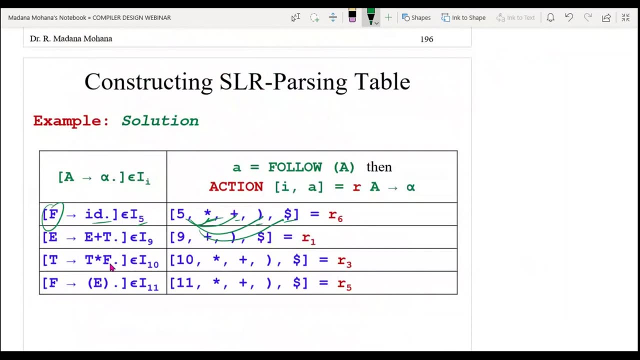 star plus, right parenthesis, dollar. five, one star. five. one plus five. one right parenthesis: five, one dollar by the production: f derives id. f derives id. what is the number six? production. so r6 you can take. so like this, you can fill all the reduction values similarly: e plus. 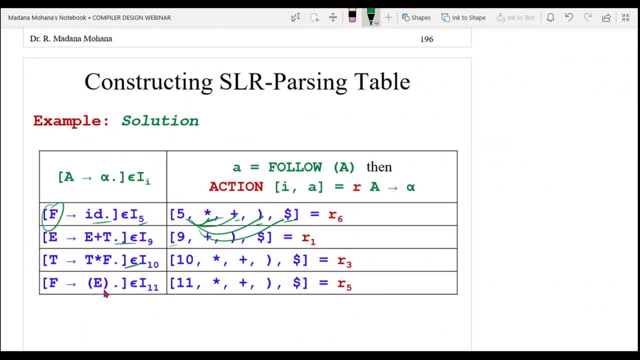 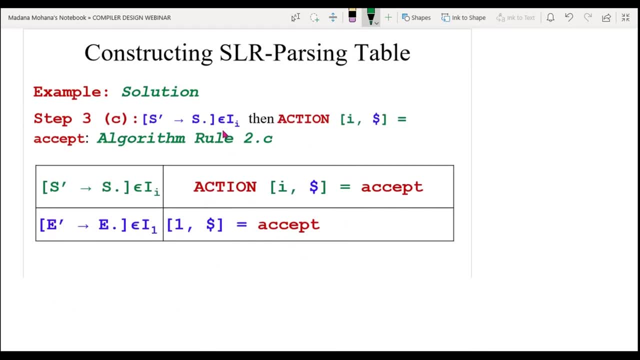 t dot, then t, derives t dot, f dot, then t, right parenthesis dot, like so all the reduction values you can fill. Then, coming to two c, The two c rule: only for one item we will get, that is for special item s dot, derives s dot. 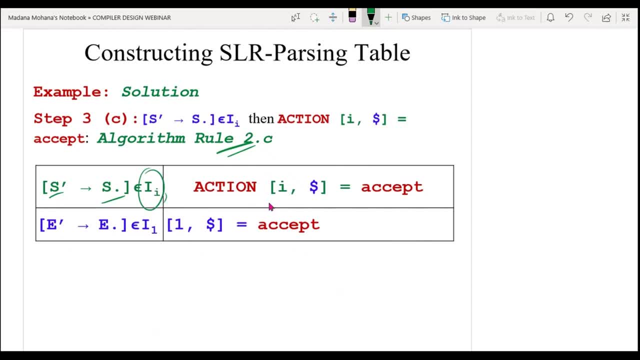 is in some item number, then this item number comma dollar. the two c rule we already discussed. action of i comma dollar equal to accept. this will occur only one time only for this item will occur only one time now in our items e dash derives, e dot is in some i1, now one. 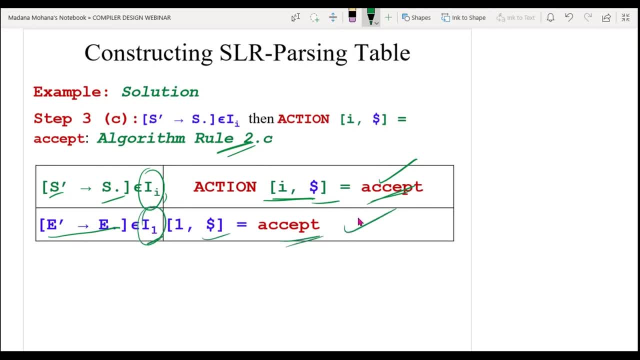 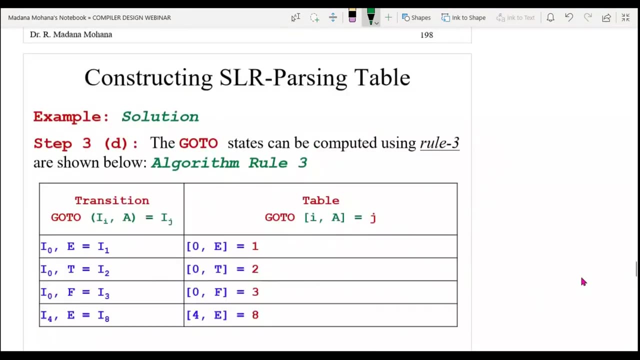 on dollar equal to accept. Now shift value is over, reduce value is over accept value is over, then all blanks denotes error. these are all only action values till now. what we constructed- only action values then- coming to go to that- is direct delta function. i alert explained previously the 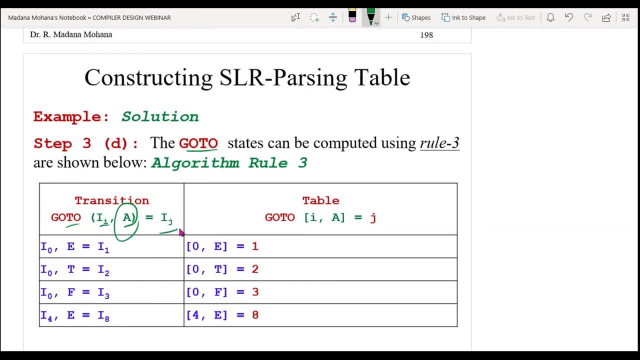 go to rule, go to of i i comma, variable, only variable you have to take equal to i j. then from state i, variable a, the next state is j, Only state number is j. So i j is equal to i j. So i j is equal to i j. 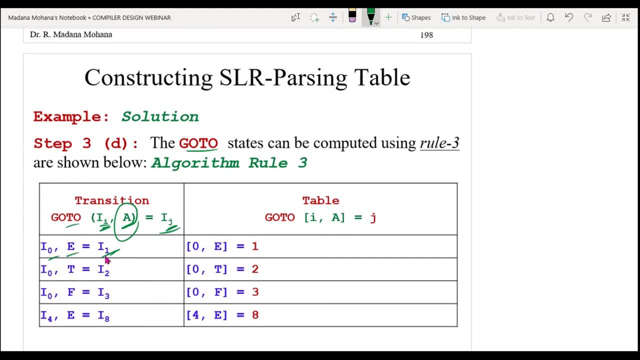 Other way you can give. now. i naught on e: it is going to i1. then zero on e equal to 1. then i naught on t: it is going to i2. zero on e equal to 2. i naught on f: it is going to i3. 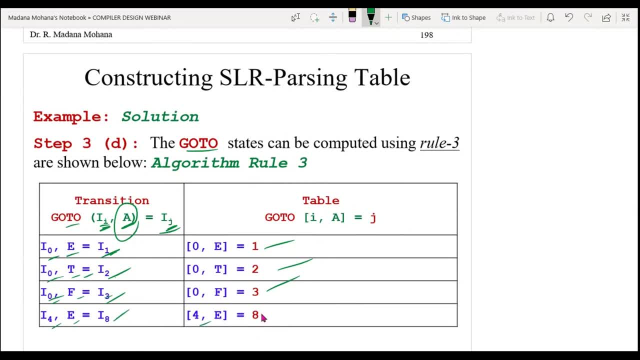 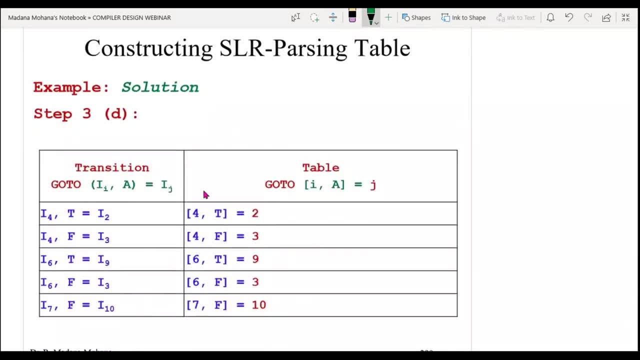 zero on f, equal to 3, then i, 4 on e, it is going to i8, 4 on e, equal to 8.. Here only you are getting single state values. like for all variable combination go to function. then i4 on t, i2, then i4 on f, i3 and so on: i7, f, i10. 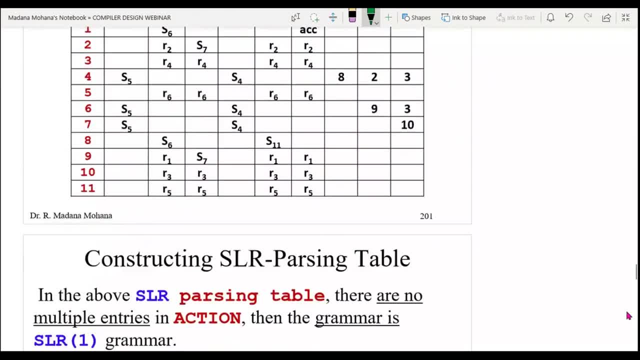 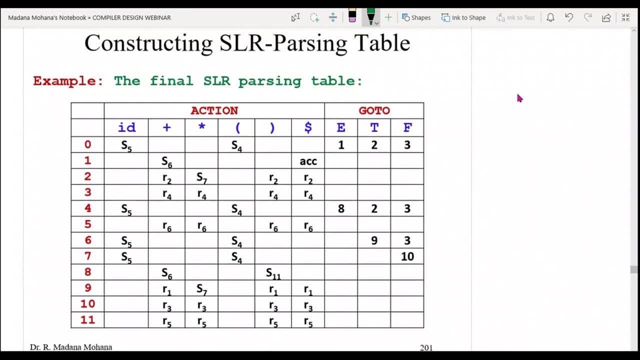 Now you can see after finding all the action, and go to values. now you can construct the table by entering those values. This is the structure of SLR parsing table. We already mentioned action part only terminals, including dollar. Go to part only variables in the original grammar, not augmented grammar. 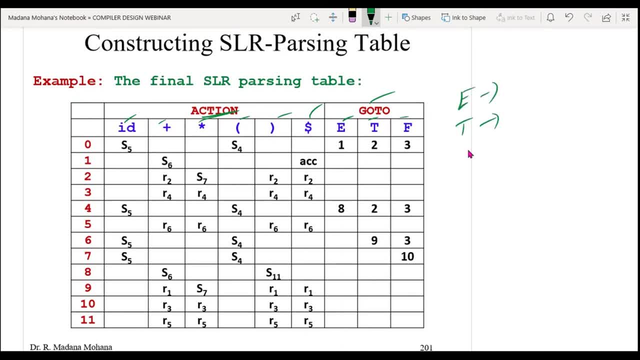 Your original grammar contains E, contains T, contains F. Only three variables. So E, T, F. Now all the states are. see, we assumed unique items I0 and so on, I11.. The suffix values 0,, 1,, 2 and so on, 11 are the states here. 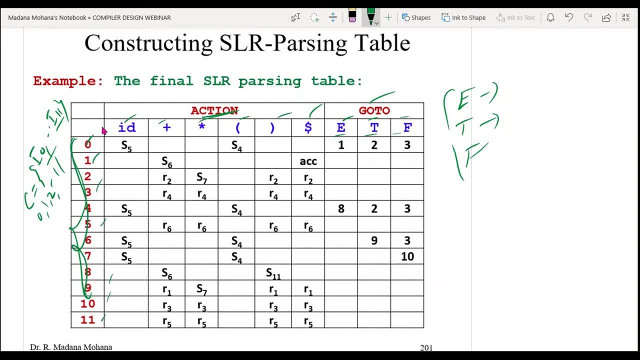 Here you can see 0,, 1,, 2, 3.. These are all unique. Now, just now we calculated action, value 0 and ID and so on. Then go to values. also we calculated. Here you can see Accept occurred only one case. 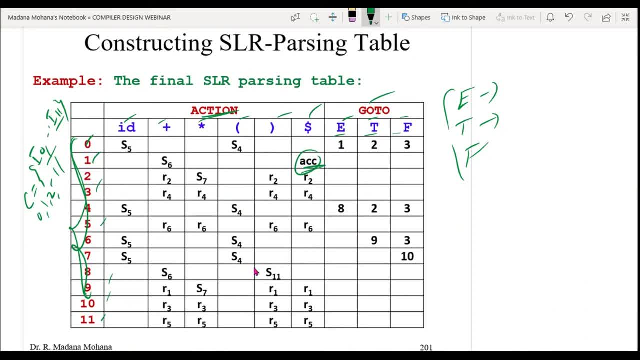 Only one place it should be occurred. Then shift values, Then reduce values are there, Then go to values, only state numbers, Then all the blanks, all the blanks. error in the action part. Why? Because for parsing action we will take only action part values. 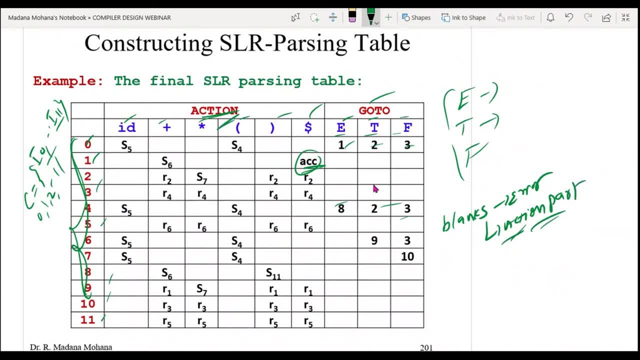 Action part Go to also wherever blank, but error only. but this we will neglect, Only action error we will consider. So this is the SLR parsing table. Now check out: is there any multiple entry? Even combination of shift, reduce value also more than one value. 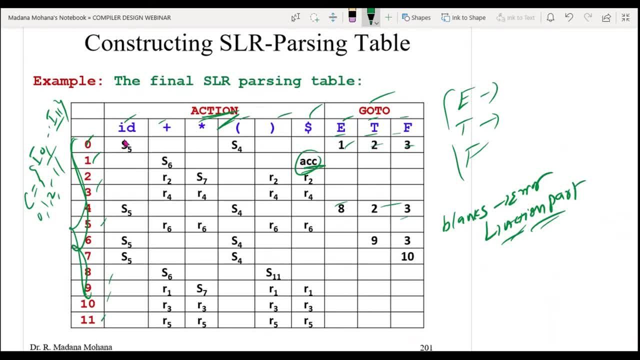 Even different values, also more than one entry in one particular entry. So here all our single values are there. All our single values are blank values only. So here no multiple entries. So this is SLR one parser, SLR one parser. Then, whatever the grammar we used, that is called a SLR one grammar in the above SLR parsing. 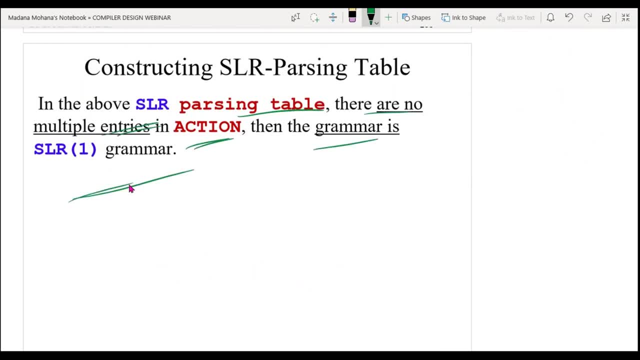 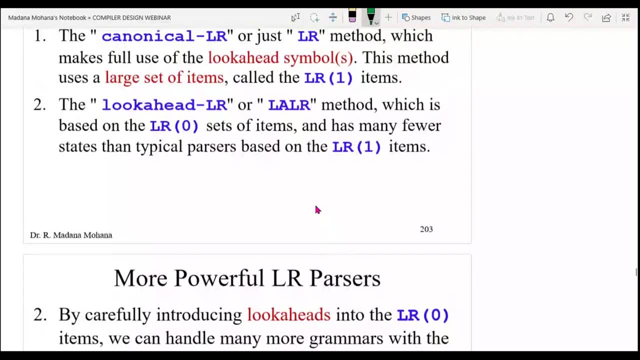 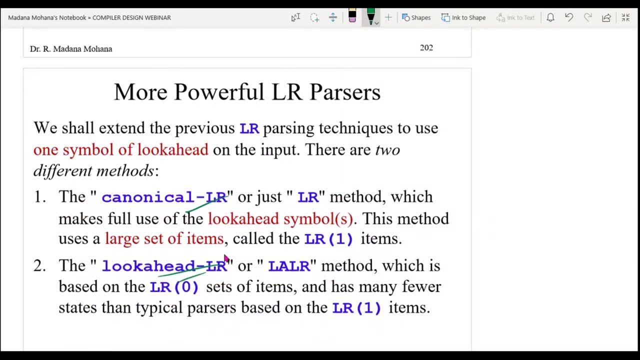 table. There are no multiple entries in the action part. Therefore the grammar is SLR one grammar. So that is the SLR one parser. They are coming to more powerful LR parsers since once we know CLR parser, LALR is very simple with this, only some modification. 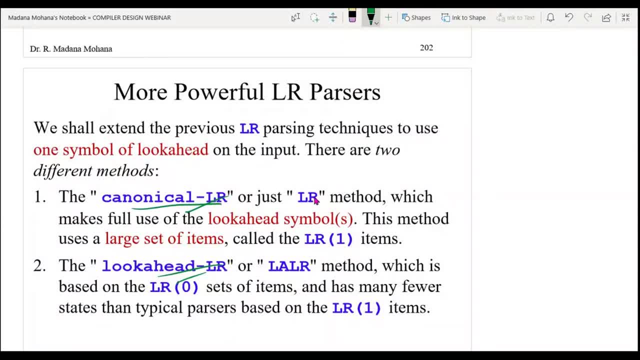 First canonical LR is one of the powerful LR parser. Just LR also will call It makes full use of lookahead symbol. Here one symbol is used: K. This method uses large set of items called LR one item. This is new How to construct LR one items. 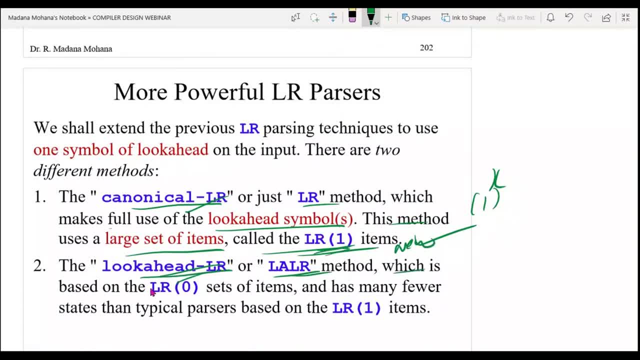 We will see Then lookahead LR or LALR, which is based on LR zero sets of items and may have fewer states in the typical parser based on LR one items, But here we will use LR one items only for this. Based on this, we will take LR one items. 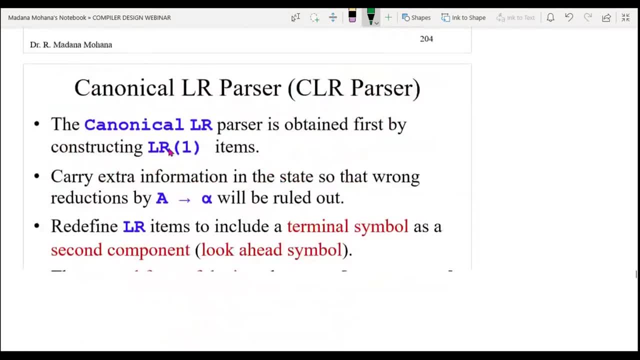 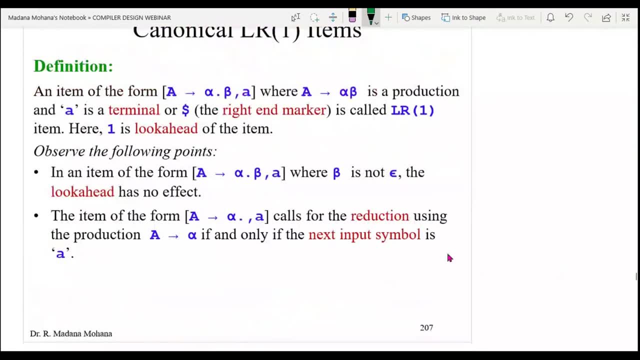 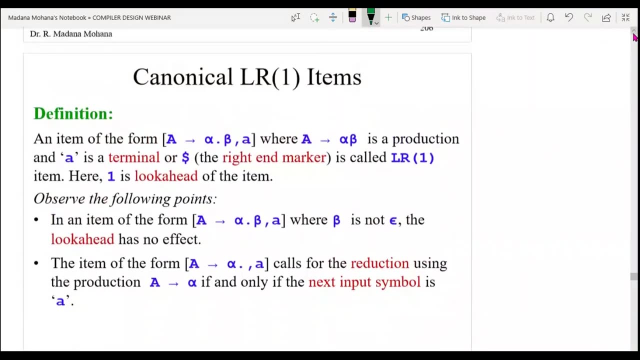 Now how to construct LR one items. Let us see here The algorithm. everything is same here, So how to construct LR one items. Let us see here So how to define LR one item, LR- zero items. whatever the methodology we use to do everything same, the only difference. 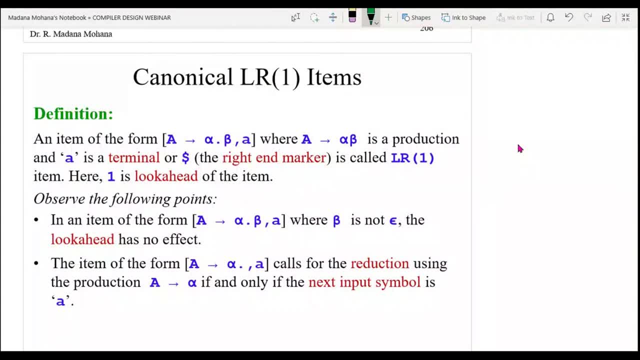 here one extra lookahead symbol will come, will be added. that is the only difference. Here you can see an item of the form A derived alpha dot beta comma a small a. So here A derived alpha beta is a production, small a is a terminal or dollar. 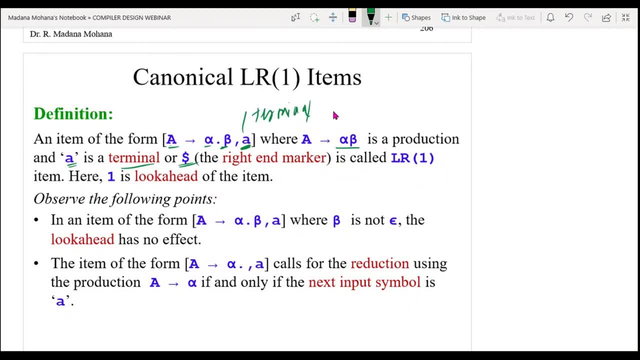 This one, Easy, It is a terminal or dollar. Dollar means right end marker. This is called as LR: one item Here one is the lookahead of the item. So here also, same as closer go to same as LR: zero items, But lookahead symbol. 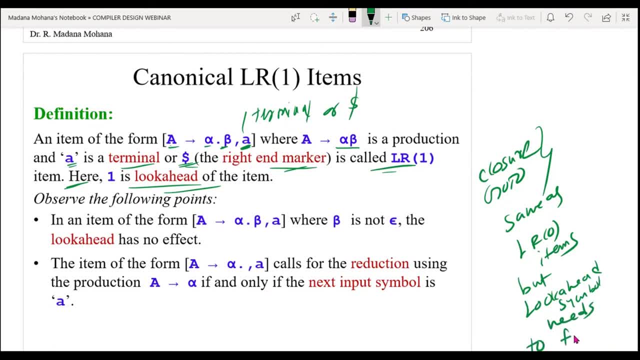 Needs to find for every item. This is a new, actually Remaining all are same. Then, how to find the lookahead symbol for every item? That is the thing we have to concentrate. So, in an item of the form A, derived alpha, dot, beta, comma a where beta is not null, this 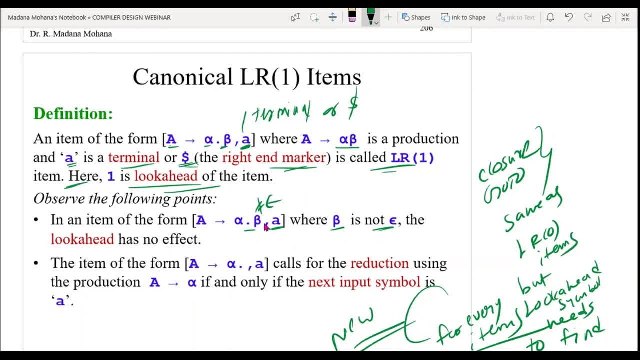 is not null, Then the lookahead has no effect. Why? Because if it is not null means no use of this. If it is null, then only this will be used. Now, if the item is of the form A derived alpha, dot after dot, beta is null here. 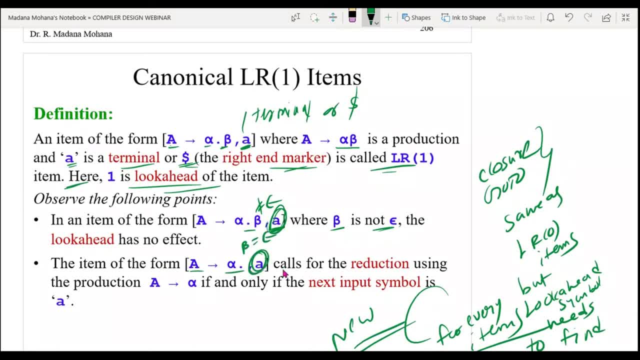 So then A impact is used here. So then call for the reduction using the production A derived alpha if, and only if, the next input symbol is A This one, That is, the use of lookahead symbol here. Now the closer function, everything is same. 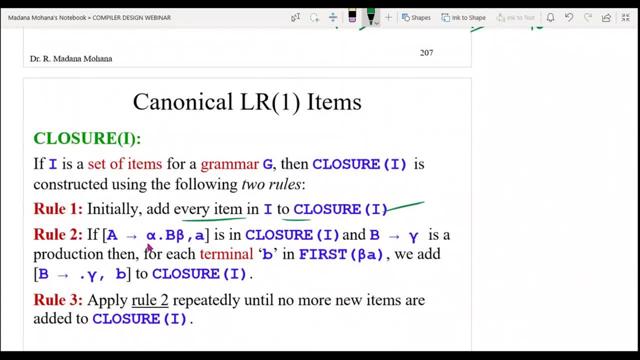 Now you can see, Initially, add every item in closer of I: A derived alpha, dot, B, beta, comma, A. So then, after dot, variable, B, B items you can add by putting dot in the right hand side beginning. So then, how to find out the lookahead symbol for these. 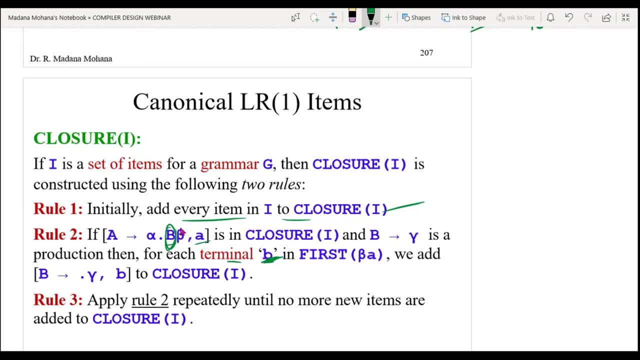 So for each terminal B, What is B After variable? whatever this one Lookahead symbol combination, You take first of beta A. You would add first of beta A as the lookahead symbol assume it as B, So here B equal to first of beta A. You know how to find first value. 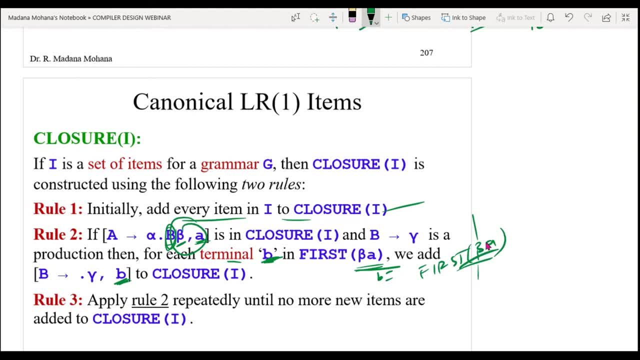 If it is terminal direct terminal value you can take. If it is not a terminal variable, it first value. you can find out like this: So whatever the B here, that is the lookahead, here that can be added to this one, Everything same, only finding the lookahead. 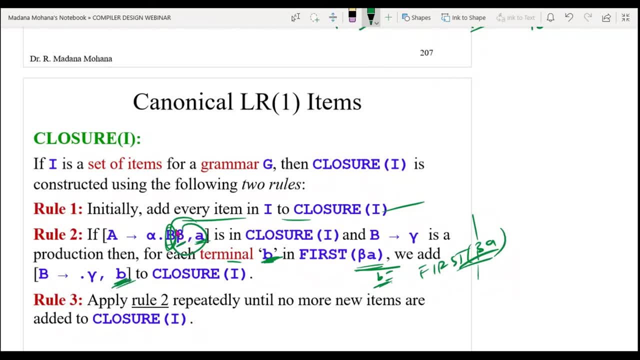 How to find the lookahead. first of beta A, Every time. first of beta A, you can consider: If beta A is null, also first of null. whatever this value, Then you will get this value only. Then apply this rule to repeatedly until no more new items are added. 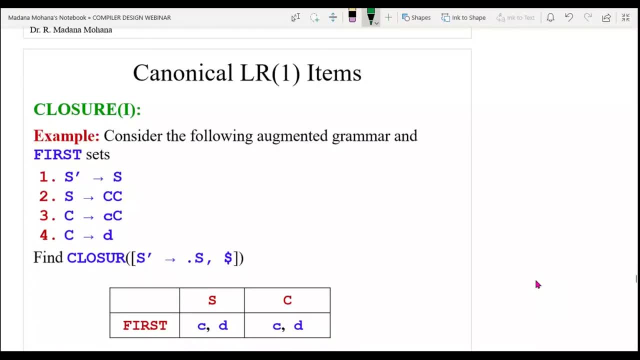 Then goto is also same. Now you can see, for example, This is one grammar S dash dash dot S. Initially, for the starting production item dollar, is added Lookahead. This is end marker, Default lookahead symbol, Default lookahead. So now 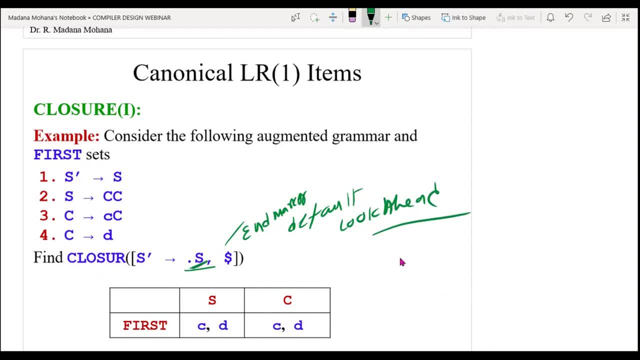 Now you are adding S items now. Now you can see S dash dot, S comma dollar. Now what are the S items? closure function: S contains dot CC. Now the lookahead you need to find out here: First of beta A, Now after S, this is beta. 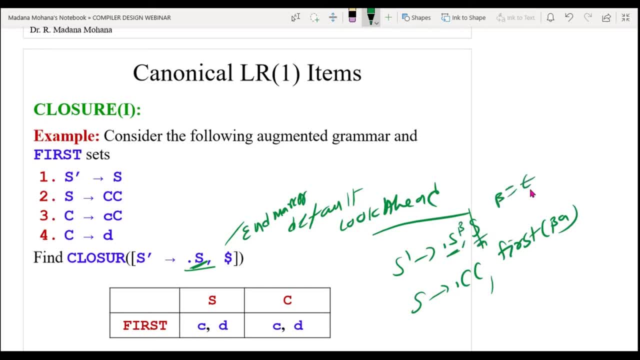 Dollar is A Here beta equal to null. Now, what you will get here. First of epsilon, A, Only epsilon means epsilon, you have to consider. But here, after epsilon, terminal, is there Whatever that you can consider? Then, first of A equal to A. 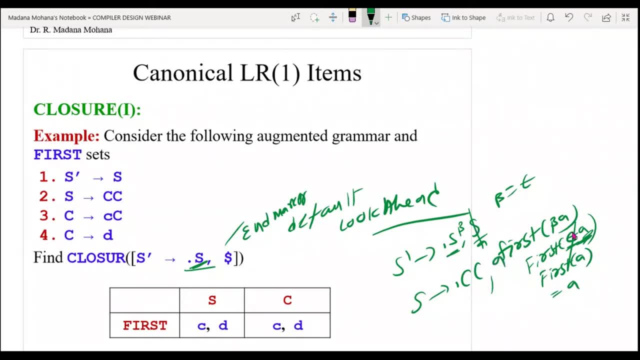 Now A is the lookahead symbol. A means dollar. So now dollar is the lookahead symbol. Now you can see S dash dot C, Variable C. Again, add C, item C. dash dot CC, C dash dot D For these two. how to find out lookahead symbol. 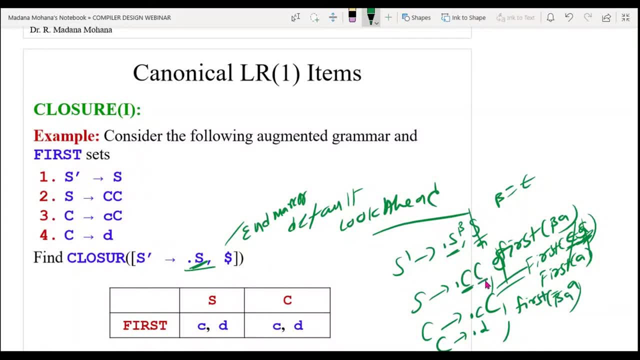 First of beta A. After C, whatever this one, This is capital C. So first of capital C, terminal A. What is first of C? Here we listed C comma D. Now you can see: First of C comma D, A. Now. first of C comma D. 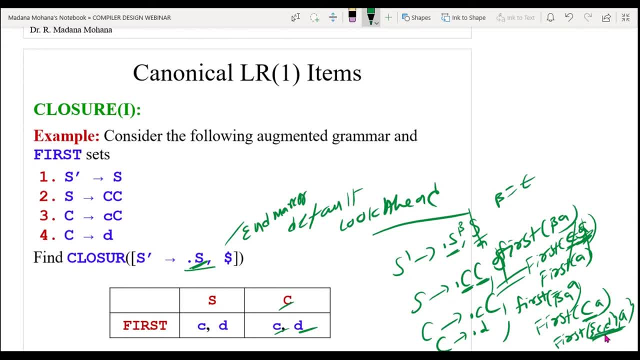 This is single. first of C value. Both you need to consider C or D First of terminal Terminal only. Okay, now Here you will get C or D added. See, this is same, Only lookahead symbols we are finding Using first of beta A every time. 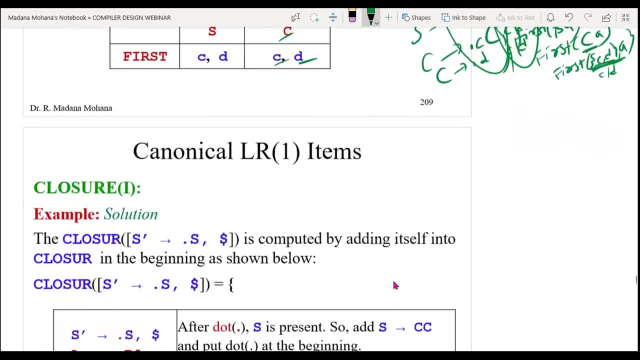 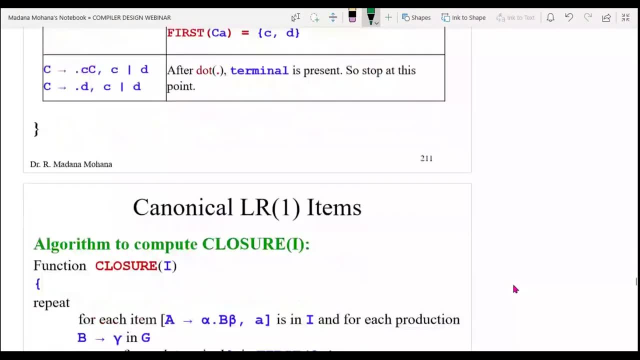 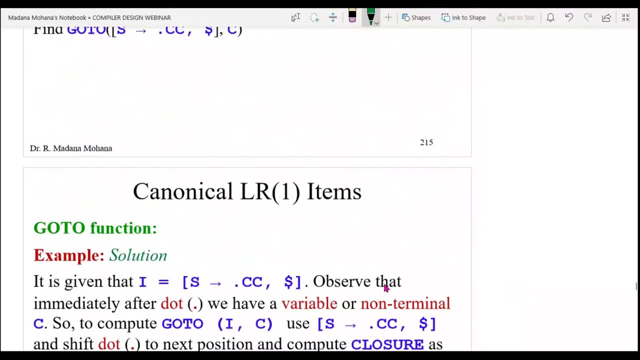 That is the only Remaining. all are same. So like that You can find out all the Closer values. Then go to value also: same Shifting dot over one symbol. Now directly Come to the problem. So in examination. 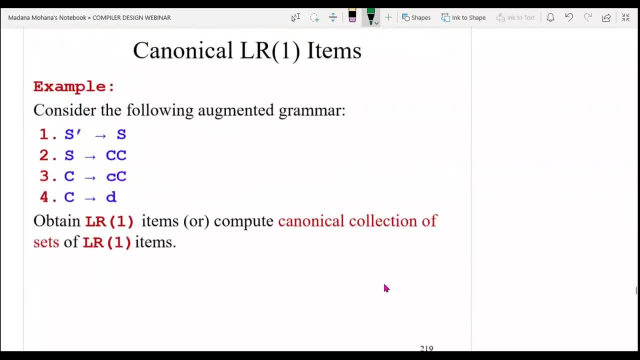 You will get the question like this For the given Augmented grammar Compute. L R 1 items are canonical collection of sets of L R 1 items. Here also you need to consider augmented grammar Here. we already Given augmented grammar only. 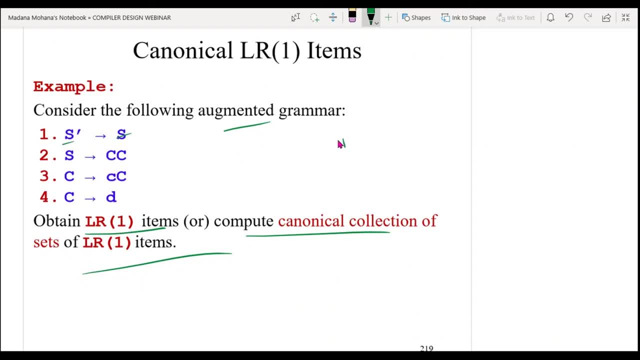 S dash not occurred anywhere in the right hand side. Okay now First I not how to find out S dash derivatives. dot S comma, dollar Default: you can add Only for this Now dot S S items. you can add S derivatives: dot C, C. 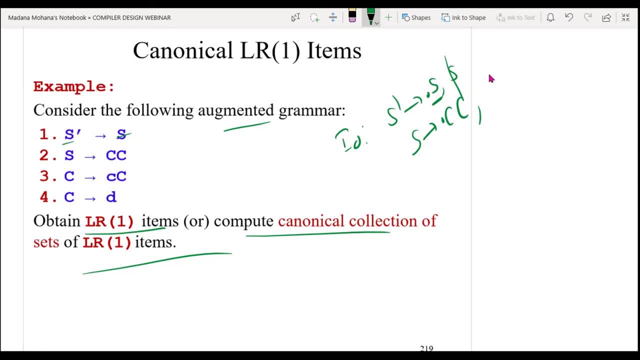 Here First of beta dollar. Beta is null. Now dollar will come. So dollar Now Here C items. He derives These two productions by putting Dot Dot, Terminal C, variable C. It is Dot D. Now the look at. 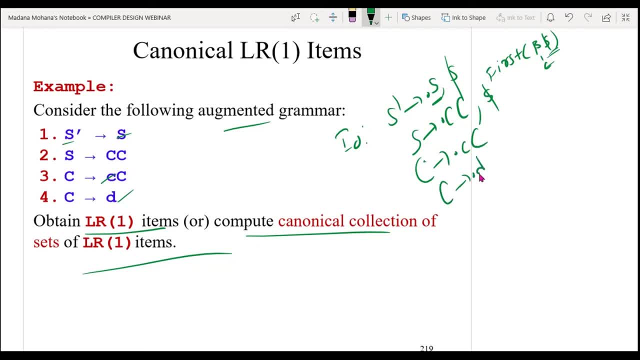 Here First of Beta A. Beta is capital C, A, A stop capital C. We already calculated C comma D. The same items Will come Now Here First of Beta A. So Same items will come. 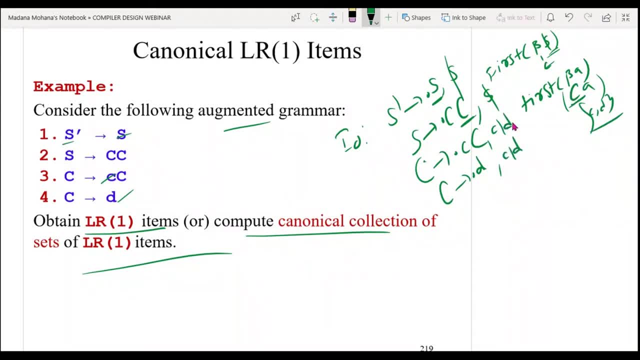 CRD, CRD. Why? Because First of C contains two values, All values We have to consider here Now. This is initial item. Then I want how to find out Further. See Dot Small C. 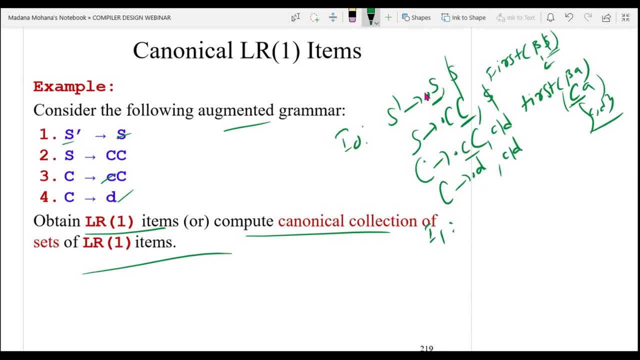 Terminal: No new items are added. Dot D- Small D Terminal. No new items are added. Now move Dot Over one symbol at a time. Now Only one time. Dot Before: Yes, Now This will become. 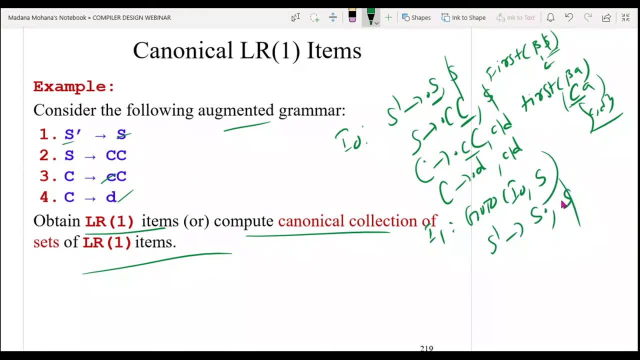 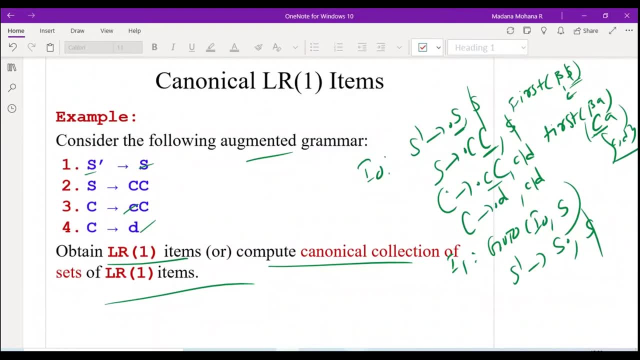 Yes, Yes, Dot. By default, The same Look ahead Will come Whenever New items are added. You can find out. Ok, Like this. Now You can Find out. This Is If You. 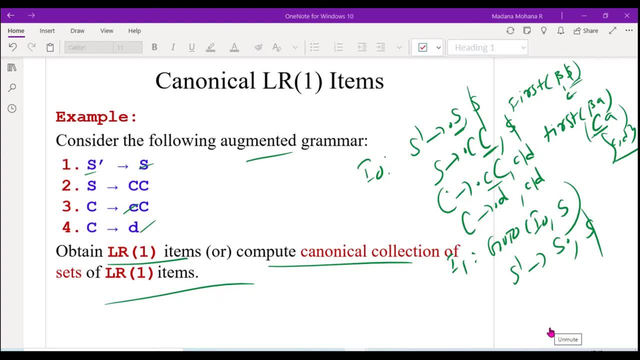 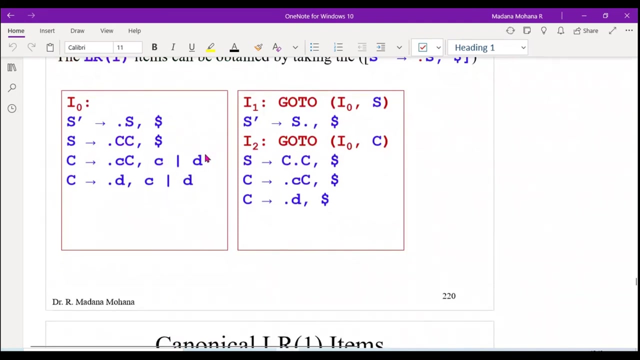 Do You Have Like this, And this Will be Even Soon, So You Don't Have Too Any Time Now You will Find Out Once all the items the same as lr0, only every time the lookouts are added here. also, you can consider. 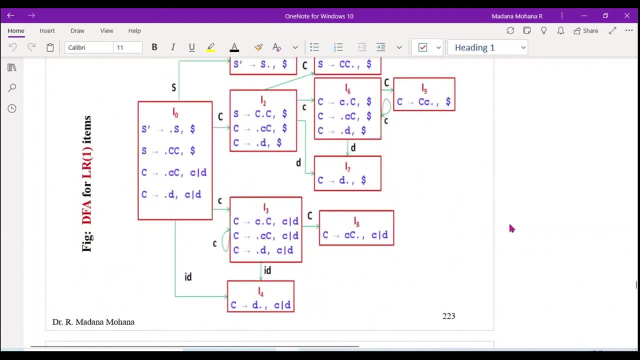 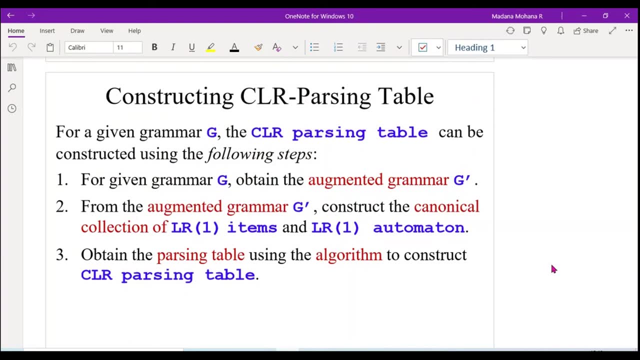 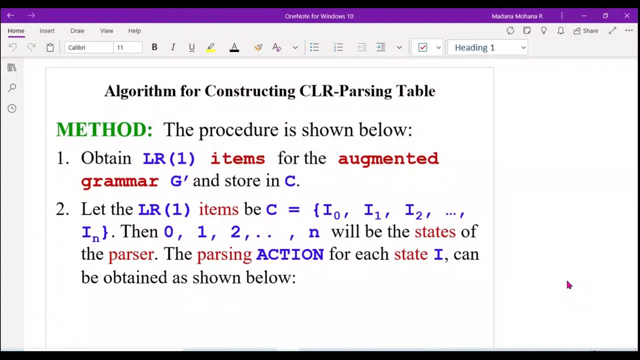 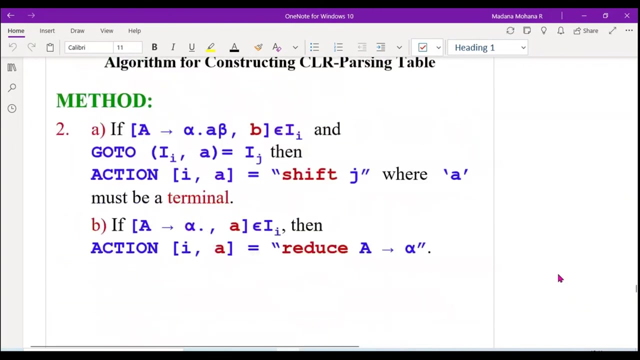 unique items only. this is the dfa for same same as lr0. now construction of the clr parsing table. also everything same. that's why, once you will get clarity on slr parsing table, remaining clr, lalr, similar, only lr1 items are there now here also you can see, but here 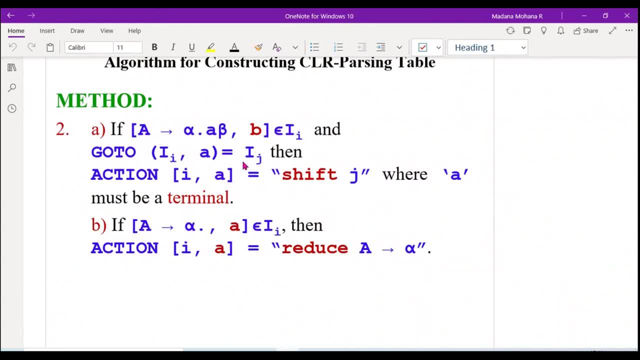 one difference you need after in rule two: here we no need to find follow value. we no need to find follow value why? because here the look ahead symbols are there. in place of follow, we will use look ahead symbols. now see to a rule. a derives alpha dot terminal. 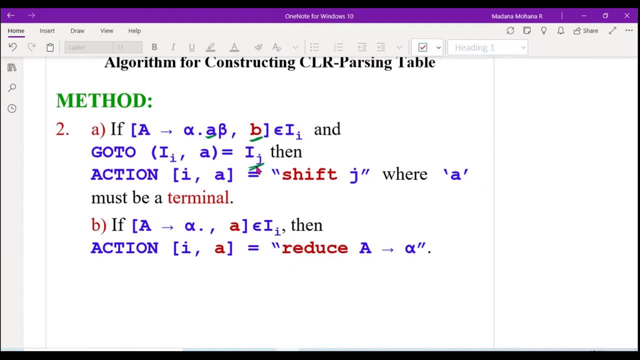 comma b now goto of ia and a equal to ij. here you can see action of i comma a, shift j. the same terminal is used here for completed item a derives alpha dot. actually in completed item fall of a we have obtained in slr parser a not required directly. look ahead, is there? 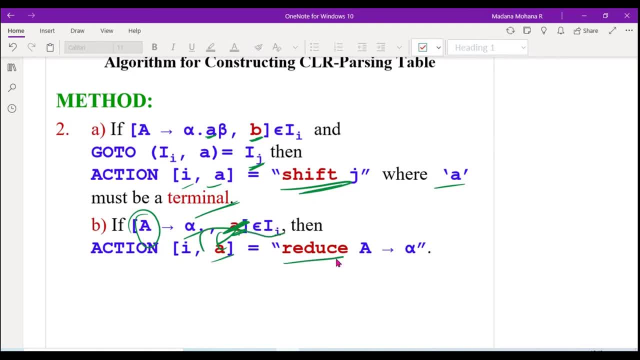 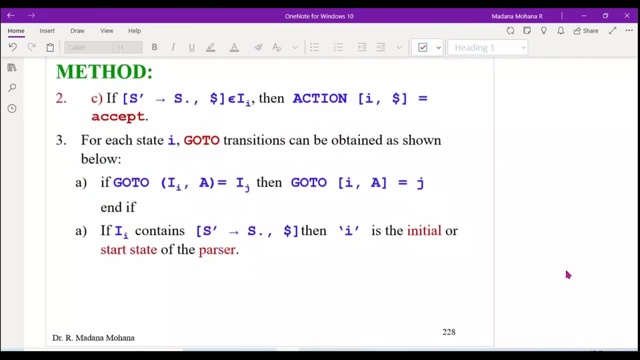 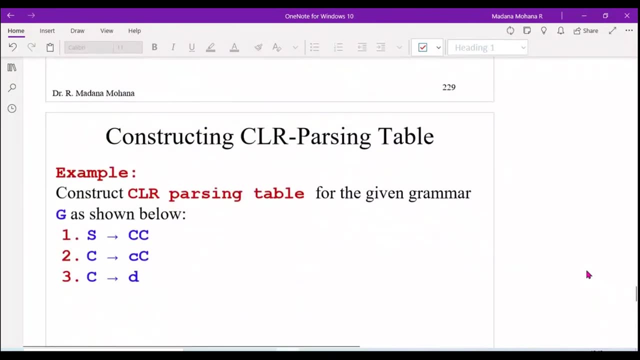 so same value can use here here i comma a equal to reduce my production number. that is the only difference remaining. all are same. remaining, all are same, no changes. only in case of completed item follow value we can take look ahead symbol. that is the only difference. now the question: constructs real or parsing? 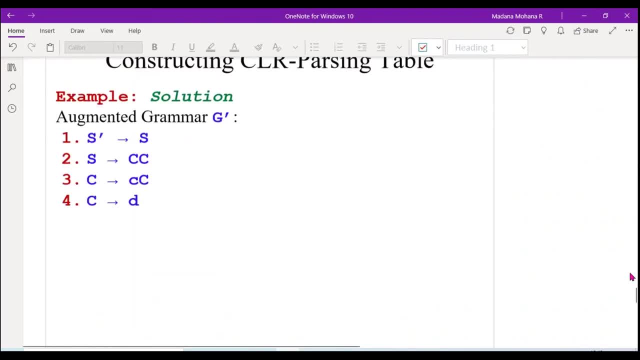 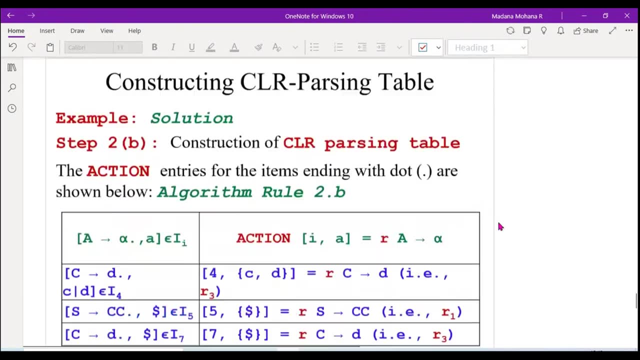 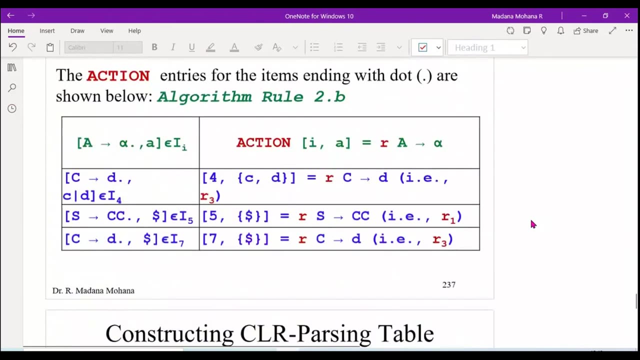 table for the grammar the same. first you need to find out augmented grammar, then all the rules. now you can see using the same rules only in case of completed item. here you can see, here we are not finding follow value directly, we are taking the look ahead value. now it. 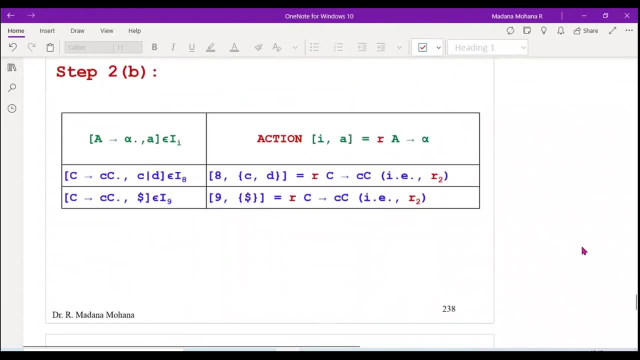 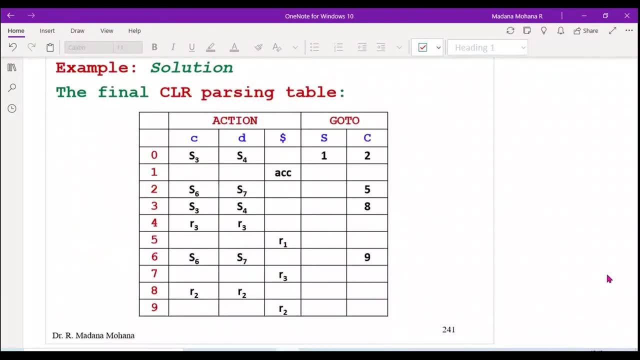 is easy comparing to slr here. no need to find out follow value, then nothing is new remaining. all are same. now you can see action go to part. the same here also. if multiple entries are there, there is not clr one. if no multiple entries, then that is clr one. parser now see the look. 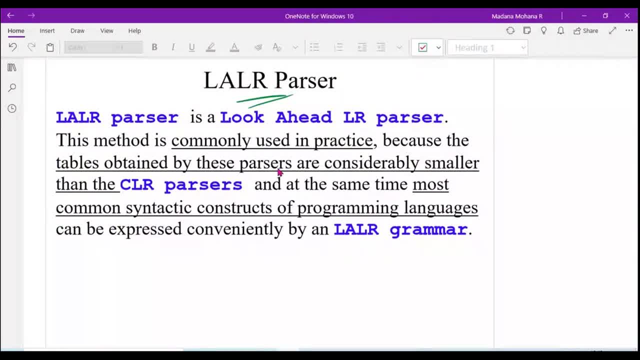 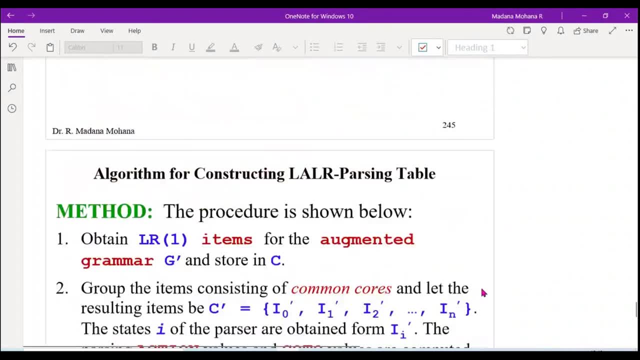 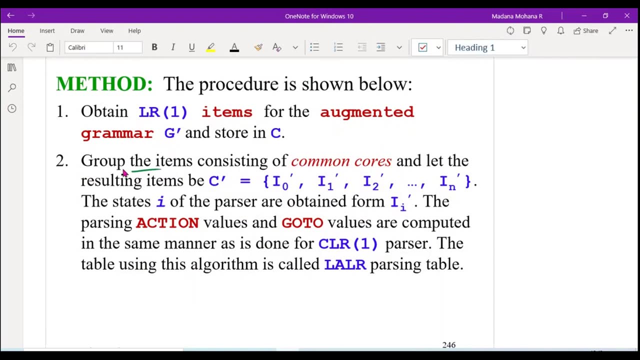 lalr parser. here, lalr parser, what you will do? everything same as clr parser, only in lr one items, the common cores, are merged. here you can see the items consisting of common cores. what is the meaning of common core? for example, you are having c d s, dot c, c, c d s, dot d. you are having dollar, for example. this is i one, i one item. 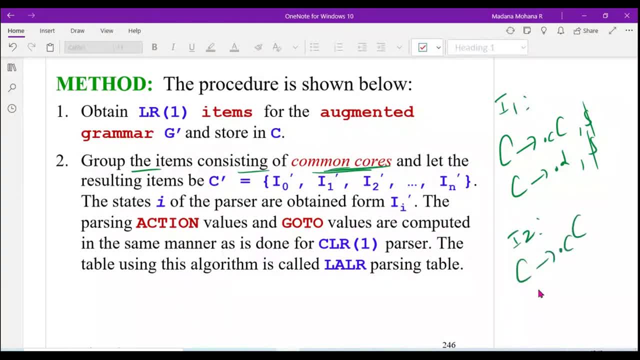 then i two item is like this: c d s, dot c, c, c d s, dot d. see, the items are same but the look aides are different. now these two are merged. you can make it as new item i one two match c d s, dot, c, c. the look ahead first one, then the second look ahead dollar r, c, r, d then. 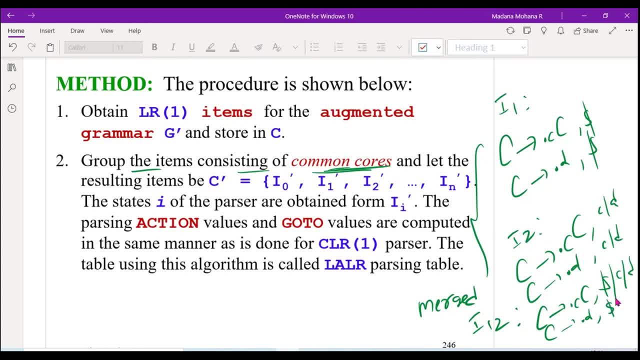 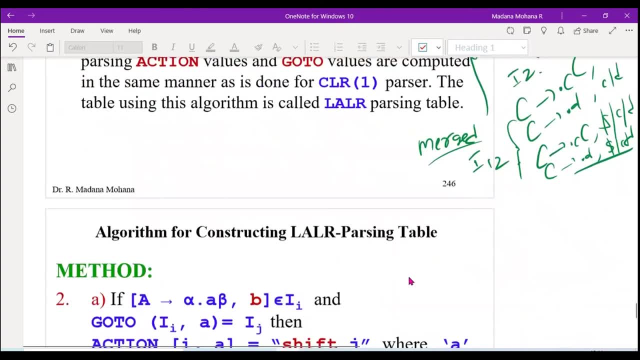 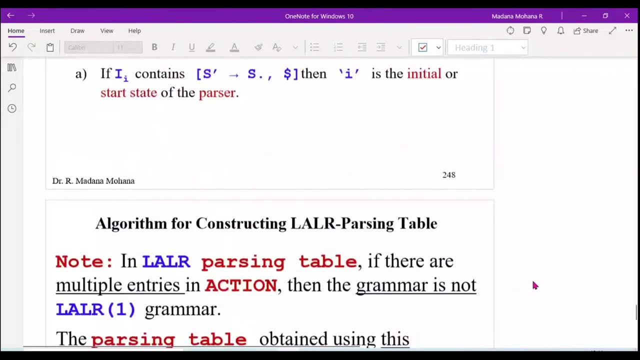 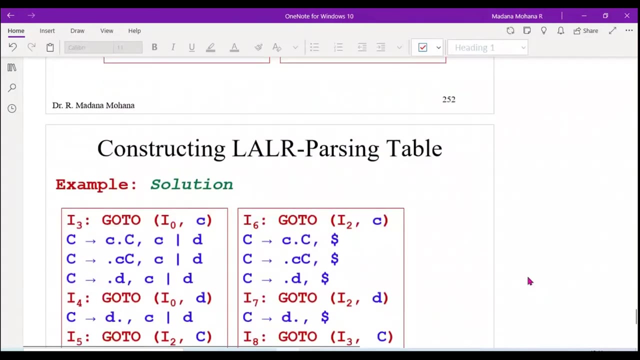 c, d, s, dot, d, dollar, r, c, r, d. this is the only difference remaining. everything same. here some items are merged. that means reduced. that is the only difference remaining. everything same at clr parser only. that is the only difference in lalr parser. now, in our previous example, let us see what are the items having common cores now here: 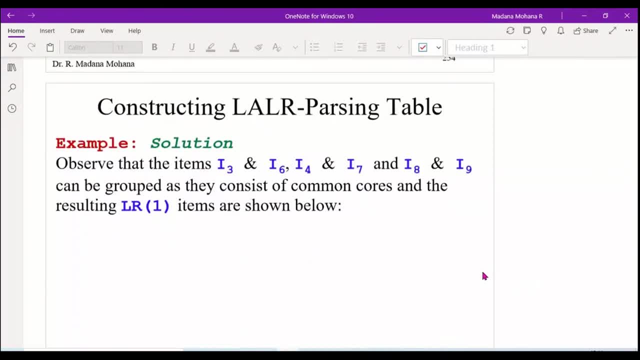 you can see. so in the above l r one items: i three, i six. items are same, look, aedes are different. you can combine these two, i four and i seven. these two can combine i eight and i nine. equal. combine now i naughty one, i two, now i three means i three, six, i four. 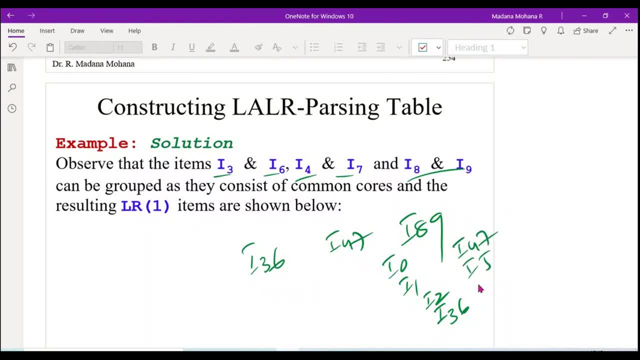 I4 means I47, then I5, I6- already merged. don't take I6, I7- already merged. I8 means I9, so then I10, not there, then I11, now these are all the unique items, the same algorithm. 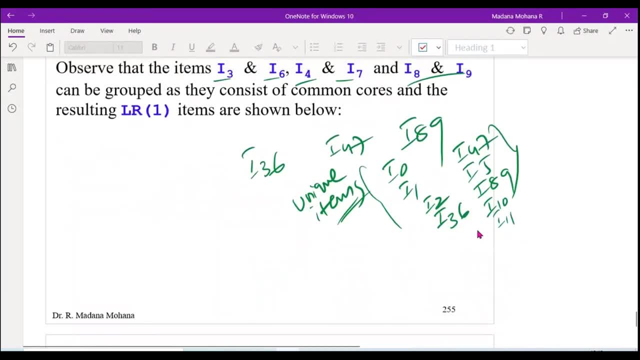 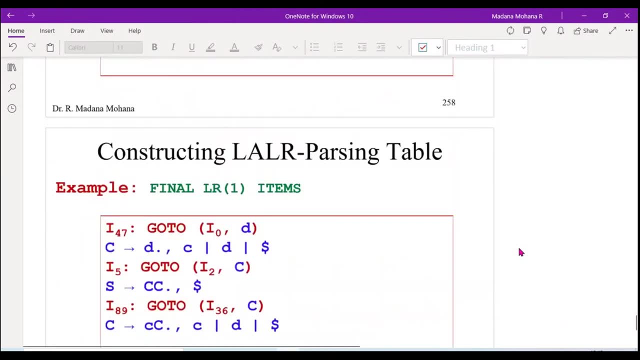 you can use. now you can construct its table. look at parsing table how you can see same is used here. here you can see 3 and 6 are merged, 4 and 7,, 8 and 9 are merged. so the 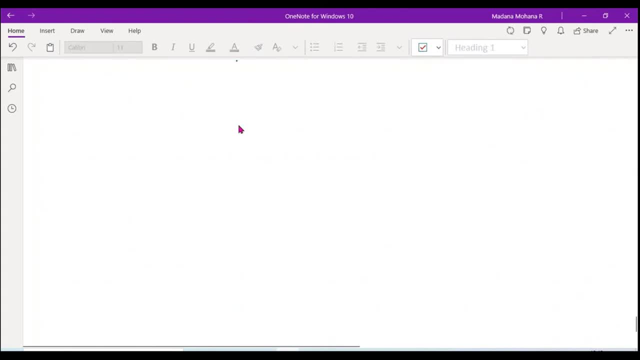 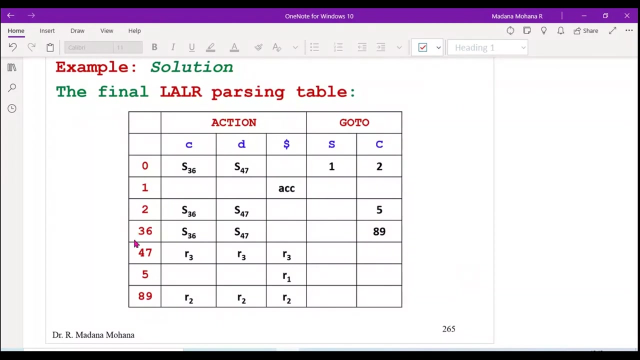 table construction. everything same. now you can see. this is the table here. now states: you can observe the states are merged: 3 and 6 are merged. 4 and 7 are merged. 8 and 9 are merged. there are shift values also. suppose you may get S3 means don't take S3. 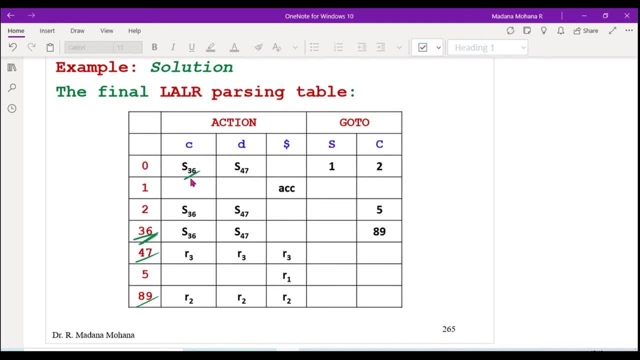 separately. whatever the combination state that only you can take 3 states. S4 means don't take S4 separately. the 4, 7 combination state you can take like this. so whatever here the state the action values are combination of the same, only it will go to also so here. 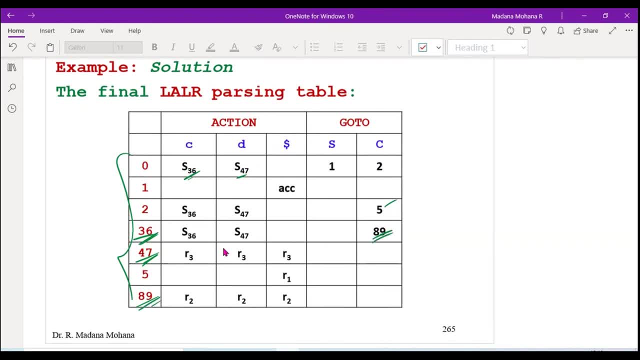 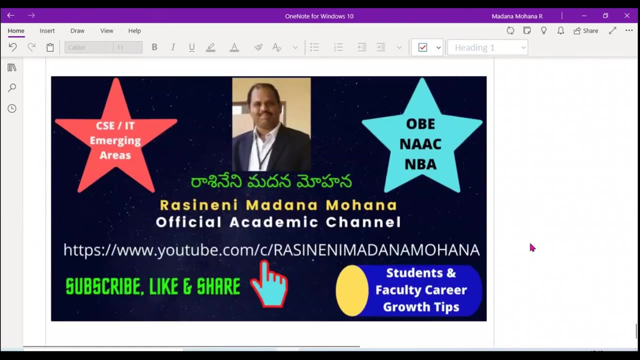 8 means we don't have 8 separately. 8,, 9,- here also, multiple entries are not there now. this is LA LR1 parser. like that you can find LALR parser easily. that's all about the LR parser. the. 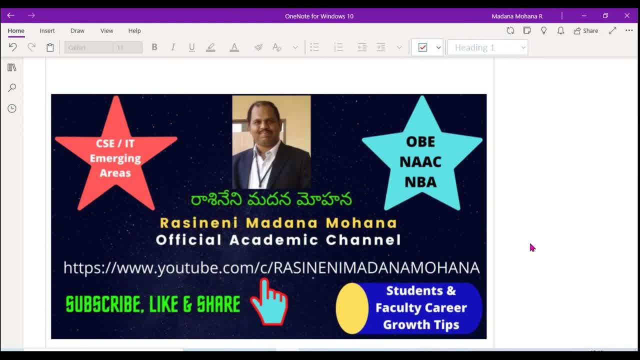 3 techniques: simple LR, canonical LR, look ahead- LR. with this now I am closing. so if you have any queries, you can ask now, because in the entire of compiler design course the problems will be from the second device. So what you need, that is parser, only top down parsing, predictive parser, LL1 parser. 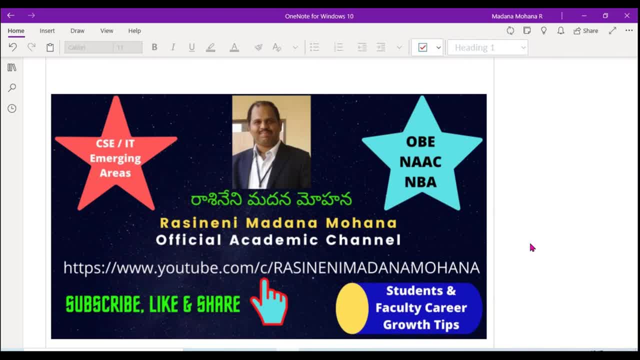 one problem: bottom up, parsing either SLR, CLR, LALR. remaining all are very easy topics. don't bother about any other topics, all are simple, just some procedure. examples like that only.